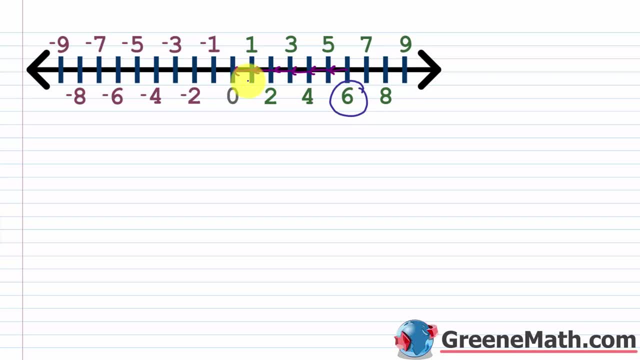 So the absolute value of six is just six. Now, similarly, if we looked at negative six, you'd find that it has the exact same absolute value. We start here and we go one, two, three, four, five, six units to the right to get to zero. So this leads us to an important concept. 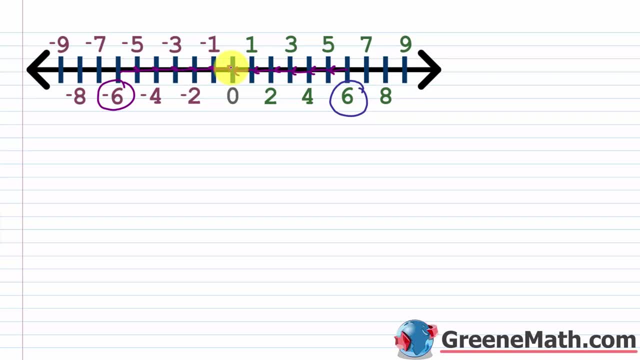 Two numbers that lie on the opposite side of the number line with the same absolute value are known as opposites. So we've talked about opposites before. So six and negative six would be opposites. Three and negative three would be opposites. Four and negative four. 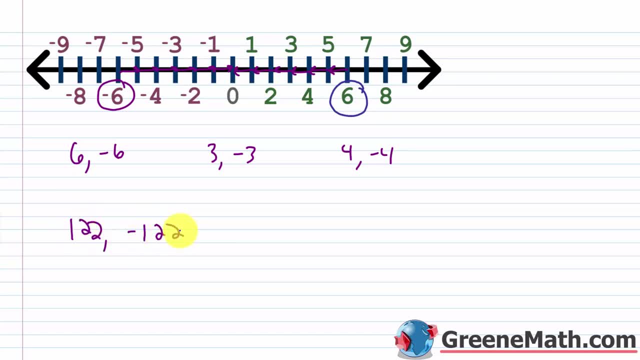 122 and negative 122. You know so, on and so forth. So let's take that as one. So if I were to go to on and so forth. One important property here- and we talked about this in a previous review session- if you add two opposites together, you get a result of zero. Think about adding. 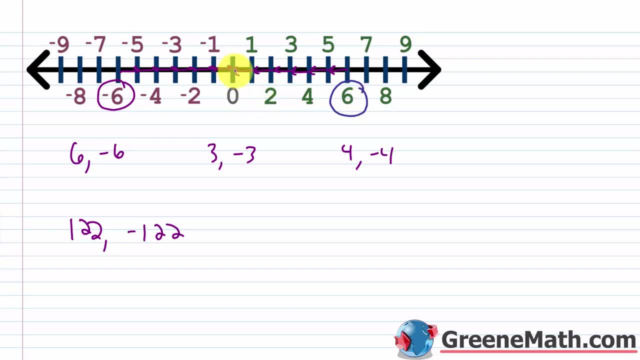 negative: six and six. Well, if I started at zero and I went six units to the left and then I went six units to the right, I'd end up back at zero. It's because their weight or absolute value is going to cancel each other out. right One is negative, one is. 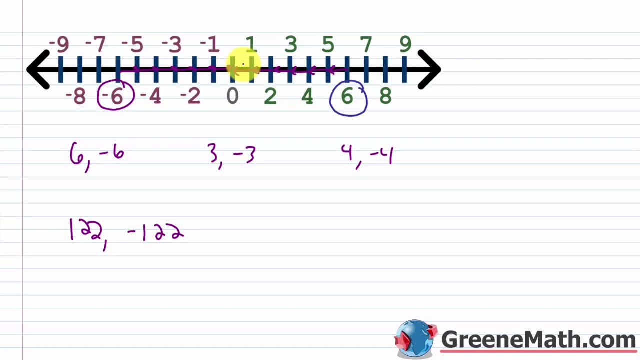 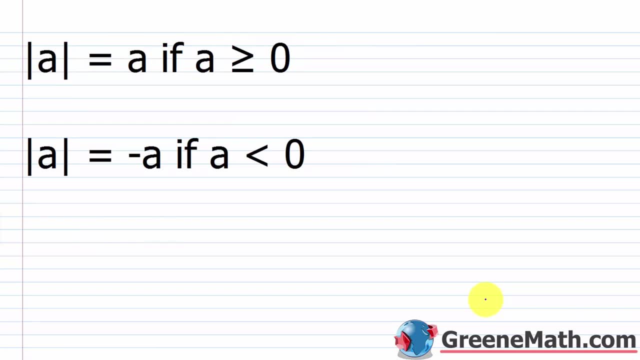 positive. they have the same absolute value, so they cancel and they end up in the middle, which is at zero. So in general, we don't need to pull out a number line every time we want to find the absolute value. We can follow a very, very simple rule: The absolute. 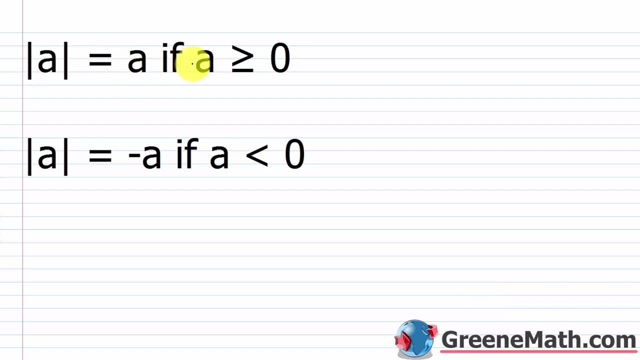 value of some real number, A is just A. if A is non-negative, meaning A is greater than or equal to zero. So if you have zero or some positive number, you take the absolute value. it's just the number. So in our example we took the absolute value. 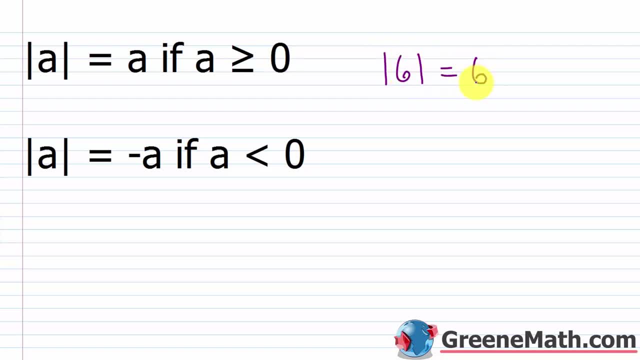 of six. it was just six, right? You just use the number, The absolute value of some real number. A is the opposite or the negative of A if A is less than zero. So if I had something like the absolute value of negative six, this would be equal to the opposite of negative. 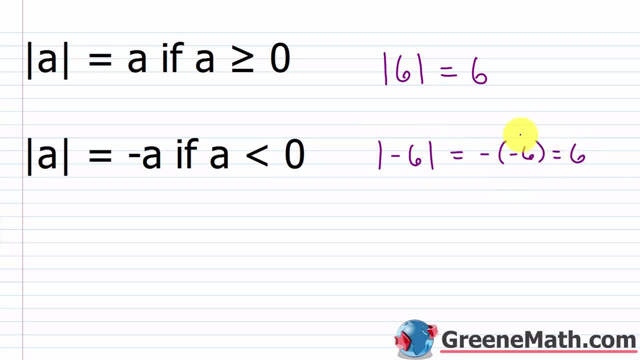 six, which is just six, right, You don't even need to go through all this. Just know that if you take the absolute value of something that's negative, you just make it positive, right? So if I had the absolute value of negative 122, that would be the absolute value of negative. 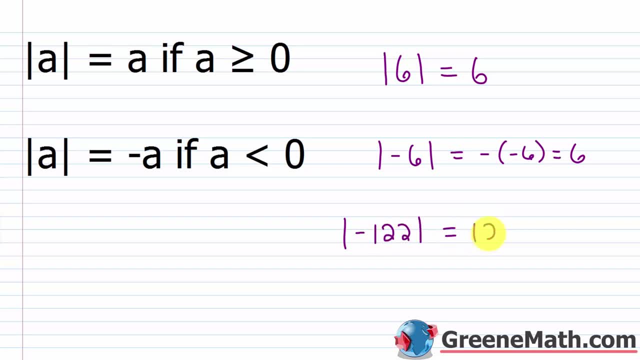 122.. I would just make the number positive. I know this is 122.. Similarly, if I had the absolute value of, let's say, negative 1,322,515,, what would I do? I would just make the number. 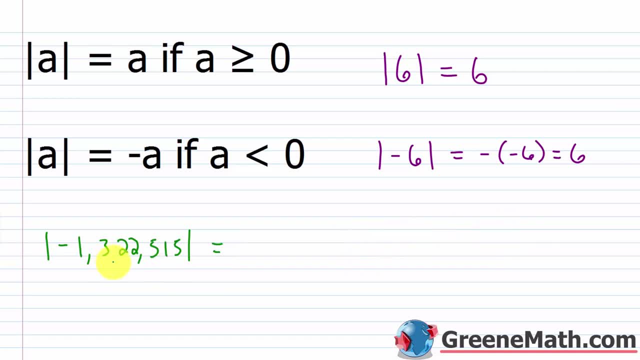 positive. Let me kind of erase this to get a little room. So I would just take this number and say: okay, it's 1,322,515,. right, Just make it positive. So if it's zero or a positive number, it's just the number. If it's a negative number, 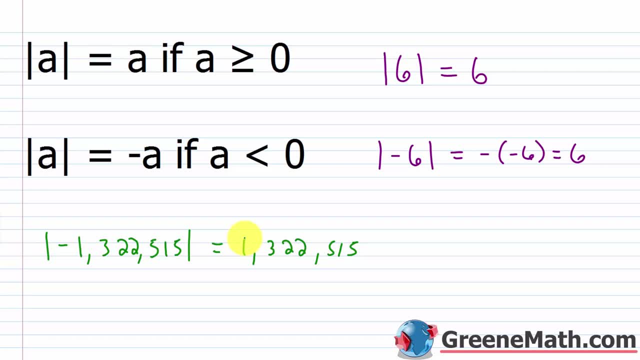 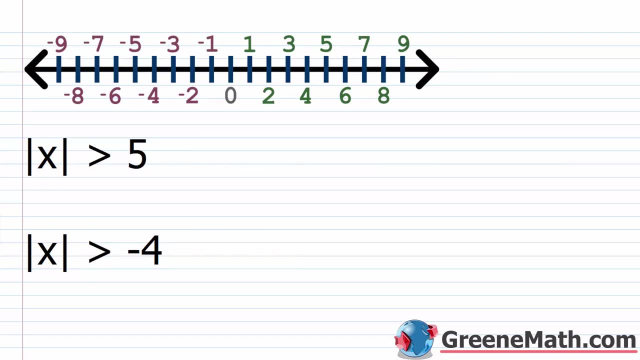 just make it positive. okay, That's all you really need to remember about finding the absolute value of a number. It's very, very simple, All right. so now let's think a little bit deeper about the concept of absolute value, especially in terms of what we're going to see in this course. We think about a statement. 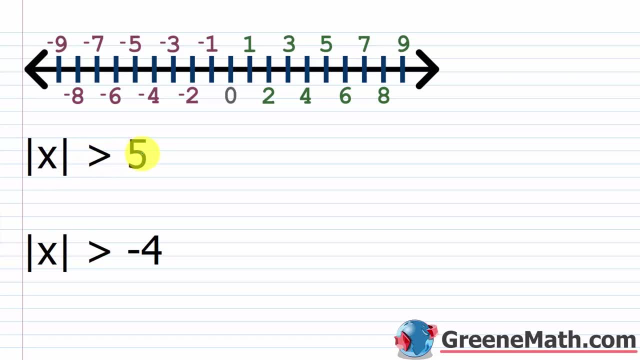 such as the absolute value of x is greater than 5.. So what does this mean? Let's break this down so that you can understand it. The absolute value of a number, again, is the distance from the number to zero on the x-axis. 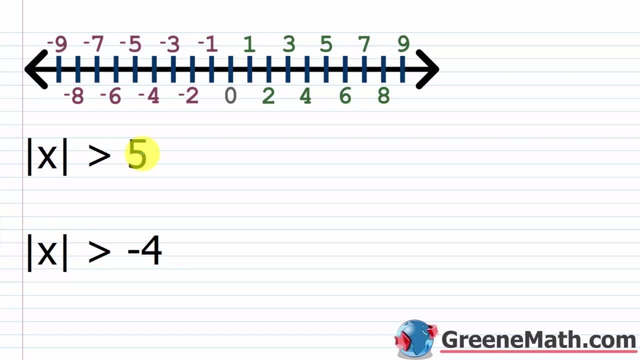 Let's break this down so that you can understand it. The absolute value of a number again is the distance from the number to zero on the number line. So what this is saying right here is any number here that has a distance from zero that is larger or greater than 5,. 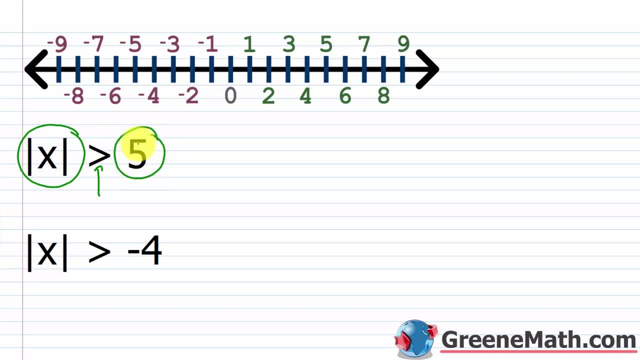 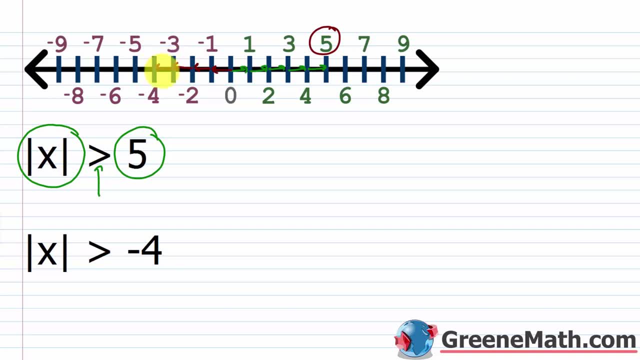 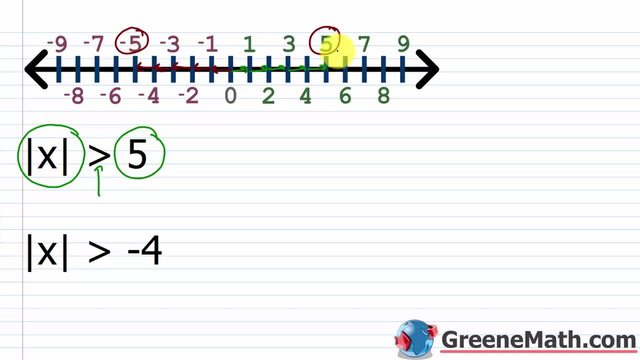 does that tell me? Well, x could be anything larger than 5.. We know from interval notation that we can kind of mark this this way. We could put a parenthesis here to say that 5 is not included, and I could shade everything to the right And x could be anything less. 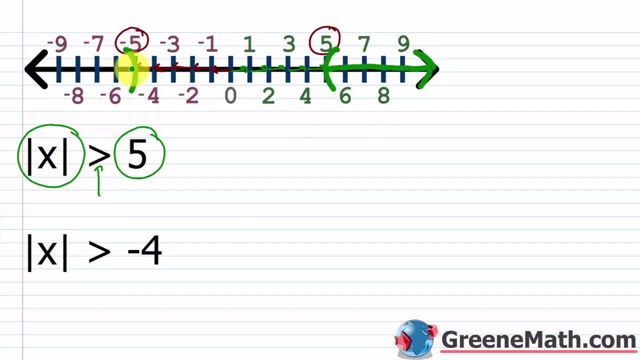 than negative 5.. So I could put a parenthesis at negative 5 facing to the left, and I could everything to the left, like this right. so anything in between here, so from five to negative five, with five and negative five included, would not work, because in those situations the values would not. 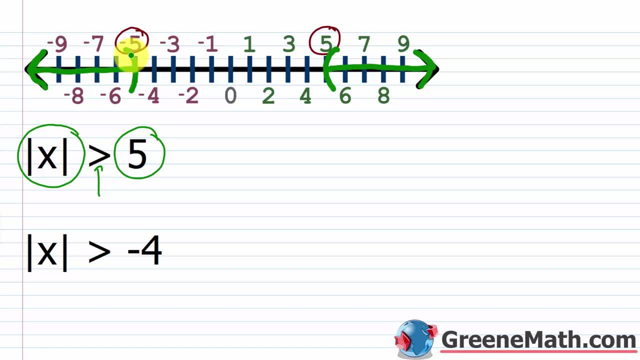 have a distance from zero that is larger than five. so as an example, let's say i took negative one. if i plug that in for x, what would i get? so the absolute value of negative one is that greater than five? no, the absolute value of negative one is what i just told you. if you have a negative, 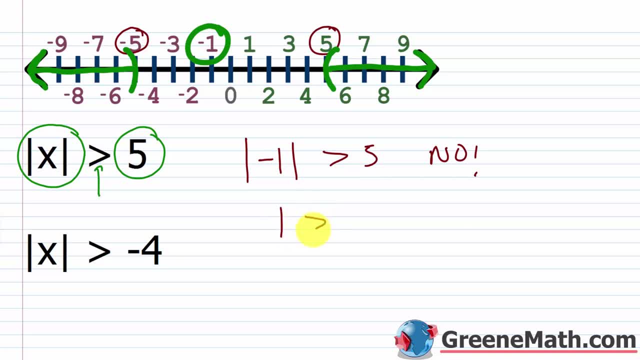 number just make it positive. so this evaluates to: one is greater than five, which is false. one is not greater than five. if i plug five in there, the absolute value of five is five. five is not greater than five. that doesn't work. i plug in negative five: the absolute value of negative five is five. 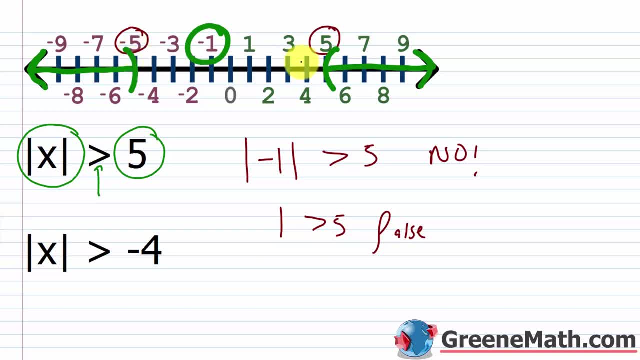 five is not greater than five. that doesn't work. so all these numbers in between here don't work. but if i chose something that is to the right of five or to the left of negative five, that would work. if i chose seven, for example. let's see what happens. 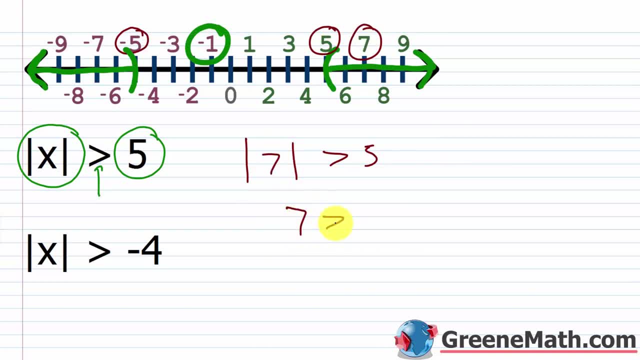 there, the absolute value of seven is seven. seven is greater than five. so we're good. if i chose, let's say negative nine. okay, let's say negative nine. the absolute value of negative nine is nine. nine is greater than five, so that works. so if we wanted to write our solution, we could say that x could be. 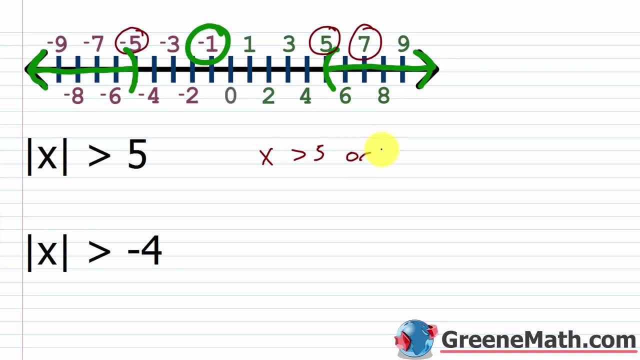 anything larger than five. so we could say that x could be anything larger than five, or- okay, you use the or statement here- x could be anything that is less than negative five. either situation would work. in interval notation we would use our union symbol, so we would have 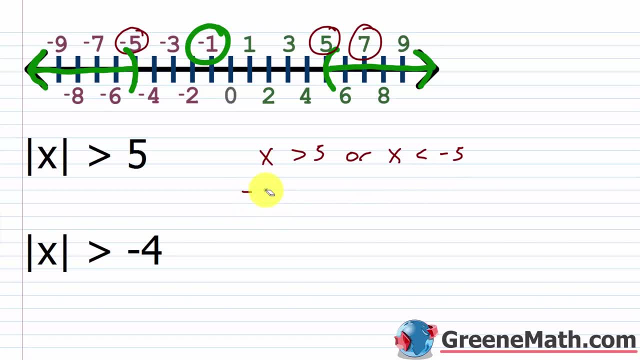 the interval from negative infinity- let me make that symbol better- up to, but not including, negative five, and it's this set and we're going to have a union with this set. so anything large than five, again out to positive infinity. so this is how you would write it, kind of using the standard. 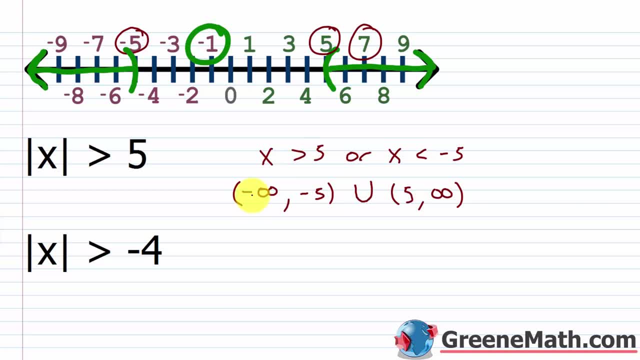 notation, where you know you're using inequality symbols, and this is how you would write it using interval notation. this is how you could display this graphically. now let's think about the other scenario we have here. this is kind of a trick question, so, before i even read it, why don't you? 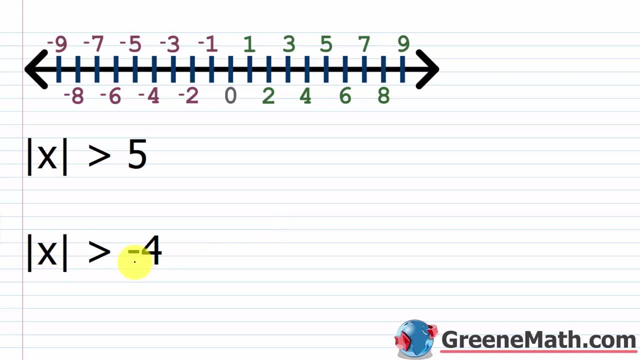 see if you can think about this one on your own. so i assume you tried this and hopefully you figured out that this is the right way to do it. so let's see if you can think about this one on your own. this is again a trap. if you see this on a test, you should be able to answer right away. all real. 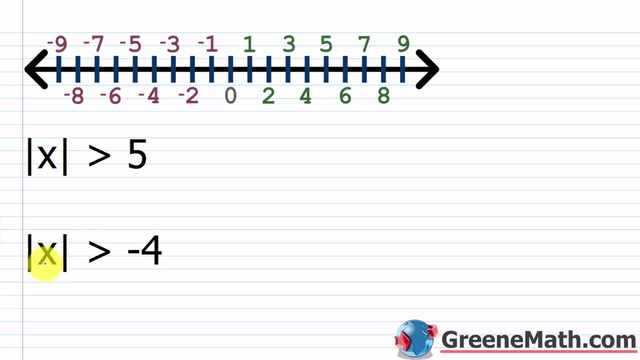 numbers. why is that the case? well, the absolute value of x is greater than negative four. okay, let's think about that again. give me a number here that you take the absolute value of it and it's larger than negative four. well, it doesn't matter what i plug in there. if i plugged in a 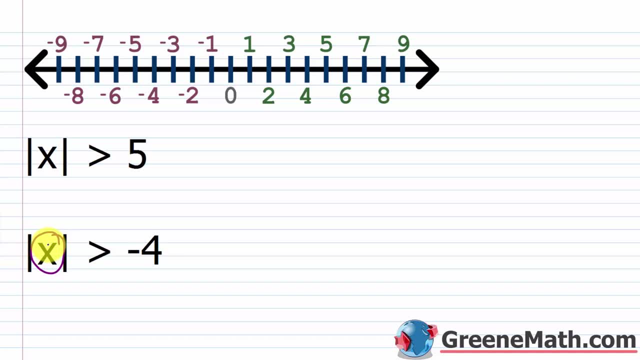 negative number, the absolute value would make it positive. okay, if i plugged in zero, the absolute value would make it zero. so if i plugged in zero, the absolute value would make it zero. if i plugged in a positive number, it would keep it positive. so anything i plug in is always going. 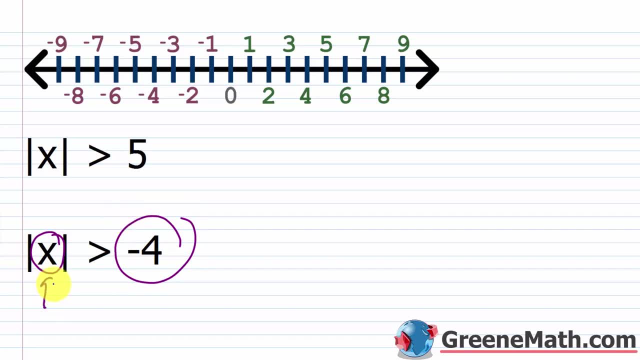 to be greater than negative 4, because the smallest this can be is: if x is zero, so the absolute value of zero is zero, so zero is automatically greater than negative four, and that's as small as this can be using the absolute value operation. okay, again if i plugged in something. 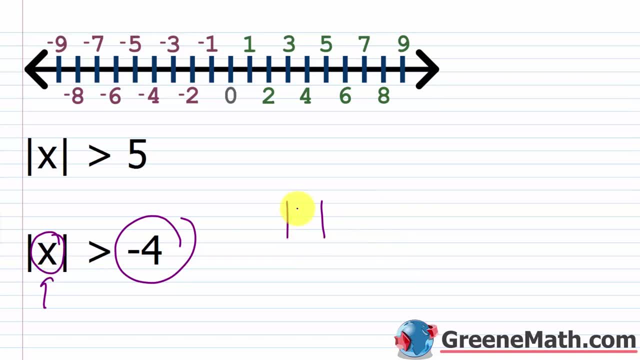 negative. let's say i plugged in negative six there the absolute value of negative six is six. six is larger than negative four. so you see that no matter what I plug in for X, it would work. so we say all real numbers. okay, you could say it like that. 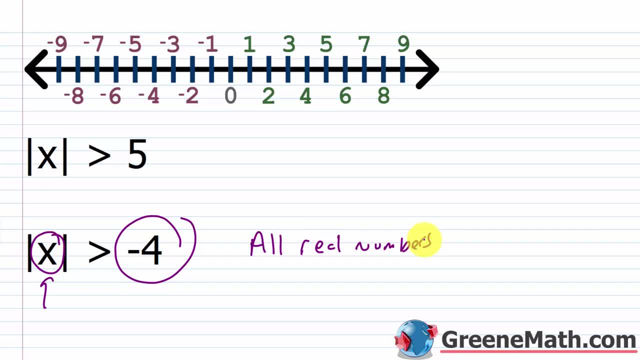 you could do all kinds of different ways to notate this. you could say you know the interval from negative infinity to positive infinity. you could shave the entire number line graphically. all right, you could take and just shave this entire thing to show that any real number on the real number line would be. 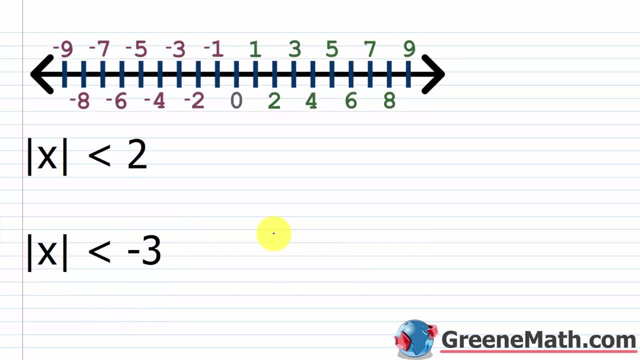 a solution for your inequality here. all right, so let's look at the other scenario here. so we start out with: the absolute value of X is less than 2. so again, when I think about X, it's it's gonna be any value whose absolute value or distance from 0 is smaller or less than 2. so if I started at 0 and I went, 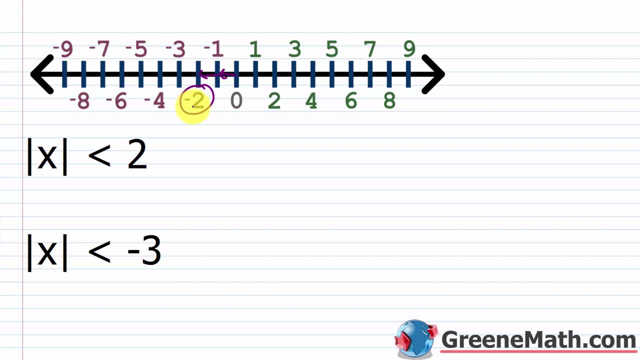 1 and then 2. so it couldn't be negative 2, right, it couldn't be negative 2, because it can't actually go. 2 units got any less than that. so let's kind of notate this by putting a parenthesis at negative 2 facing to the right. and I could do the same thing. I. 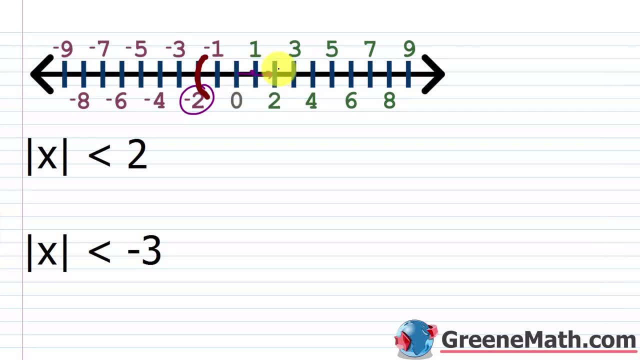 could travel 1, 2 can't quite be 2, so I'm gonna put a parenthesis here. face into the left and you just shade everything in between. so essentially, what I have here is a scenario where X can be any number that's between negative 2 & 2. 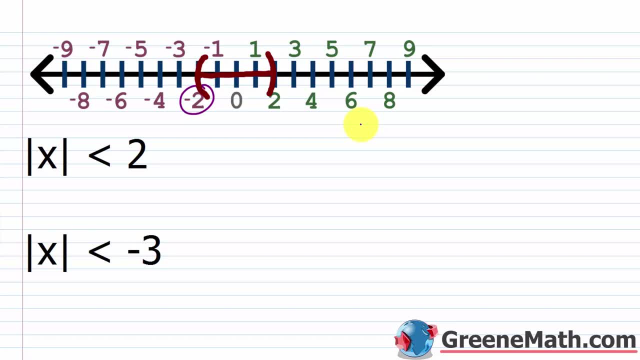 with negative 2 & 2 is opposite, so that's where I can go and I can get the two not included, right? So an interval notation, that's the interval from negative two to two. Again, neither is included, So I use a parenthesis at each end And you can try this out with. 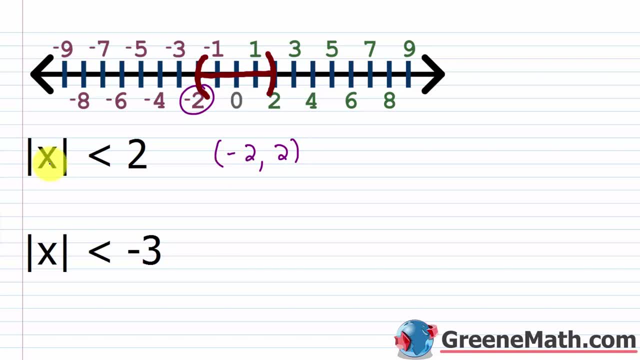 let's say the number negative one. So you plug in a negative one there. the absolute value of negative one is one. So you would have that one is less than two, which is true If you tried something outside of this range here. let's say you tried three. the absolute value of three is: 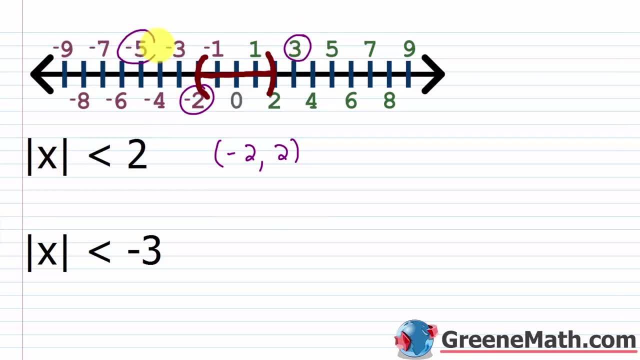 three. three is not less than two. So that doesn't work. If you tried, let's say negative five. the absolute value of negative five is five. five is not less than two. So again, you've got to be within this range here to have an absolute value or a distance from zero. 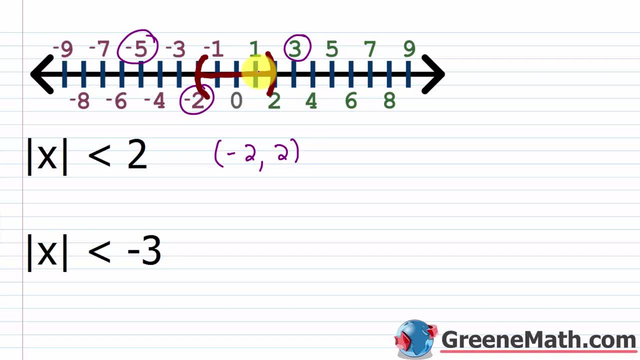 that is smaller than two. So that's your solution there, And you could also write this as: x is greater than negative two and less than two. Okay, so kind of three different ways to show the solution. All right, let's think about another one. And again, I advise you to kind of stop the video. 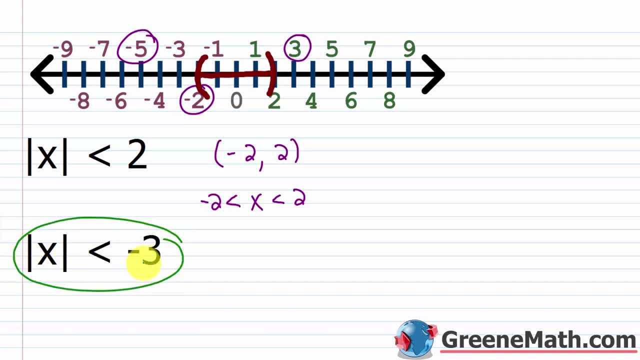 here And think about this, what's going on here? because I'm going to tell you in advance is a trick one, All right, so I assume you tried this and you would see that there's no solution. And why is there no solution Again? x represents a number whose absolute value is less than 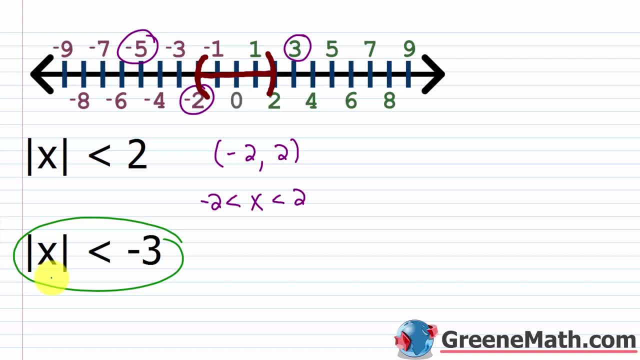 negative three. Can absolute value be negative? Just think about that for a second. Can it be negative? No, it has to be either zero, if you're plugging in zero, or negative three, Or positive. If I plug in a negative, I get a positive. If I plug in a zero, I get a zero. If I 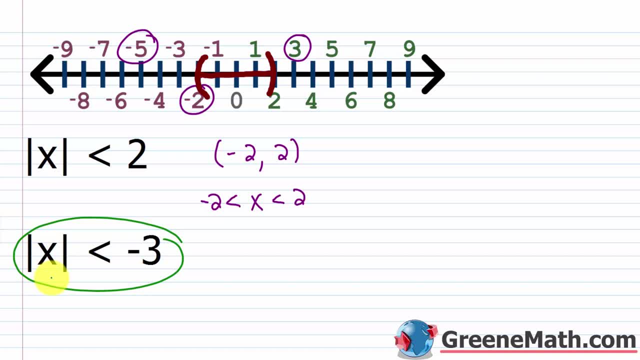 plug in a positive, I get a positive. So there's no way that the absolute value of something can be less than negative three. It's not possible. It has to be zero or larger. So there's no solution here. There's no solution. Okay, you can write no solution, Or a lot of teachers will say: make. 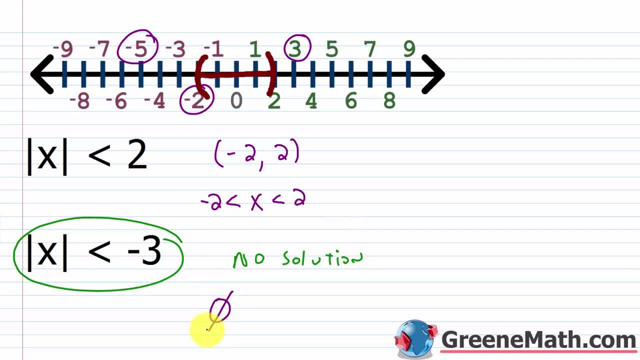 the symbol for the null or empty set, because the solution set here has no elements. And again, if I'm going over here I'm going to say zero, And if I plug in a negative I get a positive. So there's no way that the absolute value of something can be less than negative. three: 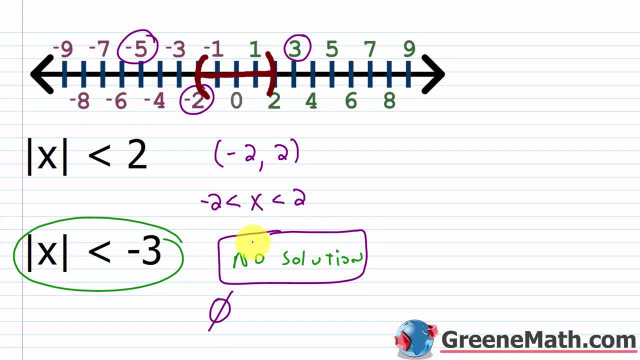 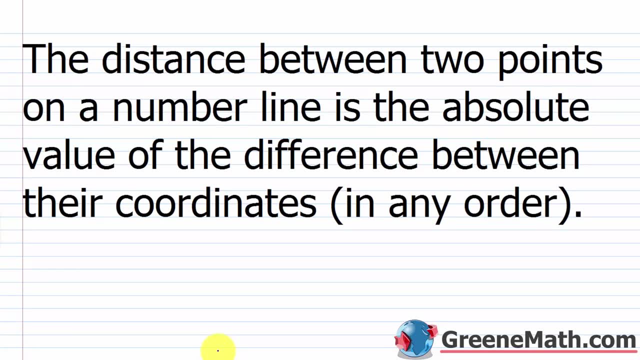 Just write: no solution. That's all you really need for the majority of the classes. So the last thing we want to think about in this lesson on absolute value is how to find the distance between two points on a number line. So this is a very, very easy thing to do, And we 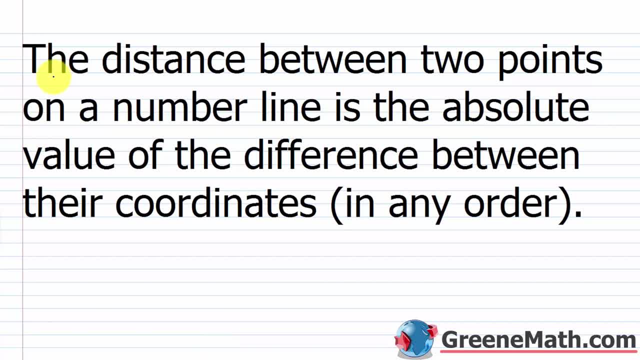 have a very simple formula that we'll see in a second. So the distance between two points on a number line is the absolute value of the difference between their coordinates, in any order. So in other words, if I wanted to find the distance between, let's say, six and let's say negative, 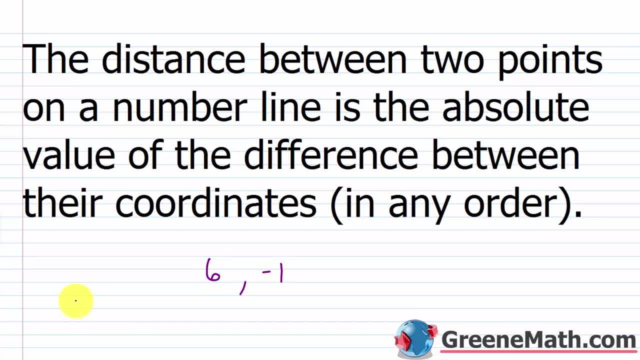 one. Well, what this is telling me is that I can say: the absolute value of six minus a negative one would give me the distance between the two. So six minus a negative one would be six plus one, That's seven. So I want the absolute value of seven, which is just seven. 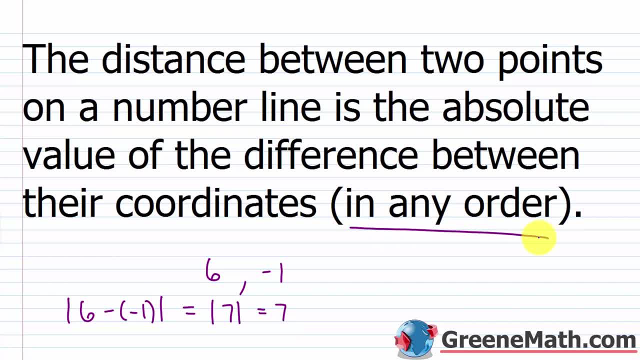 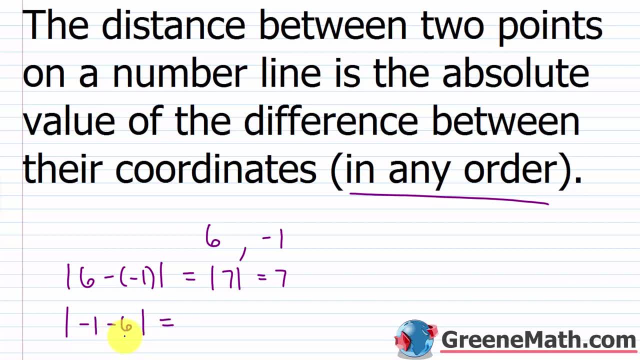 I could also, because this says in any order. I could flip this around So I could say the absolute value of negative one minus six And the absolute value of negative one minus six is the absolute value of negative seven, which again is also seven. So kind of the order doesn't matter here. 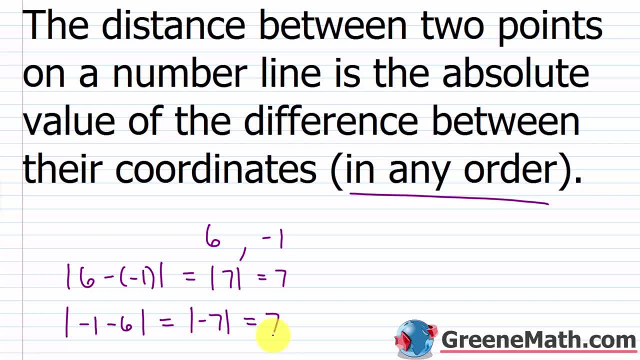 because of that absolute value operation, It's going to end up taking the sign and disregarding it, right? If you get a positive seven, it's still seven. If you get a negative seven, it makes it positive seven. So the order isn't going to matter here, because of the absolute value operation. 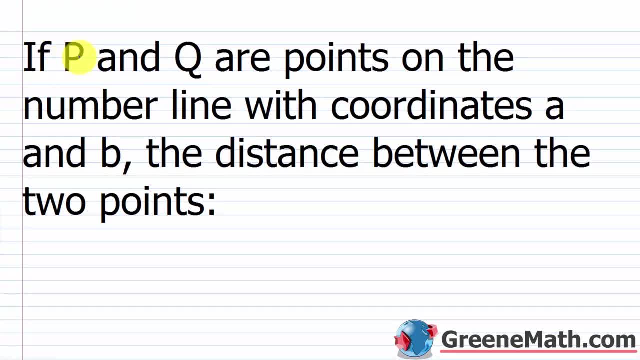 So officially, you'll see this in your textbook. If p and q are points, and don't get confused by p and q, p and q are just something we can use to label the points. So in this example here where I said we want to find the distance between six, 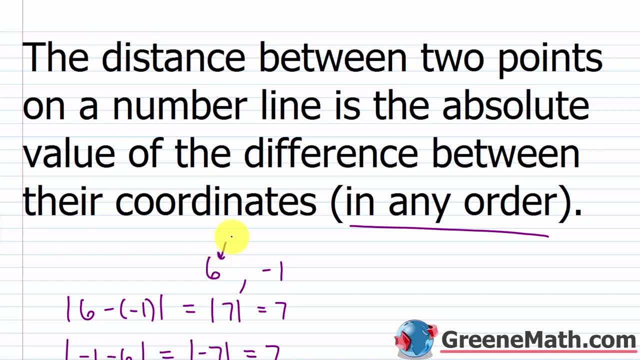 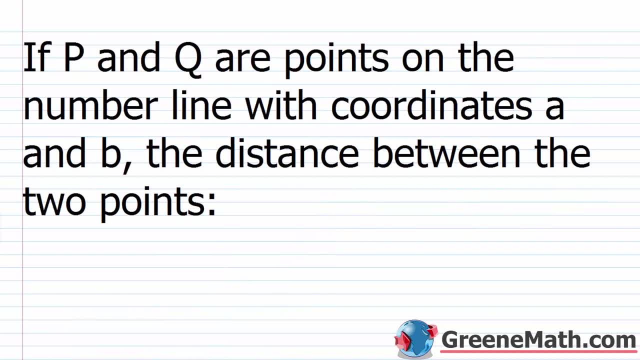 and negative one on the number line. I could label this guy as p, I could label this guy as q, right Or vice versa, it doesn't really matter. So if p and q are points of the number line with coordinates a and b, So when we say coordinates, 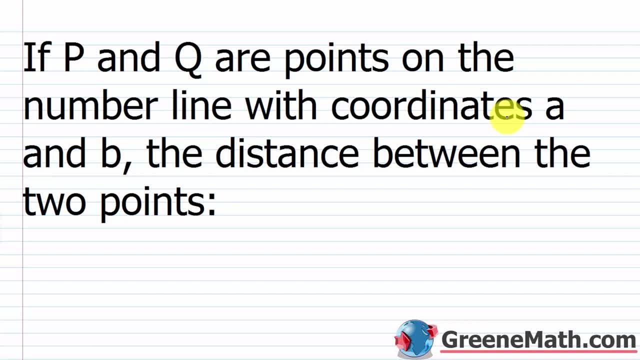 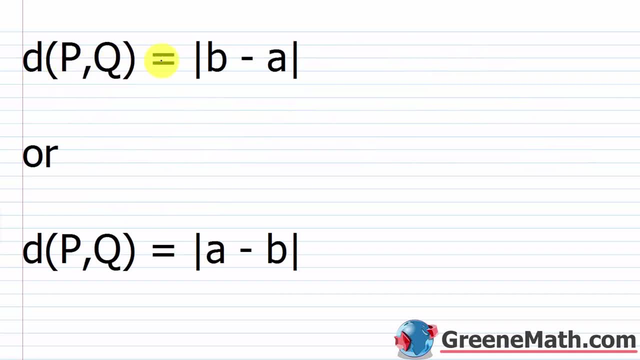 this refers to the number on the number line itself, And then we'll say: the distance between the two points is given by this formula here. So the distance between p and q is equal to the absolute value of b minus a, or the distance between p and q is equal to the absolute value. 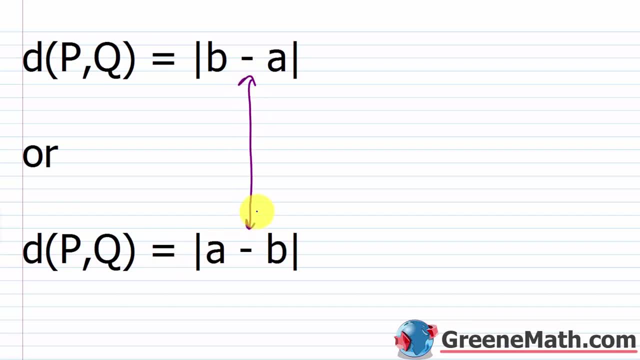 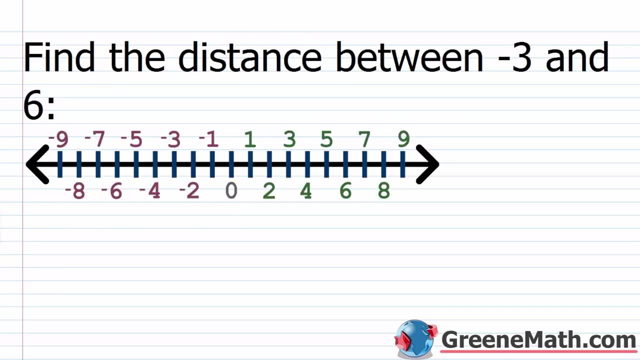 of a minus b, So again we can change the order around and get the same result because of this absolute value operation. So let's look at a sample problem here. We want to find the distance between negative three and six. So here's negative three and here's six, If I was to just count the units out. 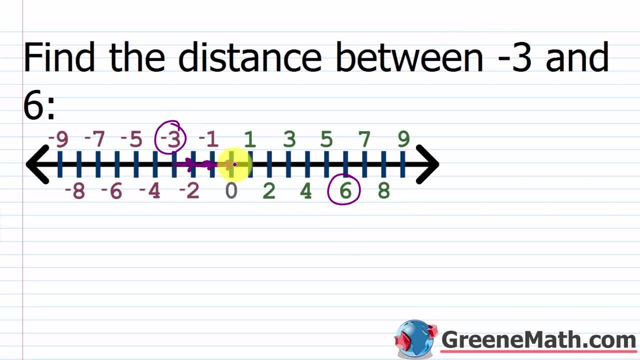 I could start at negative three and go one, two, three, four, five, six, seven, eight, nine, right? So they're nine units apart. If I started at negative three and with the six takes me nine units to get there. If I started at six and went back to negative three, it would also take me nine. 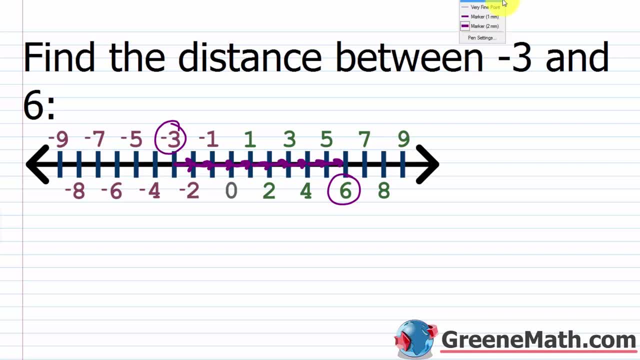 units to get there. But again, we don't want to do that each time, we don't want to have to pull the formula, And that formula tells us to subtract right one coordinate from the other, and it doesn't matter the order, because we're going to do this inside of the absolute value. 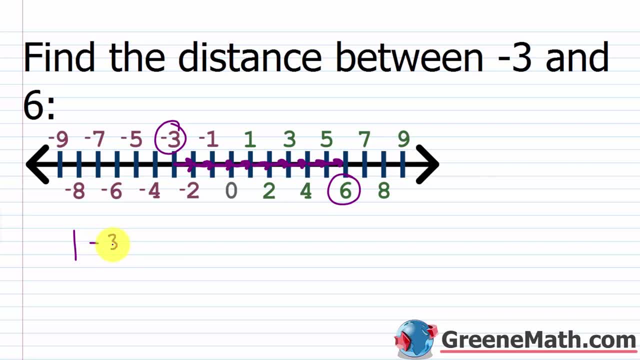 operation. So I could say the absolute value of negative three minus six, which would be equal to the absolute value of negative nine, which would be nine Again. that's what we found by just counting. We could also flip this around. we could say the absolute value of six minus a negative. 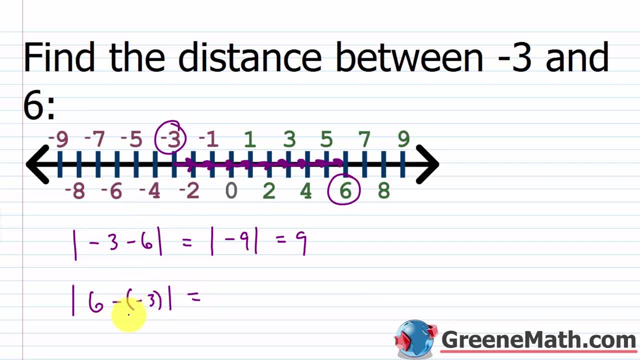 three. So this would be the absolute value of nine, which is nine. So either way we do it, if we do negative three minus six, that gives us negative nine. we take the absolute value. we get nine If we do six. 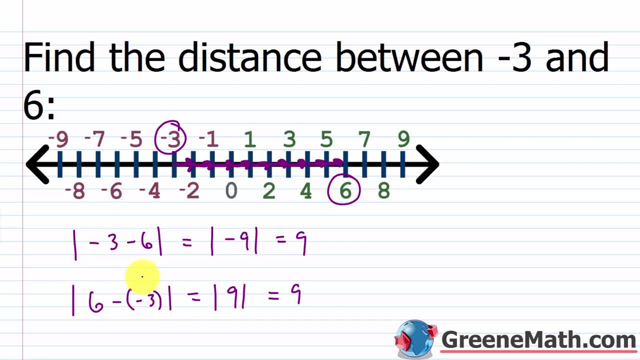 minus a negative three, that gives us six plus three, which is nine. we take the absolute value, it's still nine. So, again because of the absolute value operation, the order here doesn't matter. All right, let's look at one more. So we want to find the distance between negative four and 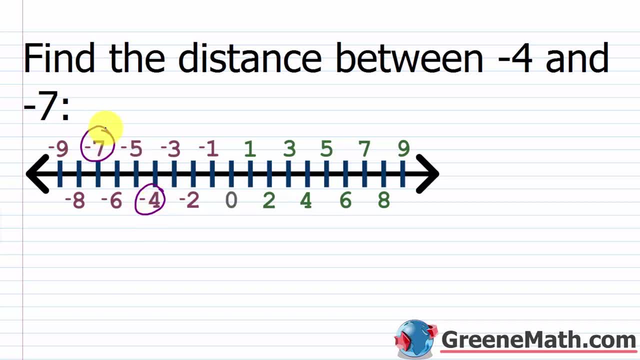 negative nine. So we're going to do this inside of the absolute value operation and we're going to negative seven. So here's negative four, here's negative seven. you can eyeball that and see it's three units right: One, two, three. they're three units away from each other. And again, to use our 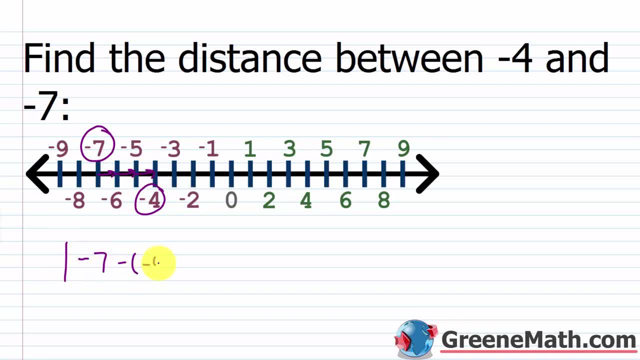 formula we could do: negative seven minus a negative four inside of absolute value bars, So this would be negative seven minus a negative four is negative seven plus four, So that would be the absolute value of negative three, which is three. Or again we could change the order around, right. 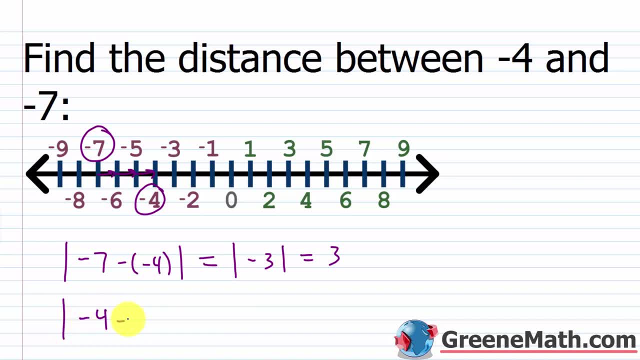 So we could do this inside of the absolute value operation and we could do this inside of the absolute value bars. We could say: negative four minus a negative seven. Negative four minus a negative seven is negative four plus seven. that would be positive three. So the absolute value of 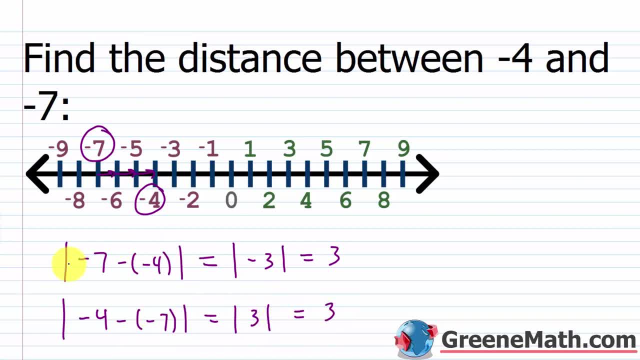 three, which is three, Again because of the absolute value operation. the order here doesn't matter. Once we evaluate, if we get negative three, the absolute value of that is three. If we get positive three, the absolute value of that is three. So, either way you do it, you end up with 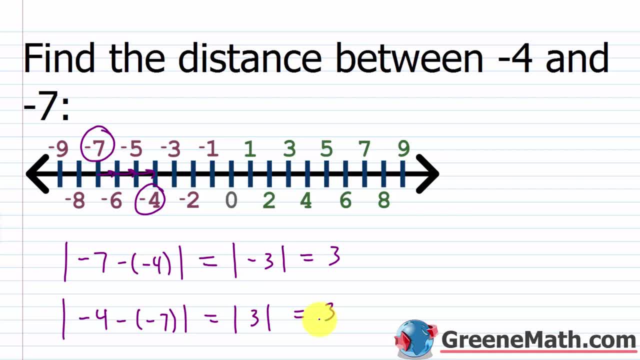 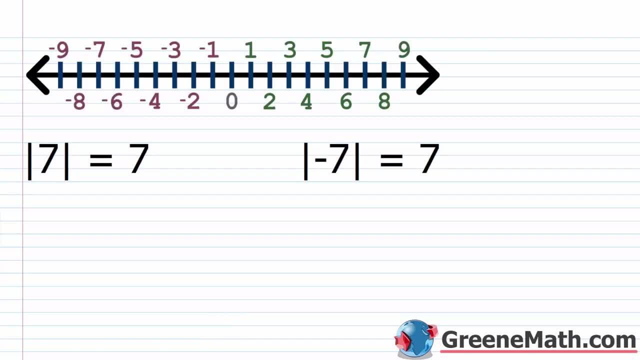 three as the distance between negative four and negative seven. So we're going to do this inside four and negative seven on the number line. In this lesson we want to review solving absolute value equations. So before we jump in and start looking at problems where we're solving absolute 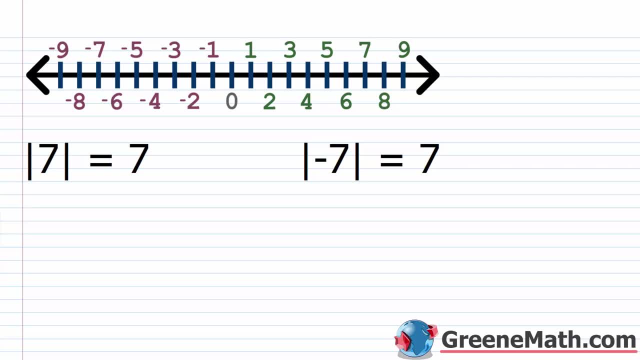 value equations. we want to make sure that we have a good understanding of the concept of absolute value, So this is something we reviewed at the beginning of the course. So if I said I want the absolute value of the number seven, what am I asking for? Well, the absolute value of a number. 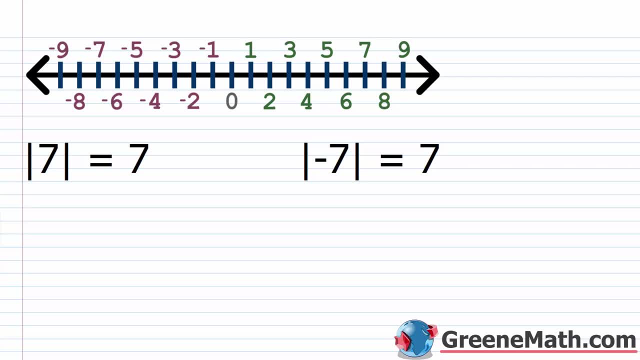 is the distance from the number to the absolute value of the number. So if I said I want the number to zero on the number line, So if I want the absolute value of seven, this is equal to seven. because if I started at seven on the number line and I counted how many units I'd have to go to get, 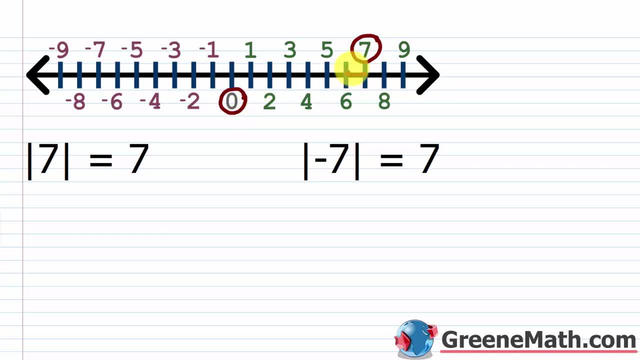 to zero. we all know it would be seven. right Start, here you go: one, two, three, four, five, six and then lastly seven units to get to zero. Similarly, if I wanted the absolute value of 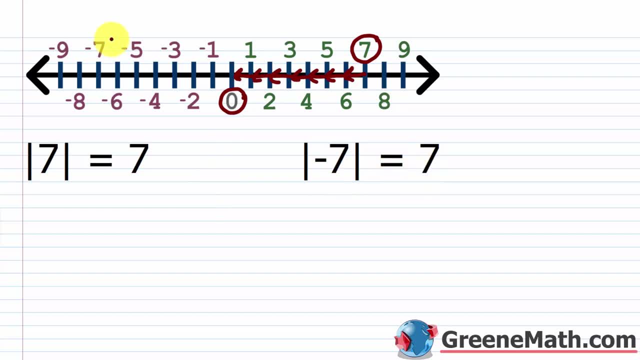 negative seven. it's also seven because if I started at seven I'd have to go to zero. So if I started at negative seven and I want to get to zero, I got to go seven units to the right. So one, two, three, four, five, six and then finally seven. So these two numbers, seven and negative. 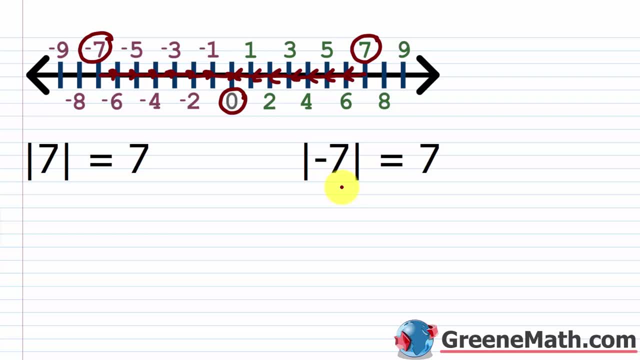 seven are known as opposites. okay, They have the same absolute value in each case- it's seven- but they lie on opposite sides of the number line. So one's going to be negative and one's going to be positive, right? So you have something like negative two and positive two. 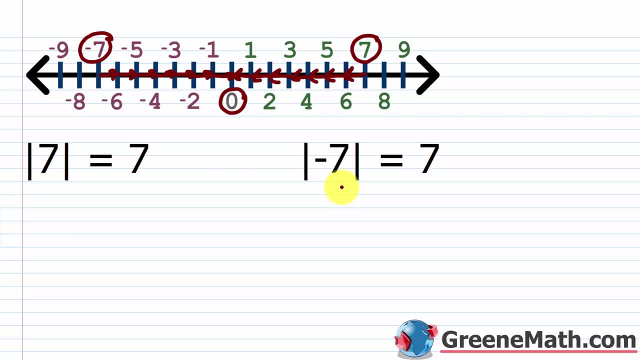 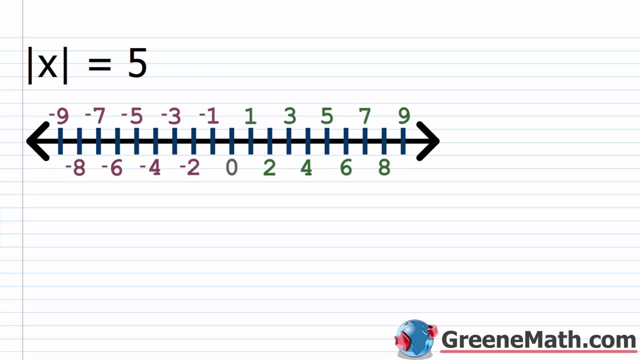 or negative two thirds and positive two thirds, or negative two million and positive two million, right So on and so forth. When we take the concept of absolute value and we start working with variables, you really have to think a little bit. So if I had something like the 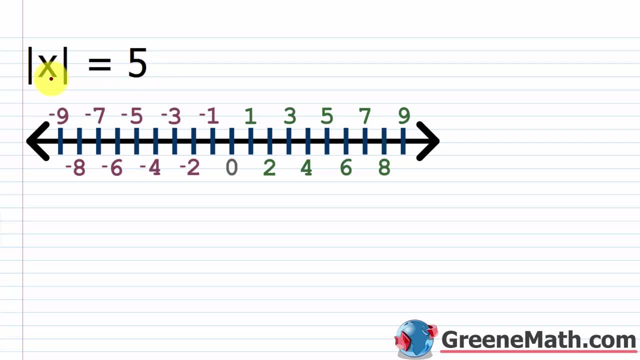 absolute value of x equals five. what can I plug in for x there and get a true statement? So the absolute value of x is equal to five. So in other words, I am asking for a value that, when plugged in here, I would take the absolute value of it meaning. I want to find the distance between that. 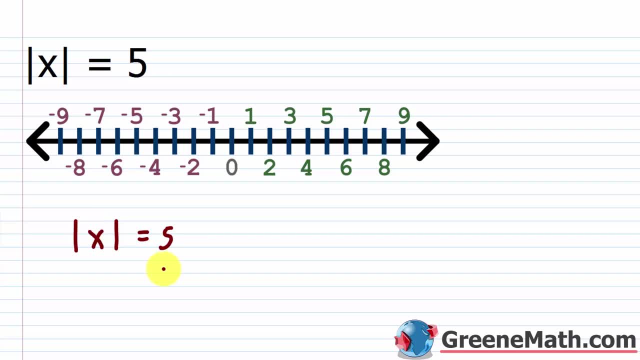 number and zero. So I'm going to plug in the absolute value of x there and get a true statement. So I'm going to plug in the absolute value of zero on the number line and it should be equal to five. Well, what numbers have an absolute value of five? Well, it's only going to be five and 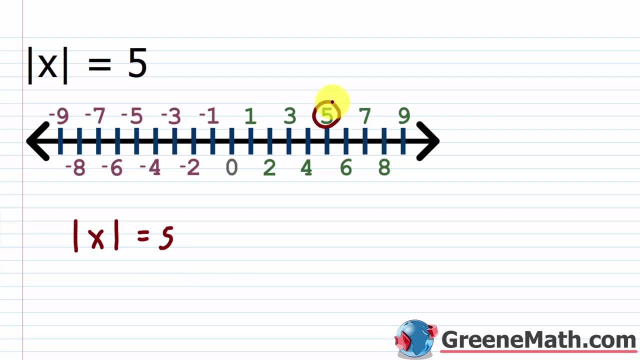 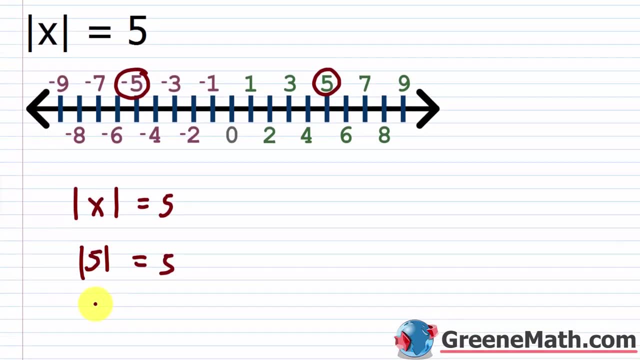 negative five. right, So five and negative five- okay, So that's what I can plug in for x. If I plug in a five there and I evaluate, I get five equals five. That's true, But again, that's not. 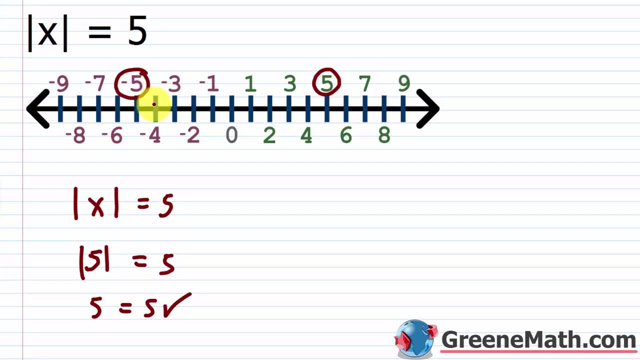 the only solution, because negative five, the opposite of five, also has an absolute value of five. So if I plugged in a negative five for x, you would get five equals five as well, which is also a true statement. So what ends up happening? 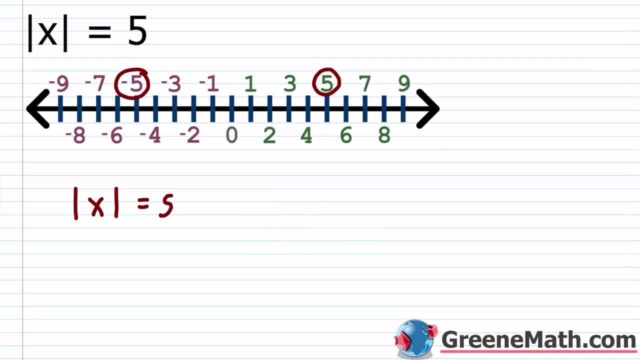 is we're going to say that our solution for this equation is going to be what It's going to be, that x could be equal to five. Then we have that keyword, or that we talked about in the last lesson, with compound inequalities. So x equals five or x equals negative five. Again, the or just tells: 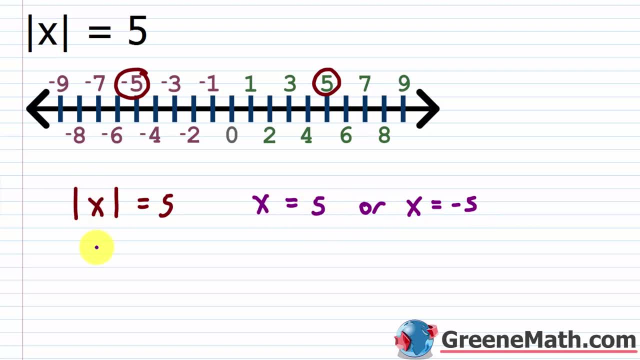 me, that either works. If I plug in a five here- take the absolute value- I get five. five equals five. that's true. If I plug in a negative five, I get five. five equals five. that's true If I. 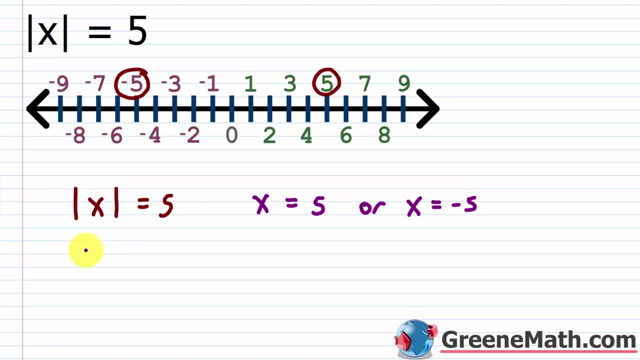 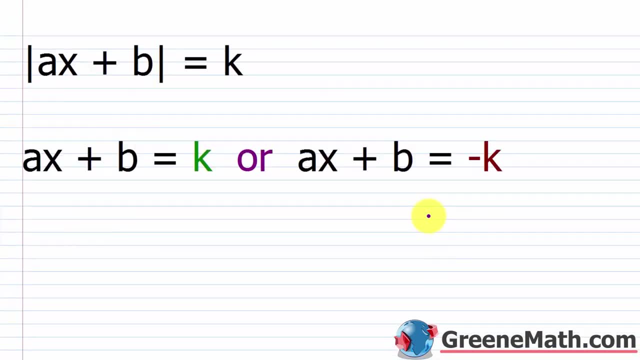 plug in a negative five. absolute value of negative five is also five. five equals five. that's also true. So either one works. That's why we use the or keyword. Now, in most cases we're not going to get something as simple as the absolute value of x equals some number. okay. 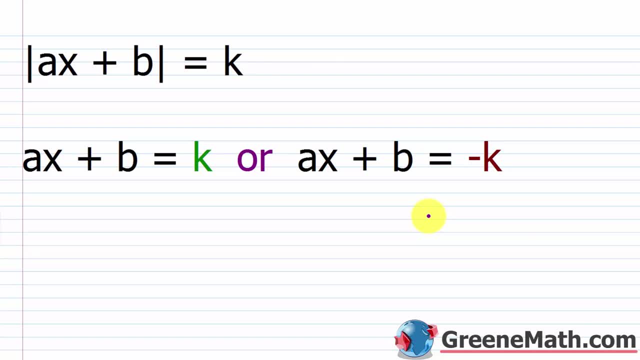 We're going to have some absolute value of an expression equal to some number, or later on we'll see things get more complicated than that. But essentially, if you have an equation in this format, you have the absolute value operation isolated on one side. 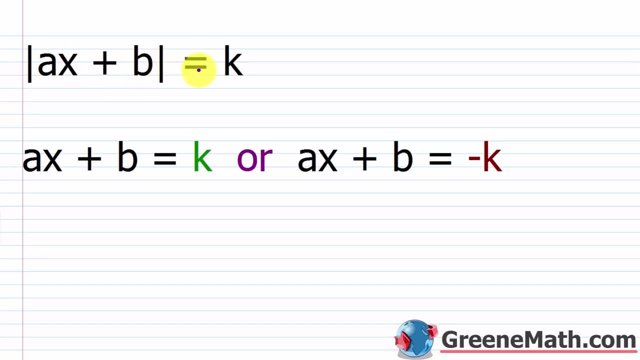 an algebraic expression inside of the absolute value bars and it's equal to some non-negative number like k. then we can go ahead and set up a compound equation with: or. We can say that this guy right here- the ax plus b could be equal to k, or ax plus b could be equal to the negative of k. 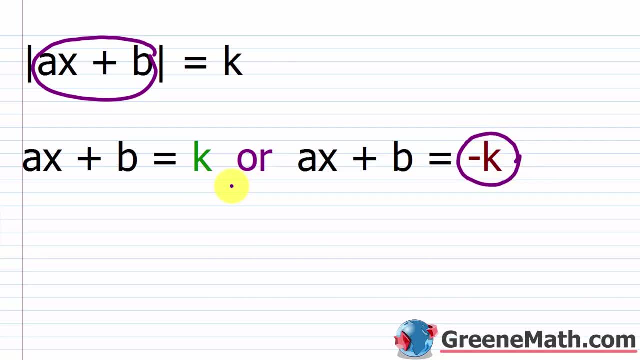 all right. Now, it's hard to understand this when you look at it in this generic formula, but I want you just to jot this down in your notes anyway. and let's look at the first example and we're going to kind of relate back to this. So we have the absolute. 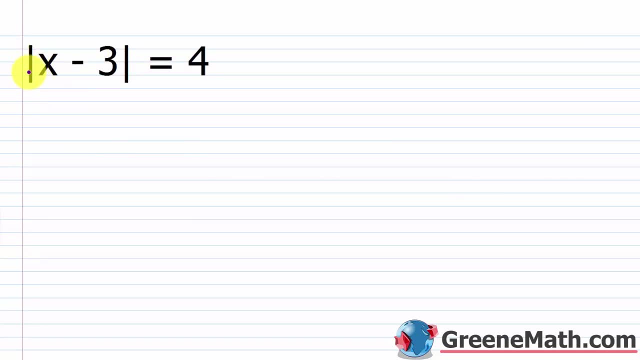 value of x minus three is equal to four. So you see that you have the absolute value operation isolated on one side. you have some non-negative number on the other. okay, So we're good to go there. So, essentially, what my formula told me to do was to take this expression here: 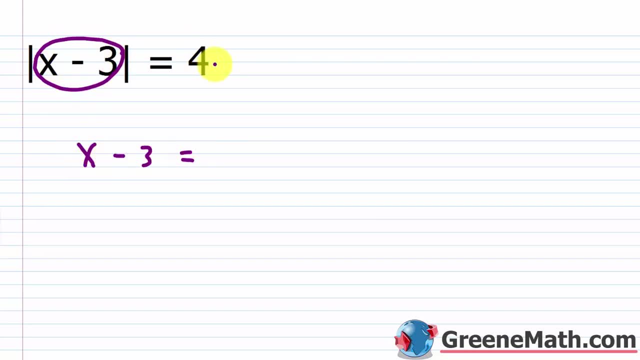 so x minus three, and set it equal to this number, so equal to k. remember, In this case k is just four, so equal to four. Then you take your expression again, so x minus three could be equal to negative four, okay, Remember. 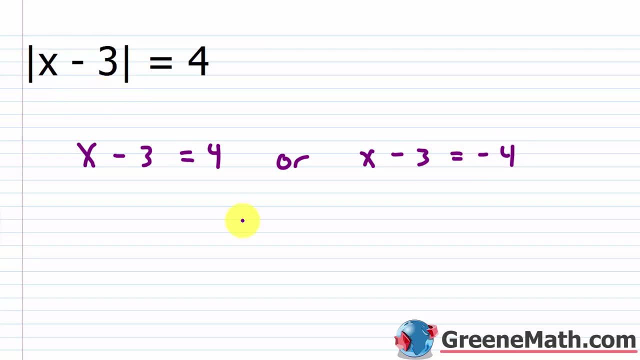 you said negative k. now it's just negative four. Now why does this thought process work? Well, think about it. If I find a value for x that when I plug it in here and I subtract away three, it's going to give me four, Basically, I'm going to be evaluating the absolute value of four. 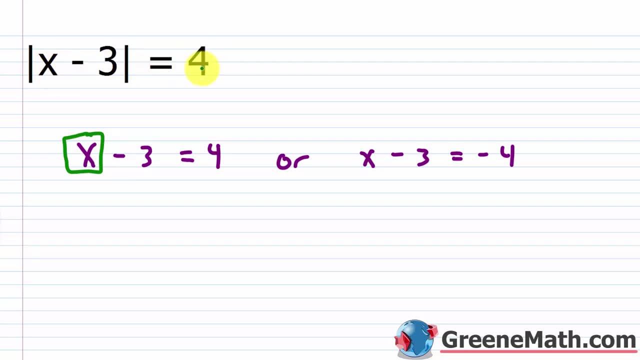 and that is four. so I'm good to go there. Alternatively, if I find a value for x, then when I subtract away three, I'm going to be evaluating the absolute value of four. I get negative four. Well, I'm going to be evaluating the absolute value of negative four. 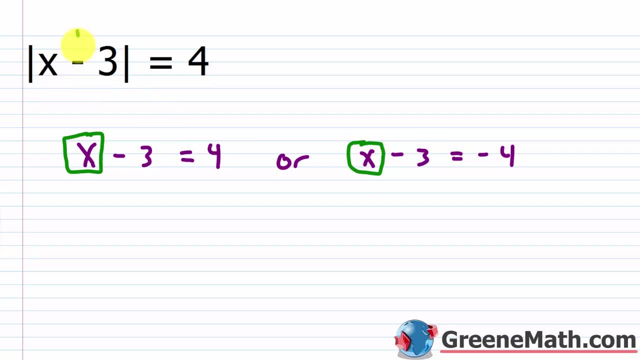 which is also positive four. So that's what I'm looking for. I'm looking to get a result, inside of the absolute value of ours here, of either four or negative four. It doesn't matter which one it is, because in each case I will get a value of four. So let's go ahead and solve this. 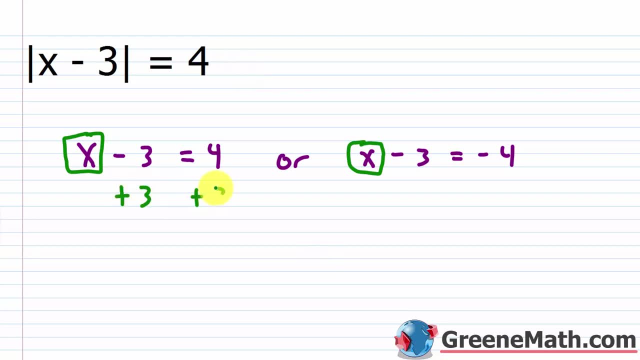 really quickly. On this one, I would just add three to each side of the equation. I'm going to get that x is equal to seven. For this one, I'm going to add three to each side of the equation and I'm going to get that x is equal to seven. So I'm going to get that x is equal to seven. 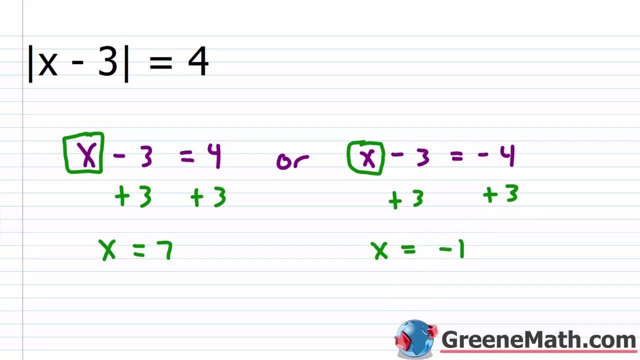 to negative one. So let's check these. It's very easy to do, So I'm going to plug in a seven for x here. So I would have the absolute value of seven minus three is equal to four. So seven minus three is four. So I would have the absolute value of four equals four, And of course that's true. 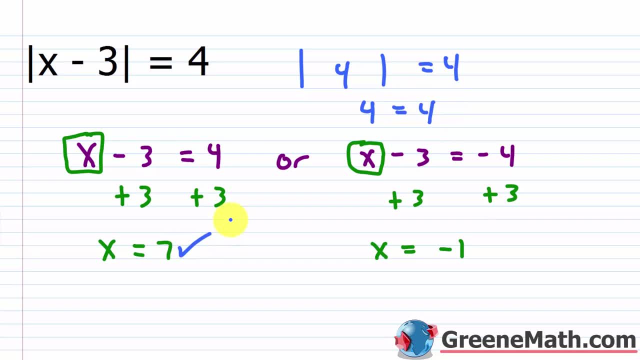 Four does equal four, So that's a big check. Okay, so that works. Now let's check the other scenario. We have x equals negative one. So if I plug in a negative one for x, right there. so negative one minus three. 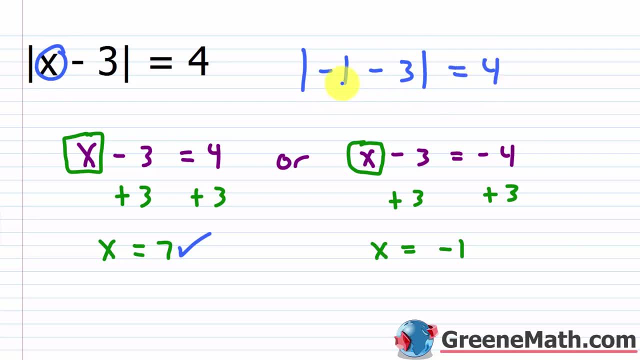 we're taking the absolute value of that, this should be equal to four. Negative one minus three is negative four. So you'd have the absolute value of negative four is equal to four, And we know that's true, right. The absolute value of negative four is four. So you get again: four equals four. 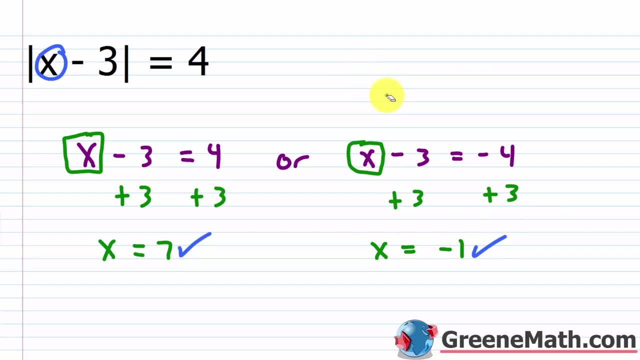 So this one's a big check too, So you can see how that ends up working. right? You take this expression right here, this guy, and you set it equal to this number And then the negative of that number. you solve those two equations. you kind of put it together with that equation. 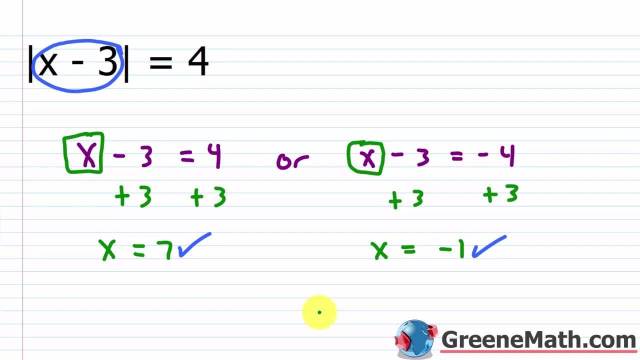 the keyword or, and then you're going to have your solution. So there's a few different ways to notate the solution. You can kind of remove these check marks. you don't need them anymore. you can just put an or there between them. So x equals seven or x equals negative one. 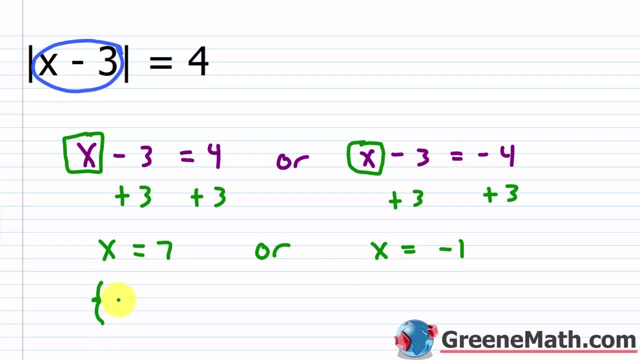 that's fine. You can use the solution set notation and say you have negative one and seven as the elements, or basically solutions that work for your equation. And then, lastly, you could also do this: you could say: x equals seven, comma negative one. 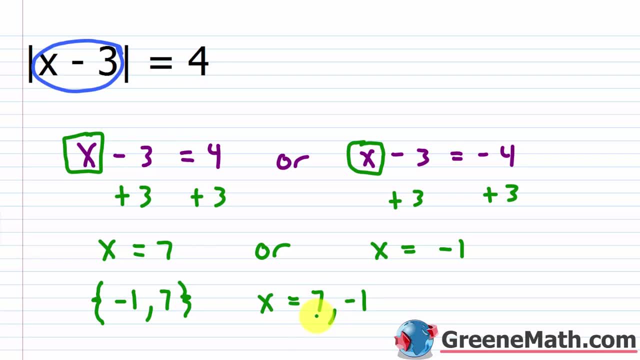 Right, Lots of different ways to notate this, but just make sure that you're indicating that each one is a solution to your equation. All right, let's take a look at another one. So we have: the absolute value of five x minus four is equal to six, So again, we're following the same thought. 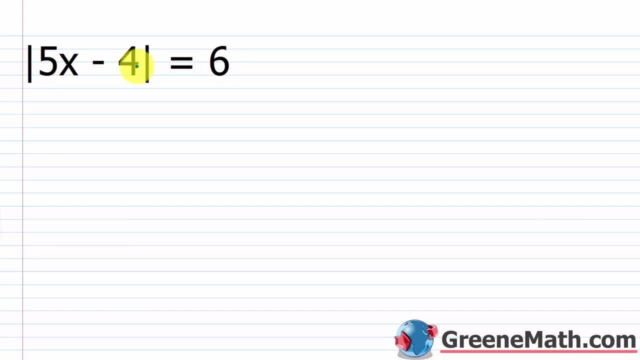 process, We're going to take this expression inside the absolute value bars. So five x minus four, we're going to set it equal to six and we're going to have, or we're going to have, five x minus four is equal to the negative of six. Okay, 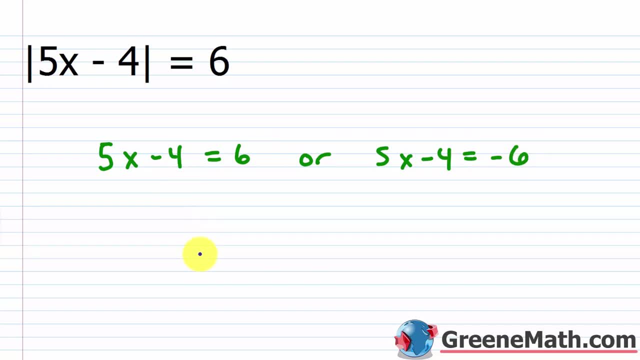 So what I want to do? I want to solve each one of these. So I want to add four to each side of the equation. here. that's going to cancel. I'll have five. x is equal to 10, divide both sides by five and I'll get that x is equal to two. Over here I just want to add. 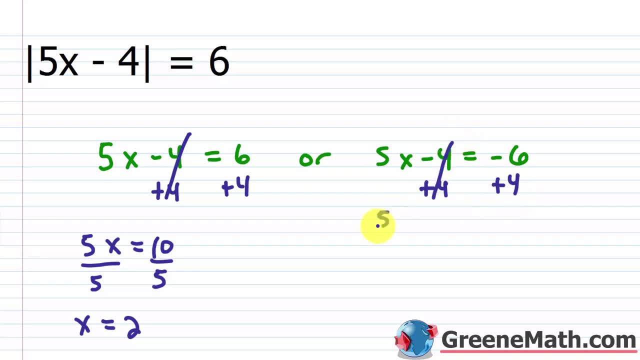 four to each side. that's going to cancel. I'll have five. x is equal to. you'll have negative two. divide both sides by five and you'll have that x is equal to negative two fifths. All right, So let's erase these. So I'm going to go ahead and say that x is equal to two or x is equal to. 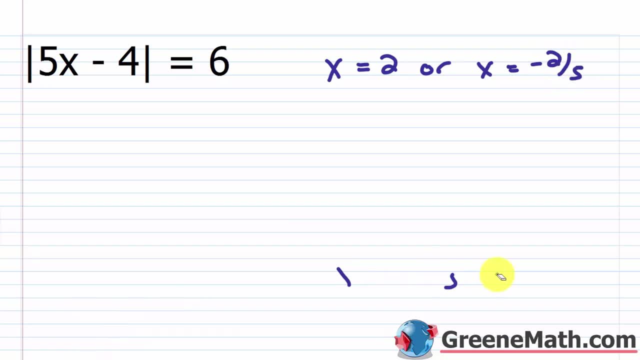 negative two fifths. like that Again. you can write it that way. you can use the solution set notation. a lot of books do that. Or you can also just say that x equals two comma. negative two fifths right. Each is a solution. Now again, if you want to check this, you could plug a two in. 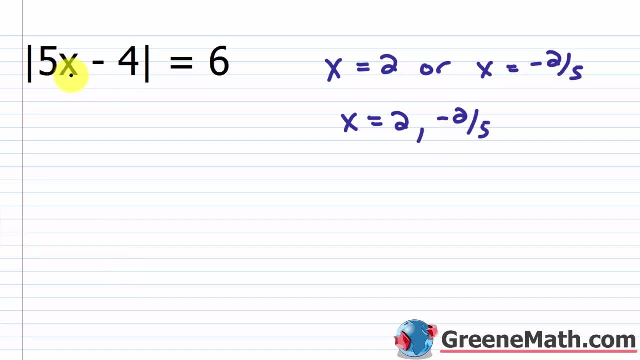 for x. you can also plug a negative two fifths in for x and you would see that the left and the right are equal. So let's go ahead and check it. So the absolute value of five times two and then minus four is equal to six. So five times two is 10, 10 minus four is six. The 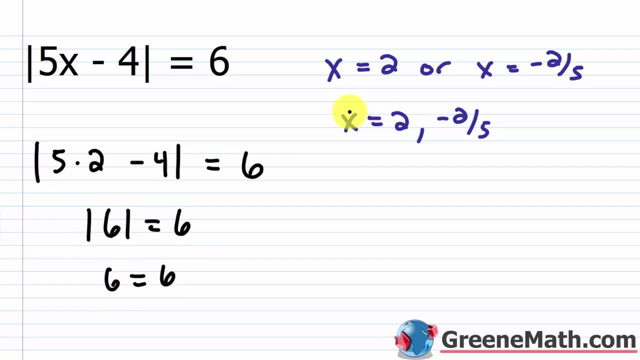 absolute value of six equals six. So six equals six. So yeah, that's true. You can check that one off. Then the other one is negative two fifths. So negative two fifths, So five times negative two fifths. the fives would cancel. You'd have negative two minus four, which 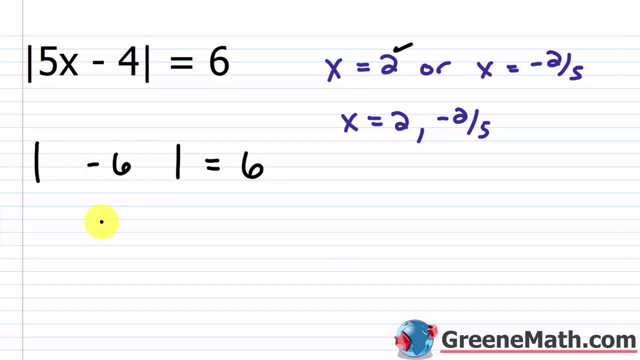 is negative six, The absolute value of negative six, which we know is six. So six equals six here. So this one checks out as well. So again, x equals two or x equals negative two fifths. Let's look at one. 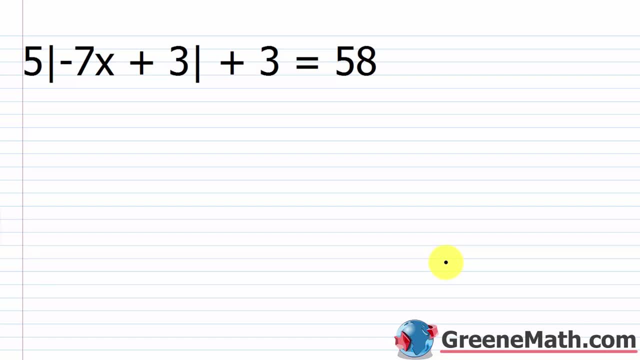 that's a little bit more complicated. It's just more complicated because you don't have the absolute value operation isolated on one side. So we have five multiplied by the absolute value of negative seven x plus three plus three equals 58. So your goal, if you get something like this: 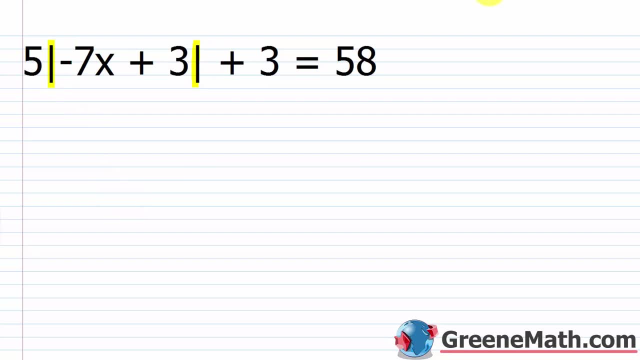 is to isolate the absolute value operation. How can we do that? It's very, very easy. You just think about what's being done to that absolute value operation. You have multiplication right, You're multiplying by five and you have addition. 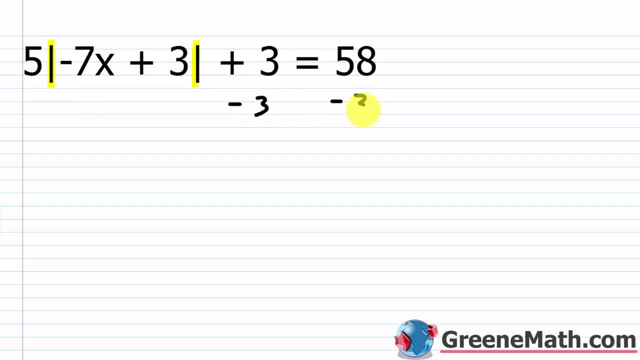 three is being added to it. So let's go ahead and subtract three away from each side to start. We'll get rid of that. We'll have five times the absolute value of negative. seven x plus three, And this equals 58 minus three is just 55. Now I can just divide both sides by five, So I divide. 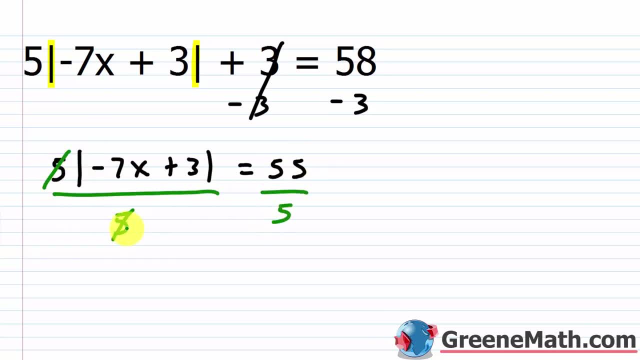 both sides by five, And this would cancel with this, And so I have the absolute value of negative. seven x plus three is equal to 55 over five is 11.. So now I have it in the format that I've been looking at And again, 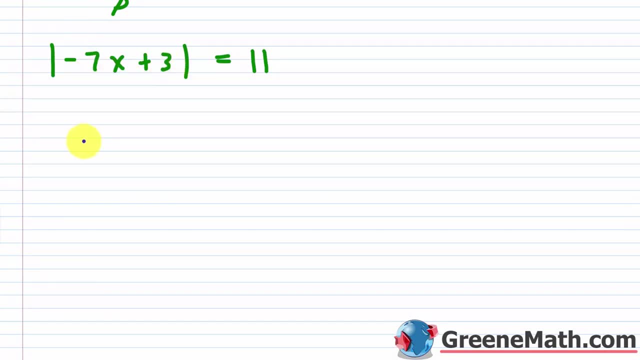 once I have it like this, it's very, very easy: I take my expression So negative, seven x plus three, I set it equal to 11.. And then I say, or I take my expression So negative, seven x plus three. 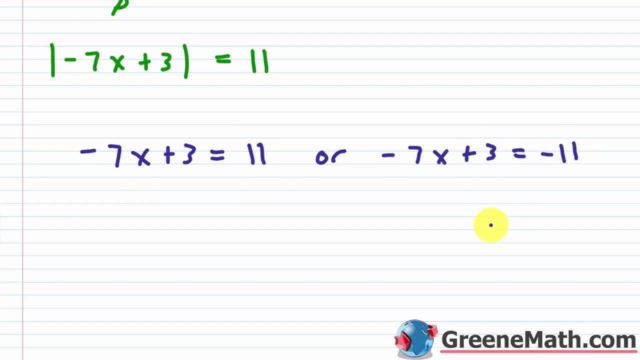 I set it equal to negative 11.. Okay, Just solve each one Very, very simple. So I'm going to subtract three away from each side of the equation. I'm going to get negative seven. x is equal to 11 minus three is eight. 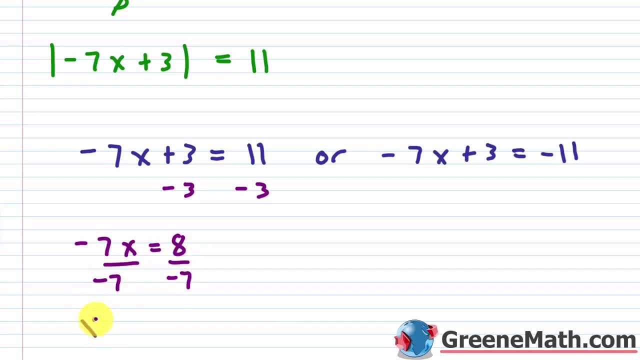 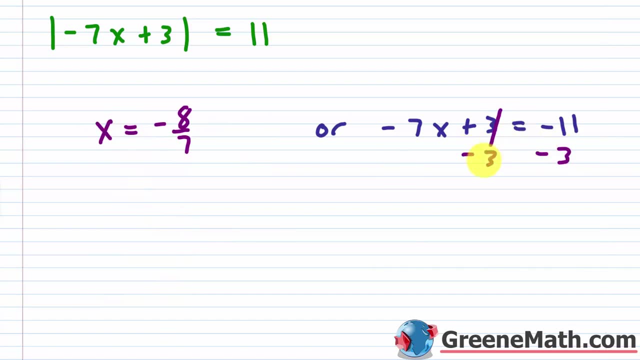 Then I'm going to divide both sides by negative seven And I'm going to get that x is equal to negative eight sevenths Over here. let me subtract three away from each side. That cancels. You'll have negative seven. x is equal to negative 14.. Divide each side by negative seven. 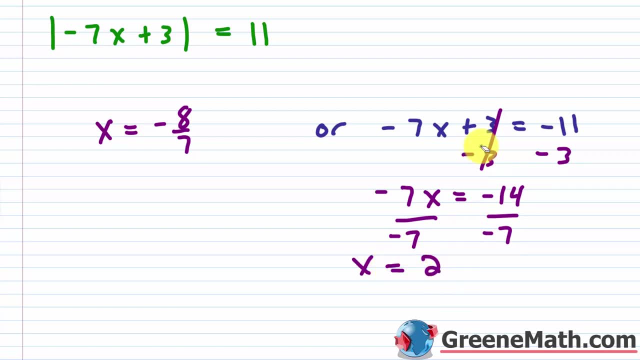 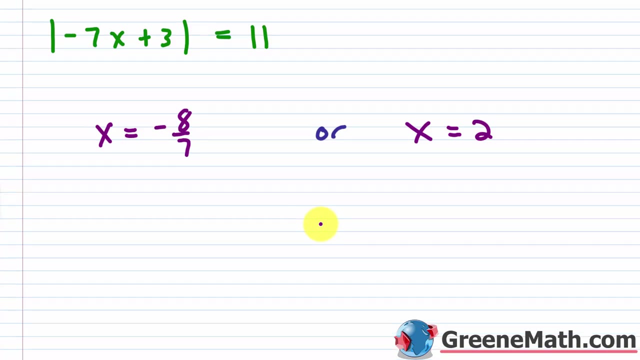 And you get that x is equal to positive two. So let me erase this. So again, x equals two. So you can leave this as your solution. Again, you could write it in solution set notation. You could put the comma. There's a zillion different things. you can do whatever you're. 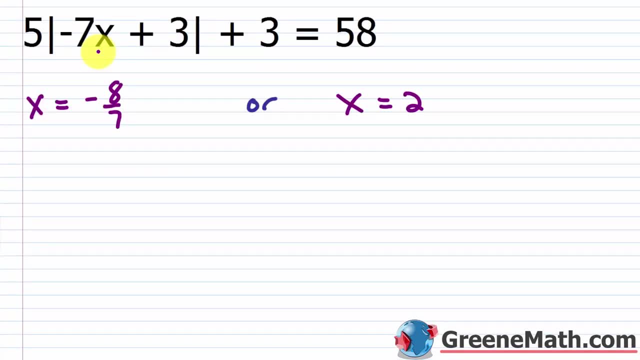 more comfortable with. So let's go ahead and check this real quick. And then all the rest of them. I'll leave that up to you to check them on your own. So I would have five multiplied by the absolute value of, I'd have negative, seven times negative. 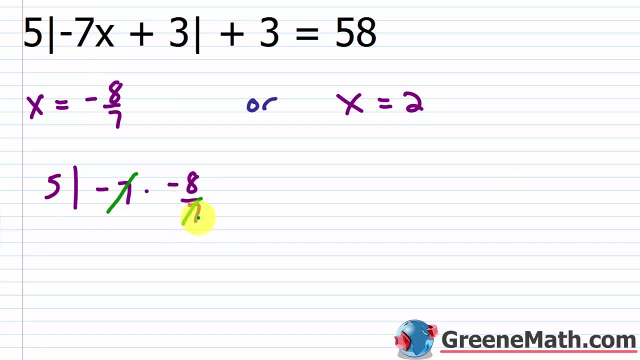 eight, sevenths. So we know that this would cancel. with this The negatives would cancel. So I'm basically just going to have an eight there. So I'd have eight plus three, which is just 11.. So then plus three equals 58.. 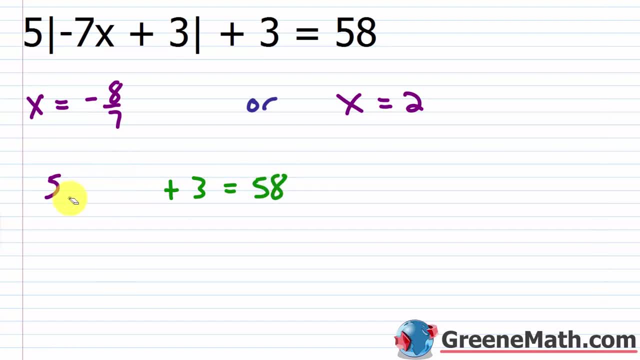 So the absolute value of 11 is 11.. So you have five times 11 there, That's 55, and then 55 plus three is 58. So this one's good to go Over. here you have the two that's going to be plugged in for x. 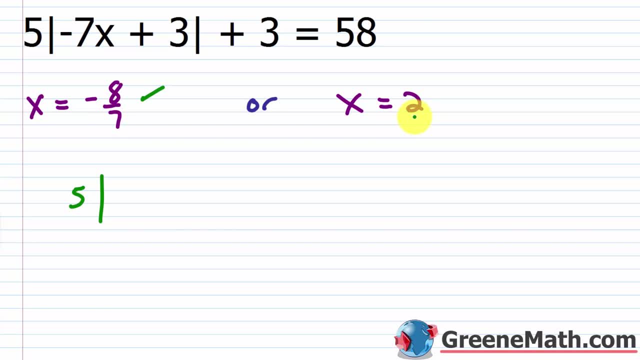 So five times the absolute value of negative, seven times two is negative 14.. Negative 14 plus three is negative 11.. But again, because I'm taking the absolute value there, it just becomes positive 11.. So five times 11, then plus three equals 58.. 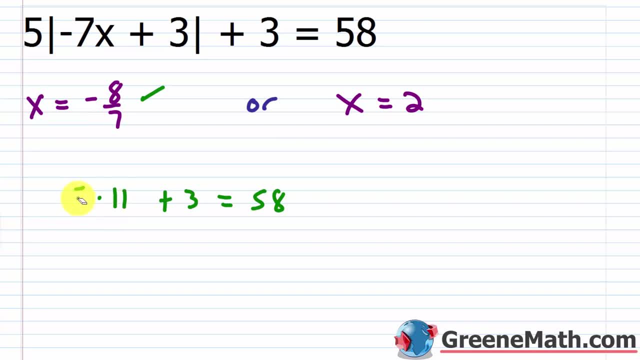 We already know that's true. Five times 11 is 55.. 55 plus three is 58. So we're good to go in each case. Again, our solution is: x equals negative eight sevenths, or x equals two. All right, let's take a look at another one. 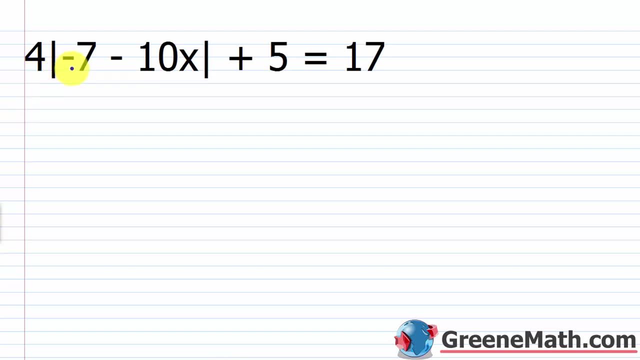 So suppose we had four multiplied by the absolute value of negative seven minus 10x. Then we had plus five, and this was equal to 17.. Again, what I want to do here is to isolate the absolute value operation on one side and then to have 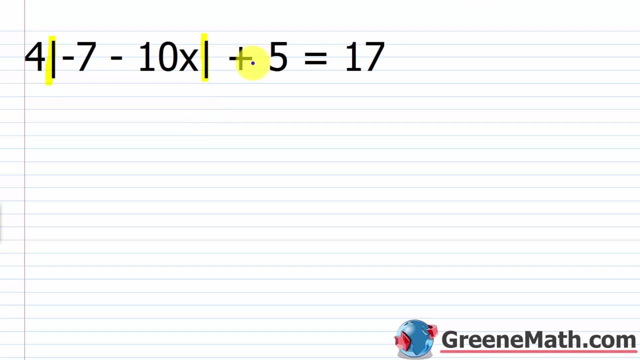 a number on the other. Okay, so what I want to do? I want to just subtract five away from each side of the equation to start. So we know this would cancel. So we'll say we have four times the absolute value of. we have negative seven minus 10x. 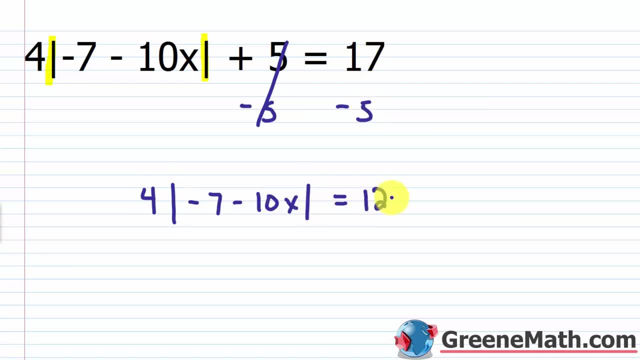 And then this is equal to 17 minus five is going to give me 12.. Scroll down, get some room going. All right, So to isolate the absolute value operation, I have four that's multiplied. So I'm going to do this. 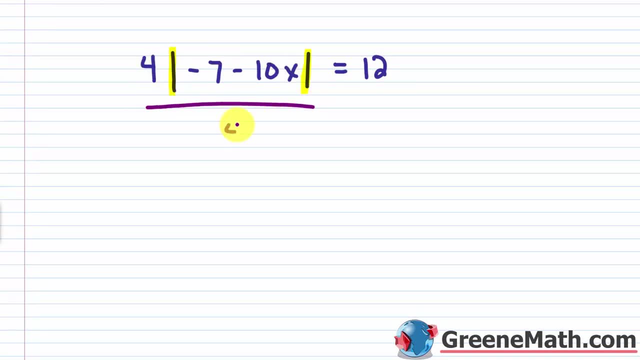 I'm going to do this. I'm multiplying it, So all I need to do is divide both sides of the equation by four. So we know that again, this would cancel. I'll have the absolute value of negative seven minus 10x. 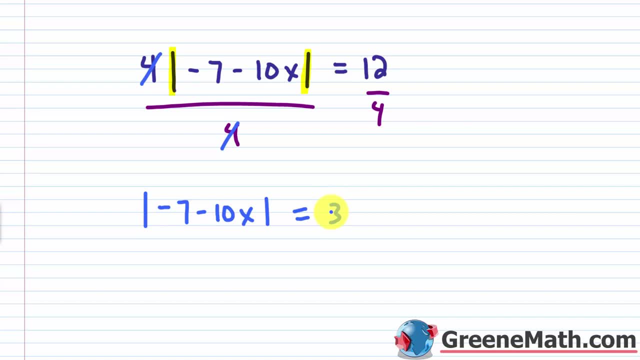 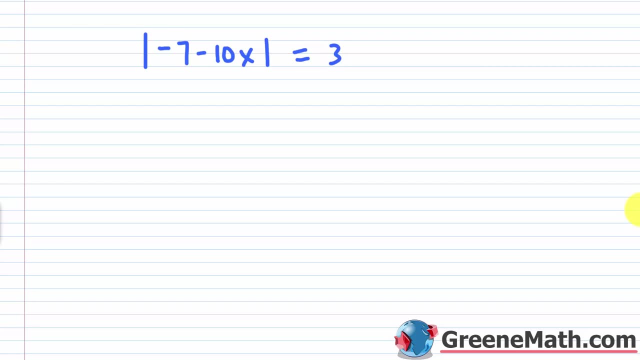 This will be equal to 12. divided by four is three. So now we have this in the format of our absolute value operation equals some number. So the absolute value operation here is equal to some number. So I can set up my compound equation with OR: 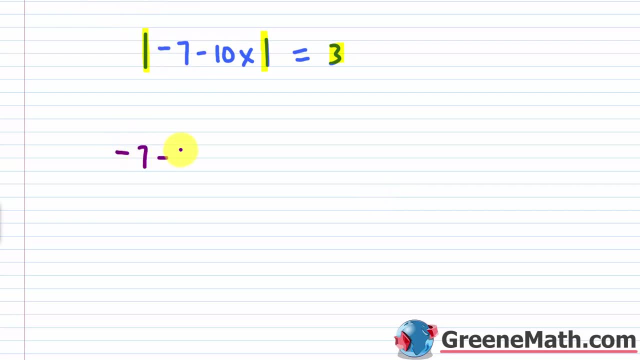 So I just take the expression inside. In this case it's negative seven minus 10x. I'm going to set it equal to three Then, OR I'm going to take my expression inside: so: negative seven minus 10x. 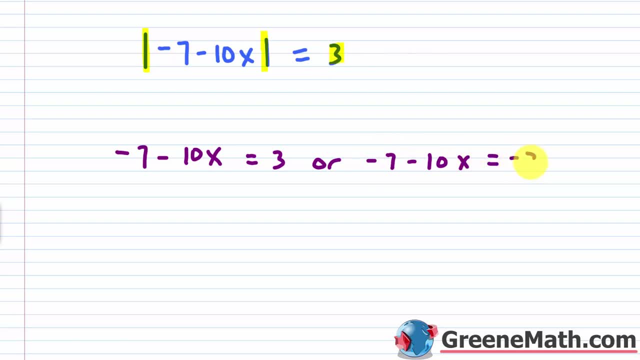 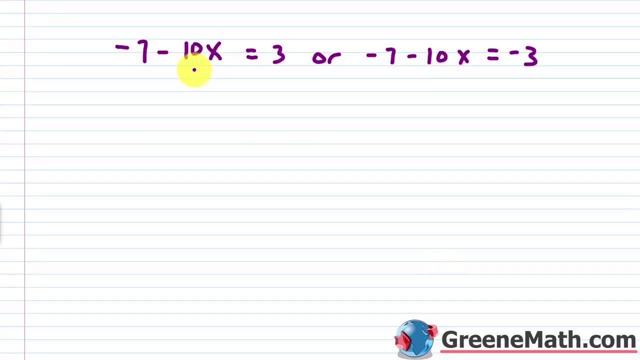 And I'm going to set it equal to the negative of three, So negative three. And then I'm just going to solve these two equations here And I'll have my solution. So, on the left, I'm just going to add seven to each side of the equation. 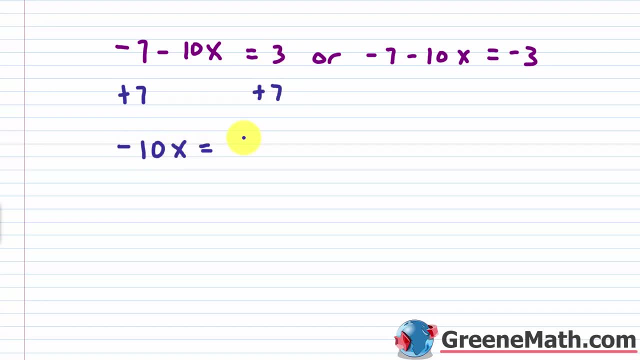 I'll have that negative 10x is equal to three plus seven is equal to four. All right, So that's just 10.. And now we can divide both sides of the equation by negative 10.. And of course, this guy's going to cancel. 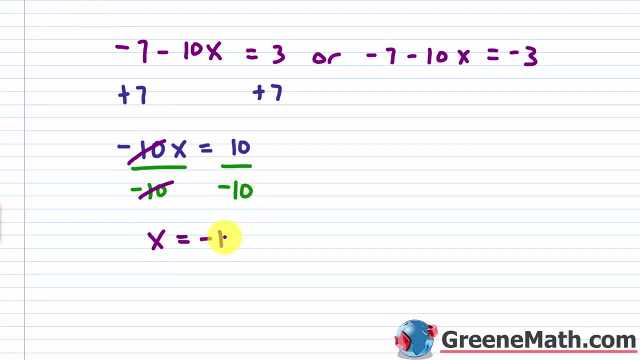 I'll have: x is equal to 10 over negative 10 is just negative one. So that's one solution. Let's get our other solution over here on the right. So again, I'm going to add seven to each side of the equation. 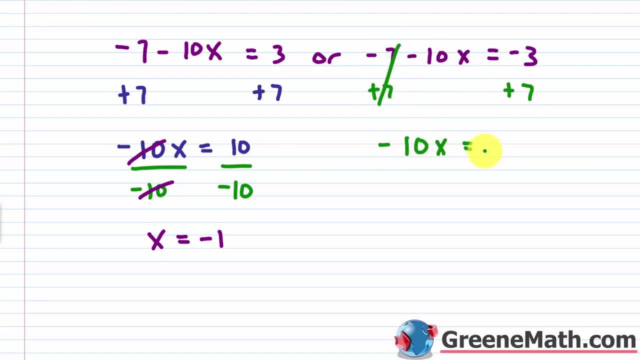 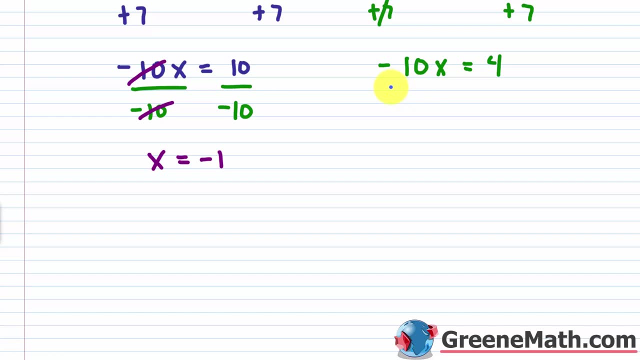 This is going to cancel, I'll have negative. 10x is equal to negative. three plus seven is going to be four. So now let me scroll down and get a little bit more room here. If I divide both sides of the equation by negative 10, then this guy right here is going. 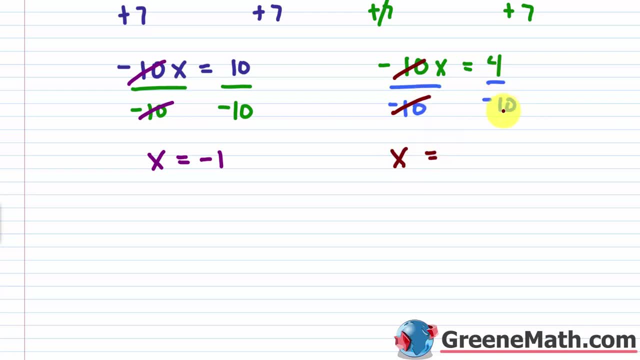 to cancel with this guy And I'll have. x is equal to four over negative 10.. We know that's negative. They're each divisible by two. Four divided by two is two And 10 divided by two is, of course, five. 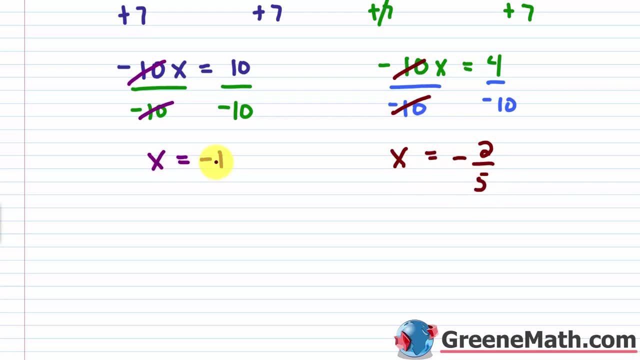 So I get x equals negative two fifths. So I can write this as x equals negative one, or my keyword, or x equals negative two fifths. Again, you can do the solution set notation, where you can just list them with a comma, whatever you want to do. 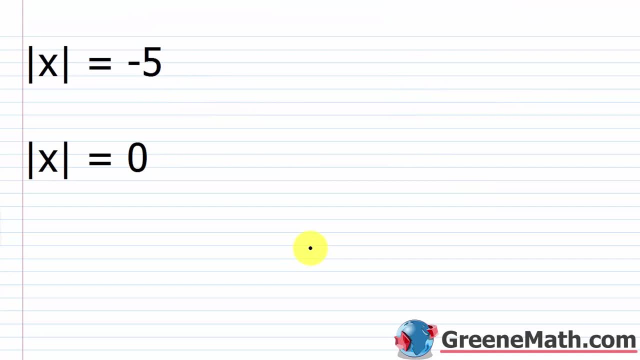 All right. So let's take a look at some special case scenarios that come up when we're solving absolute value equations. So the first one we're going to talk about is the situation where you have no solution. So something like the absolute value of x is equal to negative five. 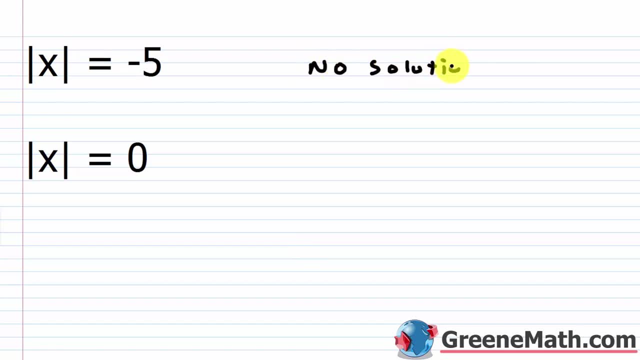 This guy would not have a solution. So no solution. Why is that the case? Well, we should know that the absolute value of some real number, x, is greater than or equal to zero, Because if I plug in a zero here, I get zero. 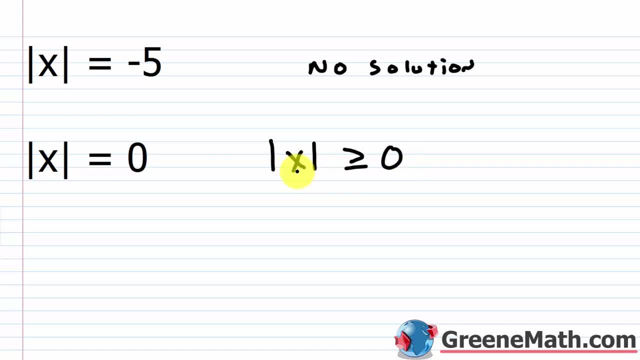 If I plugged in a negative here, I'd get a positive, And if I plugged in a positive, I would get a positive. right, This stems from the definition of absolute value. When you take the absolute value of the number, you want the distance from zero to the number. 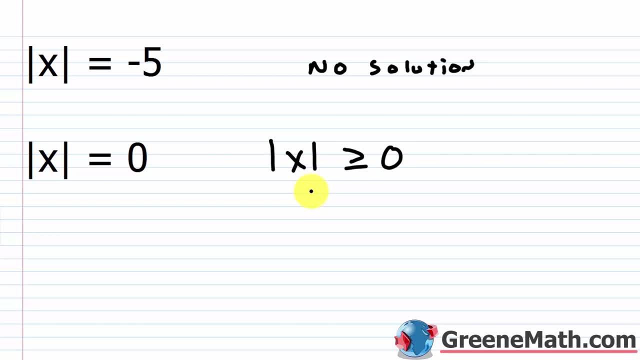 on the number line. So if it's zero, it's just going to be zero. If it's some negative, again, you'd get a positive. If it was a positive, it would just be a positive, okay, So you're never going to get a negative result. 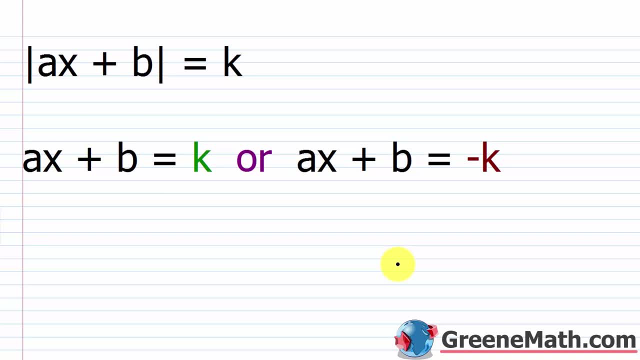 So this guy would always be no solution. When we go back to our generic formula here, I said earlier that the absolute value of x is equal to zero. So if you have an absolute value of some expression- ax plus b- if this is equal to k, k has to. 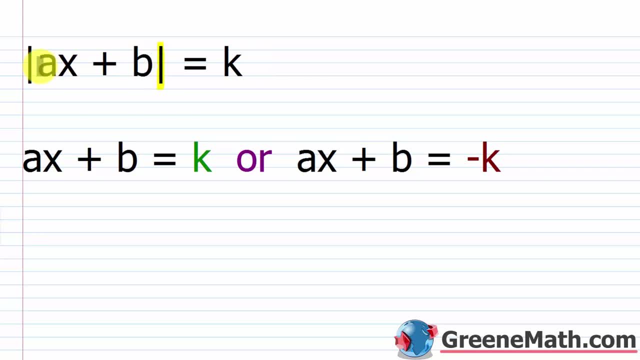 be non-negative. So if you have isolated this guy right here- the absolute value operation on one side, and on the other side you have a negative value- you can stop and say there's no solution. What you don't want to do is say there's no solution before you've isolated the absolute. 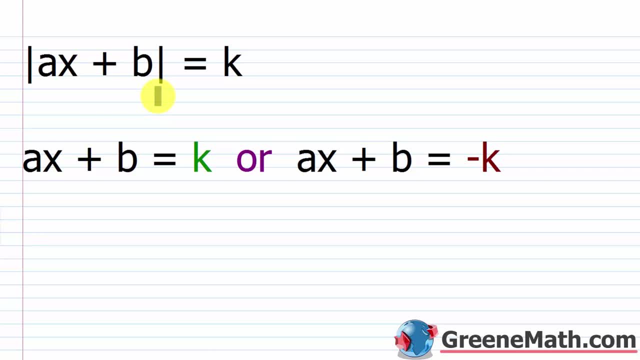 value operation on one side. That can lead to problems, okay. So you need to make sure you isolate first. All right, let's take a look at an example. So we have nine times the absolute value operation on one side. Okay, 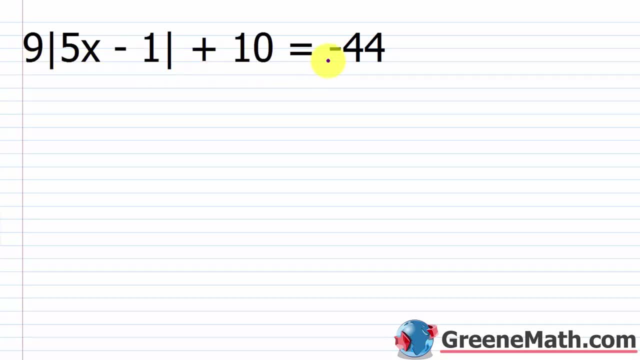 So if we have an absolute value of 5x minus 1, then plus 10 is equal to negative 44. So the idea here is that we want to isolate the absolute value operation on one side of the equation and then we want a number on the other. 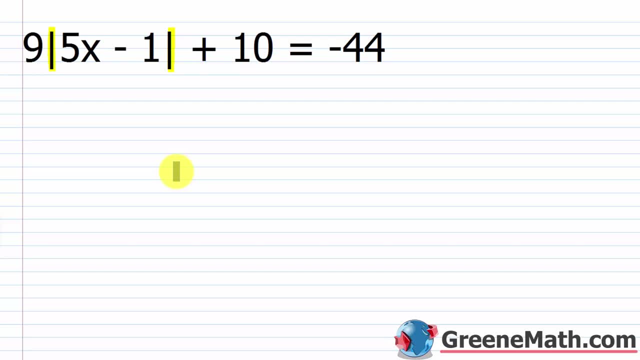 But if that number on the other side happens to be negative, we're not going to have a solution. So don't just look at the negative over here on the right-hand side and assume that this guy is going to be a no solution to start. 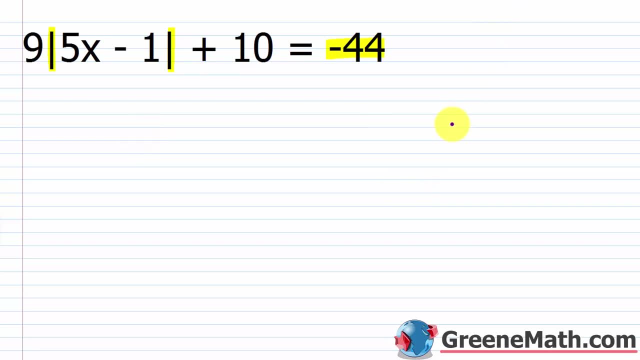 You've got to isolate the absolute value operation before you can make that determination. So I'm going to start by just subtracting 10 away from each side of the equation And we'll cancel this. We'll have 9 times the absolute value of 5x minus 1.. 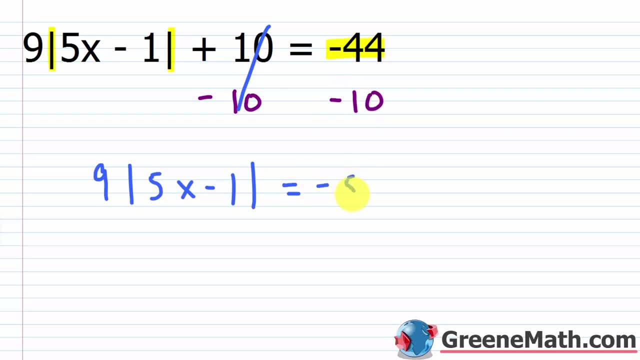 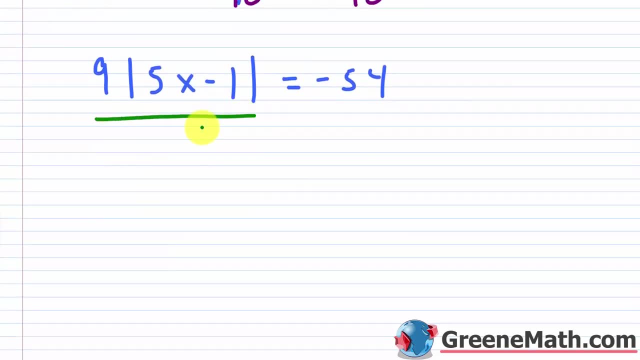 And this is going to be equal to negative 44 minus 10 is negative 54.. So at this point you pretty much know it's going to be no solution, But let's continue. Let's go ahead and divide both sides by 9.. 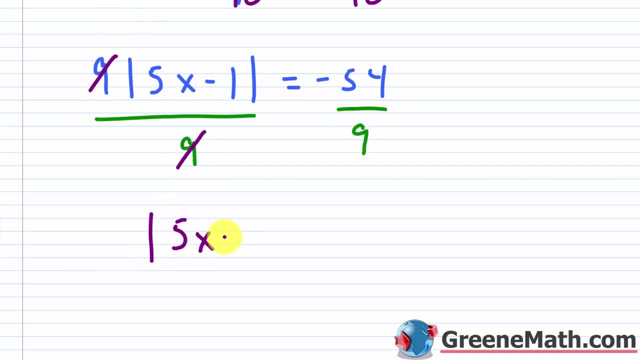 And of course this will cancel, We'll have the absolute value. of 5x minus 1 is equal to negative 54.. Negative 54 over positive 9 is negative 6.. So we know at this point there's no solution. 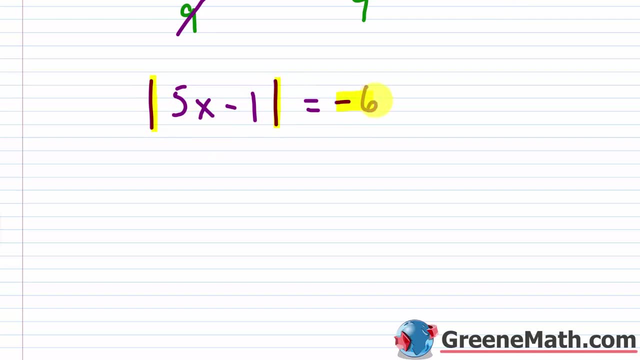 We have isolated the absolute value operation on one side and we have a negative number on the other, So we can just say that there's no solution like this. This is what I always do, I just write: no solution. A lot of textbooks again will use the symbol for the null or empty set, which looks like: 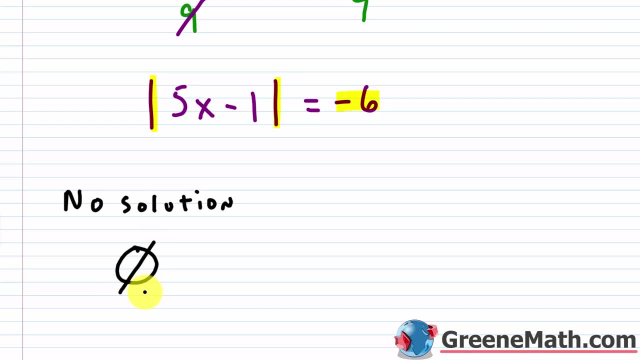 this. That's fine too, if you want to write that. It's basically anything you want to do. So again, I'm going to emphasize here why there's no solution, There's no value. I can plug in for x there. 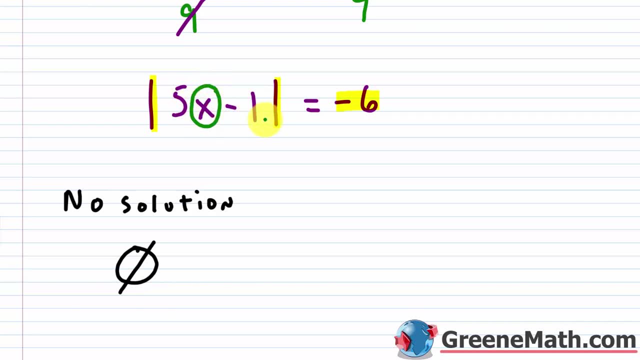 Multiply by 5, and then subtract away 1, and then take the absolute value of it and get negative 6.. It doesn't matter what this value is. Once I take the absolute value, it's either going to be 0 or positive, okay. 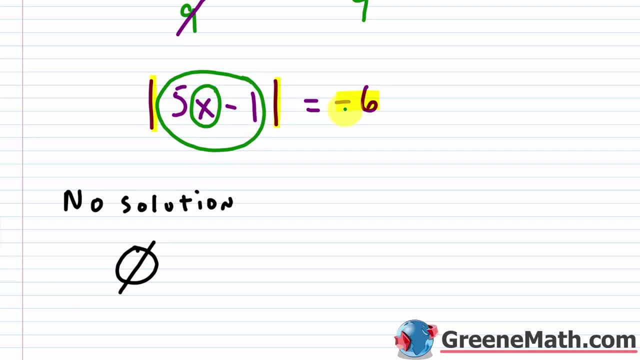 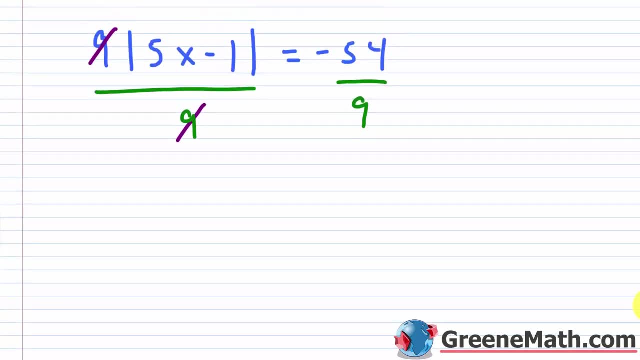 So it can never, ever, ever be negative 6. So that's why there's no solution. Now let me show you one thing real quick. I just want to make sure we're crystal clear on this before we move on. If, for example, I change this problem and I'm not going to go all the way through- 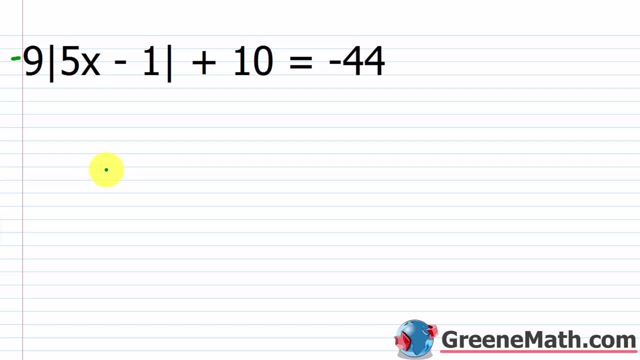 but if I change this problem to a negative out in front, you will have a solution. okay, Let's work through that real fast. I'm not going to go all the way through, but I'll just show you. If I subtract 10 away from each side here, that would cancel. 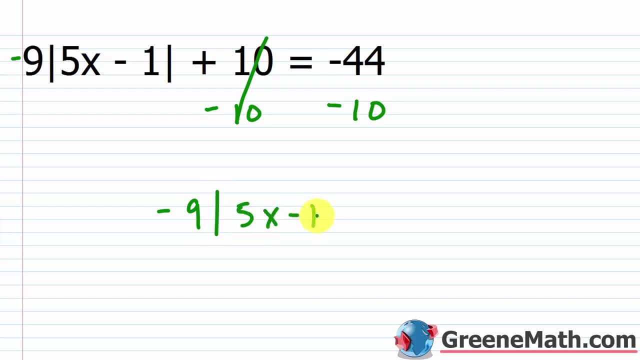 I'll have negative 9 times. the absolute value of 5x minus 1 is equal to negative. 44 minus 10 is negative 54.. Now if I divide both sides by negative 9, what's going to happen? Let's scroll down. 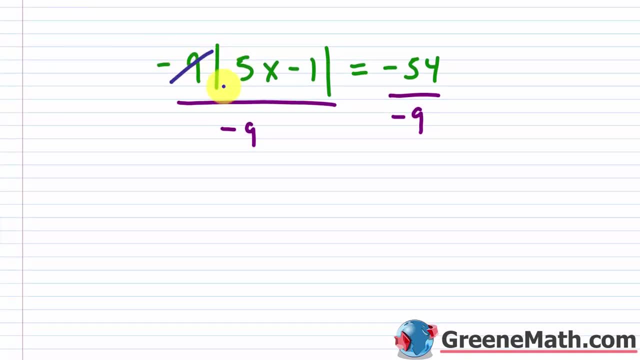 Let's scroll down and get some room. Well, we see that this guy right here cancels with this guy. So I've isolated the absolute value of 5x minus 1.. But now negative 54 over negative 9 is positive 6.. 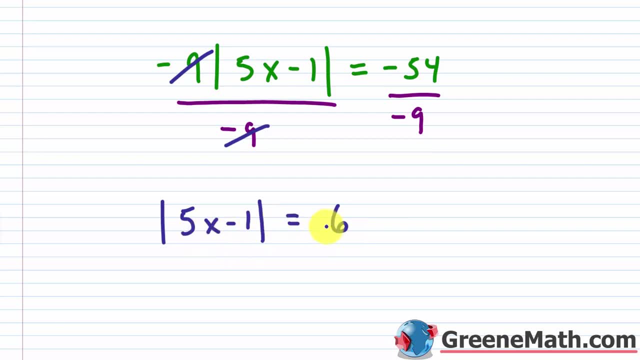 So I would have a solution here. I would have to set 5x minus 1 equal to 6, and then 5x minus 1 equal to negative 6.. So I would have that compound equation with OR and I would get two solutions there. 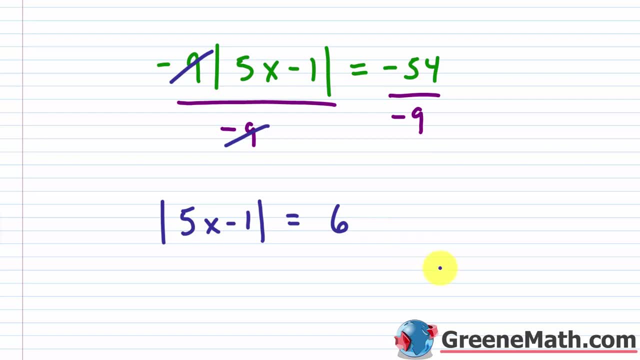 I'm not going to go through that process, but I'm just making sure that you understand that Just because I start with a negative on the right-hand side, I'm not going to go through that process- Just because I start with a negative on the left-hand side doesn't mean that I have no. 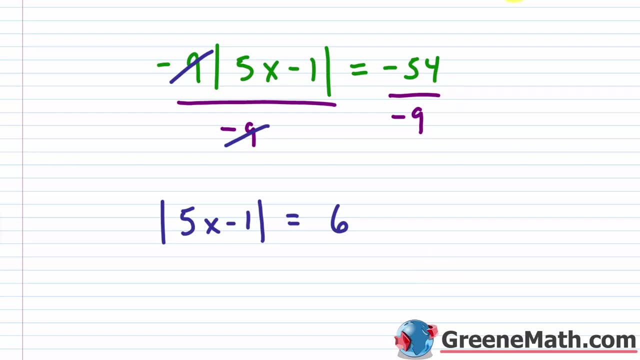 solution, You've got to get to the point where you've isolated the absolute value operation on one side and a number on the other. If the number is 0, then you're just going to have one solution, which we'll talk about in a minute. 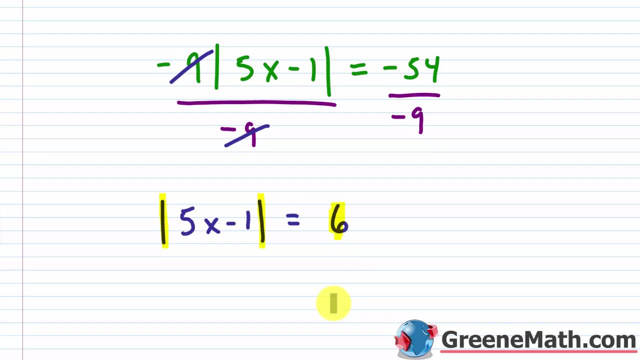 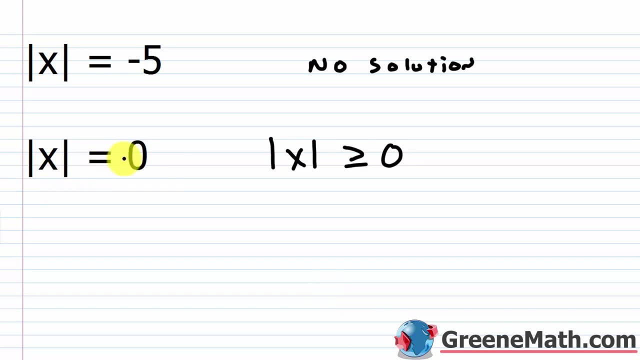 If it's positive, you're going to have two solutions, And if it's negative, you're going to have no solution. All right, Let's think about another scenario we're going to come across. So suppose the absolute value of x was equal to just 0.. 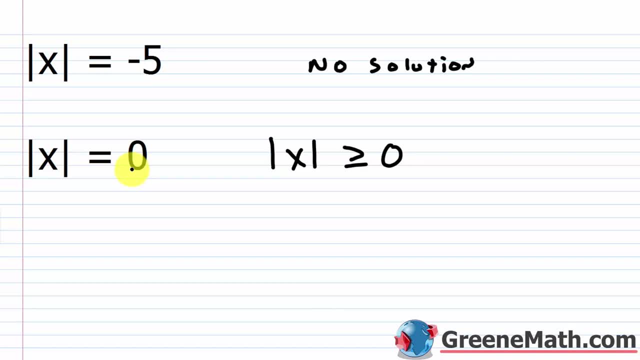 Well, in this case you're not going to have to set up a compound equation, You're just going to have one equation. The absolute value of x equals 0 only if x is equal to 0. That's the only possible solution there, because the only number that has an absolute value 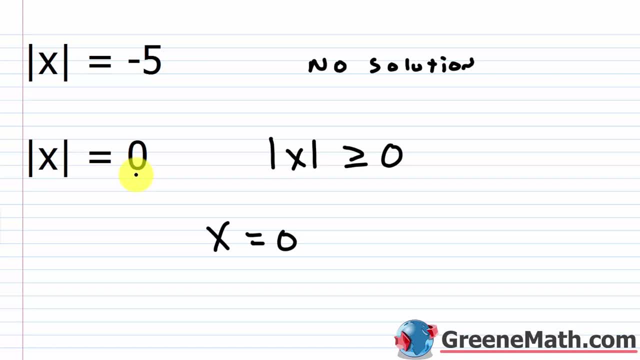 of 0 is just 0.. 0 doesn't have an opposite. If this was, the absolute value of x is equal to 2, again x could be 2, or it could be negative 2, because each have an absolute value of 2.. 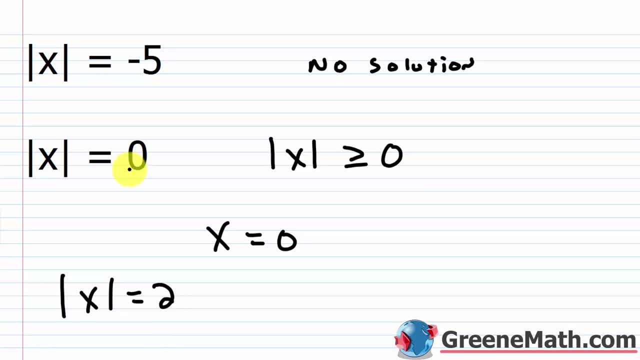 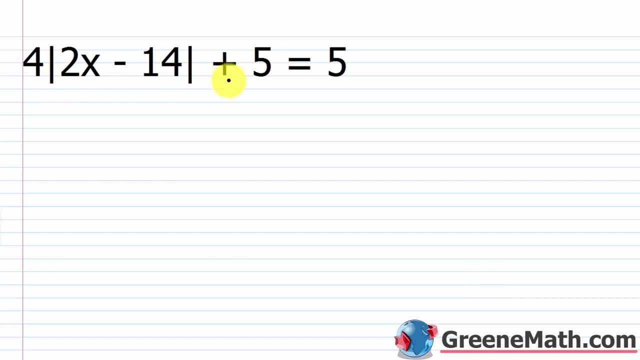 But when you get 0, there you only have one unique number that has an absolute value of 0. So let's look at this equation here. So we have 4 times the absolute value of 2x minus 14, then plus 5 is equal to 5.. 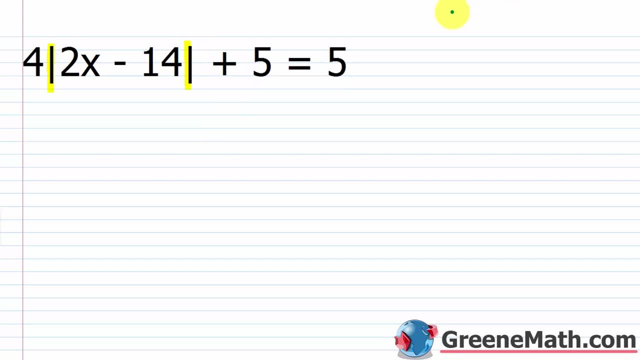 So again, our goal is always to isolate the absolute value operation, And when I subtract 5 away from each side, you're going to immediately see you have a problem. You get 4 times the absolute value of 2x minus 14, and this is equal to 0. 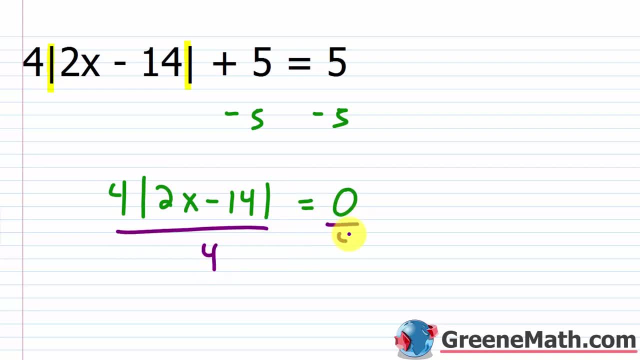 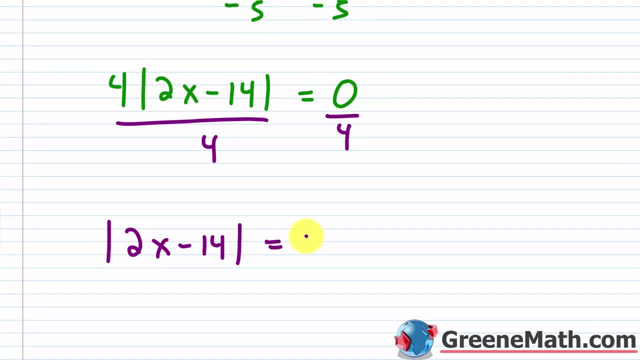 So if I divide both sides by 4, we know 0 divided by 4 is just 0, so I'm going to end up with: We have: 2x minus 14 is equal to 0. So this is a special case scenario, okay. 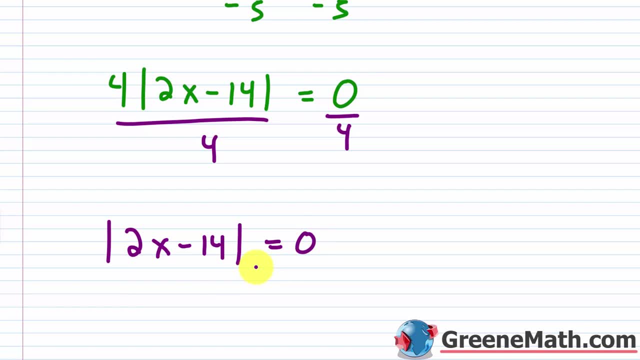 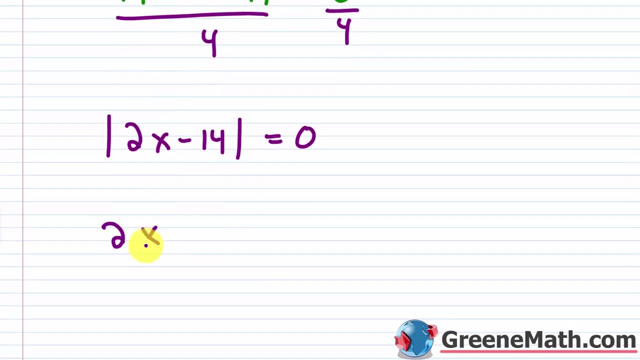 You do have a solution here, but you only have 1,. okay, You're not going to get 2.. So you need to pay close attention to what to do here. So all we need to do is say that 2x minus 14 is just equal to 0.. 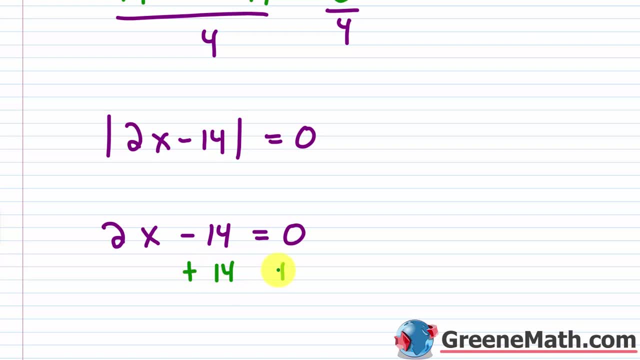 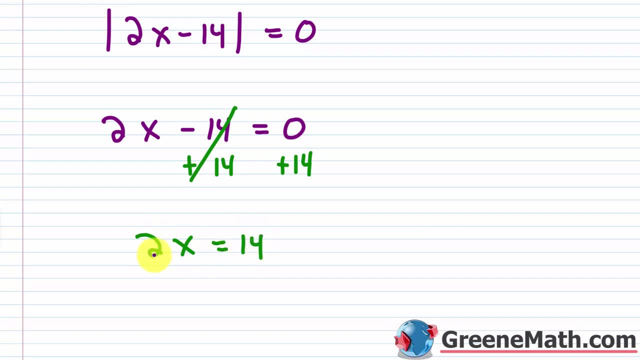 We're just going to solve that equation. So I'm going to add 14 to each side, And of course this is going to cancel. We'll have: 2x is equal to 14.. Then we're going to divide both sides by 2, and I'm going to get that x is just equal. 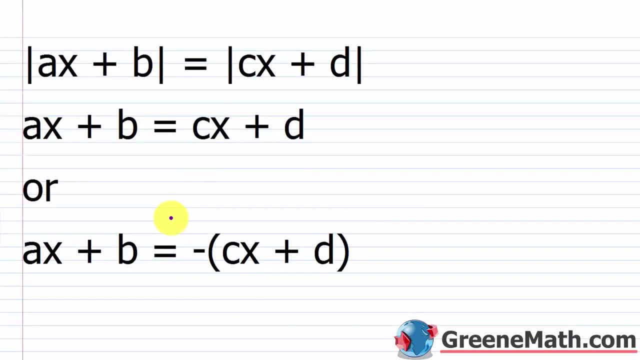 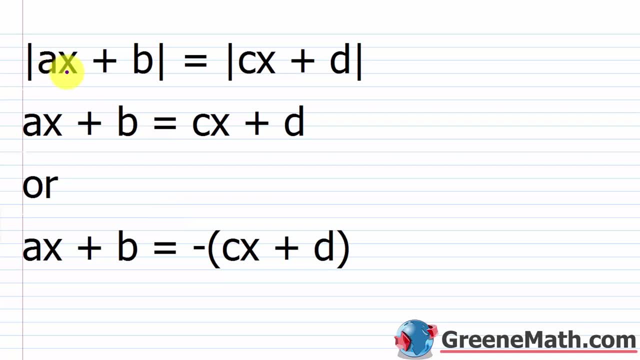 to 7.. So just one solution here: x equals 7.. So lastly, let's think about what happens when we have two absolute value operations set equal to each other. So something like the absolute value of ax plus b is equal to the absolute value of cx. 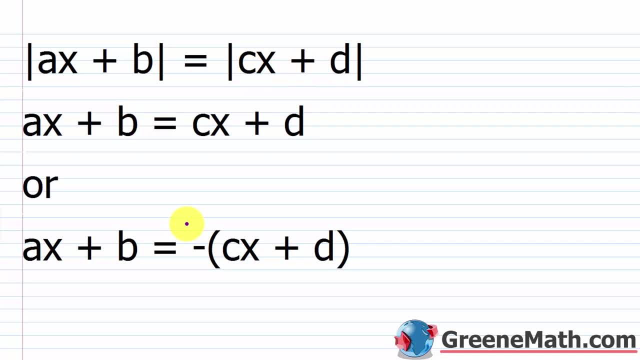 plus d. So the way we think about this is: two numbers or expressions can only have the same absolute value if they're equal to each other or if they're opposites of each other. So we would say: Let's say ax plus b is equal to cx plus d. 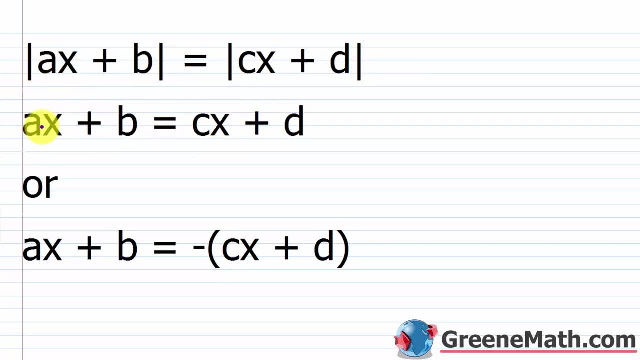 So, in the first scenario, just remove the absolute value bars and set the two expressions that were inside of the absolute value bars just equal to each other. Then or Next, you're going to remove the absolute value bars and you're going to put parentheses. 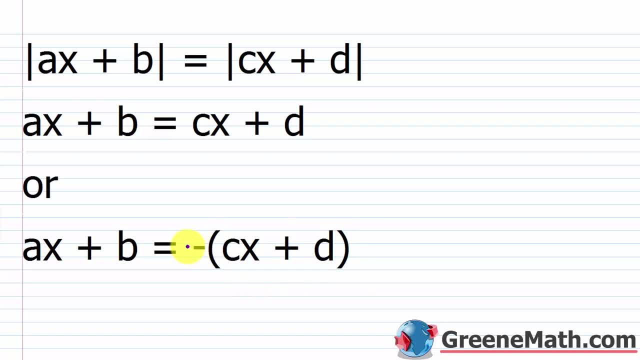 around one of the expressions and basically negate it. right, So you're going to put a negative sign in front of it or make it into its opposite. You can even put this as a negative one out in front, just to make it crystal clear what. 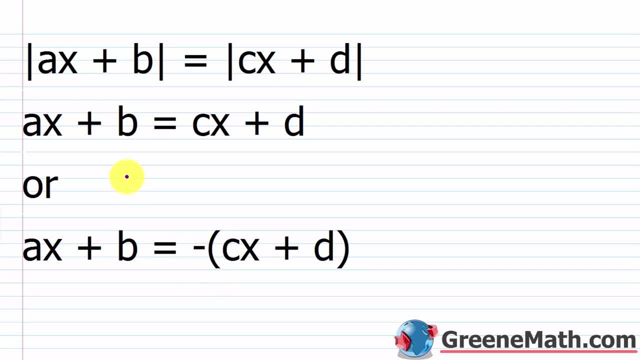 you're doing. And it would be just as valid if I said: or: and I put a negative out in front of ax plus b and said: this is equal to cx plus d. Just don't make them both negative. Only make one of them negative, because you need them to be opposites. 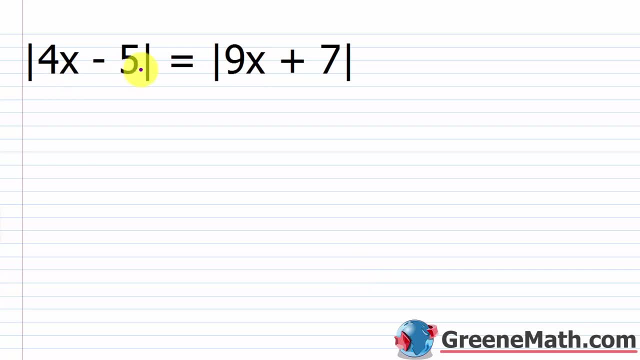 So let's look at our example We have: the absolute value of 4x minus 5 is equal to the absolute value of 9x plus 7.. So again, I'm going to drop the absolute value bars. So I'm just going to say this is: 4x minus 5 is equal to 9x plus 7.. 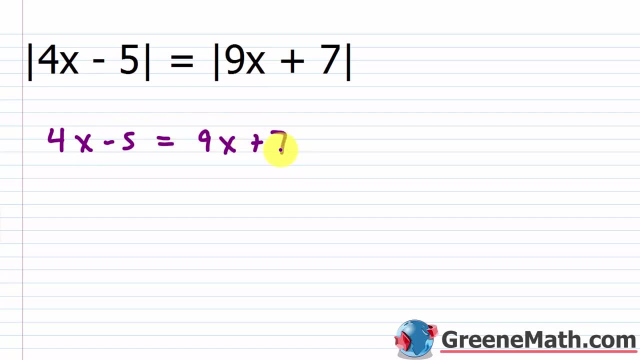 So I'm going to solve that. So I'm going to solve that. Okay, So I'm going to solve that. Then you have, or You have, or I'm going to drop the absolute value bars, So I'm going to have: 4x minus 5 is equal to. 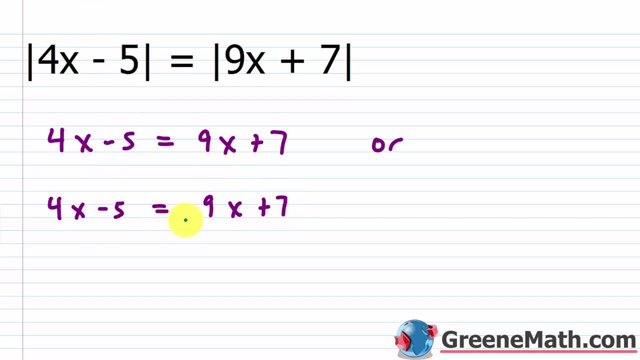 You have 9x plus 7.. So I'm going to choose one of these expressions- It doesn't matter which one you want- Wrap it in parentheses and put a negative out in front. okay, You could do this, one or again, doesn't matter. 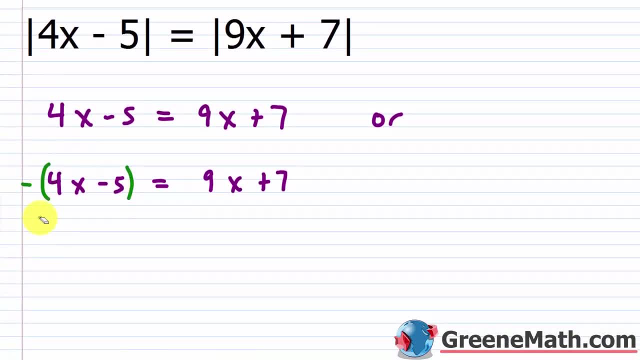 You can do this one. You will get the absolute same answer. Just for the sake of what we did earlier, I'm going to go ahead and just wrap this Okay Around here and just be done with okay. So for the first one, I'm just going to solve this. 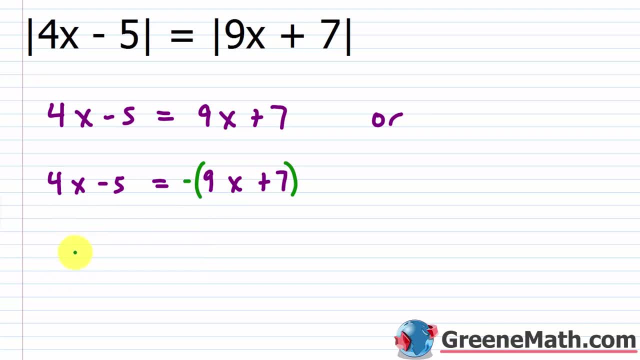 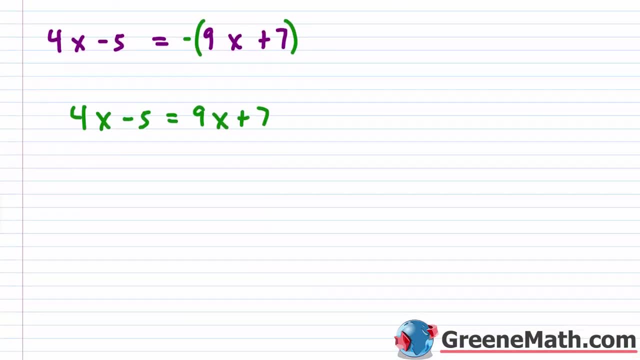 I'm going to write this down here. So we have 4x again. 4x minus 5 is equal to 9x plus 7.. Let me scroll down and I'll come back up. So to solve this is very, very easy. 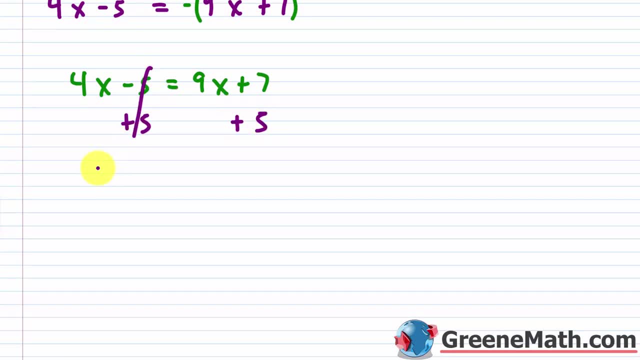 We just add five to each side of the equation. that cancels. 4x is equal to 9x plus 12.. We subtract 9x away from each side of the equation And this is going to cancel. So what I'm going to have is 4x minus 9x is negative 5x. 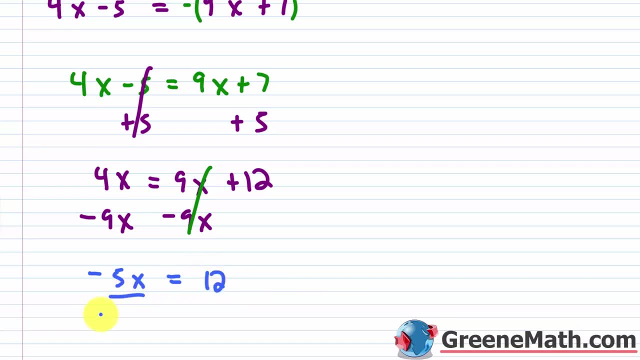 This is equal to 12.. We can go ahead and just divide each side of the equation by negative 5. We're going to find that x is equal to negative 12 fifths. So let's erase all of this. We're going to keep that x equals negative 12 fifths. 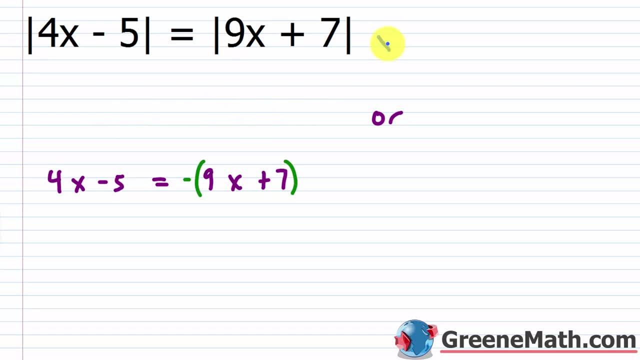 So I don't need this equation anymore. I'm just going to put x equals negative 12 fifths, And then I'm going to have my or. here I'm going to do it vertically, Then I'll have x equals something here. 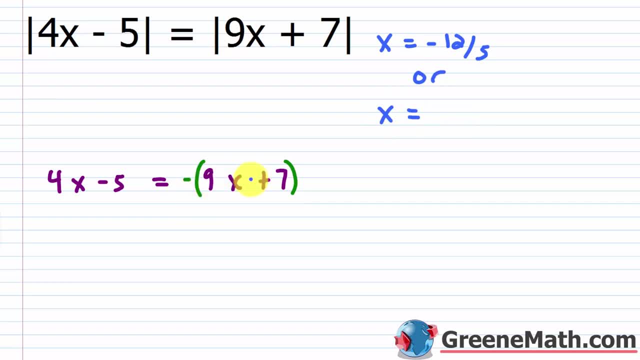 And we'll get that from this. So here I'm going to distribute my negative to each term. Again, if you have trouble with that, put a negative 1 there and then distribute. That's the easiest way to remember. So 4x minus 5 is equal to negative. 1 times 9x is negative 9x. 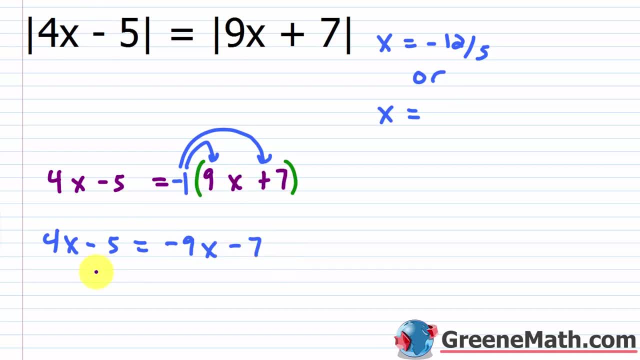 And then negative. 1 times 7 is minus 7.. Now what I want to do is add 5 to each side of the equation and add 9x to each side of the equation. So this is going to cancel, And this is going to cancel. 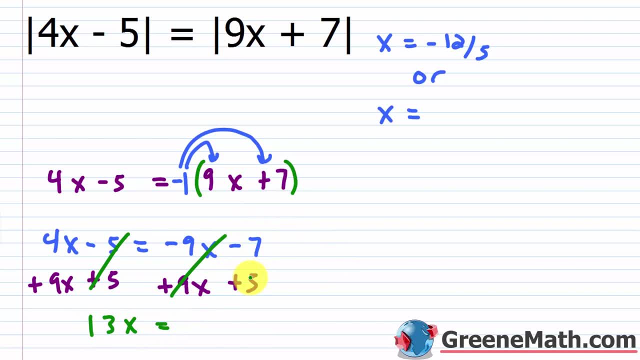 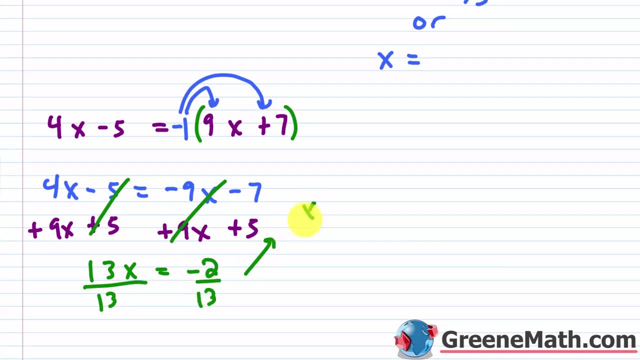 4x plus 9x is 13x. This is equal to negative 7 plus 5,, which is negative 2.. If we divide each side by 13,, we're going to get that x is equal to negative 2 13ths. 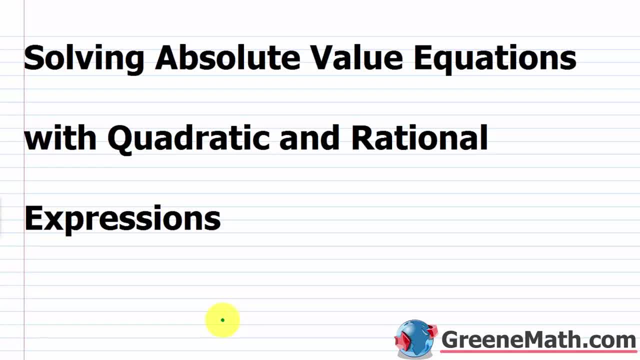 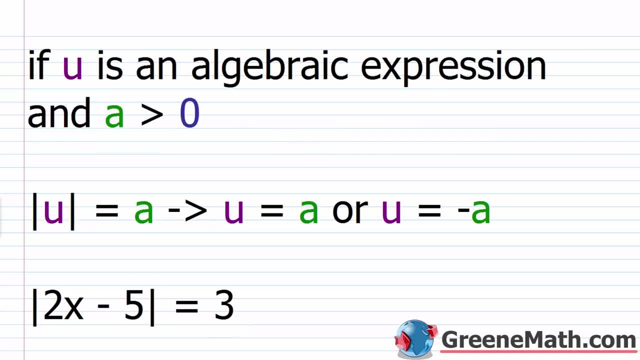 So x equals negative 2 13ths. In this lesson we want to talk about solving absolute value equations with quadratic and rational expressions. All right, so previously in our course we talked about how to solve kind of simple absolute value equations where basically we were only dealing with linear equations. okay, 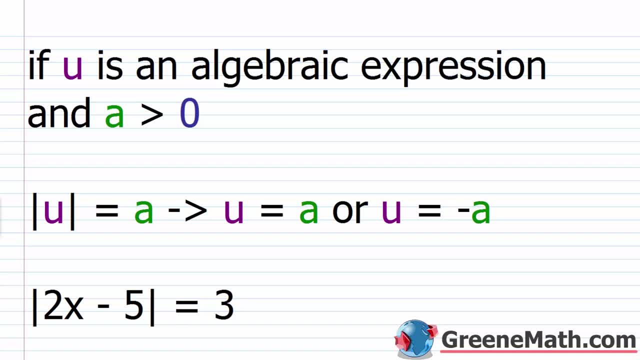 So we're going to go a little bit deeper into this topic and we're going to look at some additional examples that are slightly more challenging- You might say not more challenging, but more tedious- because we're going to involve some quadratic expressions and some rational expressions. So we'll end up having to solve some quadratic equations and also some rational. 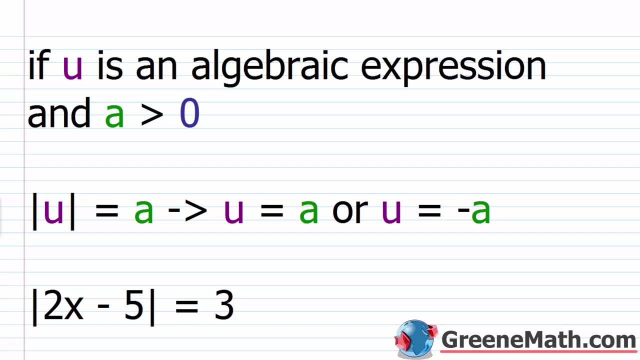 equations. okay, So we're going to boil this down to a little rule. If u is an algebraic expression and a is some positive number, so it's greater than zero. so it's not zero and it's not negative. right, Because zero and negative would each give us a special case. We'll talk about that in a 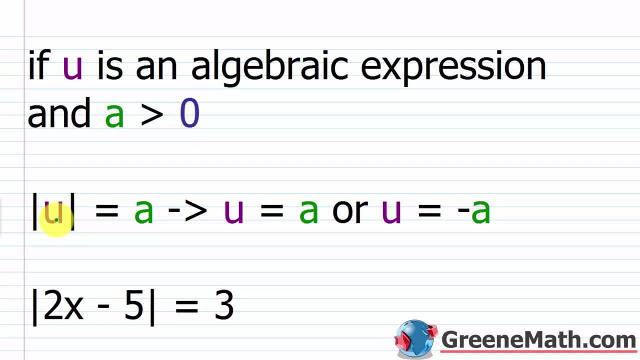 second, So the absolute value of this algebraic expression u. if that's set equal to this positive number a, then what we get is that the algebraic expression u could be equal to the positive number a, or the algebraic expression u could be set equal to. 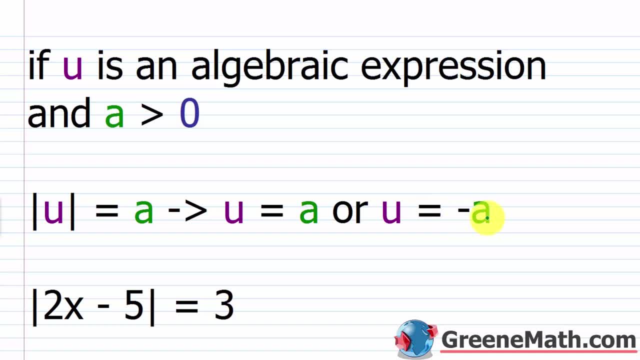 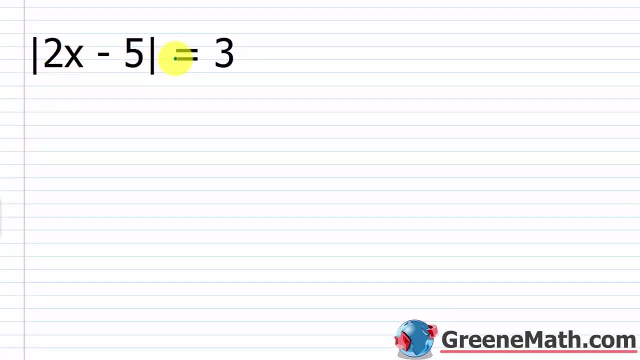 the negative of that number, a. okay, So as a quick example, this is something we already know how to do. Let's say we have the absolute value of 2x minus 5, and this is equal to 3.. The first thing is: 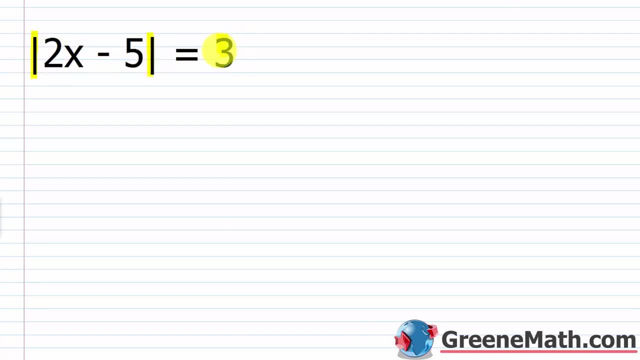 notice how the absolute value operation is isolated on one side and you have a positive number on the other. okay, So that's always what we want to set up. So then we can use our little rule Again. it's kind of cut off the screen here, but if the absolute value of some algebraic 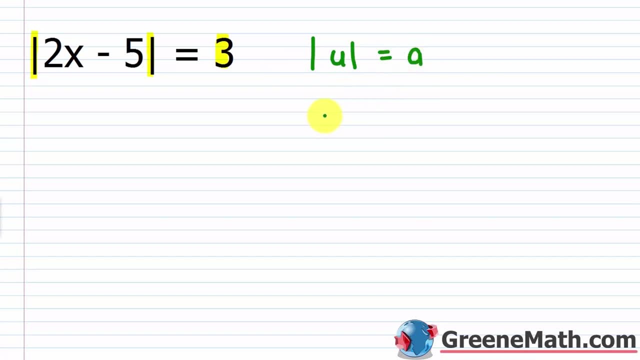 expression u is equal to some positive number, a, then u is equal to the absolute value of some algebraic expression, u equal to a or u is equal to negative a. we're just going to use that here again. this expression here: 2x minus 5, that's u, that's the algebraic expression, and then 3 is the positive number. 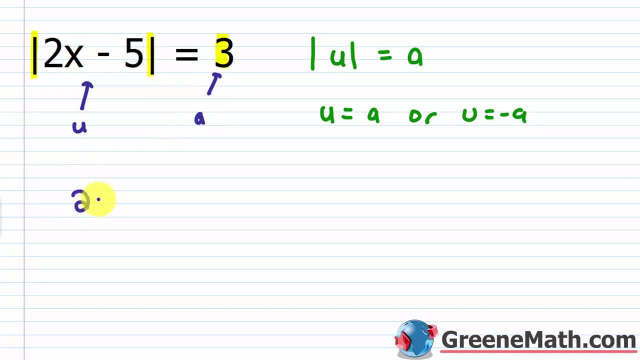 that's a, so i would say that 2x minus 5 could be equal to 3, or 2x minus 5 could be equal to negative 3.. now what we're basically saying is that this guy right here could be set equal to. 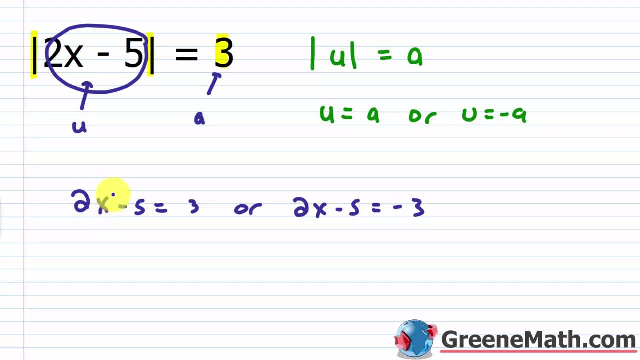 3. right, if i get a value for x that gives me a result of 3, i take the absolute value of that. i get 3.. also, this guy right here could be set equal to negative 3, because if this guy in here evaluates to negative 3, well, when i take the absolute value of negative 3, i also get 3 okay. so that's why this. 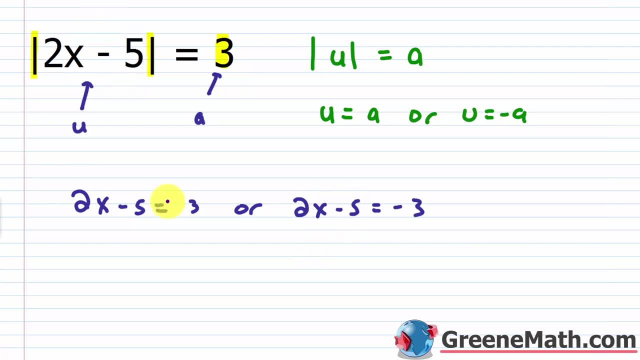 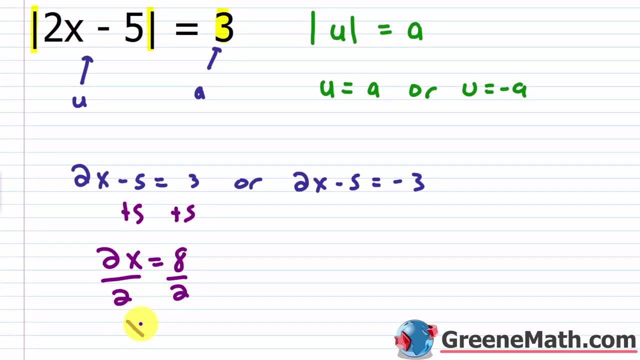 ends up working itself out. so let's just solve this real quick. i'm going to add 5 to both sides of the equation. i'm going to get that. 2x is equal to 8. divide both sides by 2. i'm going to get that. 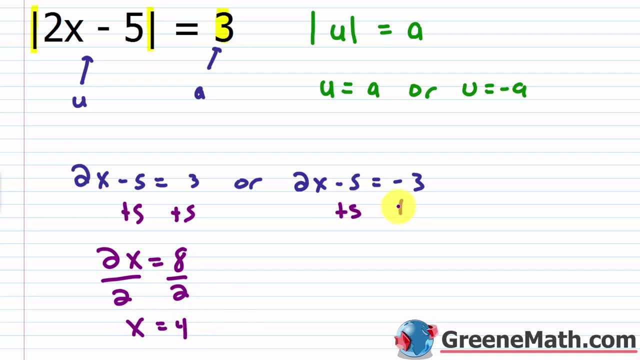 x is equal to 4.. over here, i'm going to add 5 to both sides. i'm going to get that 2x is equal to negative. 3 plus 5 is 2. divide both sides by 2. i'm going to get that x is equal to 1. okay, so we get x equals 4. 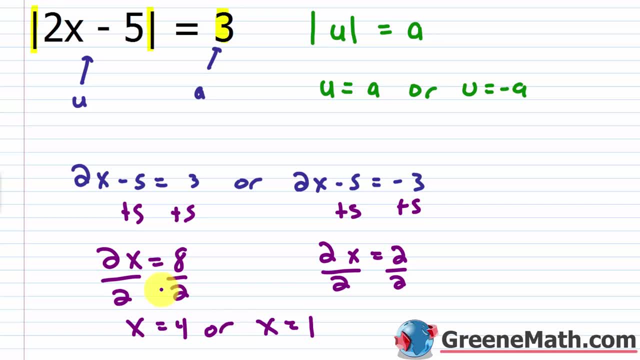 or x equals 1.. now you can easily check that. you can plug in a 4 for x there and basically, 2 times 4 is 8, 8 minus 5 is going to be 3, right, so you know, with the absolute value of 3, which is 3, 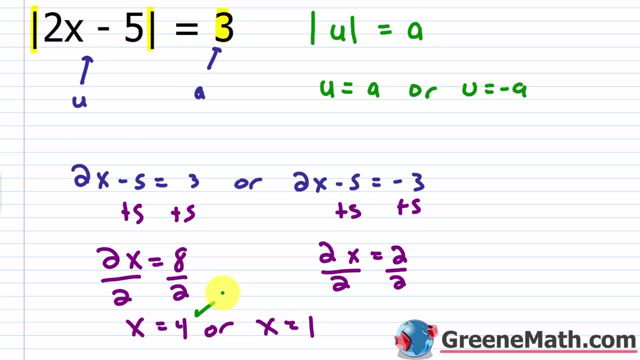 so that works itself out okay. the other scenario is going to give you the absolute value of negative 3, because that's also going to give you 3.. right, if i plug in a 1 for x, 2 times 1 is 2, 2 minus 5 is negative 3: again the absolute value of negative. 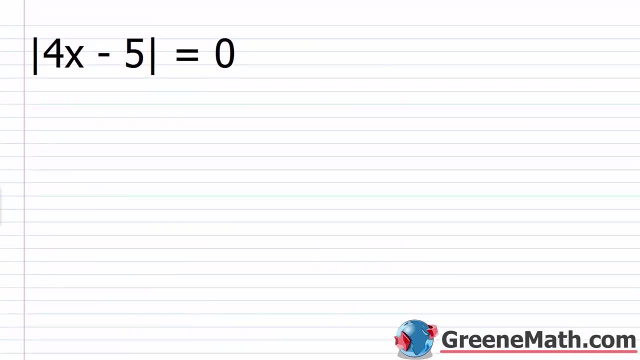 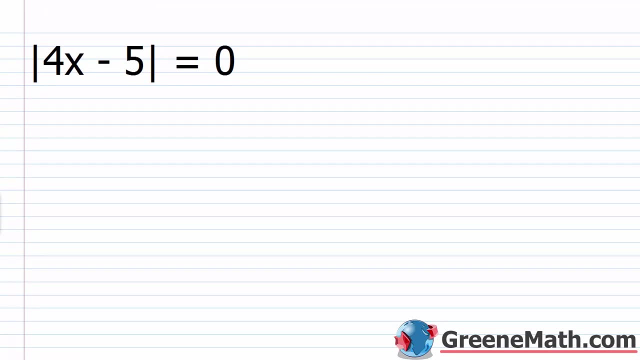 3 is also 3, so this works as well. all right, so before we go any further, we have to understand the special cases that we might run across, and we covered these earlier in the kind of course when we talked about absolute value equations. but we need to kind of jog your memory so that 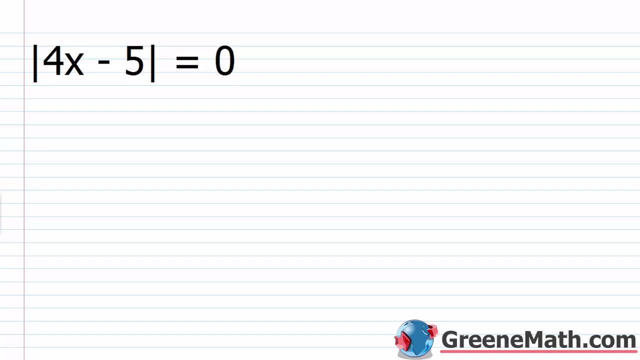 you are ready for all the scenarios you're given. so let's say you have the absolute value of 4x minus 5 and this is equal to 0.. well, what happens is if this guy is isolated and it's set equal to 0. well, think about the fact that 0 is 0 units away from. 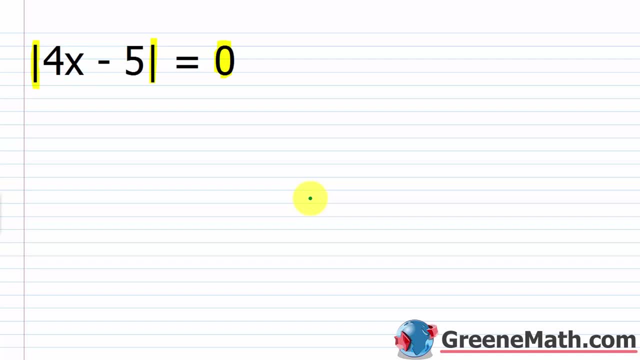 itself on the number line, right? so the only number that's going to have an absolute value of 0 is 0.. okay, so you're not going to have a compound equation with or. here you just have to set 4x minus 5, this expression equal to 0, and then just solve. okay, so this is a little bit easier. 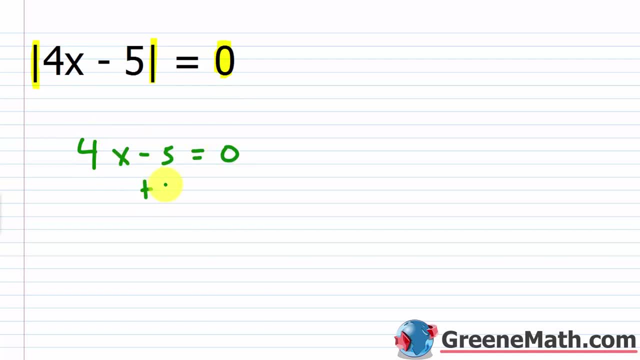 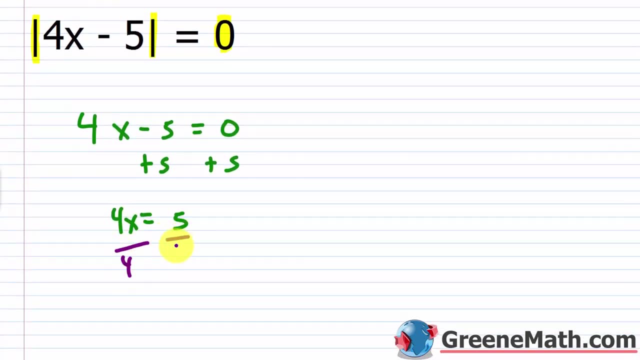 a little less tedious. so to get our solution there, we just add 5 to both sides of the equation. 4x is equal to 5 and let's divide both sides of the equation by 4 and we'll find that x is equal to 5- 4. okay, and obviously if we check that, if you plugged in a 5- 4 there 4 times 5, 4, the 4s would. 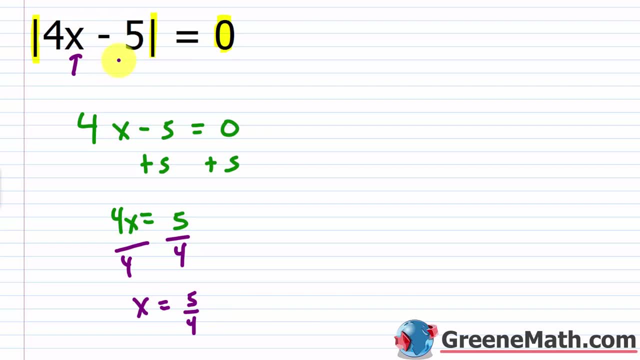 cancel. you just have a 5. 5 minus 5 is 0. the absolute value of 0 is 0, so that checks itself out as well. all right. last special case scenario is: if the absolute value operation is isolated and it's equal to some negative value, there's no solution. okay, and the reason for that is the 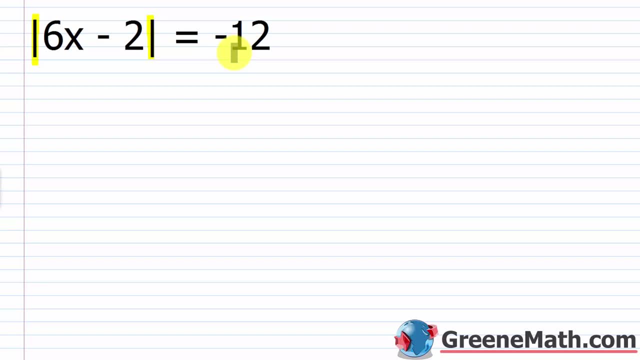 absolute value operation. takes a negative, it makes it positive. takes 0 and spits out 0. takes a positive and spits out the positive. okay, so you can't plug in anything for x here and then multiply it by 6. that guy subtract away 2, right. take the absolute value and end up with a negative. 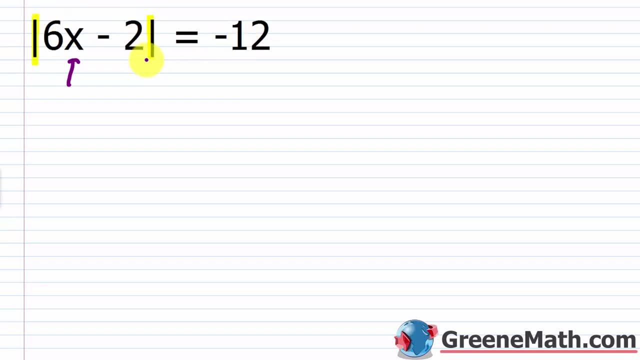 12.. right, because the absolute value operation is going to kind of stop all that, because it will never ever be equal to some negative value. so you can't get a negative 12 as an answer for that. so this is the solution. okay, so it's no solution. so we can use our symbol for the null or empty set. 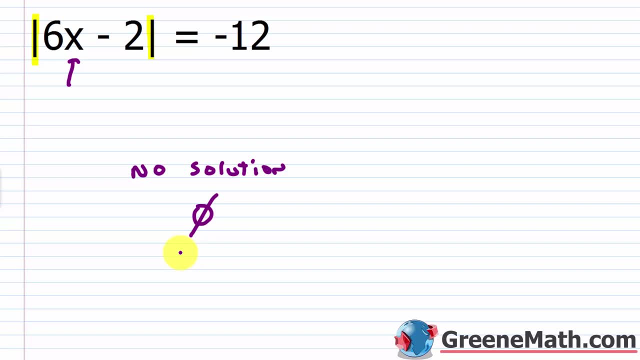 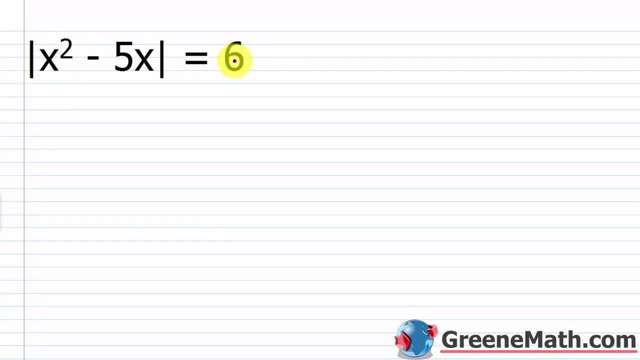 all right. so now let's jump in and look at some problems where we have some quadratic expressions involved. so suppose we have the absolute value of x squared minus 5x and this is set equal to 6.. so we have exactly what we talked about earlier: we have the absolute value of some expression u 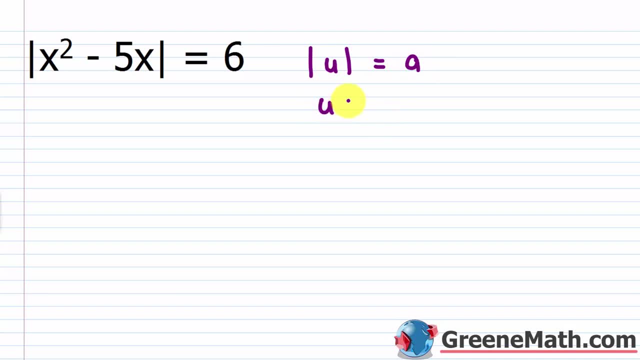 and it's set equal to some positive number, a. well then, u could be a or u could be the negative of: okay, so it's the same concept, we're just using kind of more complex expressions. so we would have x squared minus 5x, x squared minus 5x. we'd set that equal to 6 then, or we'd have x squared minus. 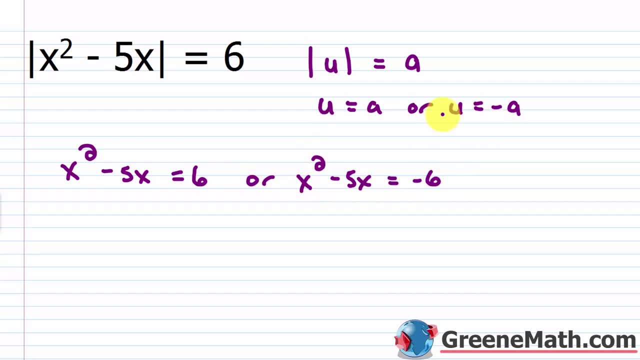 5x would be equal to negative 6. okay, all i did was follow this. this expression is my u, this guy right here, this number is my a. okay, so i'm just following that, just like we saw. okay, so now i can solve each of these. they're kind of easy quadratic equations to solve because they're both factorable. 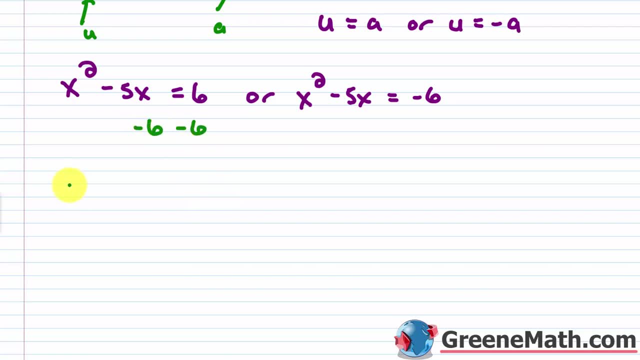 i can subtract 6 away from each side of the equation here, i would have that x squared minus 5x minus 6 equals 0, and i'll go ahead and solve this real quick. so, as i alluded to, this can be factored the left side here, if i think about two integers whose sum is negative 5 and whose product. 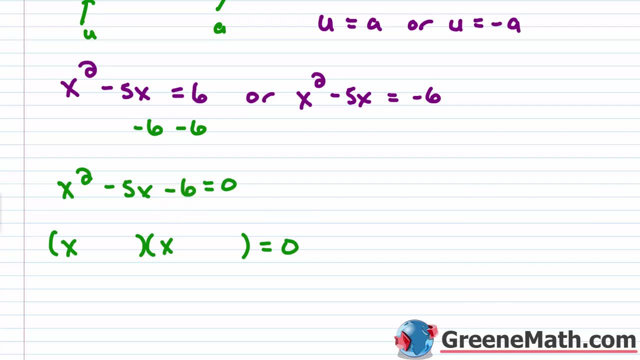 is negative 6 when you think about negative 6 and positive 1. right, negative 6 and positive, positive, 1.. Because negative 6 times positive, 1 would give you negative 6.. Negative 6 plus 1 would give you negative 5.. So this is our factorization here. Then we would set each 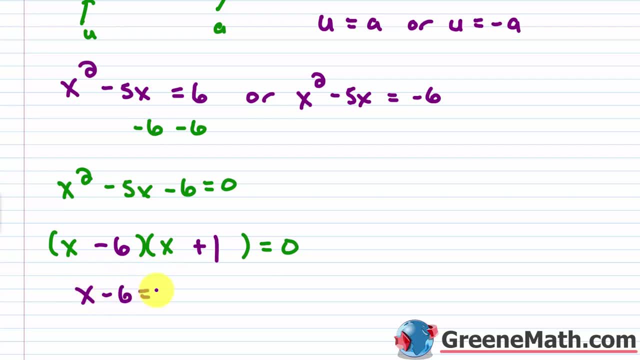 factor here equal to 0. So x minus 6 would be equal to 0. And then we'd also have x plus 1 equal to 0. And let's go ahead and solve that. So we would add 6 to both sides of the equation here. 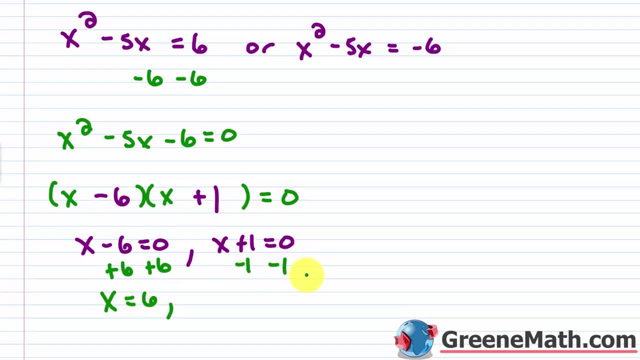 x is equal to 6.. Over here I subtract 1 away from each side of the equation, So x is equal to negative 1.. So the two solutions here are that x equals 6 or x can be negative 1.. So let me kind of copy this, because this is going to get a little bit too busy, And let me kind of 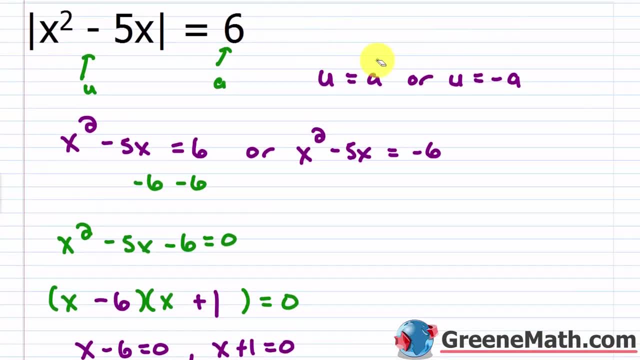 come back up here for a second And I'm just going to erase this. We already know the rule And I'll just kind of paste this in here. So those are two solutions. I'm going to go ahead and get rid of this whole branch. We don't need it anymore. All right, So for this one, 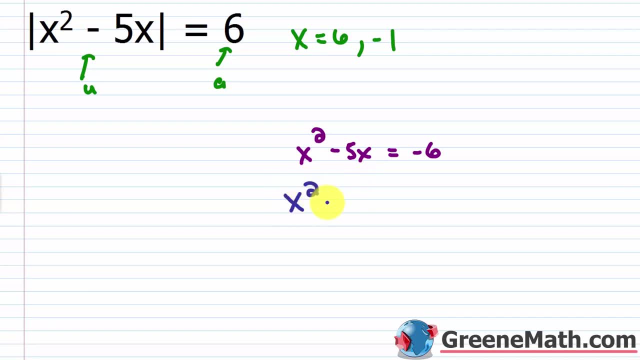 it's another easy one we can solve with factoring. So we have x squared Minus 5x. I'm going to add 6 to both sides, So plus 6 equals 0.. So I'm going to factor this guy. 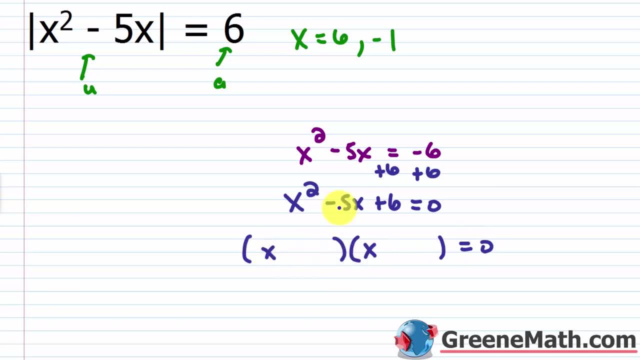 So this is x and this is x. Give me two integers whose sum is negative 5 and whose product is positive 6.. Well, that would be negative 2 and negative 3, right? Negative 2 times negative 3 is positive 6.. Negative 2 plus negative 3 is negative 5.. So we're good to go there. 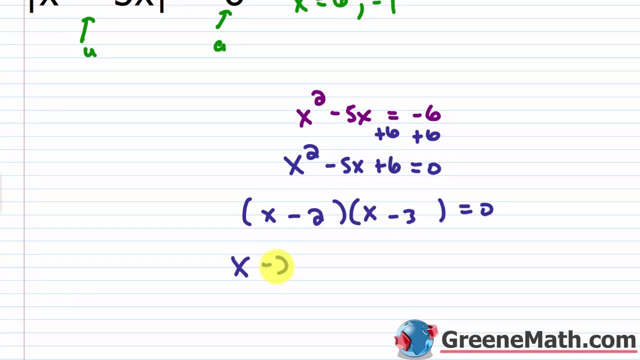 All right. So what we want to do is just set each factor equal to 0. So x minus 2 equals 0. And then x minus 3. Add 2 to both sides of the equation here You're going to get that x is equal to 2.. 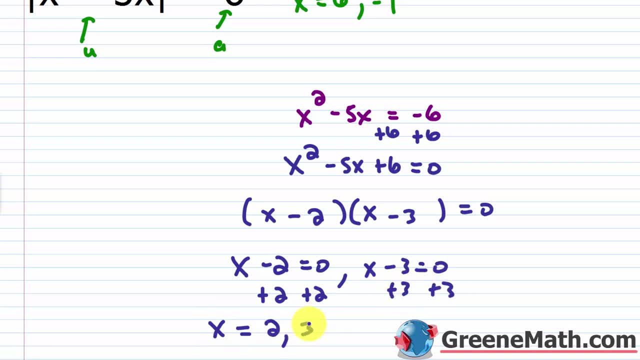 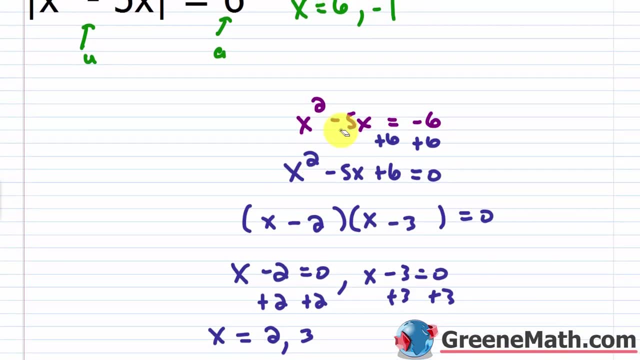 Add 3 to both sides of the equation here You'll get that x is equal to 3.. Okay, So x equals 2 or 3.. Those are another two solutions, So let's just write those in right here. Let me erase all this. 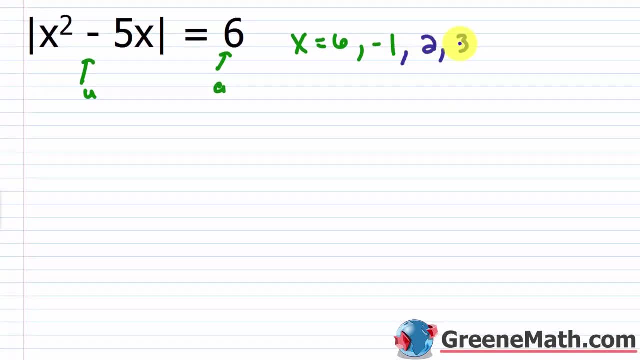 So let's pop those in here. So 2 and then 3.. So a little bit more tedious And you actually have more solutions here. You have four solutions, Whereas the problems we looked at before. in most cases you had two solutions right And you can go through and plug all these in. 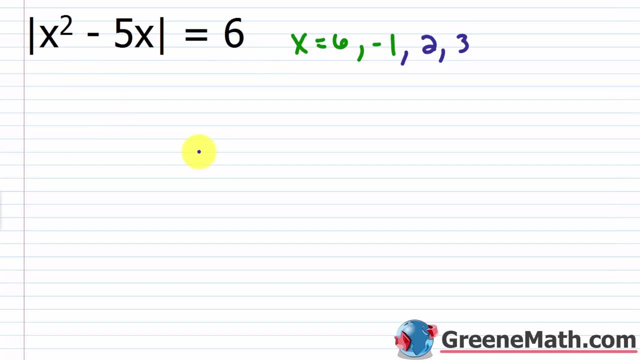 And verify they work. And just for this one, we can go ahead and check it just to see what happens. For the rest of them, I'm not going to check it just in the interest of time, But I just want to show you that you're going to have two of these that are going to evaluate here to be the absolute. 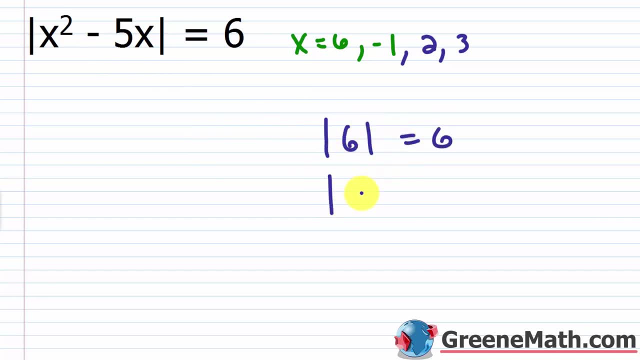 value of 6.. So that's going to work out. Then the other two are going to evaluate to be the absolute value of negative 6.. So those are going to work out as well, right? Because in each case, the absolute value of 6 or the absolute value of negative 6, it produces 6.. So the left and the 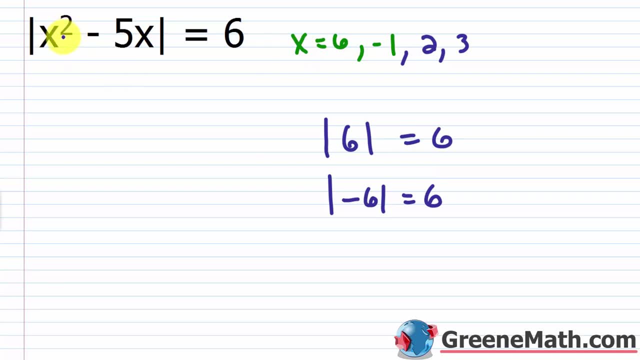 right side will be equal. Okay, So for this scenario, 6 squared is 36.. So you'd have 36 minus 5 times 6, which is 30.. 36 minus 30 is 6.. So it's this scenario here. 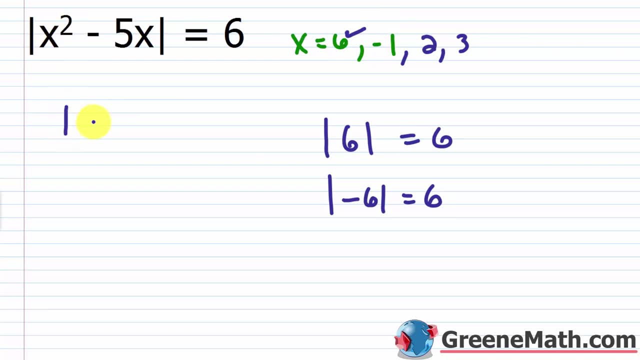 So this one works. Then, for this one here, negative 1, squared is 1.. Then you have negative 5 times negative 1, which is positive 5. So you sum those and you get 6. So again this scenario. 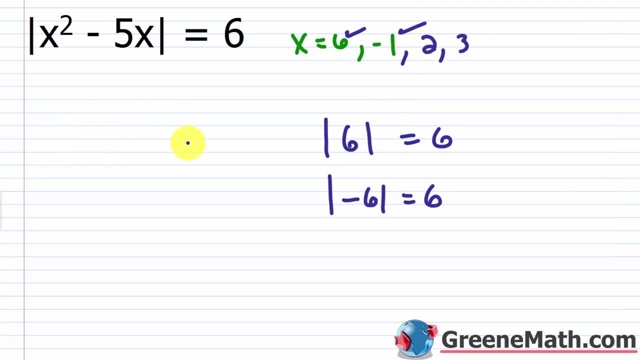 here So that one would work. Then for these two, you're going to end up with negative 6, right? So 2 squared is 4 minus You have 5 times 2, which is 10.. 4 minus 10 is negative 6.. So that's. 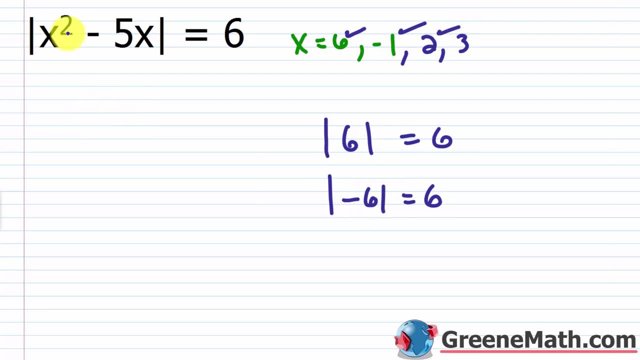 this scenario here, So that works. then the other one: plug in a 3: 3 squared is 9 minus you have 5 times 3, which is 15. 9 minus 15 is also negative 6, so this guy is going to work as well, right? so in this scenario again, we want: 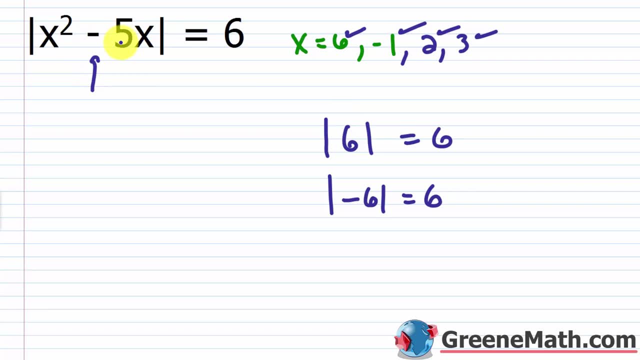 the inside of this guy right here. we want that expression to evaluate to either 6- right, that's this scenario here- or negative 6, that's this scenario here. either way, we'd end up with an answer of 6. so 6 equals 6, so our solutions here are correct. all right, let's take a look at one. 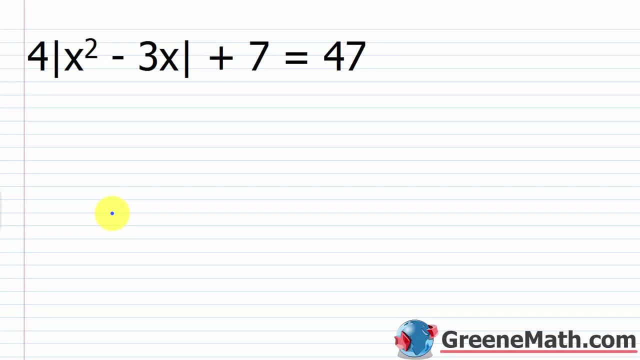 that's a little bit more challenging. it's just more tedious. we have 4 times the absolute value of x squared minus 3x plus 7 equals 47. okay, so in this particular case, our absolute value operation is not isolated. okay, we know from earlier in the course that we've got to have it isolated. 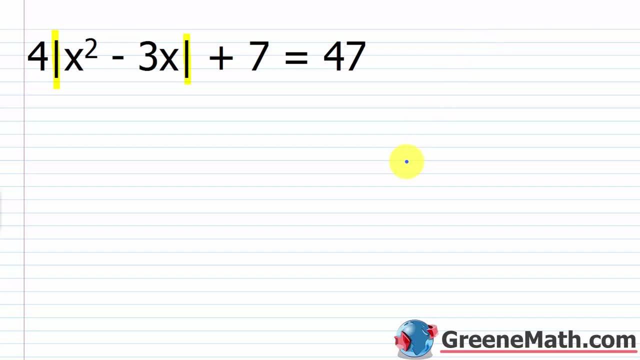 we can't just start doing stuff. i see a lot of students when they get this, they go: okay, well, this is 4 times the absolute value of x squared minus 3x. you know, plus 7 equals 47. and then they do this again and they say: okay, 4 times the absolute value of x squared minus 3x. plus 7 equals 47. 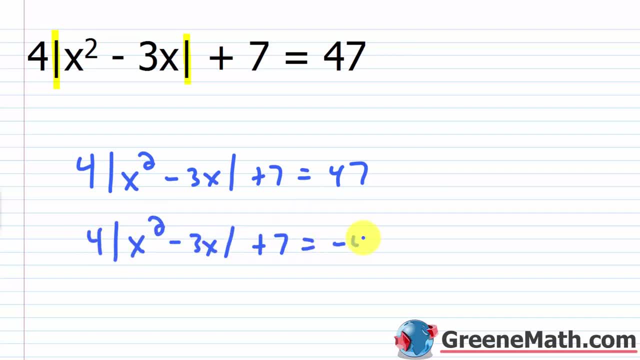 no, remember. your rule is that the absolute value of u- okay, this is isolated. if that's equal to a, then u equals a, or u equals the negative of a. okay, but this has to be isolated. notice how there's nothing else besides that absolute value of u. so if it's not isolated, you've got to do a little. 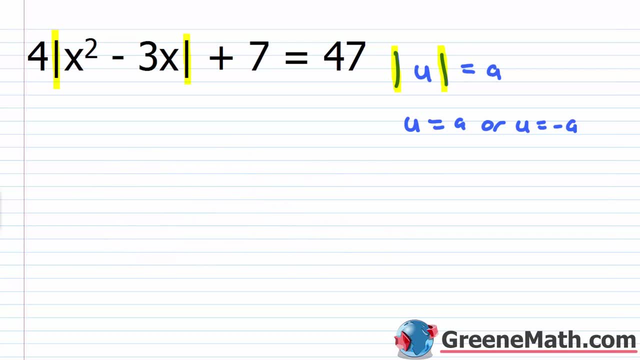 bit of work to kind of get things set up. get things started first, okay, so let's go ahead and subtract 7 from the absolute value of x squared minus 3x. plus 7 equals negative 47. away from each side of the equation, we'd have 4 times the absolute value of x squared minus 3x. 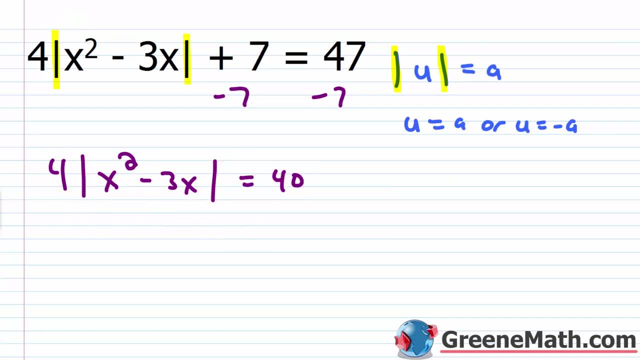 and then this is equal to 40.. now i can divide both sides of the equation by 4, right, because that's what's multiplying this guy. so this cancels. you'll have the absolute value of x squared minus 3x is equal to 10.. okay, so this is something we can deal with. this is something that matches this. 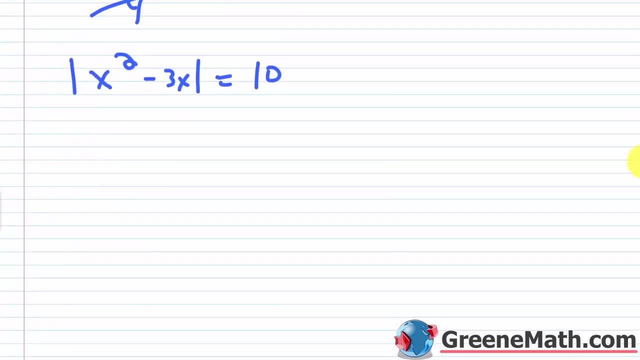 format. here again, just a little bit of extra work, but not too bad overall. okay. so let's go ahead and look at the first two cases. so the first case is that x squared minus 3x, this algebraic expression is equal to 10. okay then. or the second case is that x squared minus 3x is equal to the negative. 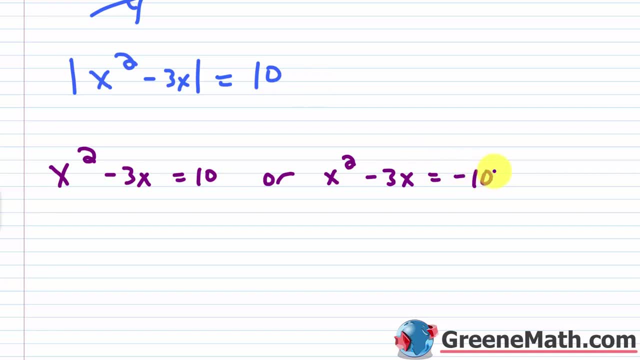 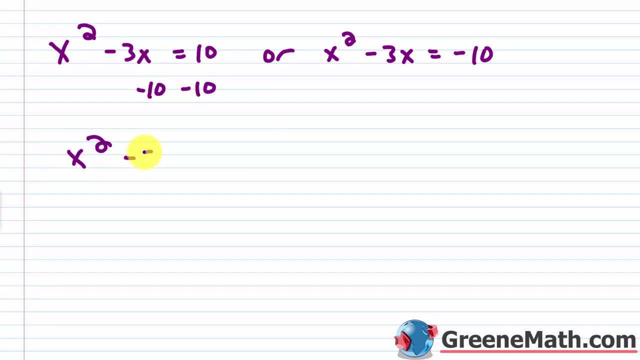 of 10, or just say negative 10. and now i'm just going to solve these two equations. so let's kind of scroll down, get some room going. this guy right here, i'll subtract away 10 from each side of the equation. i'm going to have that x squared minus 3x minus 10 is equal to 0 and i can solve this guy. 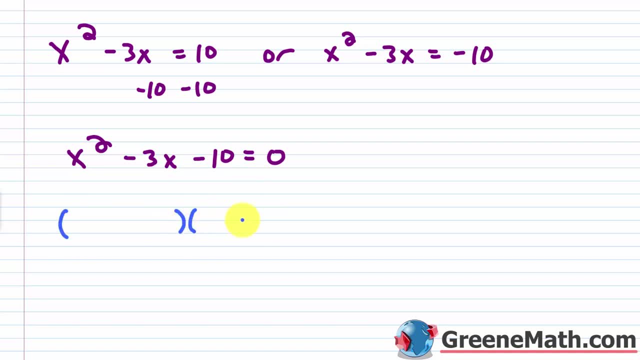 with factoring. so the left side of this guy. i can set this up as x here and x here. give me two integers that sum to negative 3 and then have a product of negative 10. that's going to be negative 5 and positive 2, right? negative 5 times positive 2 would give me negative 10. negative 5 plus 2 would. 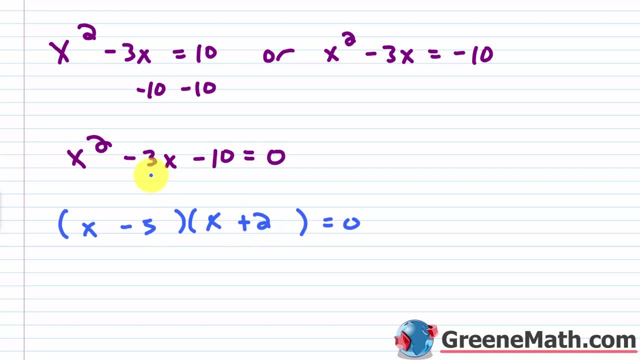 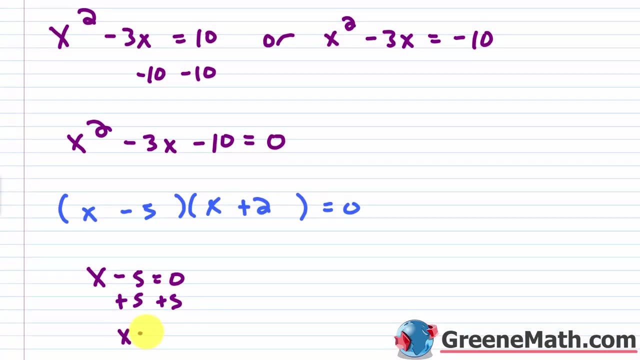 give me a negative 3.. so let's set each factor equal to 0. so i'll say x minus 5 equals 0. add 5 to each side of the equation. i get x is equal to 0 to 5.. then over here i would say: x plus 2 is equal to 0. subtract 2 away from each side of the equation. 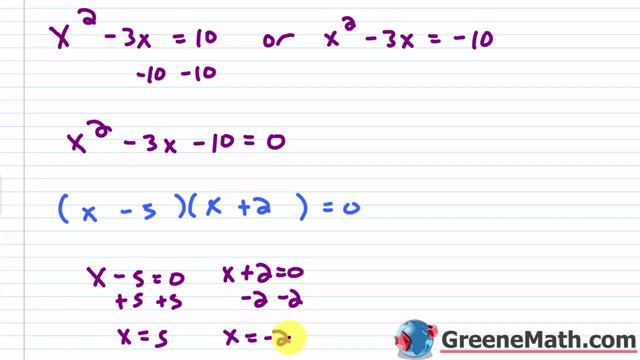 i get: x is equal to negative 2.. so those are two solutions. we've got x equals 5 and x equals negative 2.. so let me erase this part. we don't need it anymore because we already have the solutions. i'm just going to erase this and i'm going to go back to the top. 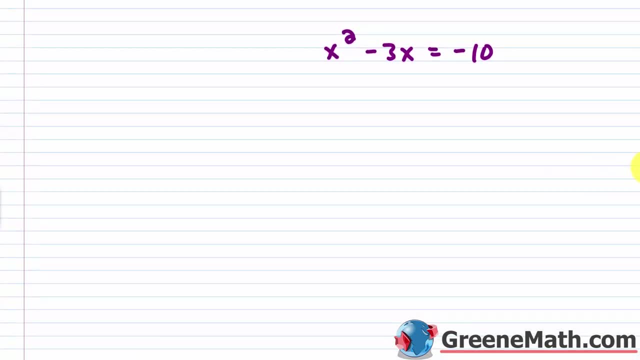 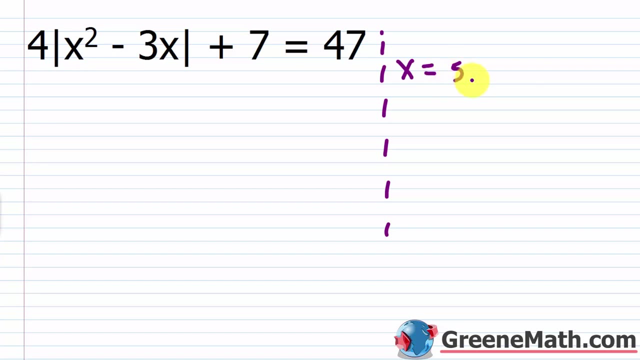 and just kind of write my answers up there, because the screen is just going to get a little too full. okay, so i'm just going to write that x is equal to. again we have 5 and then negative 2. okay, so let me go down, and now we're just going to solve this equation here. 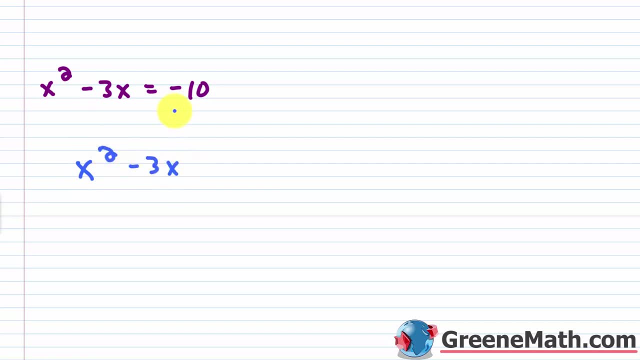 okay. so we have x squared minus 3x. i'm going to add 10 to both sides of the equation, so plus 10, this equals 0.. so unfortunately, this guy is not going to be factorable. this is something we need to use our quadratic formula to get a solution for. so, with our 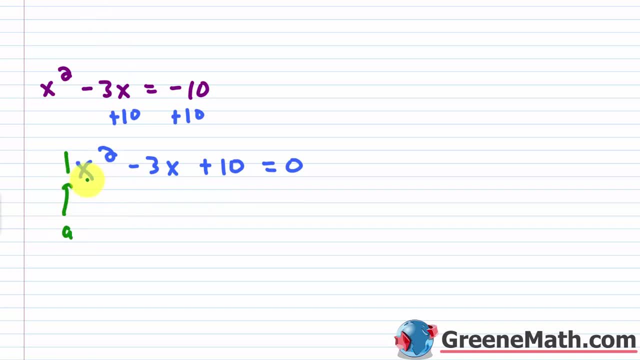 quadratic formula. we're going to label this as a right. we have a, 1, an understood coefficient there, so 2a a squared. so for the second equation, we got x squared, 2x squared. we're going to label this, this negative 3, as b. we're going to label this, this 10, this constant, as c. so 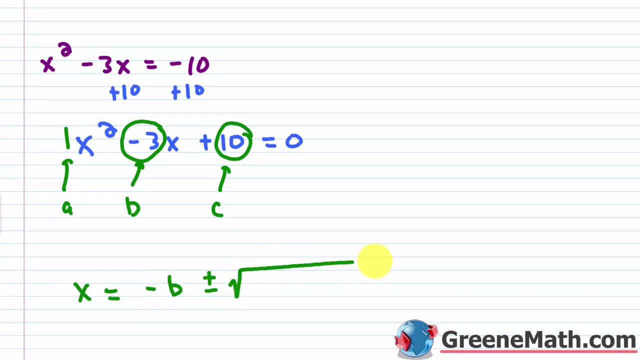 the quadratic formula, if you will recall, x is equal to the negative of b, plus or minus the square root of. you've got your b squared minus your 4ac all over 2a. so what is b? again, that's negative 3. so the negative of negative 3 is 3.. i'm going to go ahead and write it down here. then negative 3 squared would be 9.. so what is b plus or minus 3 squared? minus b squared acting on negative 3 would be 9.. 7 is y, which means 10.. keep ale everywhere with me until you get to. 11 will be my character. so what's b squared minus 3 is a. you're able to going with that further, so let me do that. 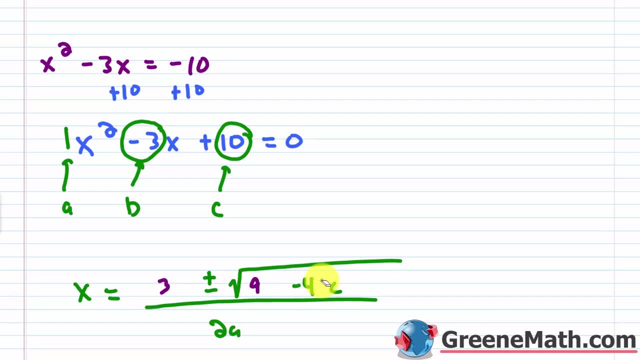 so negative 4 times 1 is just negative 4, then times 10,, which is c, negative 4 times 10, is negative 40, so you would have 9 minus 40,. 9 minus 40 is going to be negative 31,, so this is negative. 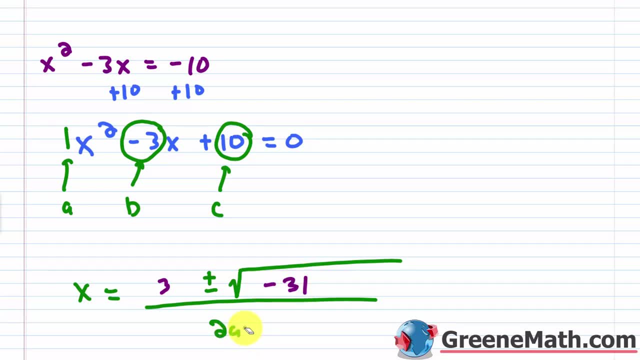 31 here, and then a again is 1, so this is just 2,. okay, so x equals 3 plus or minus the square root of negative 31 over 2, we can clean this up by using our imaginary unit, so we'll say x is: 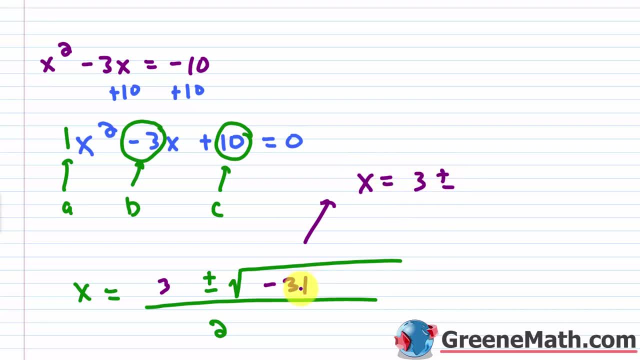 equal to 3 plus or minus. I'm going to pull the negative out as i times the square root of 31,. again, this is over 2, okay. so again this is two solutions. it's 3 plus i times square root of 31. 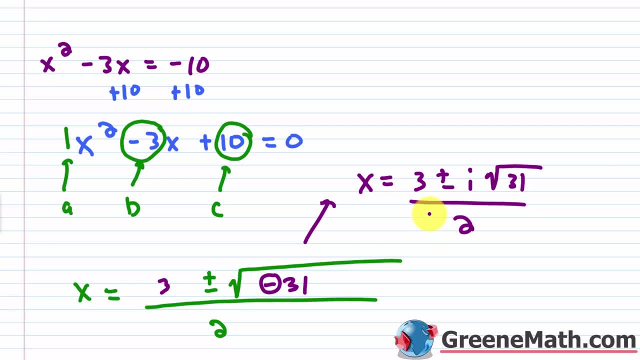 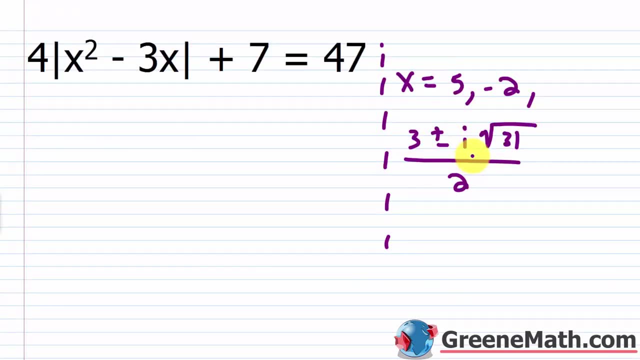 over 2, and it's 3 minus i times square root of 31 over 2,. okay, so let me copy this and I'm going to erase everything else. okay, so I'll put comma and I'll put this here. 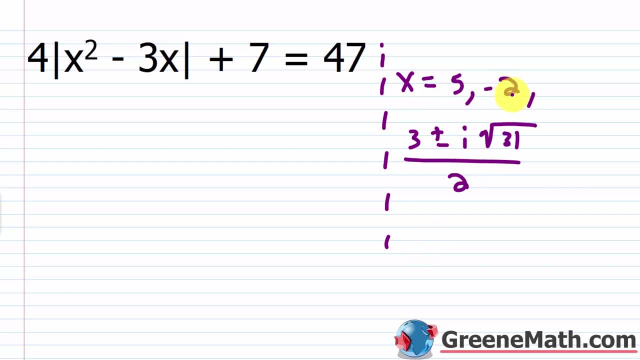 so we have four solutions: x can be 5, x can be negative, 2, x can be 3 plus i times square root of 31 over 2.. And then, lastly, x can be 3 minus i times square root of 31 over. 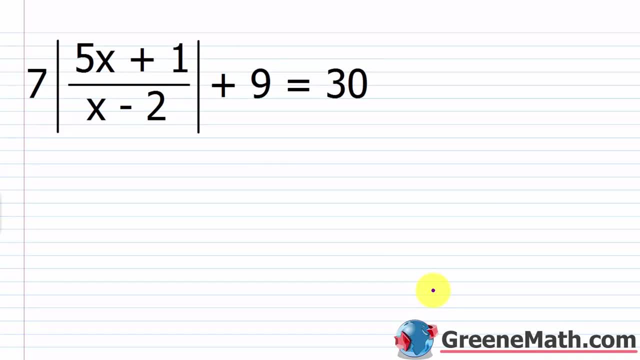 2.. All right, let's move on and look at one with a rational expression involved. So here we have 7 times the absolute value of. we have 5x plus 1 over x minus 2, then plus 9,. 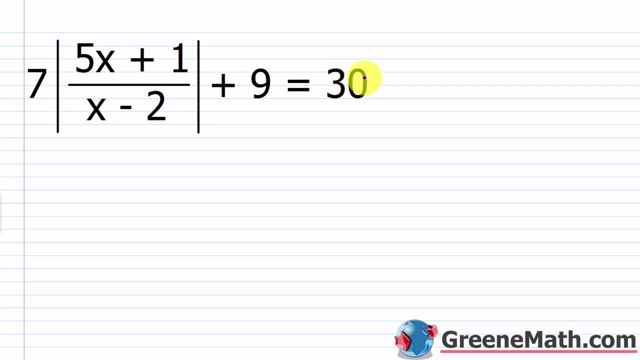 this equals 30.. So again, it's the same thing. What we want to do is isolate this absolute value operation Because again I'm just going to write this rule- the absolute value of u, this algebraic expression u, which is this: in this case, if that's equal to some positive number, a, then u. 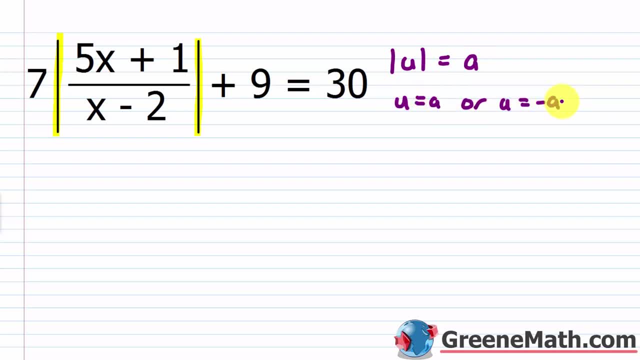 equals a or u equals negative a. So what can we do? Let's just subtract 9 away from each side of equation. We're going to have that 7 times the absolute value of 5x plus 1 over x minus 2 is 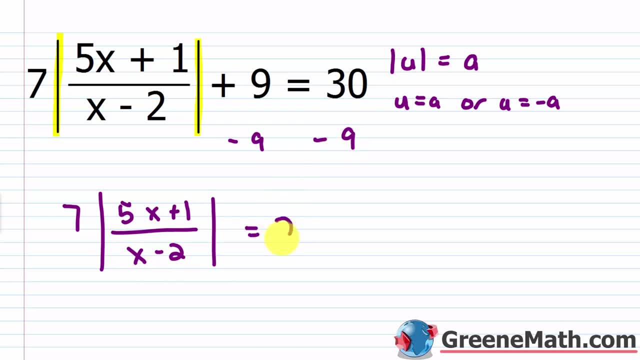 equal to 30 minus 9 is going to be 21.. So 7 is multiplying this absolute value operation. So let's divide both sides. Let's divide both sides by 7. And that's going to get us to what This cancels at the absolute. 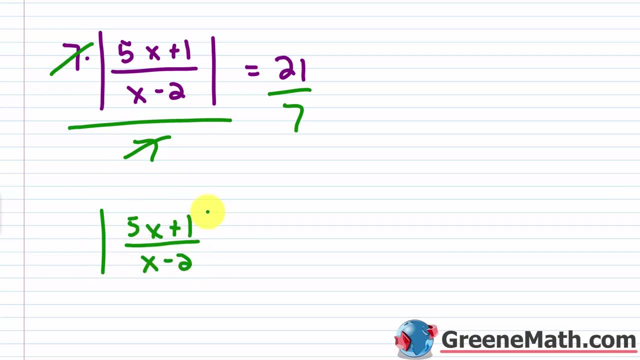 value of 5x plus 1 over x minus 2.. And this is equal to 21 over 7 is 3.. Okay, So at this point again I have an absolute value operation that's isolated. on one side I've got a positive number. 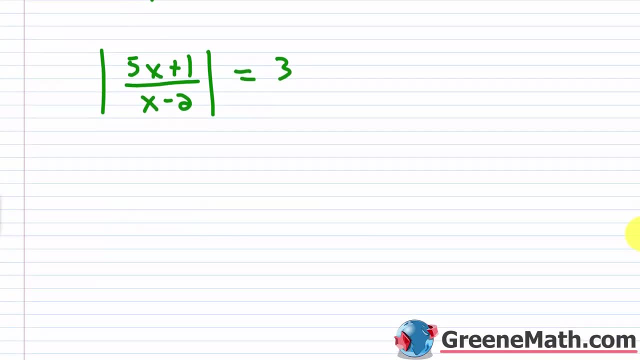 on the other. So I can go ahead and just use my rule, And what I'm going to say is that I have 5x plus 1 over x minus 2, that's set equal to 3.. Then, or we have 5x plus 1 over x minus 2, that's equal to negative 3.. Okay, So pretty easy to solve. 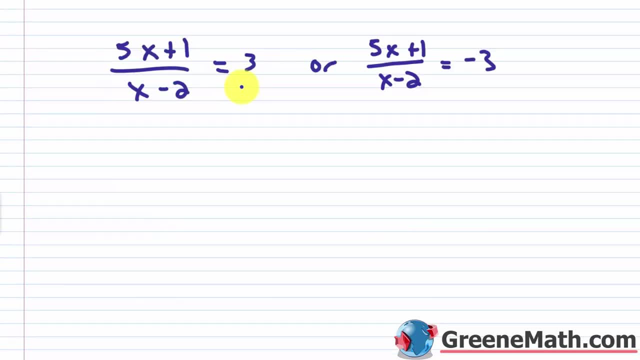 these In each case. here it's going to be quickest to just cross multiply, So I'm going to just write this as 3 over 1.. I'm going to write this as negative 3 over 1.. So x minus 2 times 3 would be. 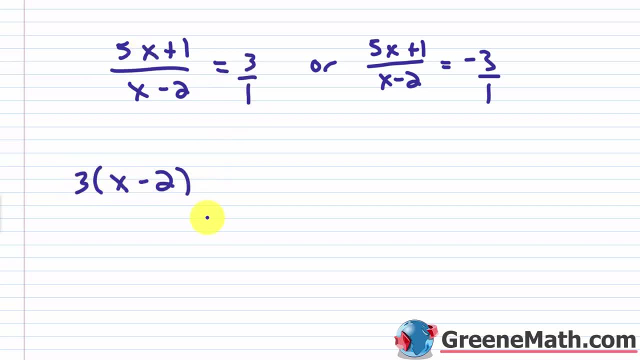 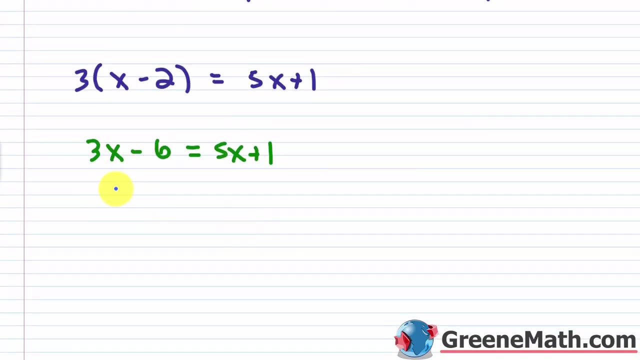 3 times the quantity x minus 2.. And then 1 times 5x plus 1 is just 5x plus 1.. Okay, So if I go through, use my distributive property, this would be: 3x minus 6 is equal to 5x plus 1.. Alright, so to solve this we can just: 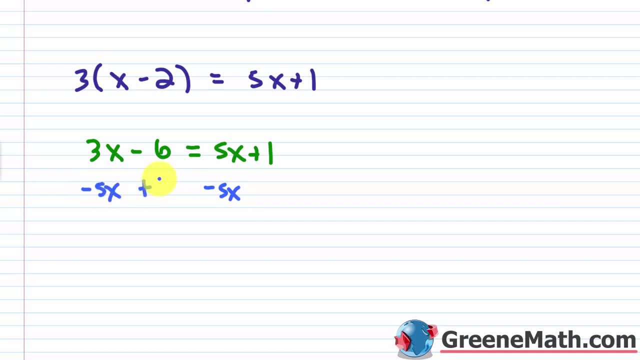 subtract 5x away from each side of the equation and then add 6 to each side of the equation, So we know this cancels and this cancels. 3x minus 5x is negative 2x. This is equal to 1 plus 6,. 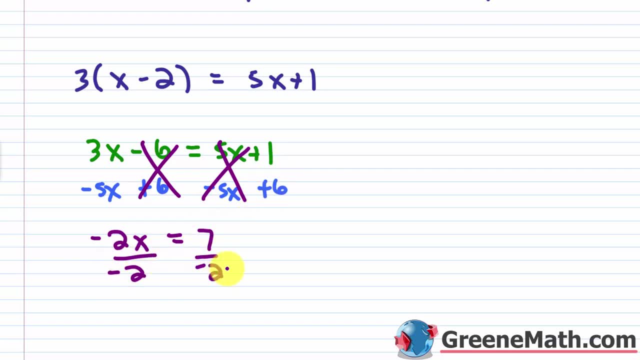 which is 7. Divide both sides by negative 2. And we're going to end up with x is equal to negative 7 halves. Okay, Okay, So that's one solution. Let me kind of erase this, because the screen gets just too packed And I'll. 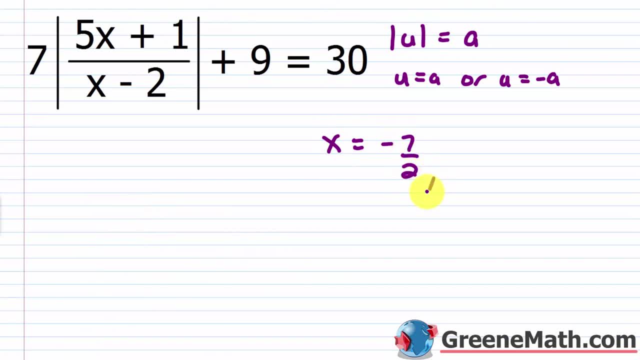 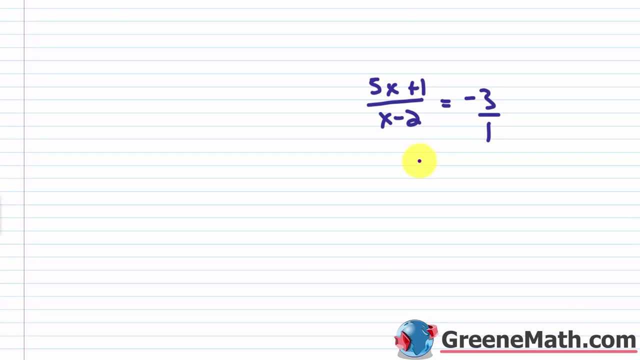 just say that x is equal to negative 7 halves. Okay, That's one solution. We're going to have another, So let's go back down. So now let's work on this one Again. I'm just going to cross, multiply So I would have negative 3 times the quantity x minus 2. This is equal to 1 times the. 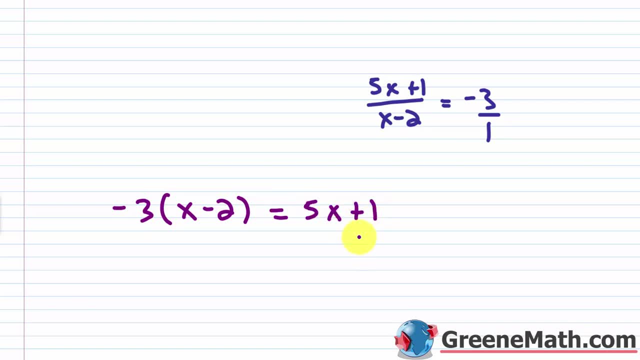 quantity 5x plus 1, which is just 5x plus 1.. Okay, So negative 3 times x is negative 3x. Negative 3 times negative 3 is negative 3x. So that's one solution. We're going to have another solution. 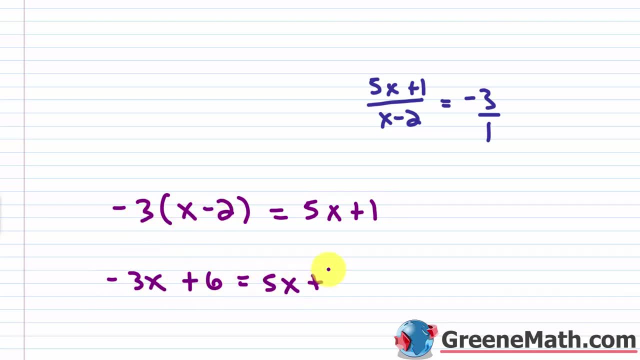 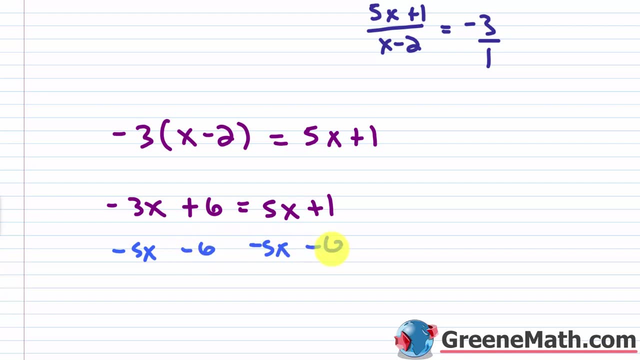 Negative 2 is plus 6. This equals 5x plus 1.. So to solve this, let me subtract 5x away from each side of the equation and subtract 6 away from each side of the equation, So we're going to see that. 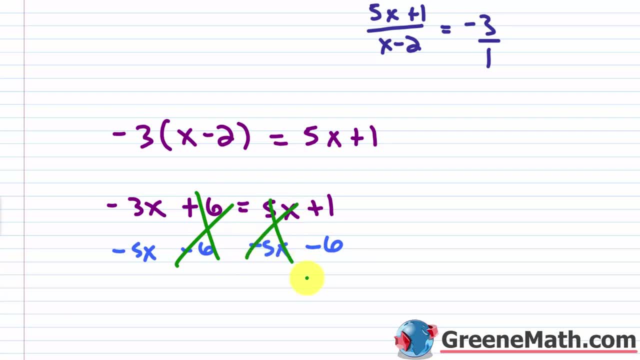 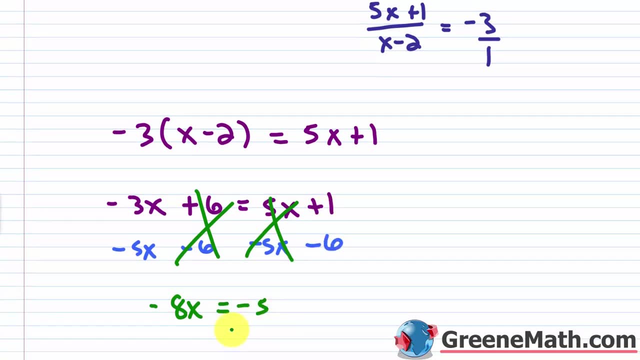 this is going to cancel and this is going to cancel. So negative 3x minus 5x is negative 8x. This equals 1 minus 6 is going to be negative 5.. Let's divide both sides by negative 8.. 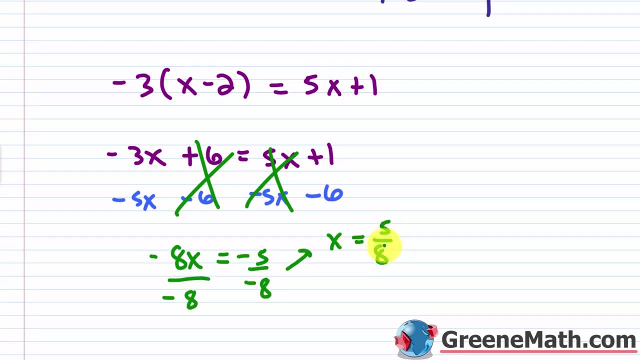 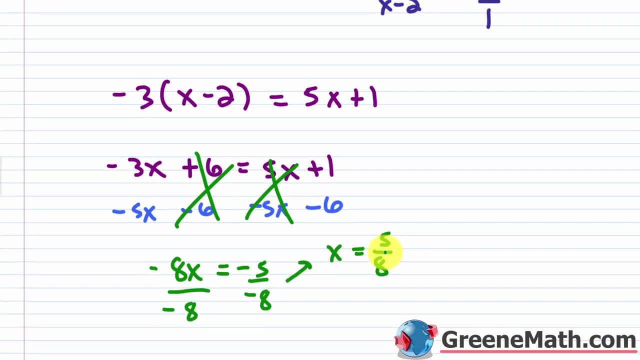 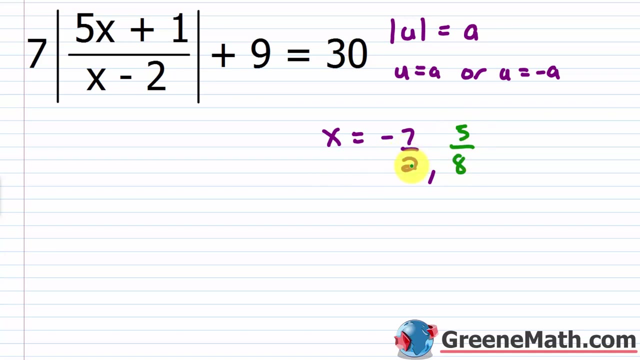 And we're going to end up with: x is equal to 5x. Okay So 5x is a solution and negative 7 halves is a solution. So let's go back up and just list 5x as another solution. Okay, So this guy again. x equals negative 7 halves and x equals 5x Again. 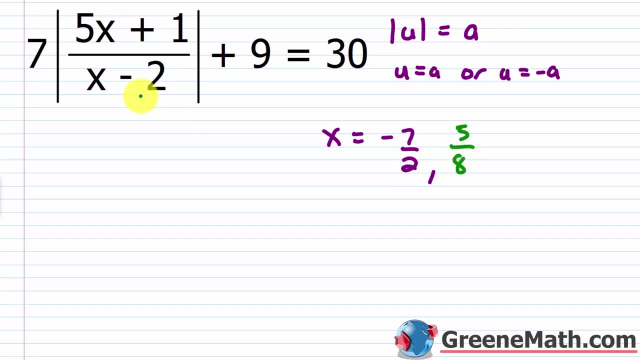 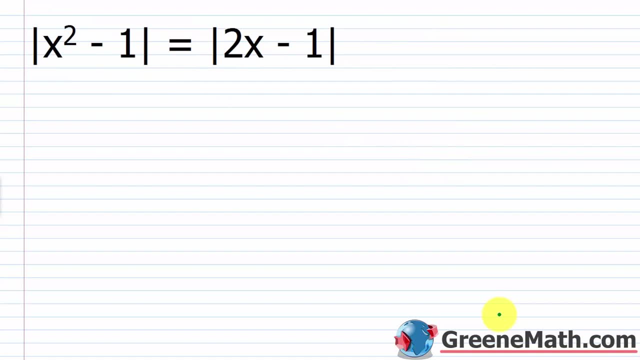 you can check it. I'm not going to in the interest of time, but you'll see that each one of these does give you a true statement when you plug it in for each occurrence of x, All right. So, additionally, we might see some problems where we have two absolute value. 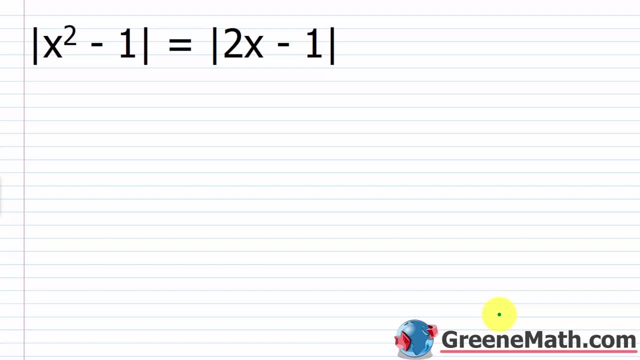 operations. Is that equal to each other? We talked about these earlier when we looked at absolute value equations. in our course, And again for this, basically what you have is you have to think about the fact that two numbers can only have the same absolute value if they're the same number. 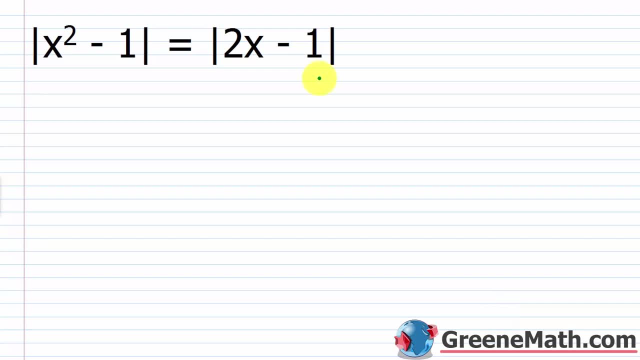 meaning they're equal to each other, or if they're opposites. So for this scenario, you're going to set up another compound equation with: or. For the first case, you're just going to drop the absolute value bars. So for the first case, I'm just going to say that x squared minus. 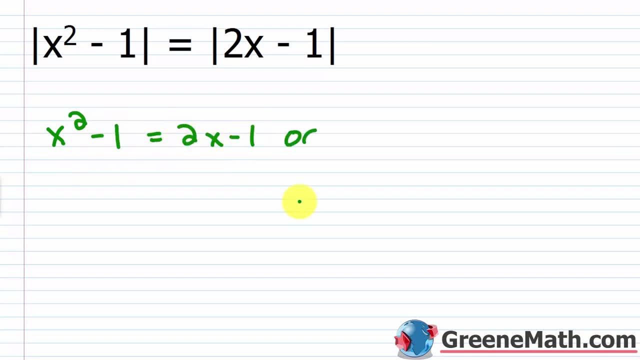 1 is equal to 2x minus 1.. Okay Then, for the second case, I'm going to drop the absolute value bars. So I'm going to say: x squared minus 1 is equal to 2x minus 1.. But what I'm going to do is: 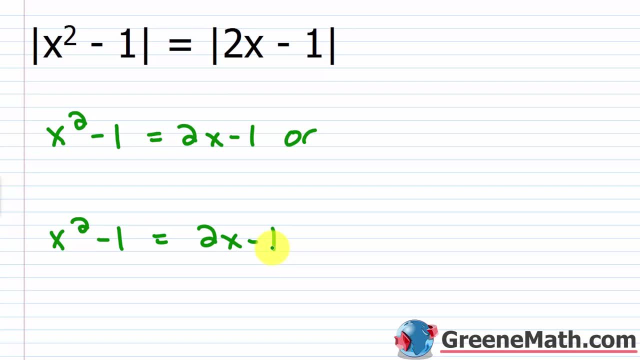 I'm going to make one of the expressions into its opposite. Okay, So the way to do this is just to wrap the expression inside of parentheses and just put a negative in front. So you can do this one or you can do this one, but don't do both. Right, If you did both, then you're basically just going. 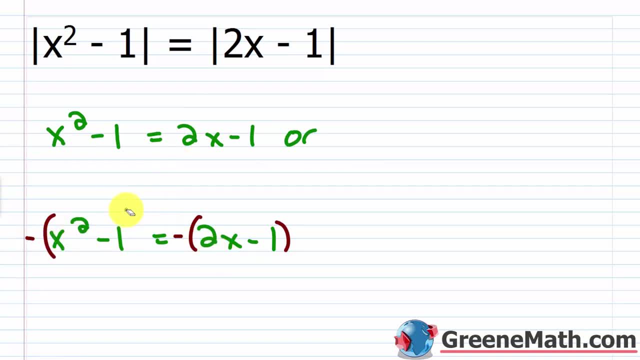 back to this, because I can divide both sides by negative 1.. Okay, So, make sure you just do one of those. Okay, So I'm going to solve this one first and let me put my- or kind of- in the middle here and I'll just drag this down so I have enough. 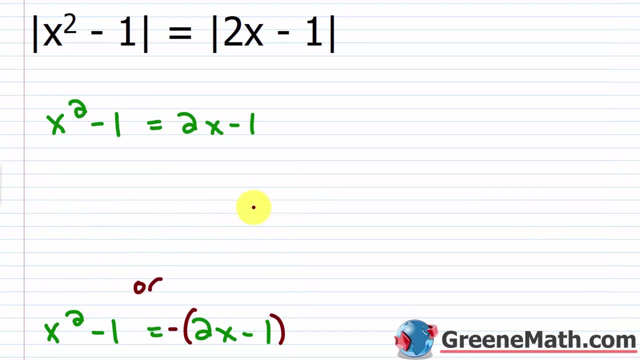 room to work, And so let me start by kind of moving everything to the left side. So let me subtract 2x away and let me add 1 to both sides, So this is going to be 0 over here on the right. 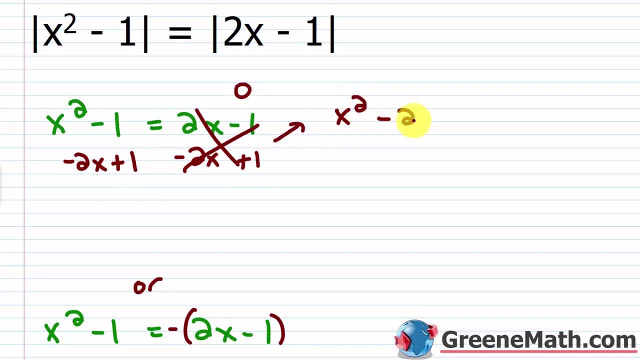 So what we're going to have is that x squared minus 2x, negative 1 plus 1 is 0, so this is just equal to 0 over here. Okay. So x squared minus 2x equals 0.. I can quickly. 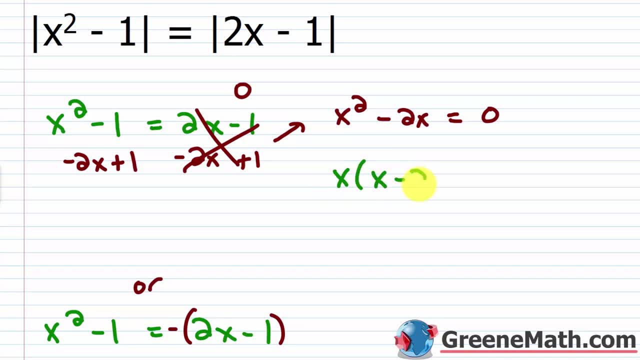 solve that with factoring. Pull an x out, you'd have x minus 2.. So basically, x could be what, It could be 0, or it could be 2.. Right, So x could be equal to 0, and I found that by just. 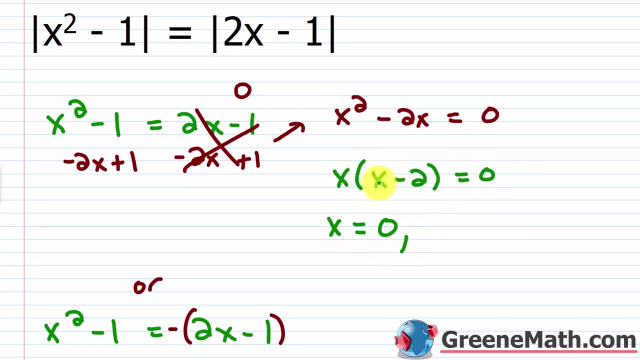 setting x equal to 0, or x could be 2.. I found that by saying x minus 2, this factor here set that equal to 0,, x would be 2.. Okay, So those are the two solutions from there. 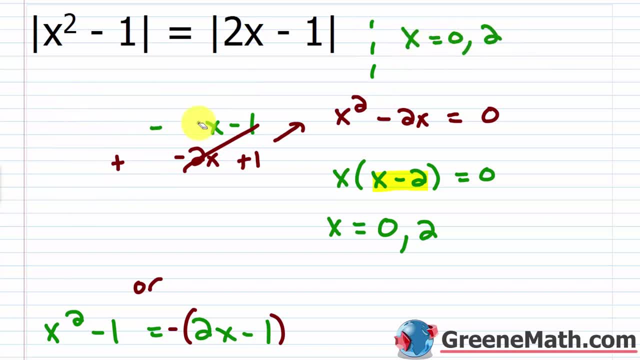 x equals 0, or 2.. Okay, Let's look at the other kind of equation that's involved here. So I'd have: x squared minus 1 is equal to. we've got to make that a little better. You have this negative. 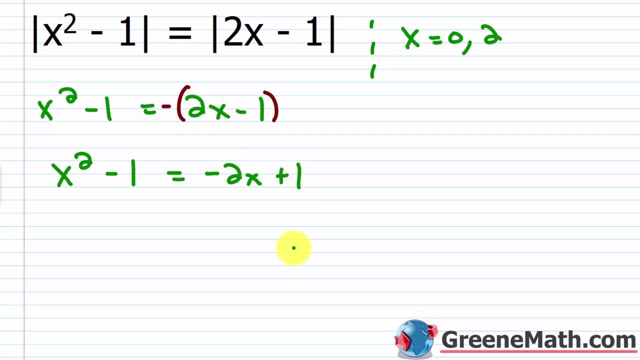 that's got to get distributed. so it would be negative 2x and then plus 1.. Okay, So again, move everything over, So you're going to have x squared. add 2x to both sides of the equation. 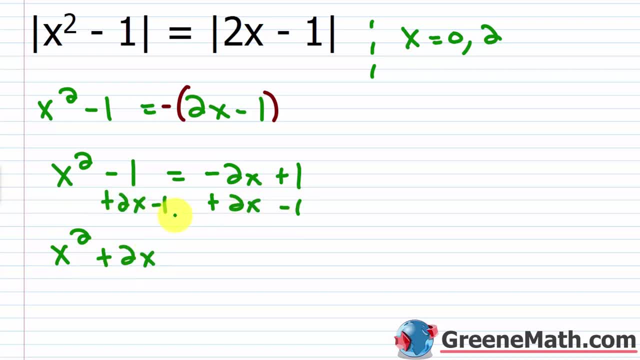 so plus 2x, subtract 1 away from each side of the equation. So over here again. this is 0, and then negative 2x, and then plus 2x, subtract 1 away from each side of the equation. 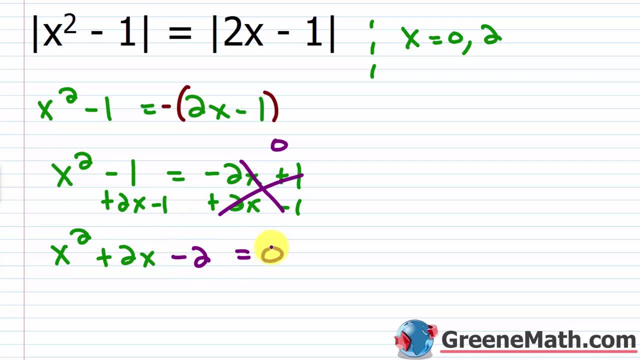 So negative 1 minus 1 is negative 2. This equals 0. So can we solve this with factoring? No, this guy isn't going to be factorable, So let's go ahead and set up our quadratic formula. So let me erase this. so we have a little room to work, And we already know that this has an. 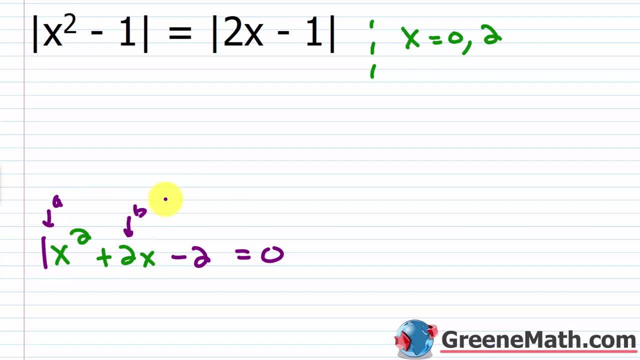 implied coefficient of 1.. So that's my a, this is my b and this negative 2. here is the c. So x equals what It's negative b, b is 2, so negative 2, plus or minus the square root of. 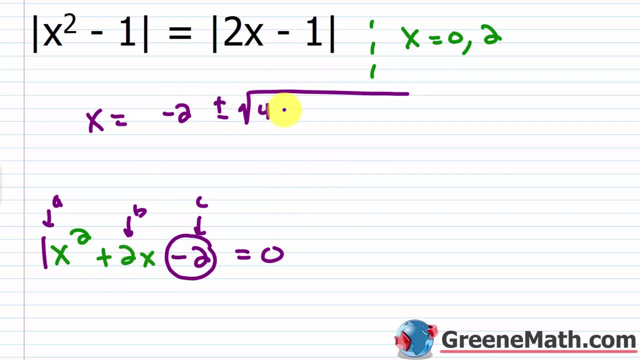 b. squared Again, b is 2, 2 squared is 4, minus 4 times a, a is 1, times c, c is negative 2.. So negative 4 times negative, 2 is positive 8.. 8 times 1 is still 8.. So you would have 4 plus 8, which is 12.. Okay. 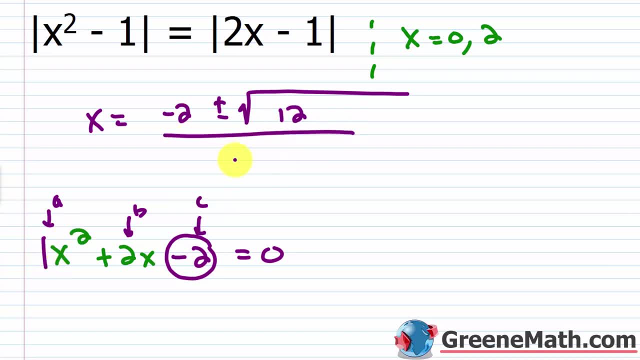 so this would be 12 here. This is over 2 times a. a is 1, so just 2.. Okay, So square root of 12, I know that 12 is 4 times 3.. So let's write this as 4 times 3.. We know the square root of 4 is 2,. 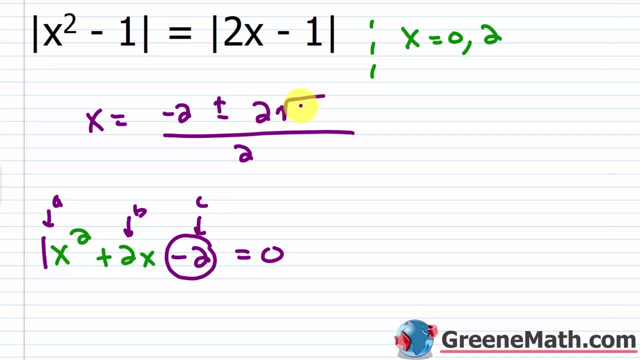 so I can pull this out and say: this is 2 times square root of 3.. of 3. okay, so let me erase this. now. we know we can simplify this a little bit, so to make this simpler, let me factor out a 2 from the numerator. that would give me a negative 1 plus or minus. 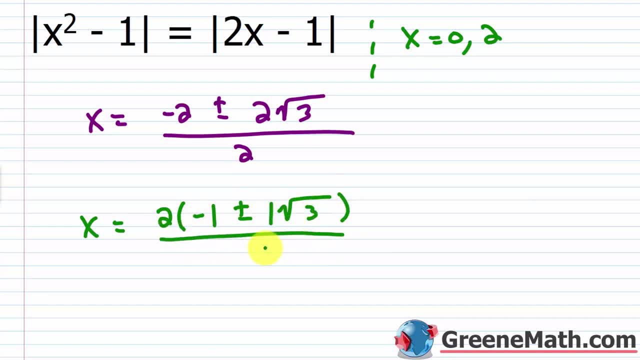 a 1 times square root of 3. this is over 2 and we can see that this would cancel with this, and so what i'm left with i can just erase this. i don't need a fraction anymore. i basically have negative 1 plus or minus the square root of 3. okay, so my other two solutions would be negative 1. 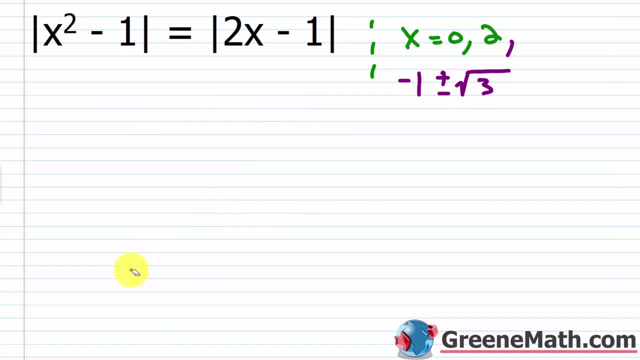 plus or minus the square root of 3. so those are my four solutions: x could be 0, x could be 2, x could be negative: 1 plus square root of 3. or x could be negative: 1 minus the square root of 3. all right, 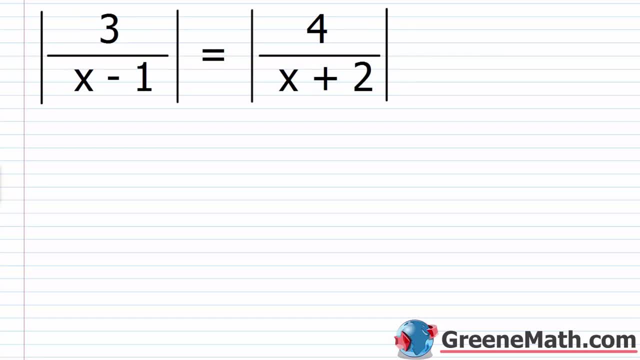 let's take a look at one more example of these, and this is with rational expressions. so the absolute value of 3 over x minus 1 is equal to the absolute value of 4 over x plus 2. so for this, again the first scenario, just drop the absolute value bars. they could just be equal. so 3 over x. 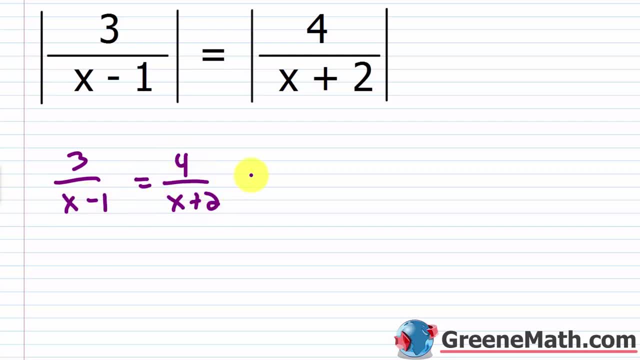 minus 1 is equal to 4 over x plus 2. then, or for the second scenario, drop the absolute value bars, so 3 over x minus 1 is equal to 4 over x plus 2, and then make one of the expressions into its. 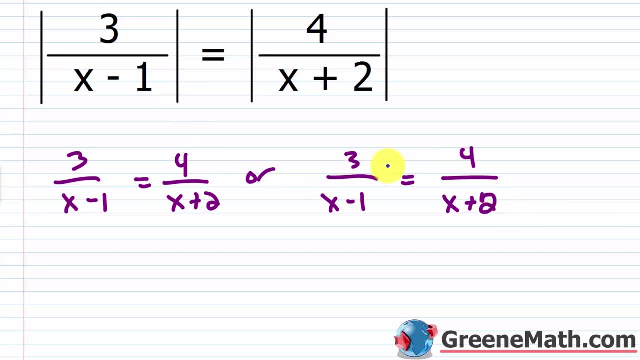 opposite. so for this guy all i need to do is make one of the numerators negative, so i can just say this is negative. or i can say this is negative, but just don't do both of them, okay. so let me just solve this one first. i'm going to cross, multiply so you'd have 4 times. 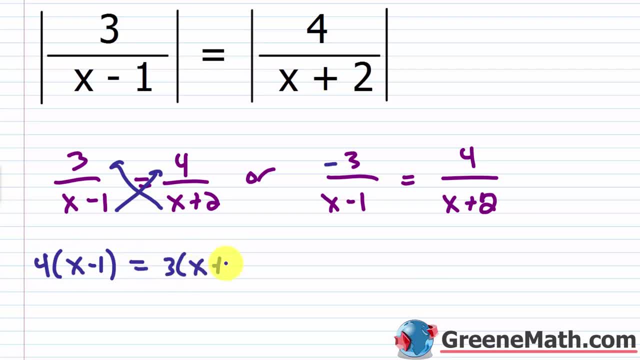 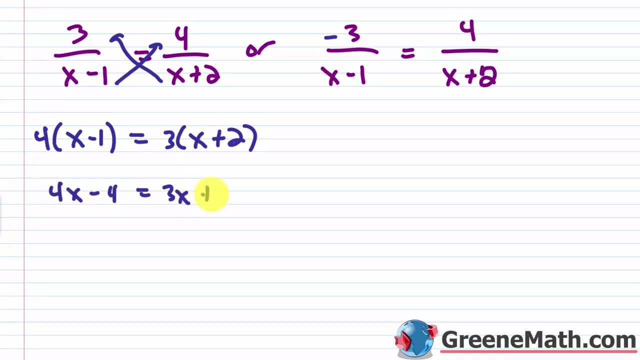 the quantity x minus 1 is equal to 3 times the quantity x plus 2.. let's kind of scroll down and solve this, so you'd have 4x minus 4 is equal to 3x plus 6.. so now let me subtract 3x away from each. 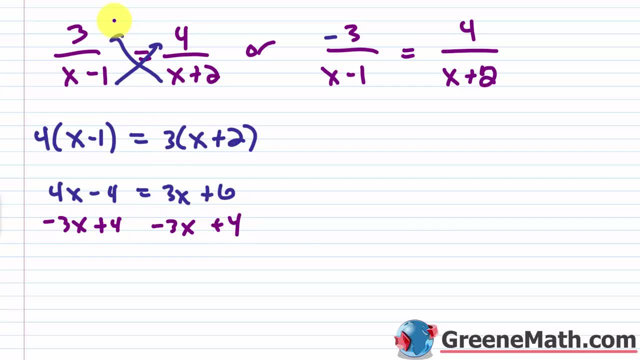 side of the equation. let me add 4 to both sides of the equation and this guy is going to cancel. this guy is going to cancel. 4x minus 3x is x, 6 plus 4 is 10.. so one solution is that x is equal to 10. 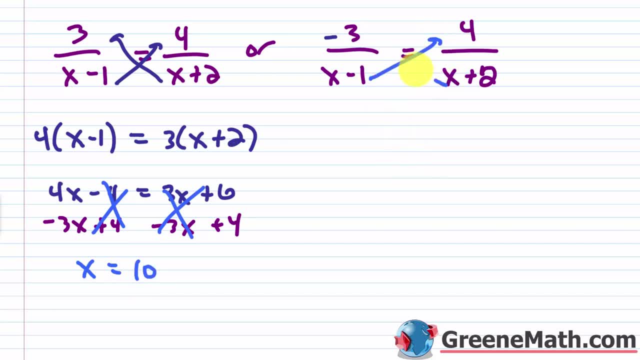 then over here let me cross multiply so you'd have what you'd have: that negative 3 times the quantity x plus 2 is equal to 4 times the quantity x minus 1. negative 3 times x is negative 3x. negative 3 times 2 is minus 6. this equals 4 times x, which is 4x, and then 4 times negative 1 is. 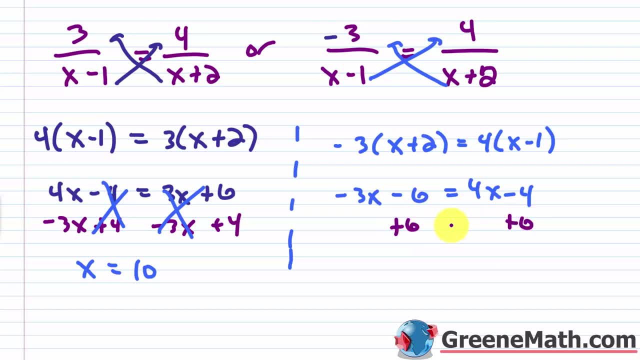 negative 4. okay, so let me add 6 to both sides of the equation. let me subtract 4x away from both sides of the equation, so this is going to cancel, and this is going to cancel. you have negative 3x minus 4x, which is negative 7x. this equals negative 4 plus 6, which is going to be 2. we can finish this. 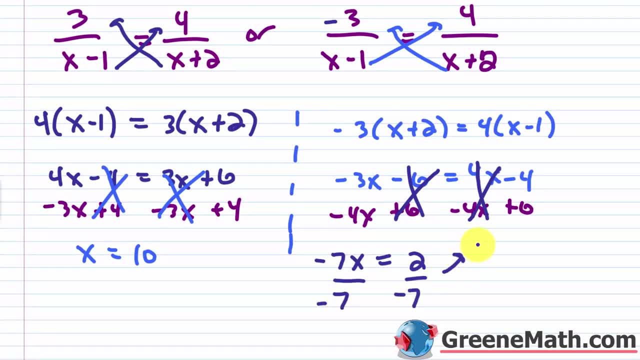 up by just dividing both sides by negative 7, we're going to find that x is equal to negative 2 7s. okay, so here x could be 10 or x could be negative 2 7s. so let me erase everything. so i'll say that x could be equal to 10. 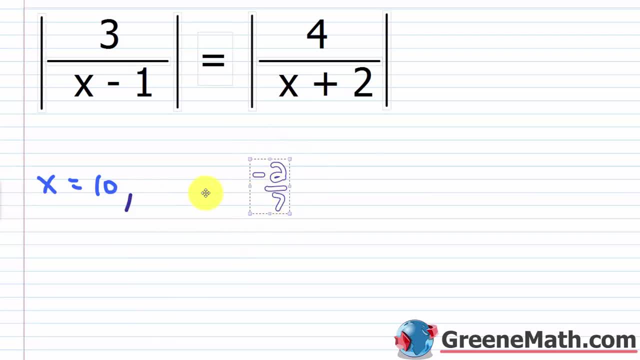 or it could be negative 2 7ths. Okay, that's going to be our answer And again, you can check this. if you want, Plug in a 10 for each occurrence of x, you'll see you get the same value on the left. 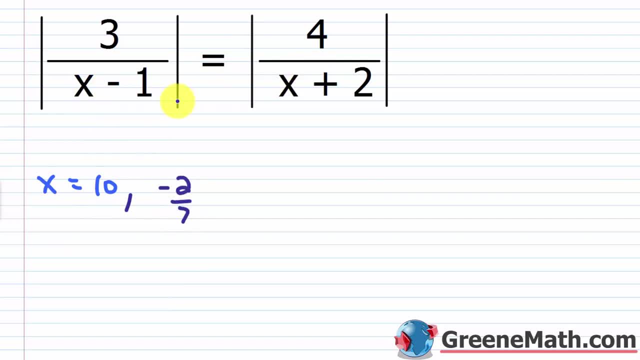 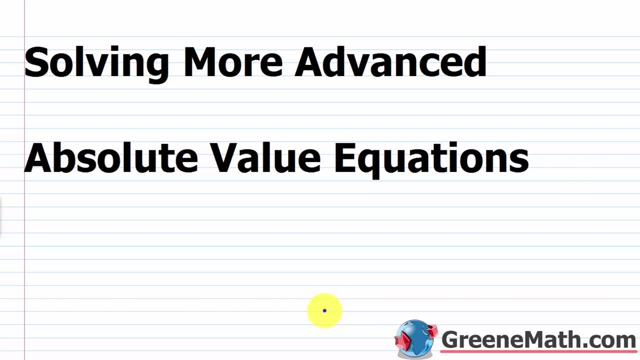 and the right. Plug in a negative 2 7ths for each occurrence of x. you'll again see that you get the same value on the left and the right. So this guy is correct In this lesson we're going to talk. 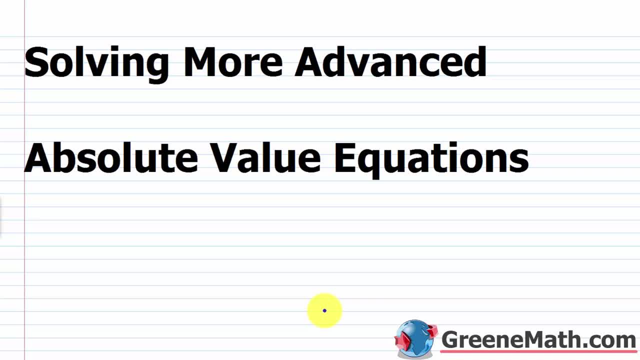 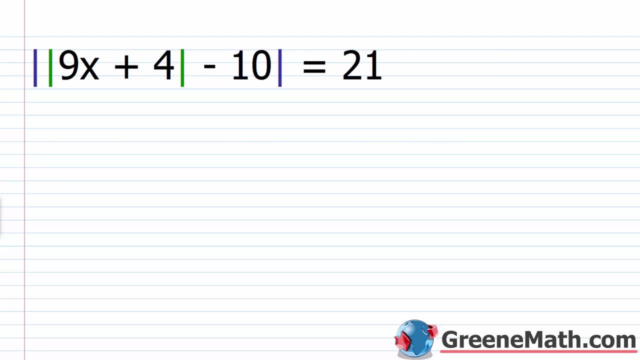 about solving more advanced absolute value equations. So up to this point we've worked with some absolute value equations that can be solved pretty easily. In pretty much all the cases we just needed to isolate the absolute value operation And then we could set up a. 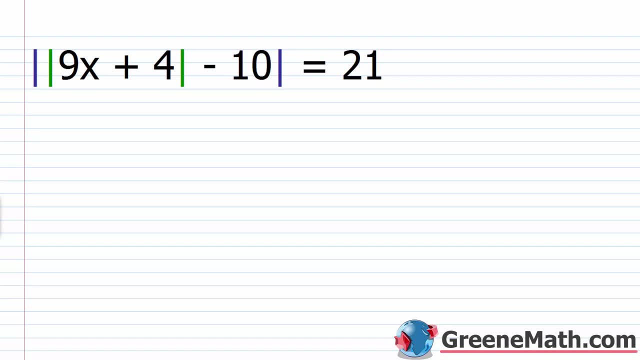 compound equation with or. Now I know we looked at some more challenging scenarios in the last lesson, where we involve some quadratic equations and some rational equations, But now we're going to go even further and look at some absolute value equations that end up either being challenging to 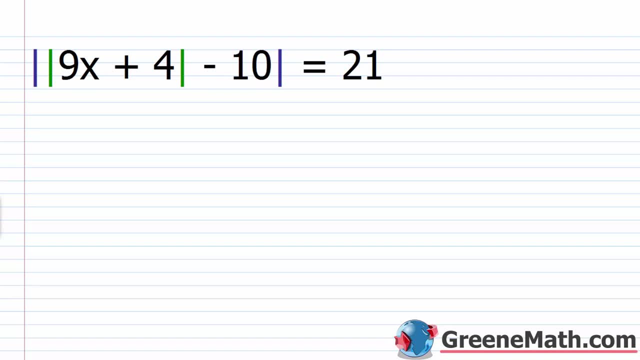 solve, or being really tedious to solve. Okay, a lot, a lot of extra work. So let's get started. So let's start out by talking about how to solve an absolute value equation where one absolute value operation is nested inside of another. So this is a common problem, you will see. So suppose, 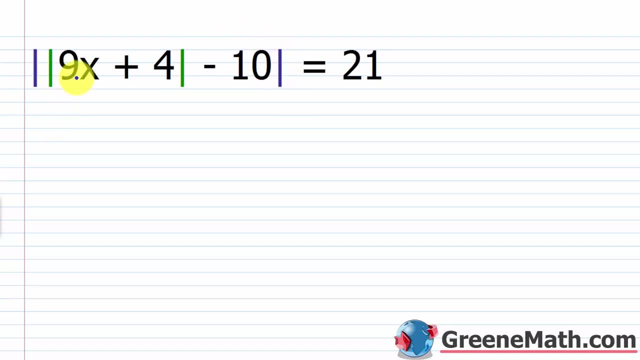 we had something like the absolute value of the absolute value of 9x plus 4 minus 10.. And this is equal to 21.. Okay, so notice that you have an outer absolute value operation And then- let me highlight this in a different color- you have an inner absolute value operation. Okay, so the 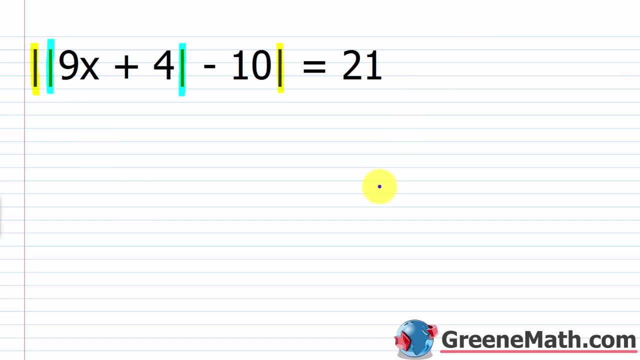 way you kind of attack this problem is you first consider the larger absolute value expression, okay, the one that surrounds the entire left side of the equation, the one that I highlighted in yellow. So what we're going to do is we're going to set up an or with this guy, So we're going to 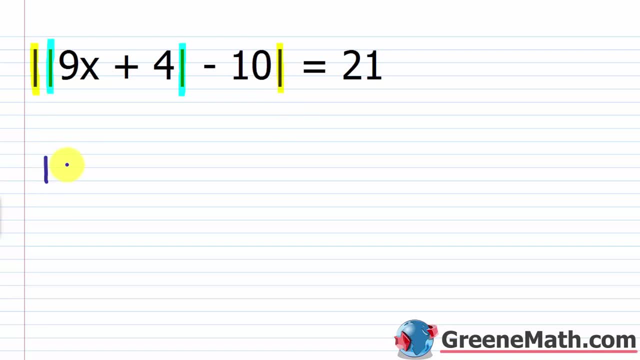 drop those absolute value bars, So that would give me the absolute value of 9x plus 4, and then minus 10.. And then I'm going to say: this is equal to 21,. then I'm going to do my or. So now I'm going to. 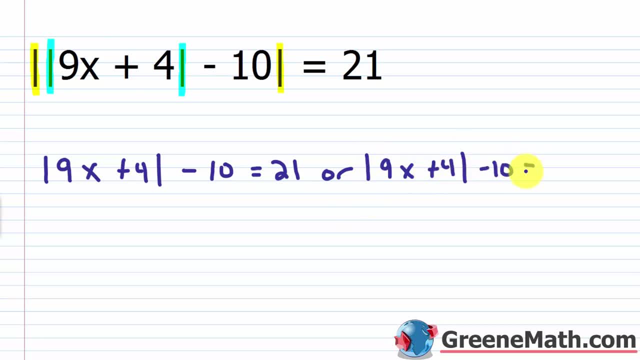 get the absolute value of 9x plus 4.. Okay, again minus 10.. Now it's going to be equal to negative 21.. Okay, so it's the same thought process as what we used in the previous kind of lessons. 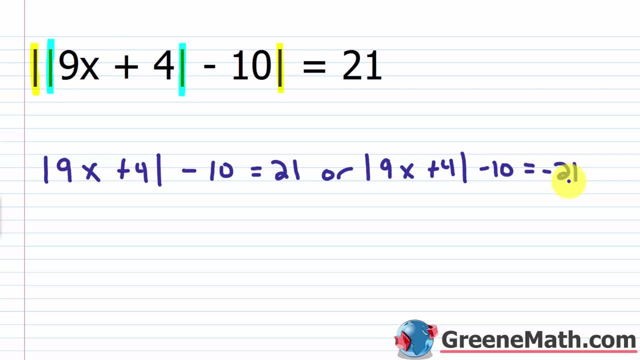 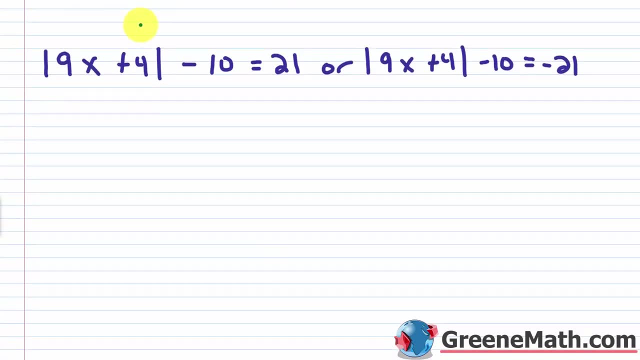 But we're going to have to do this basically twice. Okay, so just extra work, Okay. so for this guy on the left, let me kind of move down just a little bit. We know how to solve this. This is basically what we've looked at in the past, So let me isolate the absolute value operation. So I'm 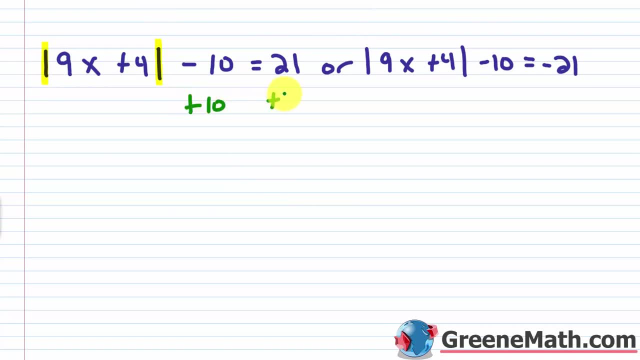 going to isolate this guy now. So all I'm going to do is I'm going to add 10 to both sides of the equation. I'm going to get that the absolute value of 9x plus 4 is equal to 21 plus 10 is 31.. 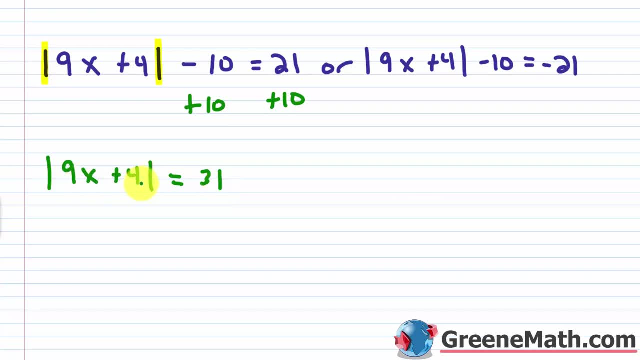 Okay, so now all I've got to do is set what's inside of the absolute value operation equal to 31,. then say: or what's inside the absolute value operation is equal to the negative of 31.. Okay, so we get: 9x plus 4 is equal to 31,, or 9x plus 4 is equal to negative 31.. And you can see how. 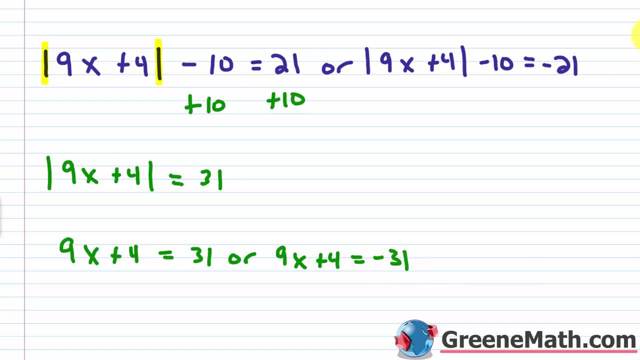 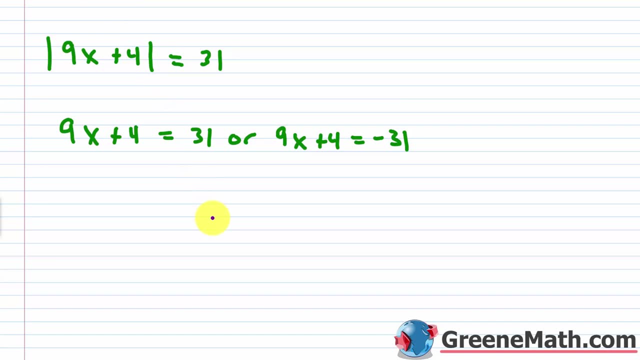 tedious this becomes. This is just one of those ones where it's not hard once you kind of understand the steps. it just takes a long time, a lot of scratch paper And sometimes that can involve you making some mistakes if you're not really careful. So for this guy on the left I'm going to subtract 4 away. 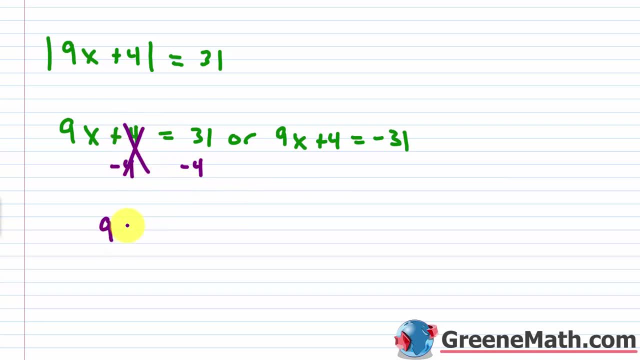 from each side of the equation. this is going to cancel. I'm going to have that 9x is equal to 31 minus 4 is 27.. Okay, so if I divide both sides of the equation by 9, I get one solution And 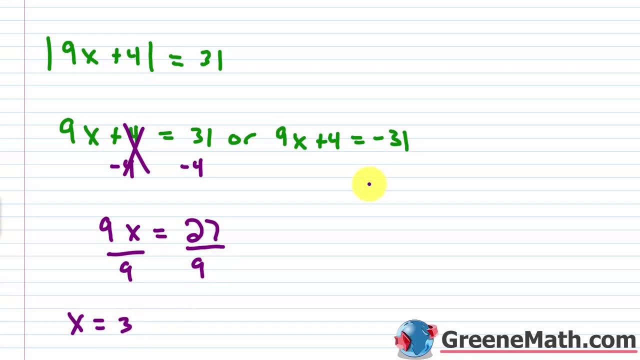 that's that x is equal to 3.. Okay, so that's one solution Over here. if I subtract 4 away from each side of the equation, this cancels, I'm going to get that 9x is equal to negative 31 minus 4. 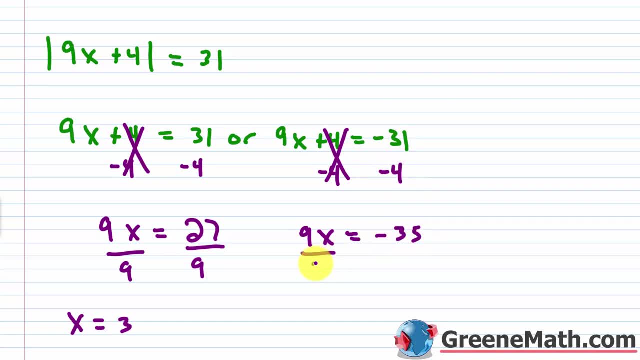 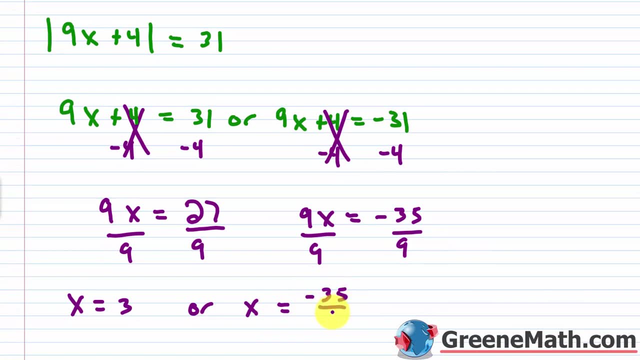 is negative 35.. Again, I'm going to finish this up by dividing both sides by 9.. And I'm going to find that x could also be equal to negative 35 nights. Okay, so those are two solutions that we have, But we've got to go back up and deal with the other scenario, So let me just kind of copy. 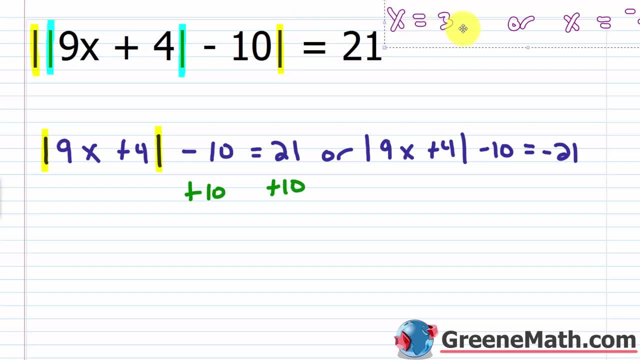 this real fast And I'm just going to erase all this work. Okay, and I'm just going to paste that in: right here, Right there. Okay, so that's for this guy, right here. So I'm just going to erase all of this. 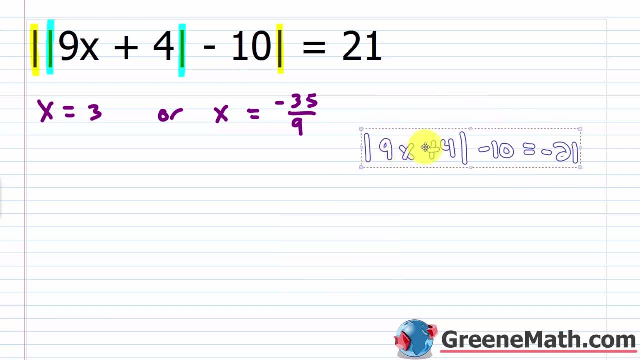 we don't need that anymore, And let me kind of drag this over here And let's work on this guy now. So what I'm going to do is I'm going to add 10 to both sides of the equation to kind of get. 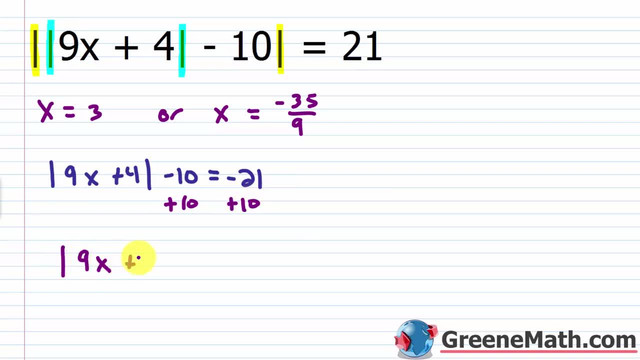 things started, I'm going to have the absolute value of 9x plus 4 is equal to negative. 21 plus 10 is going to give me negative 11.. Now you'll notice that there's a problem here. We know that. 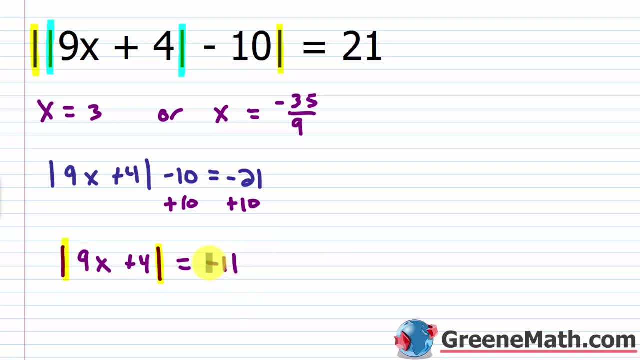 if we have the absolute value operation isolated one side and we have a negative value on the other side, there's no solution. Okay Again, if I take the absolute value of a negative number, it becomes positive. If I take the absolute value, 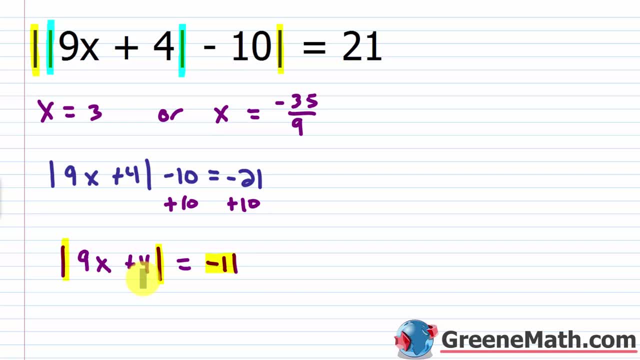 of zero, I get zero. If I take the absolute value of a positive, it stays positive. So there's nothing I can plug in for x here. multiply by nine and then take that and add to four and take the absolute value and get a negative 11.. Okay, it's not going to happen Because again the 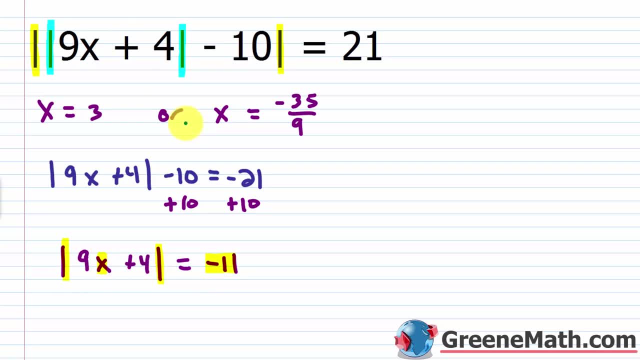 absolute value operation is going to give you a non negative result, And so this guy could never get a negative 11.. So for this part, we would say there's no solution. Okay, there's no solution, Okay. But for the equation as a whole, we found that one part had a solution. So this is going. 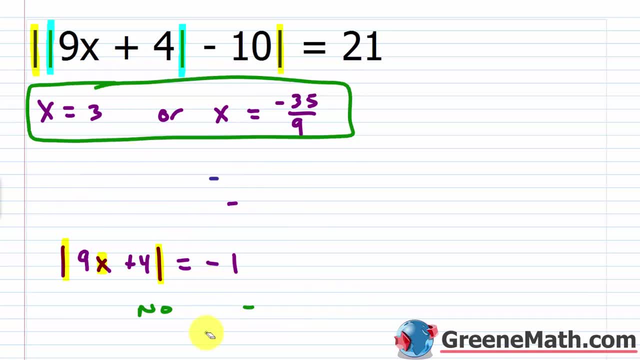 to be the solution for the whole thing. This guy, you can just throw it away, right. That part just leads to a no solution type of answer. Okay, So for this guy as a whole, the solution is going to be x could be three or x could be negative, 35, ninths. All right, let's take a look at another. 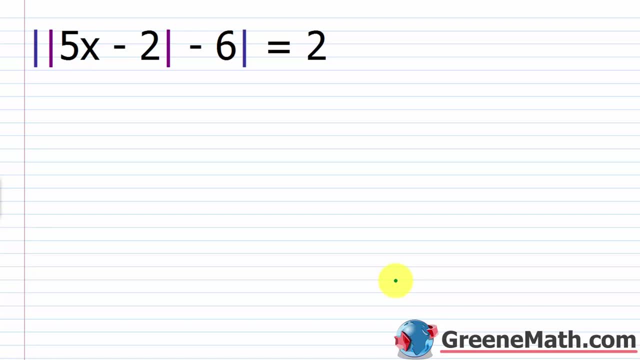 one of these, And then we'll move on and talk about another type of problem That you'll probably encounter. So we have the absolute value of, and then inside of that, you have the absolute value of five x minus two, and then minus six. this whole thing is equal to. 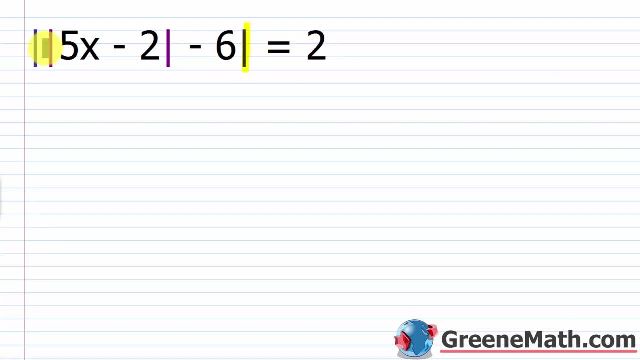 two. So again, I'm going to start with the outside absolute value operation And what I'm going to do is I'm going to set up two scenarios. I'm going to say that the absolute value of five x minus two minus six is equal to two. then, or I'm going to also say that the absolute value 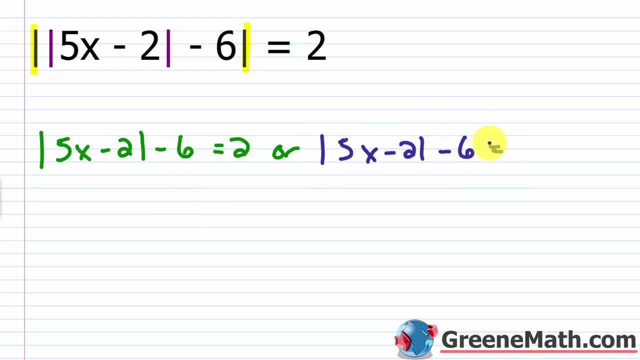 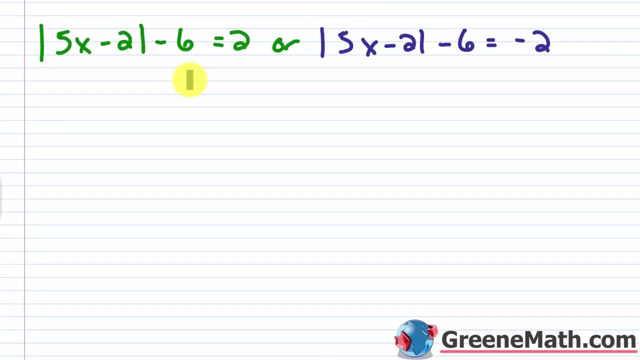 of five x minus two minus six is equal to what it's equal to the negative of two. Okay, so just split it up into two cases, And then we're just going to start working. So over here. I know I want to isolate the absolute value operation, So I'm going to do that by adding six to both sides. 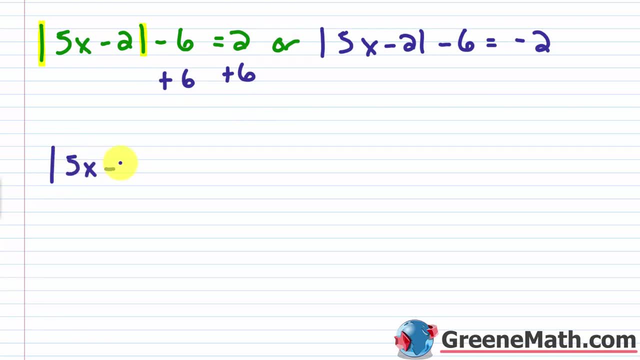 of the equation. So I'm going to get that the absolute value of five x minus two is equal to two plus six is going to be eight. Okay, so this splits up into two more cases, right, So we can say that five x minus two. 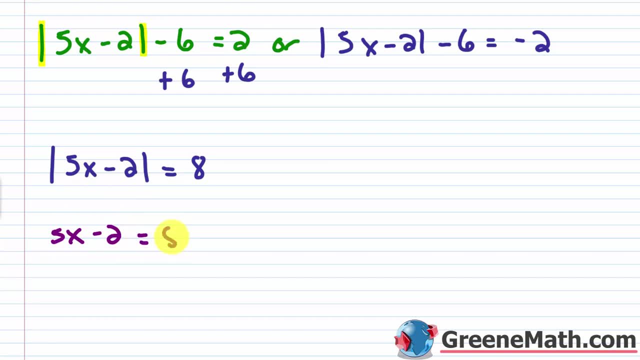 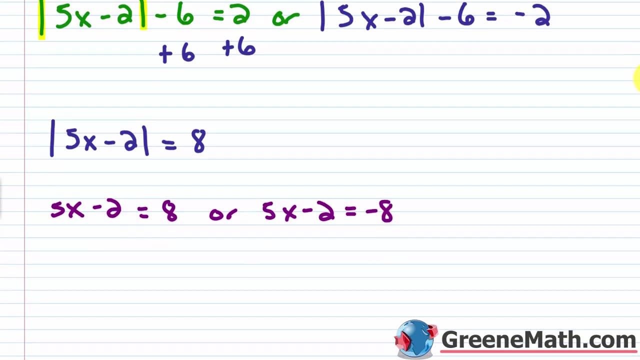 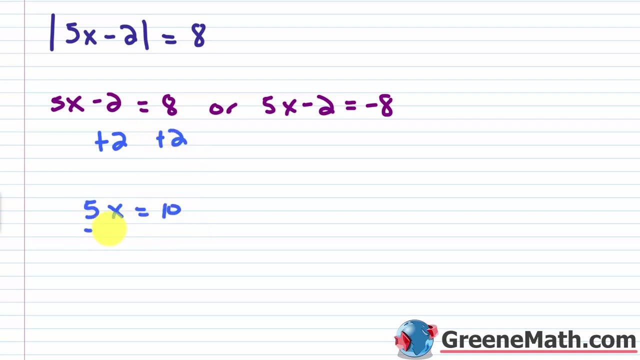 this expression, inside the absolute value bars, is equal to eight, or five x minus two is equal to negative eight. Okay, so let's solve those real quick. we'll come back up. So let me go ahead and add two to both sides of the equation. we're going to have that five x is equal to 10.. Let's divide. 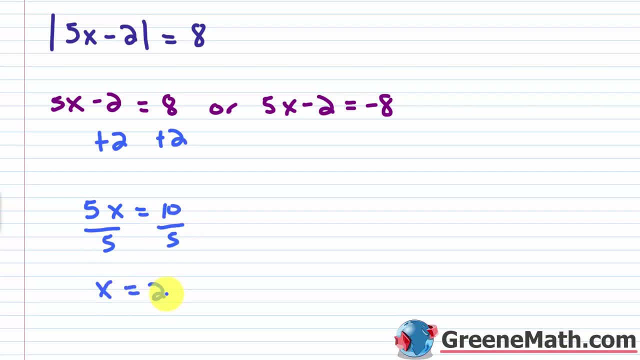 both sides of the equation by five, we're going to get that x is equal to two. Okay, so that's one solution Over here. let me add two to both sides of the equation And I'm going to get that five x. 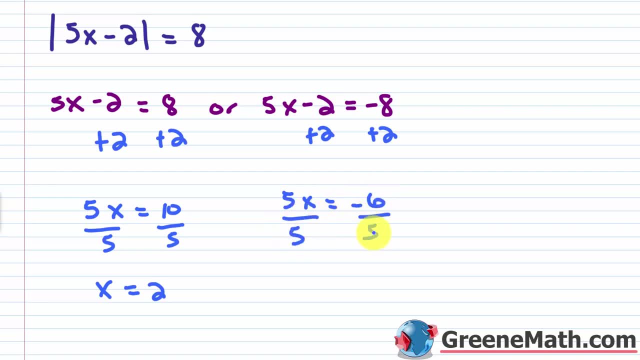 is equal to negative six. both sides by five and i'm gonna get that x is equal to negative six fifths. okay, so we have two solutions. we've got x is two or x is negative six fifths. so let's work on the other side and see. 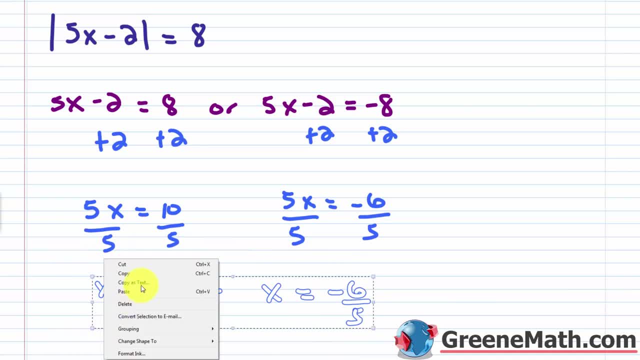 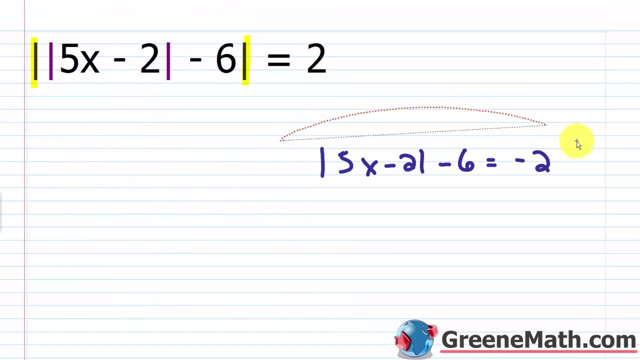 about getting some more solutions. okay, so let me just copy these and i'm going to erase all this work. we don't need it anymore. all right, so i'm just going to erase this part right here and let me just drag this other one over here, because we need to work with this, and i'm just going to paste. 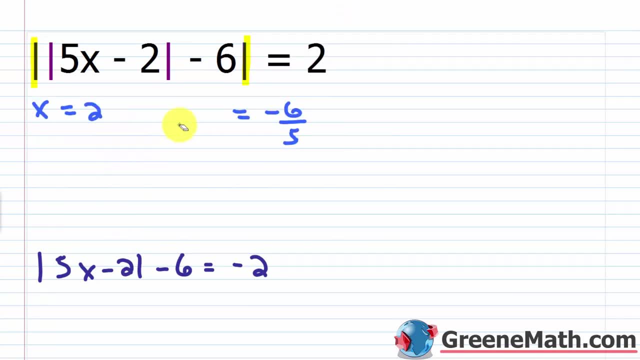 these solutions in. this is what we have so far and i'm just going to erase this and put a little comma. so x equals two and i'll put comma negative six fifths. okay, let's take a look at this kind of second case. so again, we want to isolate the absolute value operation and what we're going. 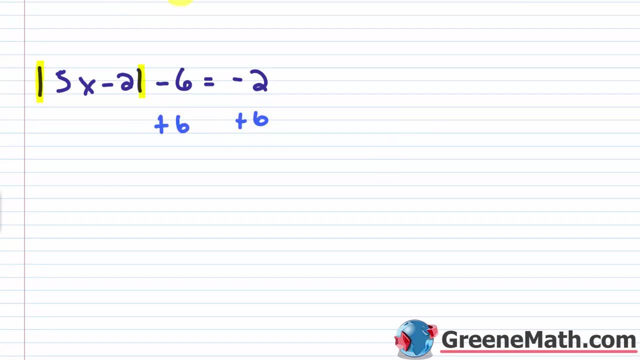 to do is just add six to both sides of the equation, and so this guy is going to cancel. we would have that the absolute value of 5x minus 2 is equal to y negative, 2 plus 6 is positive 4.. so in the other example we saw that in our kind of second case we had something with no solution. 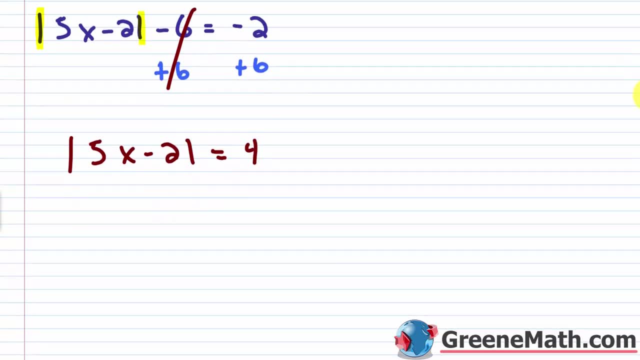 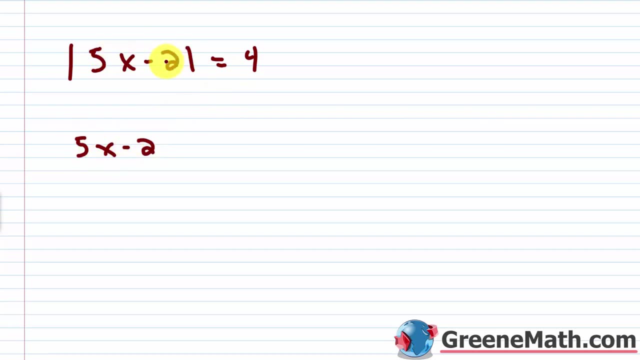 in this example we don't have that, so we can keep going. so what we're going to do is again set this up into two more cases. so 5x minus 2, the expression inside the absolute value bars could be equal to 4, or 5x minus 2 could be equal to negative 4.. okay, so we're just going to solve. 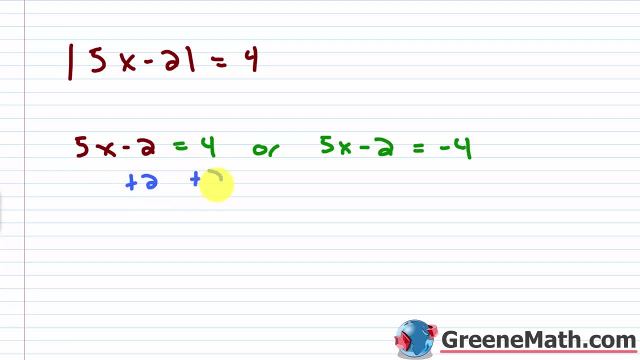 those two scenarios. so let me add two to both sides of the equation here. i'm going to get that 5x is equal to 6. divide both sides by 5, we're going to get x is equal to six fifths. okay, so that's the solution over here. i'm going to add two to both sides of the equation and i'm going to get. 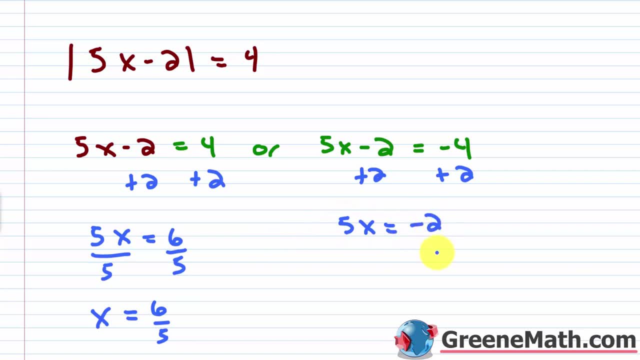 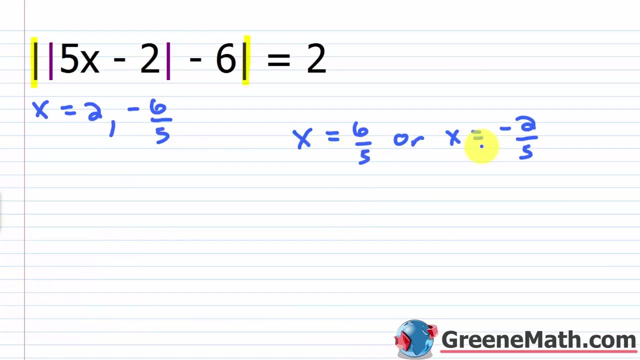 that 5x is equal to negative two. we're going to divide both sides by five, so i'll put: or here x could also be equal to negative two bits. okay, so we're gonna have a total of four solutions. let me kind of copy this and i'll erase everything. okay, so we have six fifths and negative two, and 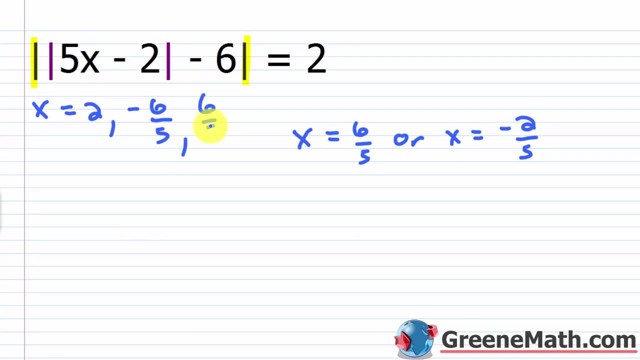 a two fifths. so let me put comma six fifths and comma negative two fifths. okay, so those are our four solutions. i'm not going to check them in the interest of time, but you can plug each one in for x and you see that you get a true statement in every case, right? so x is two negative six fifths. 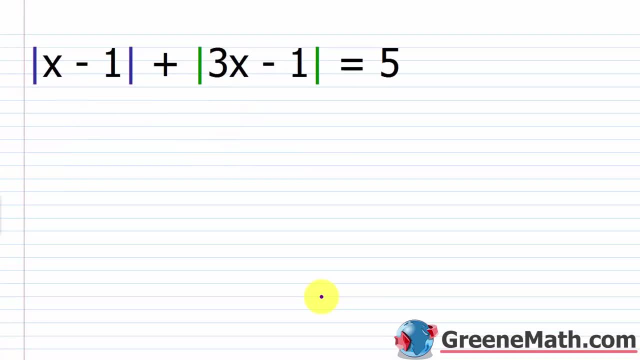 six fifths, or negative two fifths, all right, so now let's move on and look at something that's even more tedious. so we've previously seen examples where two absolute value operations were equal to each other. okay, so for that scenario it's very easy to solve. but what happens when we have 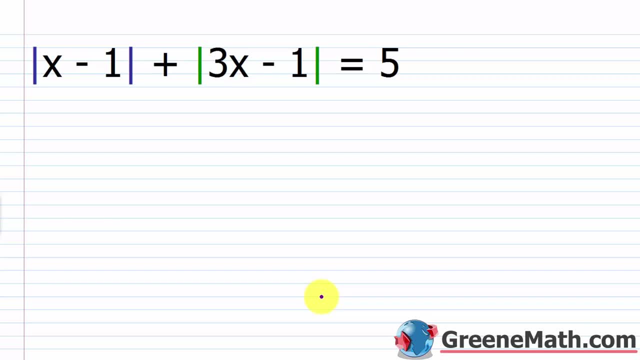 an equation with two absolute value operations and then kind of an extra or a loose number, okay, so this is a very common scenario that you'll come across. so something like the absolute value of x minus one, then plus the absolute value of three x minus one, and this is equal to five. okay, 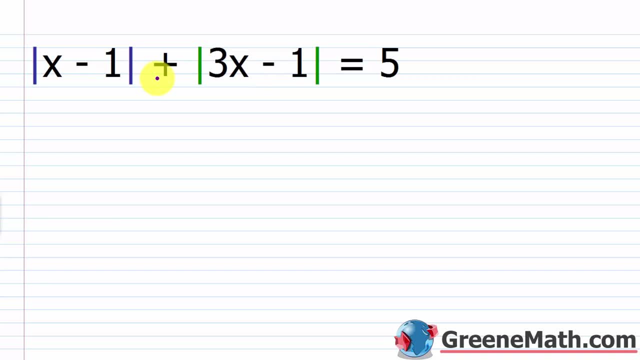 so in this case we can't directly set the two absolute value operations equal to each other. okay, so we can't use that method, so we have to kind of turn to a more advanced approach, or, you could say, a more tedious approach. now there's other ways to do this than what i'm 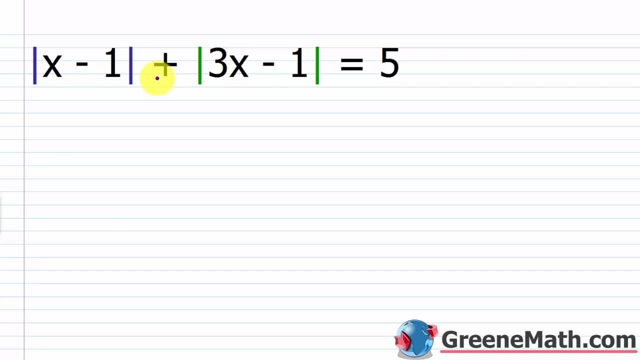 going to show you, and i'll explain that when i get done with this method. so what we're going to do is we're going to think about the expressions that are inside of the absolute value operations. so you've got two of those, okay. so what we want to do is think about where these expressions 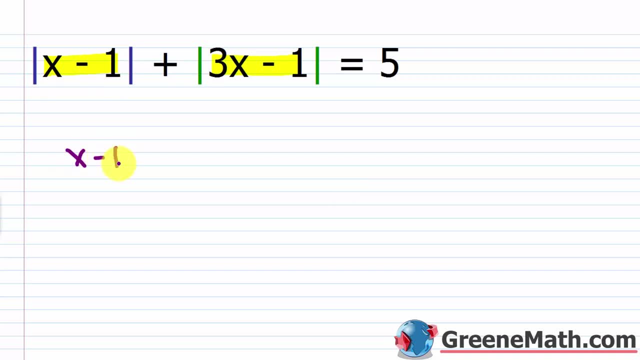 are zero, okay. so where is the expression x minus one equal to zero, and where is the expression 3x minus one equal to zero? okay, because those represent basically our turning points. it's where the sign is going to change from positive to negative or from negative. 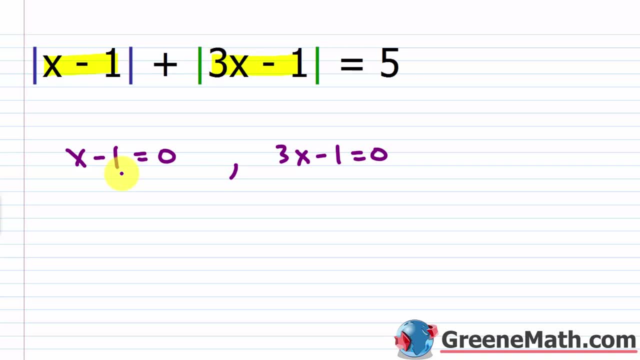 to positive. okay, this can only happen at a value of zero. so for this one, i'm just going to solve, i'm going to add one to both sides of the equation. so i'm going to have that x is equal to one. okay, for this one, i'm going to add one to both sides of the equation. i'm going to get that 3x is equal. 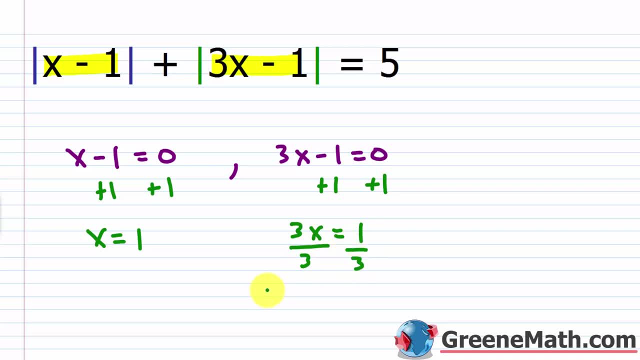 to one. i'm going to divide both sides of the equation by three and i'm going to say that x is equal to one third. so this value here of one is what makes this expression here to zero right. if i plugged in a one there, one minus one would be zero. okay, this value of one. 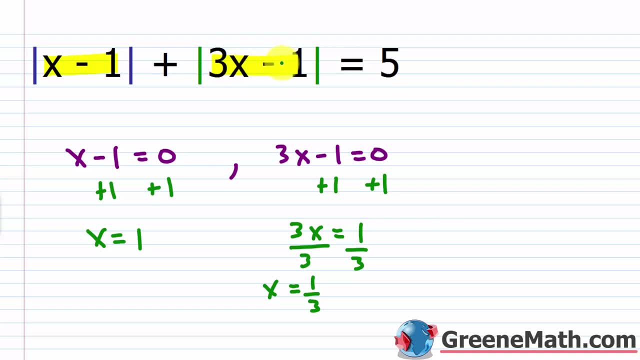 third is what makes this expression equal to zero three times. the third is one. one minus one is zero. so we can see that. so we're going to use these two values to kind of split the number line up into intervals. so let me go down here real quick to a little table. so this is a good way to kind of 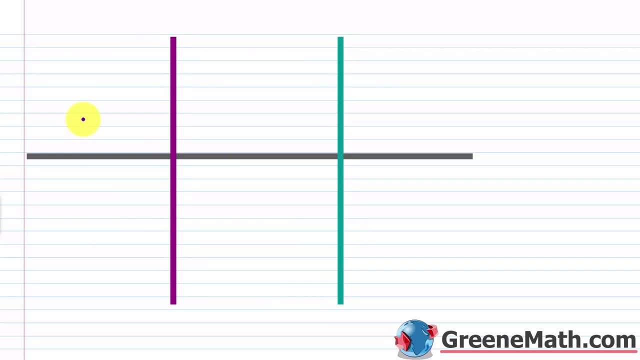 organize the information. so one interval would be anything from negative infinity up to, but not including, one third. so this interval here. so we have negative infinity and we have one third, and again neither of those is going to be included here. then the next one. if we go back again, the values were one third and one. so i want to think about between one third and one. 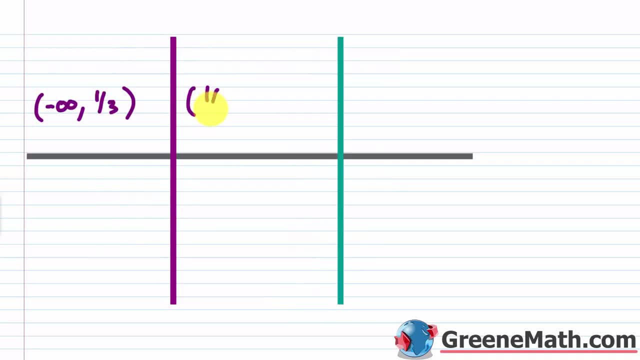 what's going to happen? so what happens between one third and one? okay, neither of those is going to be included, and then my last interval would be anything greater than one, so i'll put a one next to a parenthesis and then comma infinity. okay, so that interval there. so what we're doing here in. 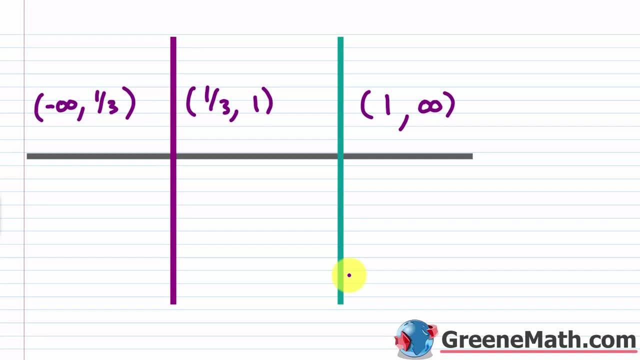 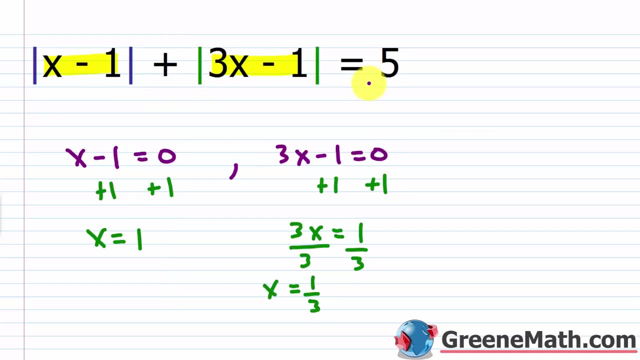 this interval is. we're thinking about the value of the expression in each interval. okay, so, if it's negative, we're going to replace the expression with the opposite, and if it's positive, we just replace it with the expression itself. okay, so, if i go back up again, this guy right here, i'm just 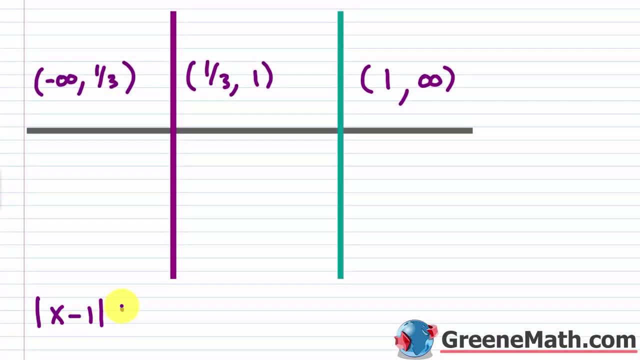 going to copy this down here. so we have the absolute value of x minus 1. then, plus the absolute value of 3x minus 1, this is equal to 5.. so when we think about this interval, anything that's negative- we know that both of these guys would be negative. okay, because this guy right here is zero. 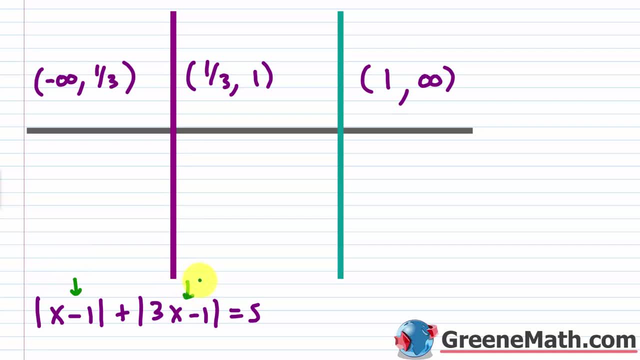 when x is equal to 1, and this guy right here is 0 when x is one third. so if it's less than one third, both of those guys would be negative, and so you would take each expression, okay, each expression, and you would make it into its negative or its opposite, okay. so, in other words, this guy would be 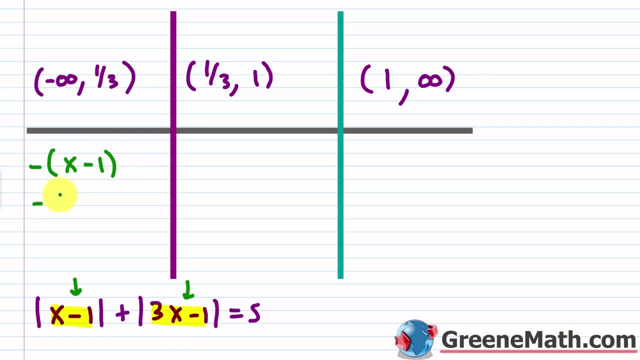 negative of x minus one that quantity. this guy would be the negative of: you have 3x minus 1 that quantity. okay, so that's the expressions. we're going to be dropping the absolute value bars in each case and we're going to be replacing those. 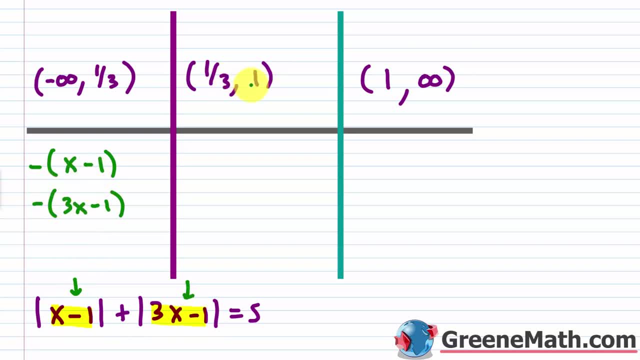 with these kind of expressions we're setting up here now, between these two numbers, one third and one. remember, this guy is made zero by one third, so anything larger than one third means that this guy is going to be positive. so i can replace this one with the just expression itself: so 3x minus one. 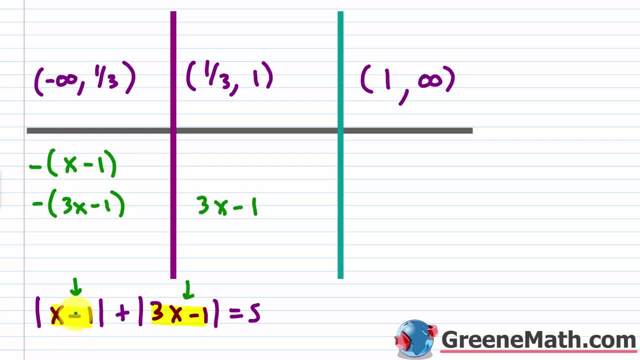 then for this guy right here again, one is what makes it zero. so anything that's less than 1 is going to result in this being negative. so this is negative of the quantity x minus 1.. then in this scenario here, where we're larger than 1, both of these guys. 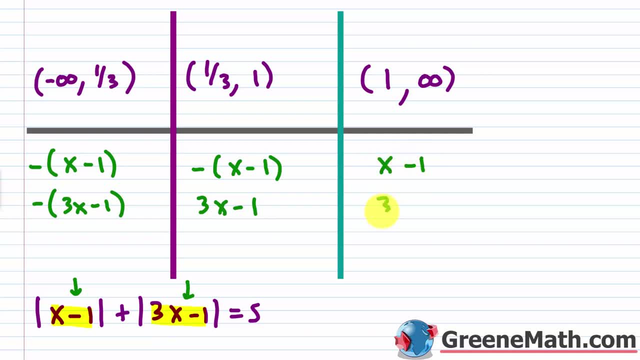 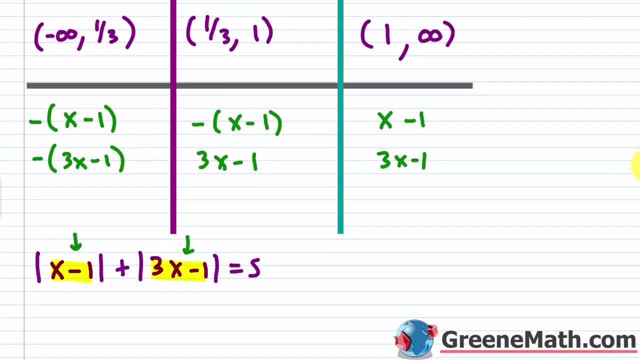 are going to be positive. so i can say this is x minus 1 and this is 3x minus 1.. okay, so what i'm doing here is i'm going to go through- let me kind of scroll down a little bit- and i'm going to. 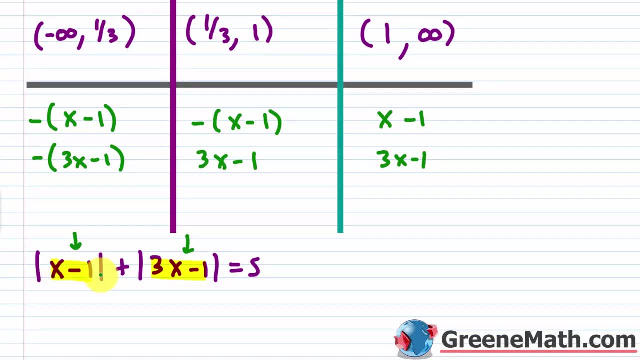 basically replace my absolute value expression in each case with what i came up with for the interval. instead of having the absolute value of x minus 1 because this guy is negative, i'm going to say it's negative of x minus 1. then we would have plus. you'd have the negative of this guy as well. so 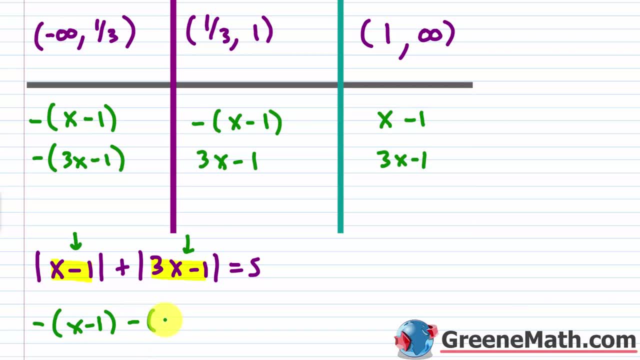 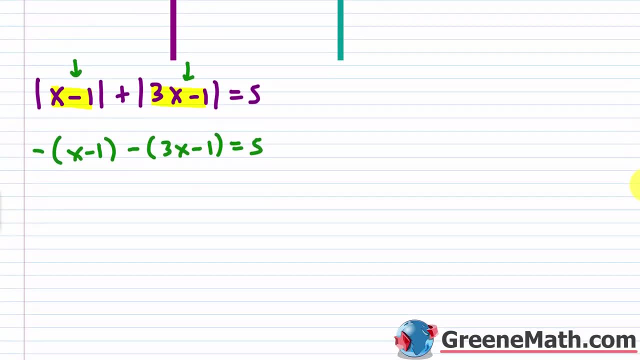 you can put plus negative or you just put minus. doesn't matter. so minus, you have the quantity 3x minus 1 and this is equal to 5.. okay, so let's scroll down and solve this and then we'll come back up. we just want to make sure we have enough room, so i'm going to distribute the negative to: 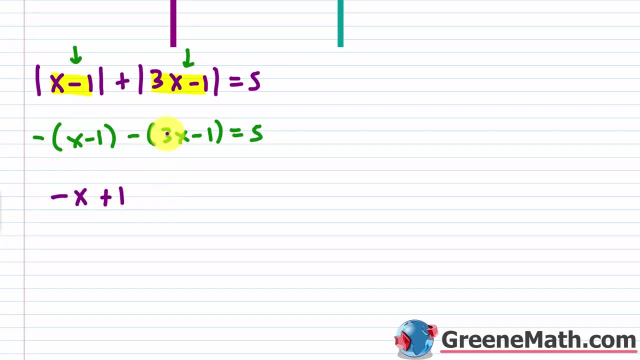 each part here. so this would be negative x plus 1. distribute the negative, so negative x minus 1. 3x plus 1, this equals 5.. so negative x minus 3x would give me negative 4x. 1 plus 1 is 2, so plus 2. 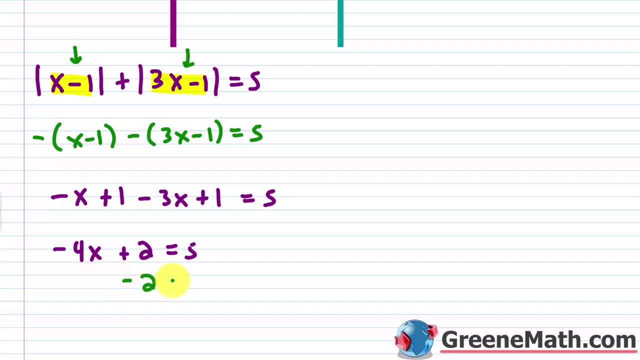 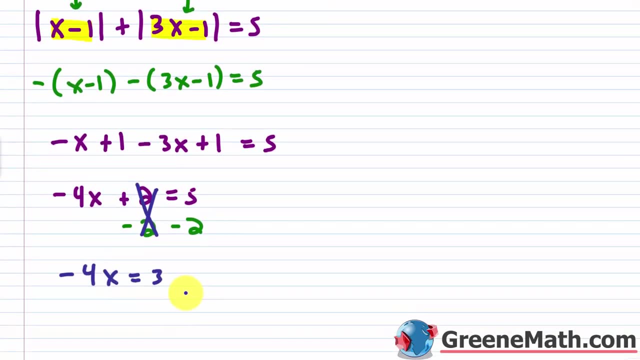 this equals 5.. and then what i'm going to do here is i'm going to subtract 2 away from each side of the equation and we're going to find that this is going to cancel. we're going to have that negative 4x is equal to 3.. we're going to divide both sides of the equation by negative 4.. so divide this by: 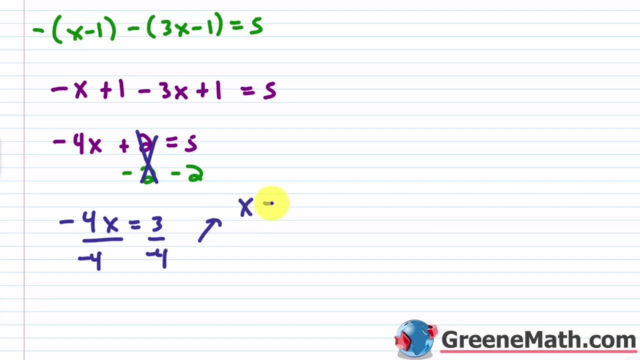 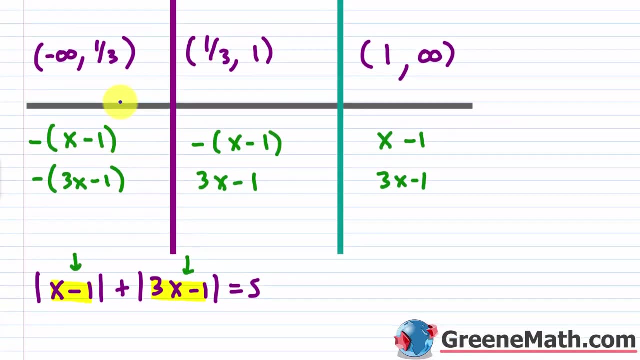 negative 4, and this by negative 4.. we're going to get that x is equal to negative three fourths. okay, so i want to erase everything and i want to show you what we do here. so let me erase all this. so the solution we found in this interval is that x is equal to negative three fourths. now what you? 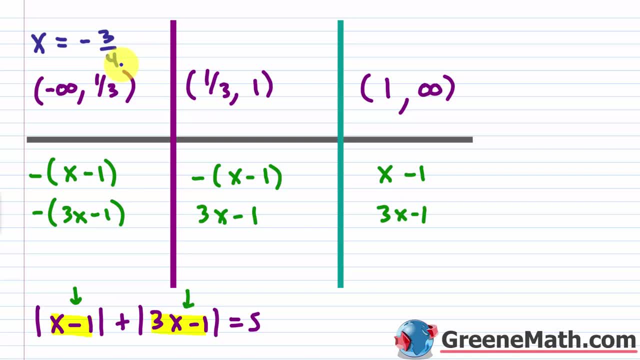 end up doing in this process is: if your solution lies in the interval, you accept it. if it lies outside of your interval, then you're going to reject it. since negative 3- 4 is in this interval, right from negative infinity up to, but not including one third, we can accept this solution. 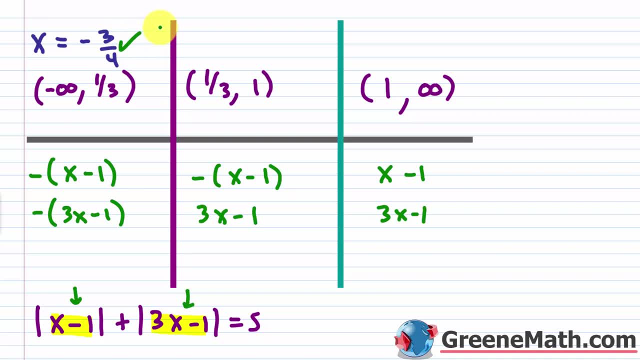 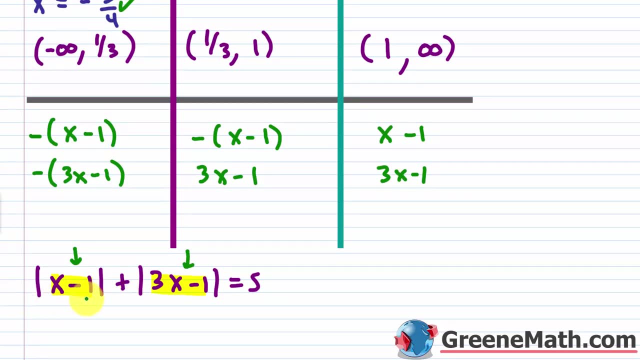 okay, so we're going to put that as part of our solution. okay, now we're going to work in this interval. okay, so let me go down a little bit. so this guy right here is going to be replaced with its negative, so the negative of x minus 1. 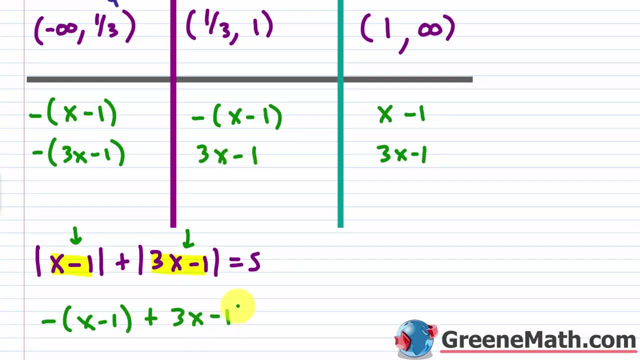 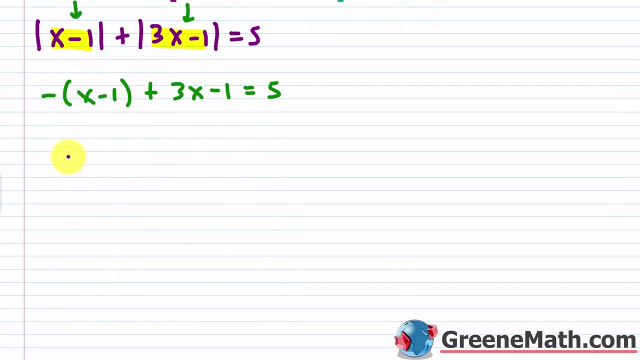 then plus this guy is positive. so we just say 3x minus 1, this equals 5.. okay, so let's go ahead and solve this and then we will come back up. so distribute the negative to each part. you have negative x and then plus 1, then plus 3x and then minus 1 equals 5.. so we know that 1 minus 1- those 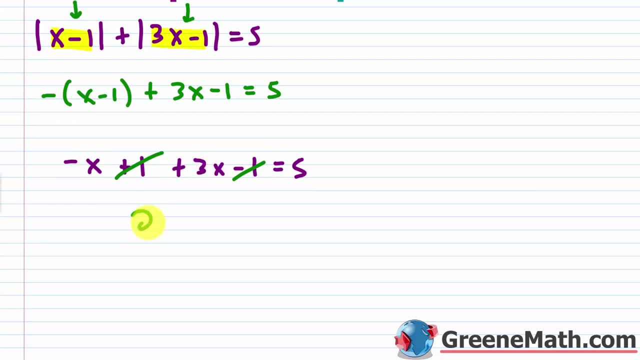 are the variables right, that's basically 0.. so you have negative x plus 3x, which is 2x. this is equal to 5.. okay, so what i'm going to do from here is i'm going to divide both sides of the equation by 2. 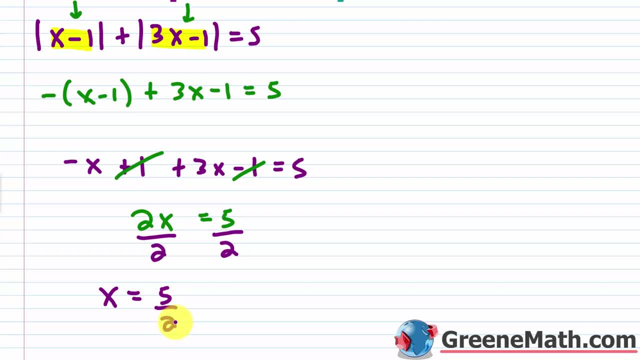 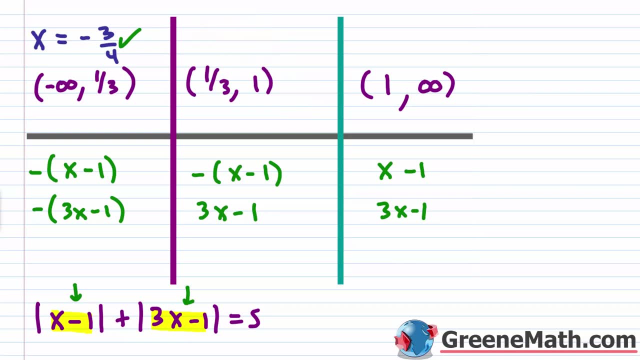 and i'm going to get that x is equal to 5 halves. now let me erase everything. let me paste this in so we have x equals 5 halves. let me kind of do this in a different color so it doesn't get confusing. so x equals 5 halves. those five halves lie in the interval. 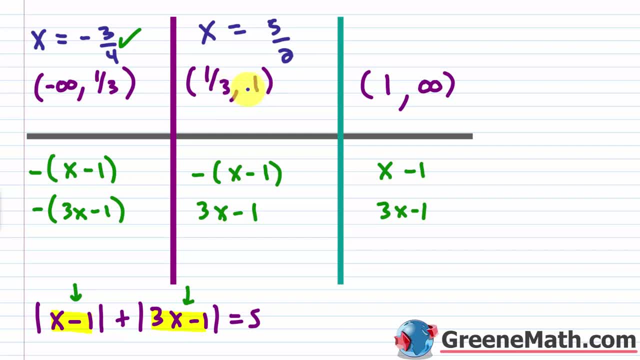 which is between and 1, right, With neither included? No, it doesn't, because 5 halves is 2.5.. So this is a solution we're going to reject, right, We're going to reject this solution. Now, we're going to move. 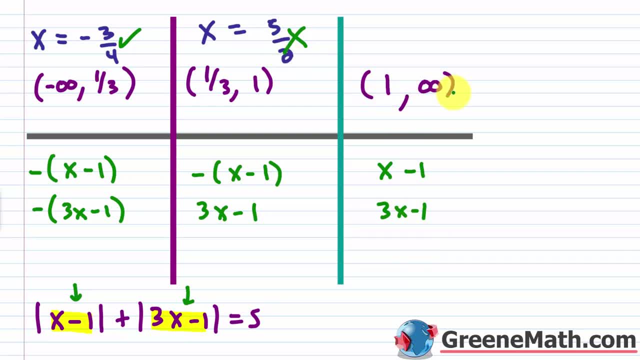 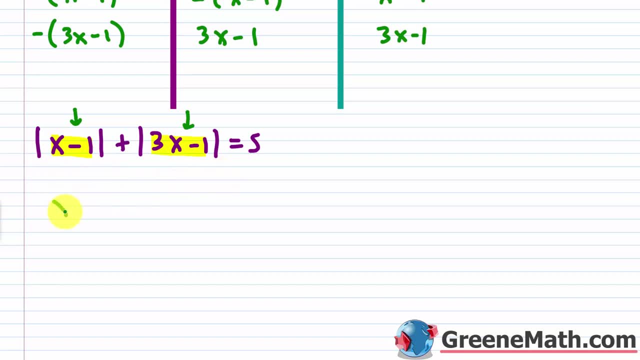 on to this interval right here, which is anything larger than 1.. So in this interval, both of these are positive. So what I'm going to do is I'm going to drop the absolute value bars in each case and just write what I have. So I'd have x minus 1 plus 3x minus 1, and this is equal to 5.. So then, 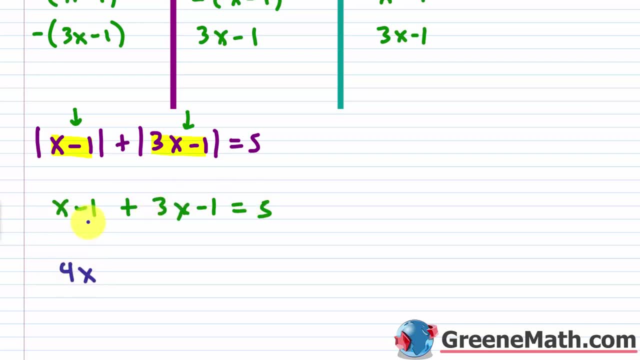 I would add x plus 3x, that's 4x. Negative: 1 minus 1 is negative 2. This equals 5.. We would add 2 to both sides of the equation, And so we would have that 4x is equal to 7.. We can divide. 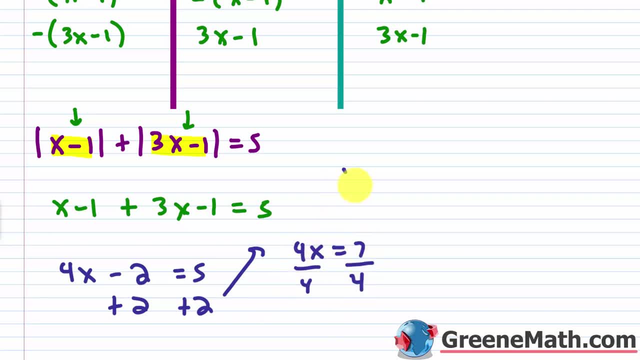 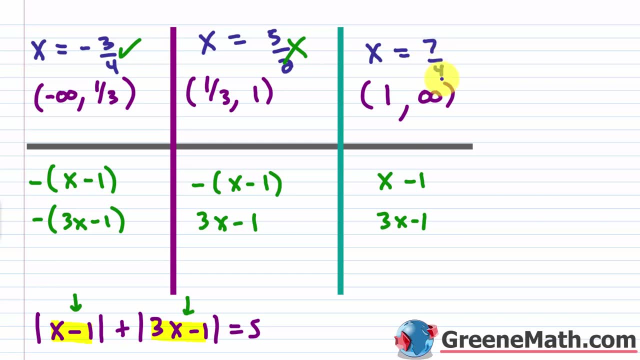 both sides of the equation by 4 and find that x is equal to 7 fourths. okay, So let me erase this once again and we'll say x equals 7 fourths. okay, So is 7 fourths in the interval again. 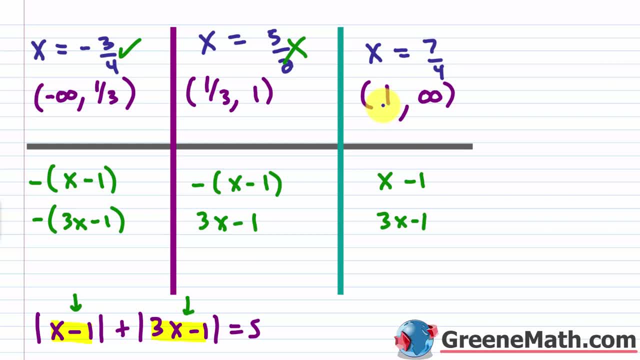 anything larger than 1?? Well, yes, it is. 7 divided by 4, in decimal form, is 1.75, so that's clearly larger than 1.. So your two solutions here. let me just kind of check this off. you would have that x is equal to negative 3 fourths, or x is equal to 7 fourths. So let's. 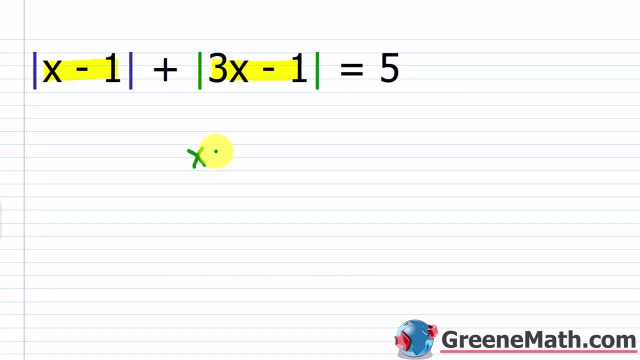 go back up here. I'm just going to erase this and we'll say that x is equal to negative 3 fourths and then also 7 fourths, right, And we rejected 5 halves. That didn't work. You can check this. 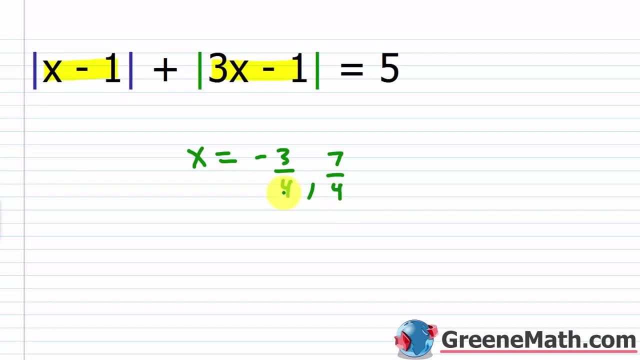 out. You can even check 5 halves and prove that to yourself, that it doesn't work If you plug in negative 3 fourths here. so you have the absolute value of negative 3 fourths minus 1, so minus 4. 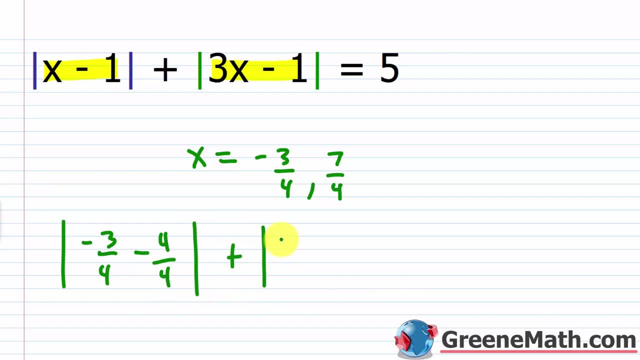 fourths. I'm just getting a common denominator, Then plus the absolute value of 3 times negative 3 fourths. okay, Then minus 1, and then this is equal to 5.. Negative 3 minus 4 is negative 7,. 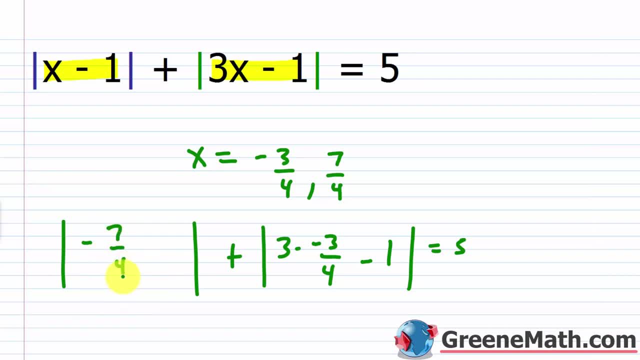 so this would be negative 7 fourths. And then if I took the absolute value of that, I'd have 7 fourths. okay, So this would be 7 fourths, so that works Okay. And then this guy right here, 3 times negative. 3 is negative 9, so this is negative. 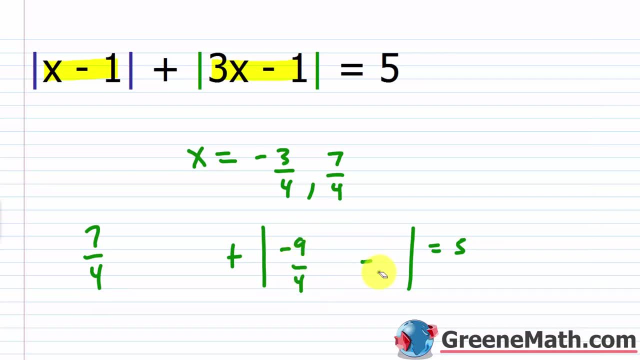 9 fourths. Again getting a common denominator. just write this as 4 over 4.. Negative 9 minus 4 is negative 13,. so you'd have negative 13 fourths. okay, So you'd have negative 13 fourths. Take the. 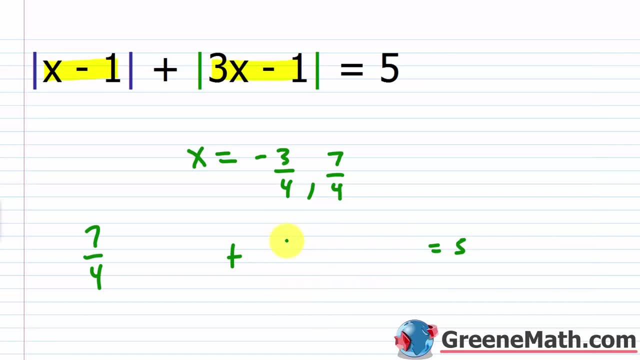 absolute value of that, you get 13 fourths, okay. So this is 13 fourths here, And what do you get? 7 plus 13 is 20 over the common denominator of 4, you would get 5, right? So you know this one. 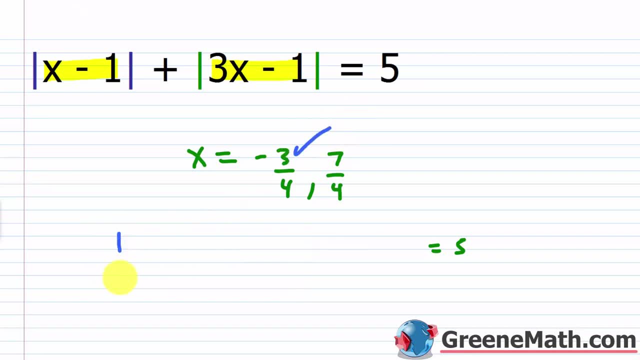 itself out. So this one checks out. All right, so let's check the other one. So the absolute value of you'd have 7 fourths minus for one. I'm going to put 4 fourths And then plus the absolute value. 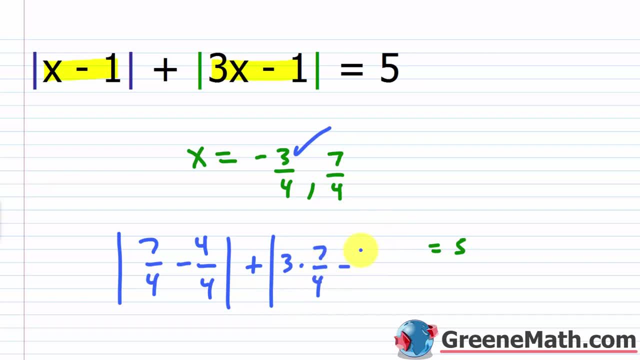 of 3 times 7 fourths minus. again for one, I'm going to put 4 fourths. So what do we have here? 7 minus 4 is 3, so over the common denominator of 4, this would be 3 fourths. Absolute value of 3. 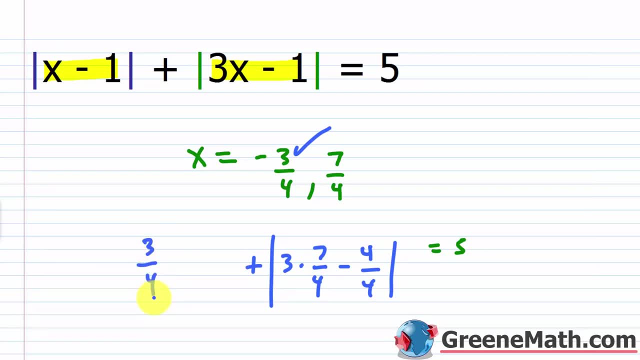 fourths is 3 fourths. okay, So that's 3 fourths. Then this guy here: 3 times 7 is 21,. so you would have 21 minus 4 is 17.. So you would have 17 fourths. okay, 17 fourths. Absolute value of 17. 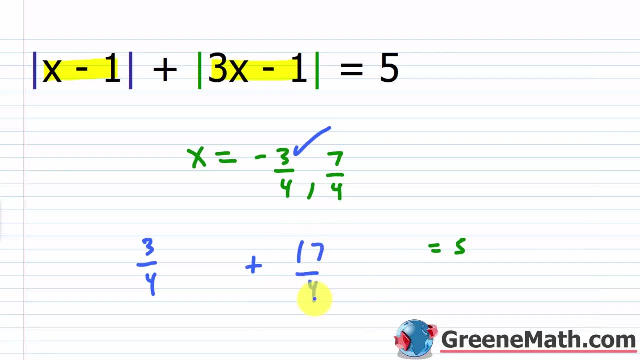 fourths is 17 fourths, And you see that this works right. 3 plus 17 is 20,, 20 over 4 is 5, so you get 5 equals 5.. So this works out as well. So you can also do 5 halves and prove that it. 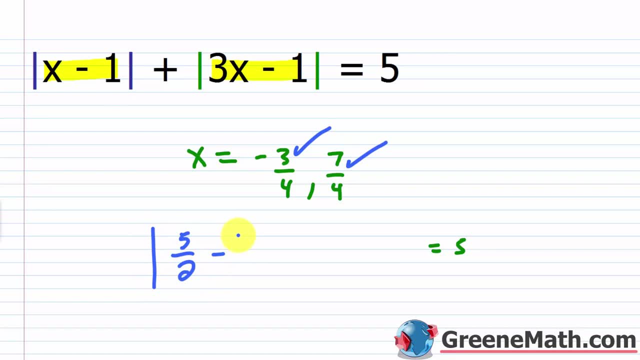 doesn't work. So you'd have 5 halves minus. in this case I'm going to write: 1 is 2 over 2. And then plus you'd have 3 times 5 halves and then minus 1.. 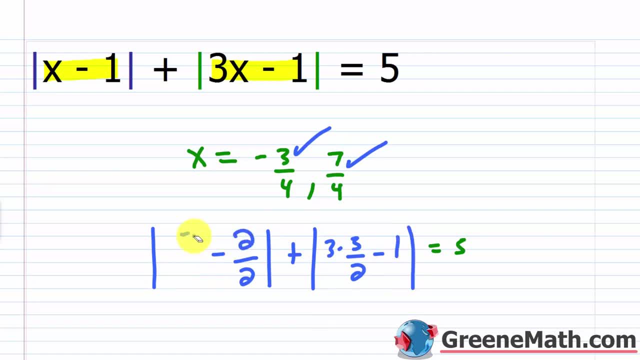 So we know that this would be what. This would be: 3 halves, This would be 3 halves. Absolute value of 3 halves is 3 halves. so this would be 3 halves. And then this guy 3 times 5 is 15,. 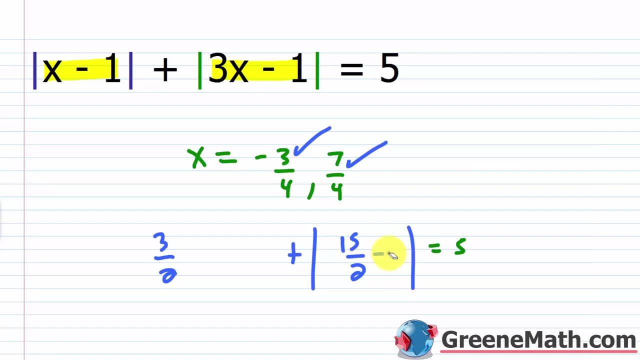 so you'd have 15 halves. Again, I'm going to write this as 2 over 2.. 15 minus 2 is 13,, so you'd have 13 halves. Absolute value of 13 halves is 13 halves. 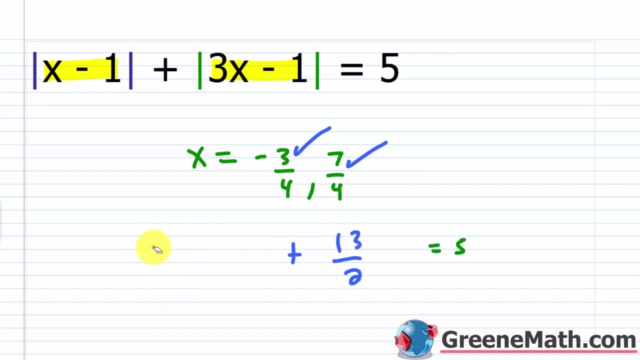 So in this case you'd get 3 plus 13,, which is 16.. And so you'd have 16 over 2, which is 8.. 8 equals 5, which is false. okay, That's false. So that solution where x equals 5 halves. 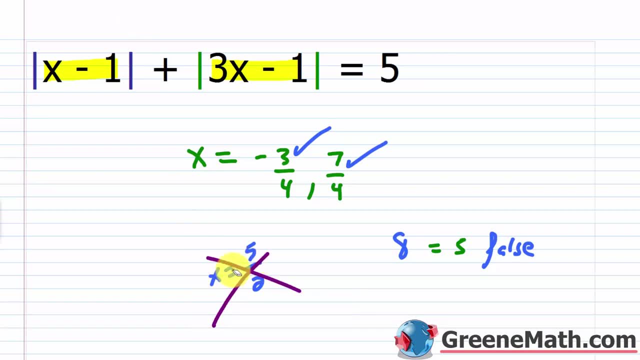 again, you've got to reject this. This does not work okay, And we found that because it wasn't in the interval. we knew it wasn't going to work. Now let's talk a little bit about the alternative method to solve this. This is one that I don't recommend, because it just takes a lot more time. 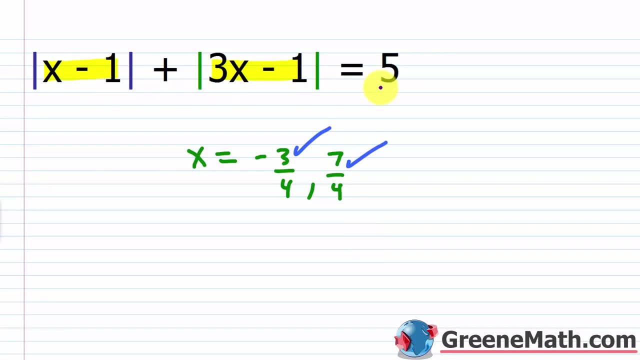 So what you can do is you can consider all the cases that you would be presented with this. So, in other words, you would be able to solve this with the alternative method. So you would be able to solve this with the alternative method. So you can consider if this expression is positive and 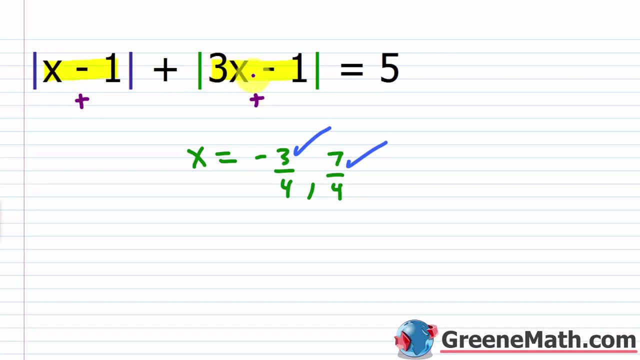 this expression is positive, you would just have x minus 1 plus 3x minus 1 equals 5, okay. So that's one scenario that you would encounter. Then another scenario would be this one's negative and this one's positive. So, in other words, I would put a negative out in front of this and 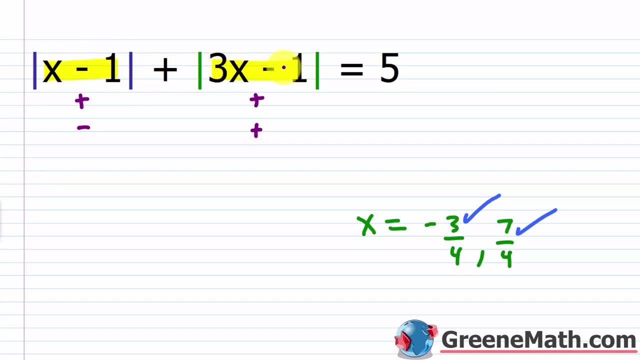 say the negative of x minus, 1 plus, and then this guy's positive, so 3x minus 1, and this equals 5.. So I'd solve that equation right And you keep going. So this would be positive and this would. 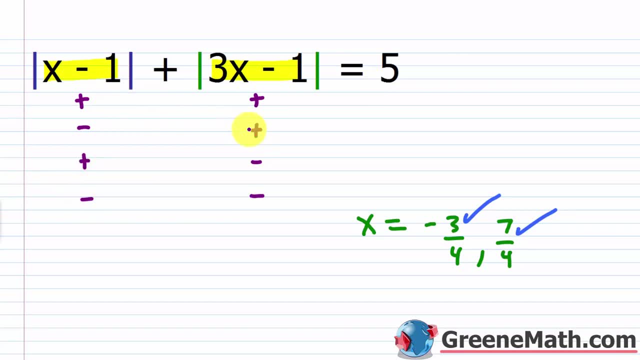 be negative, and this would be negative and this would be negative. So you basically have to solve that: four equations to set up and solve, but then you get extraneous solutions, So you have to go back and check each one of those. okay, And with our method we really don't need to check, We just 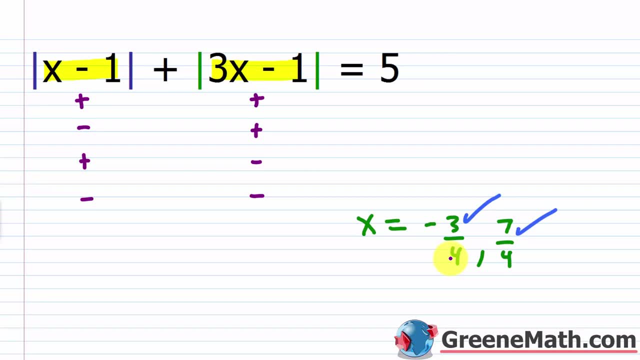 need to verify that our solution lies in the interval that we've created, and then we're basically good to go. okay, So once more, the solution here is that x equals negative 3 fourths or 7 fourths. All right, let's go ahead and take a look at another one of these. So we have the. 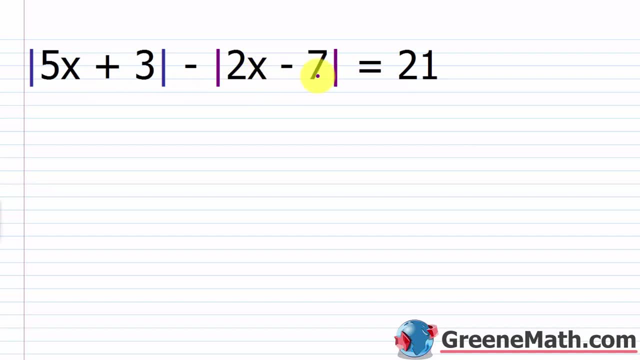 absolute value of 5x plus 3,, then minus the absolute value of 2x minus 7, and this equals 21.. So again, it's the same thought process I'm thinking about where this guy is 0 and where. 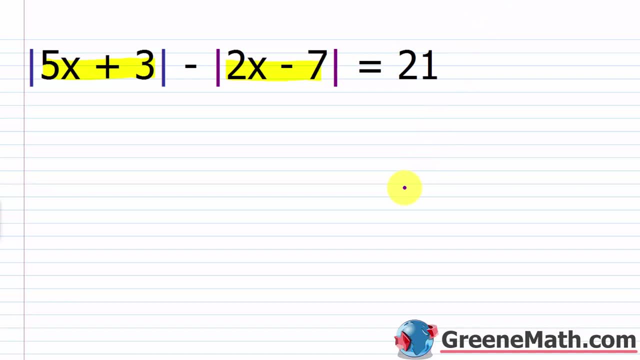 this guy is 0. I'm using that to kind of set up intervals on my number line. So we'd have 5x plus 3, and we'd say: where is that equal to 0?? So I would subtract 3 away from each side of the. 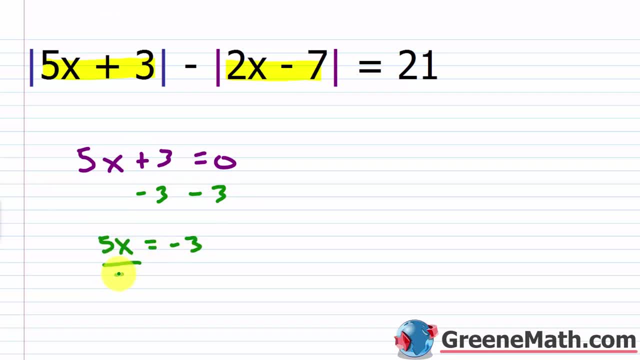 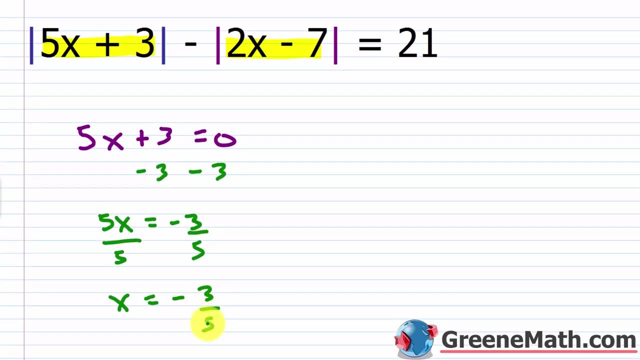 equation I would get: 5x is equal to negative 3, divide both sides by 5, and I get that x is equal to negative 3 fifths. okay, So that's going to be one of those guys. Then, for this guy right here: 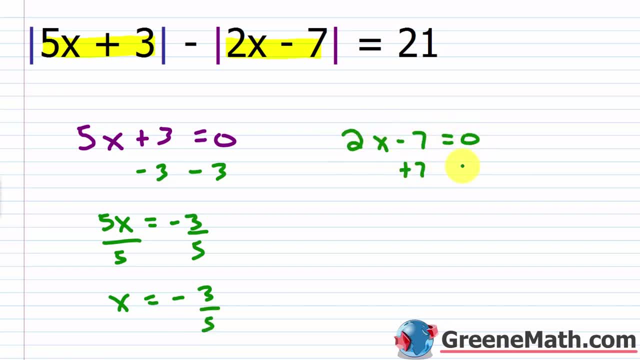 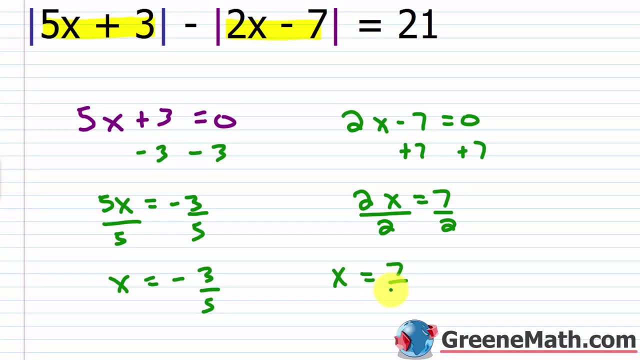 2x minus 7 equal to 0.. Let's add 7 to both sides of the equation. We get 2x is equal to 7, divide both sides by 2.. We get x is equal to 7 halves okay. So basically I'm going to have an. 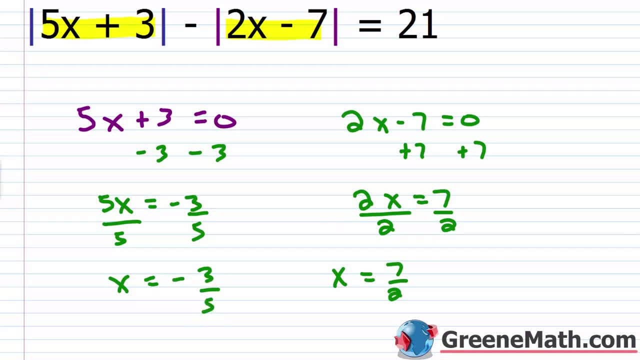 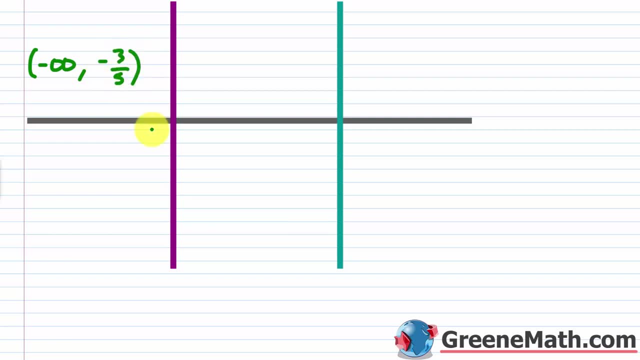 interval that is anything less than negative 3 fifths. So let's write that first, So we'll put negative infinity here up to, but not including negative 3 fifths. Then I'm going to have an interval between negative 3 fifths and 7 halves, with neither included. So you have. 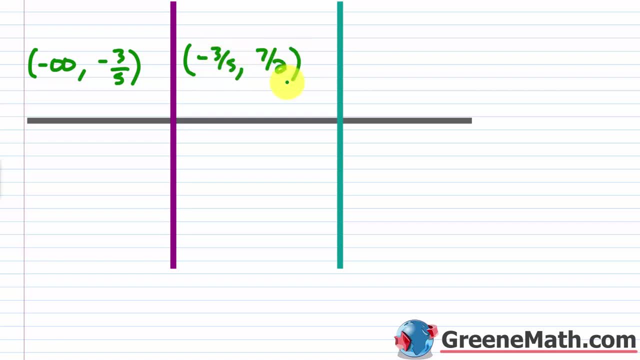 negative: 3 fifths and 7 halves. Again, neither one's included. And then, lastly, we have an interval where we're greater than 7 halves. okay, So where we're greater than 7 halves, Okay. so let's rewrite our absolute value equation, So we have the absolute value of 5x plus 3,. 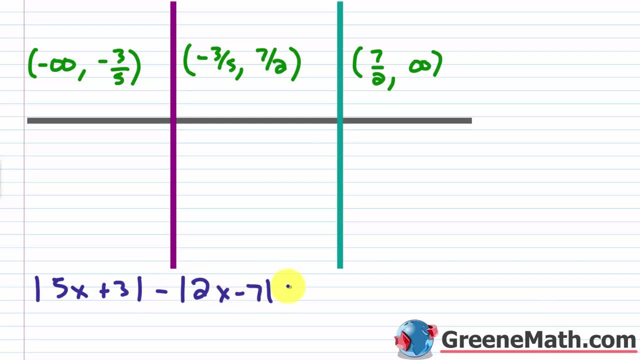 and then minus the absolute value of 2x minus 7. This guy is equal to 21.. So again, I'm just going to write positive and negative. Again, if it's positive, I can just kind of drop the absolute value bars. If it's negative, I can drop the absolute value bars, wrap it in parentheses. 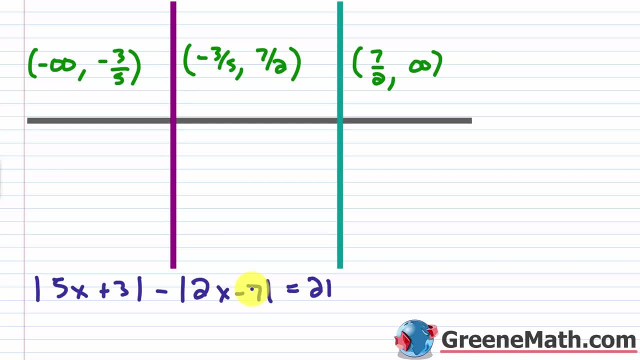 and put a negative out in front right to change it into its opposite. So we know that if we're less than negative 3 fifths, both of these expressions are going to be negative, right? So 5x plus 3, I'd wrap that in parentheses- put a negative out in front 2x minus 7,. 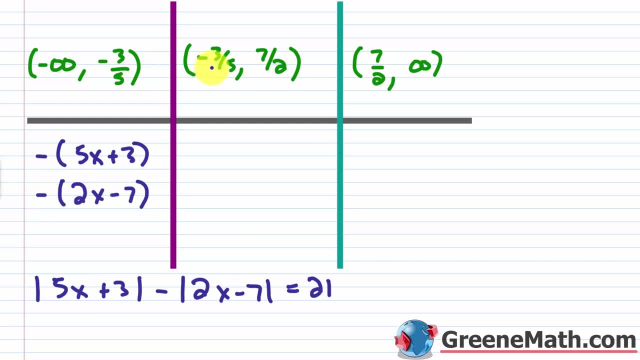 I'm going to wrap that in parentheses. put a negative out in front. If I'm between negative 3 and negative 7, I'm going to put a negative out in front. So I'm going to put a negative out in front. 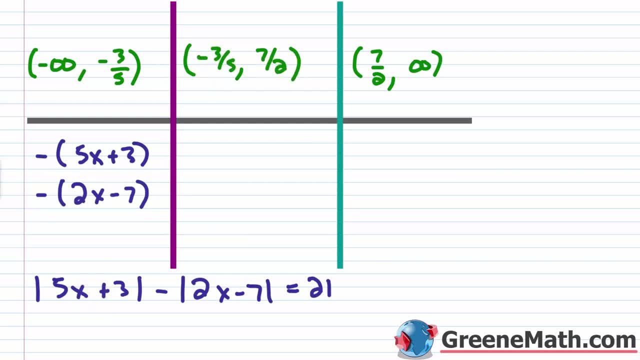 3 fifths and 7 halves. I know this guy right here is going to be 0 at negative 3 fifths. So if I'm greater than negative 3 fifths, that guy's positive right. So 5x plus 3 is positive And I can go. 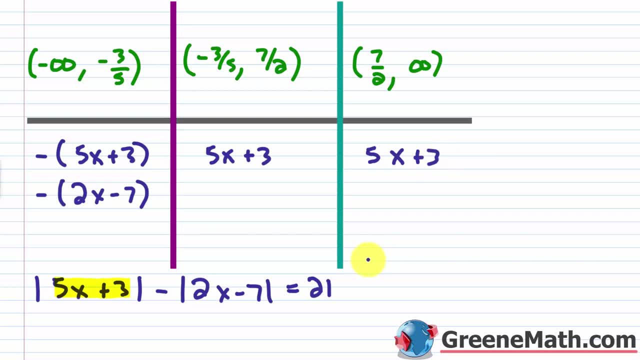 ahead and just say it's going to be positive in this interval as well. right Now, this guy right here, this 2x minus 7, this guy is going to be 0 when x is 7 halves. So it's still going to be. 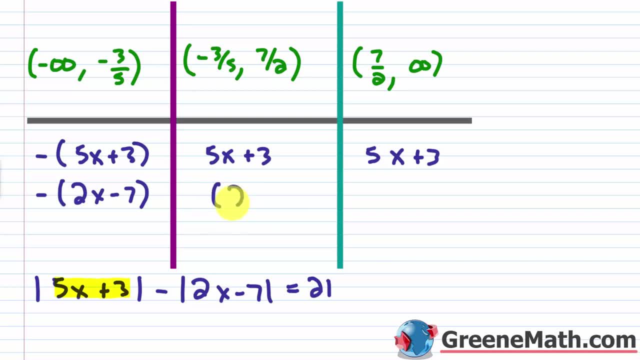 negative in this interval here, So we would wrap this in parentheses and put a negative out in front, And again in this interval. it's positive because everything's positive once we get larger than 7 halves, because 7 halves makes this guy 0. So we'll say this is just 2x. 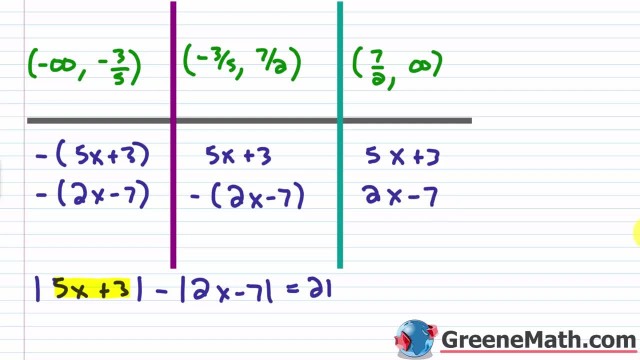 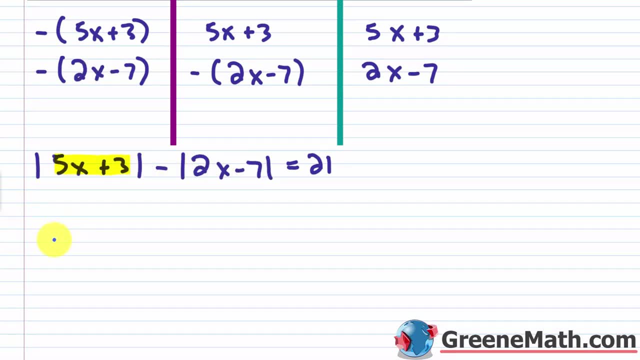 minus 7.. Okay, So let's go through the possibilities, Let's scroll down, Let's think about the first one. So, all the way to the left, I'm going to replace each one of these with their opposites. So I'm going to have the negative of 5x plus 3. And then minus. you've got to be very 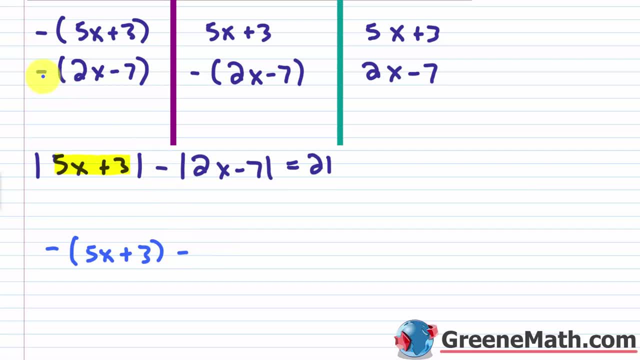 careful, because this is a minus here, And then you're putting a negative out in front. So I'm going to put a negative out in front. So minus a negative is really plus a positive, right. So minus a negative and then times the quantity 2x minus 7, I'm going to put plus, Okay, So plus. 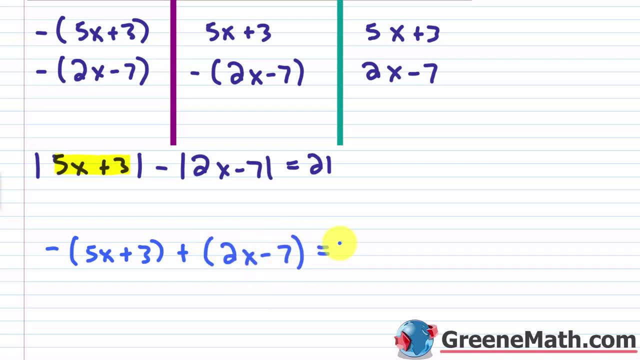 2x minus 7.. Okay, And then this equals 21.. All right, So I'm going to distribute this negative to each term. I'll have minus 5x and then minus 3, and then plus 2x and then minus 7.. This equals. 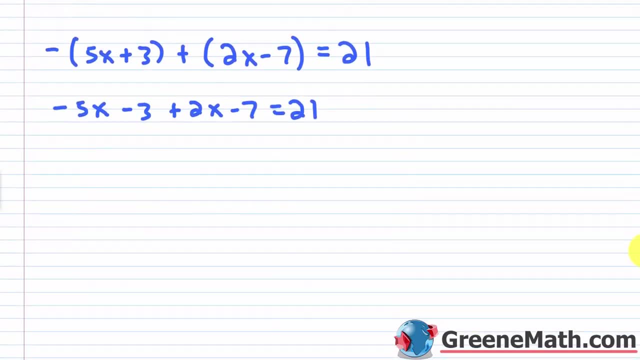 21.. Okay, Let me scroll down and get some room going. We'll come back up. So this guy right here. so negative 5x plus 2x, that's going to be negative 3x, And then negative 3 minus 7 is negative 10.. This equals 21.. Let's add 10 to both sides of the. 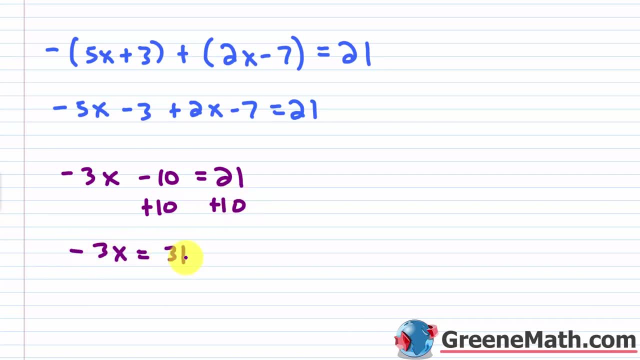 equation We're going to get: negative 3x is equal to 31.. We're going to divide both sides of the equation by negative 3. And we're going to get that x is equal to negative 31 thirds. Okay, So. 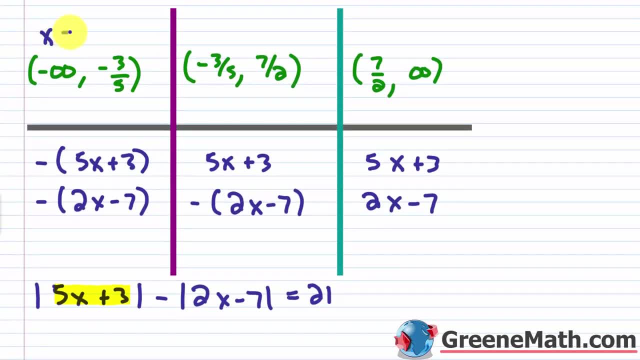 let's copy this, So let me just write that in here. X equals negative 31 thirds. Okay, Negative 31 thirds. So is this valid? You just need to ask yourself the question: does it lie in this interval? And the answer to that is yes, Right, Negative 31 thirds. 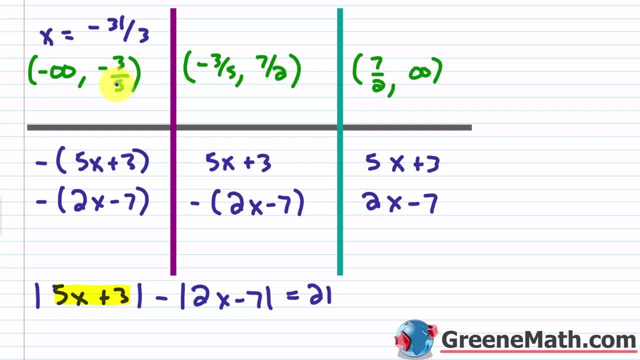 is more negative or to the left of negative three fifths. So you can clearly see it would be in this interval. So this guy, we'll go ahead and check it off and say that's a valid solution. All right, Let's talk about in this interval here between negative three fifths and seven halves. 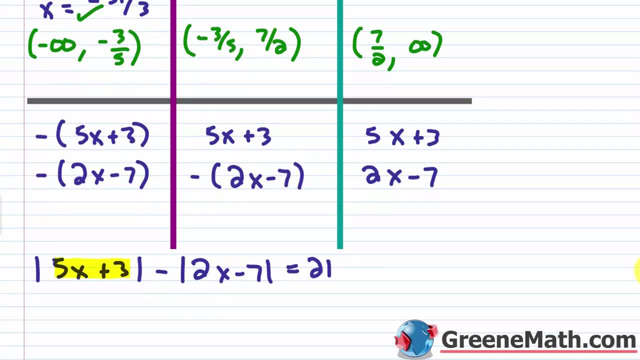 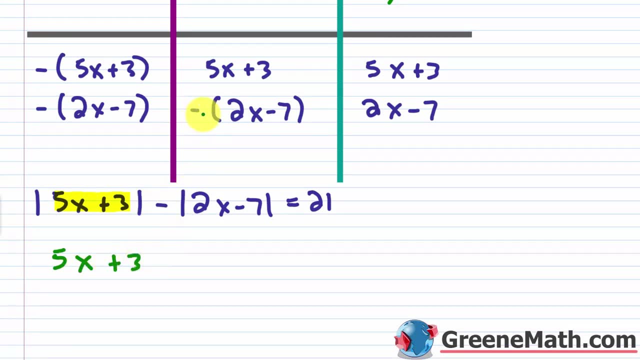 So this guy's positive and this guy's negative. So let's scroll down a little bit and we'll say plus three. Again, if I have a minus, a negative, it's plus a positive. So you just say plus there again, two X minus seven. And I really don't need the parentheses, I can just drop them. 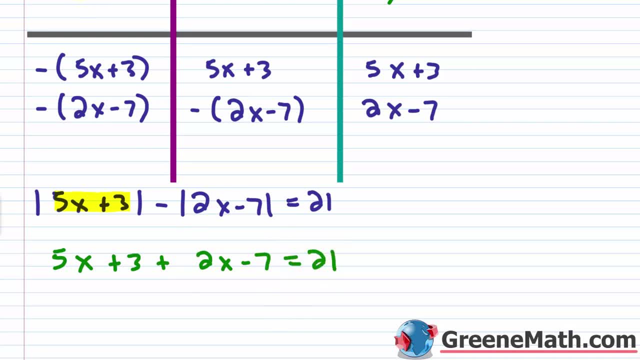 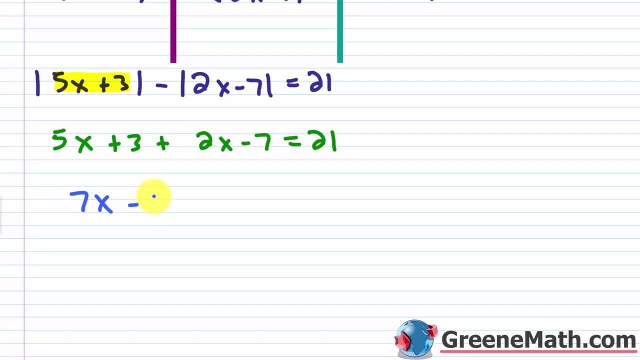 And then this equals 21.. So let's just solve this real quick. I'm just going to scroll down and get a little room going. We'll come back up. So five X plus two X is seven X. three minus seven is negative four. This equals 21.. And let's go ahead and add four to both sides of the equation, So we 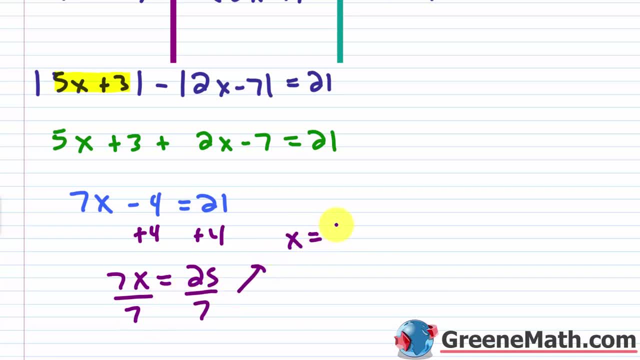 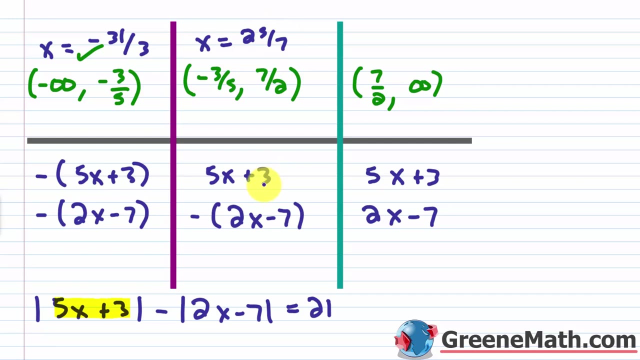 divide both sides of the equation by seven, We'd find that X is equal to 25 sevenths. All right, So let me kind of copy this real quick. I'm just going to erase all this work. We're going to go back up. So again, X is equal to 25 sevenths. So 25 sevenths. So is that in the interval again, 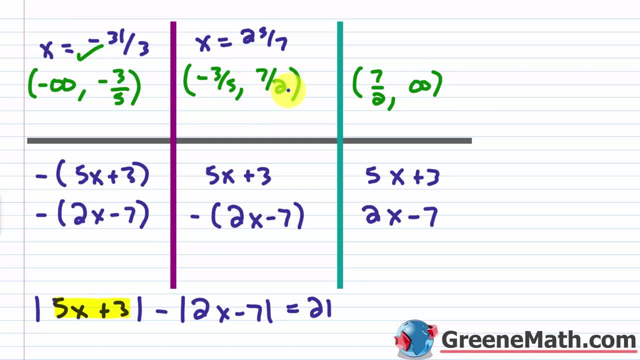 between negative three fifths and seven halves. Well, negative three fifths is basically negative point six as a decimal, Seven halves is three point Okay. And if I think about 25 sevenths, that's a little bit larger than 3.5.. It's 3.571.. If you. 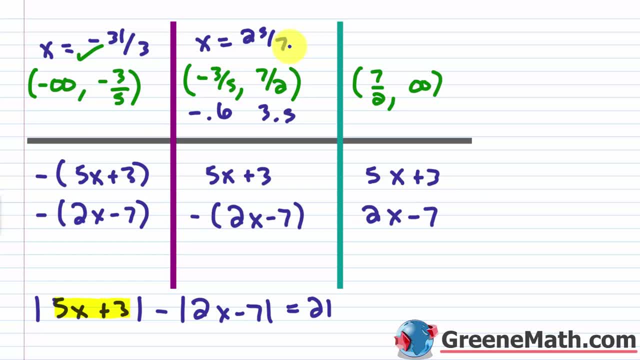 wanted to kind of go to three decimal places, So it is larger than 3.5.. So it's outside of this interval. So we're going to end up rejecting this solution. Okay, It's not going to work. So let me do that in red. I'm going to reject this, And so now we just have to check this. 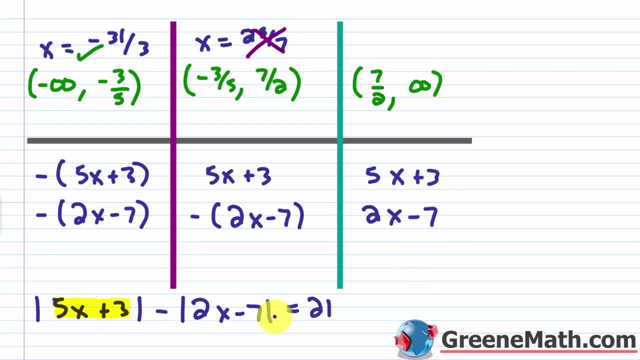 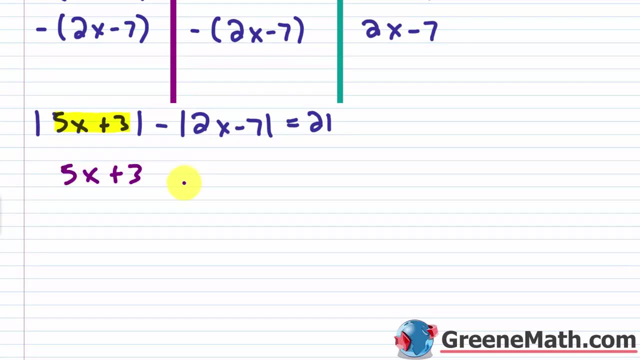 interval here, So everything's positive. So I can just drop the absolute value bars, So we kind of go down and do that. So we would have five X plus three, And then basically you're subtracting away this whole thing. Okay, You've got to be careful there. So what I'm going to do is I'm going to 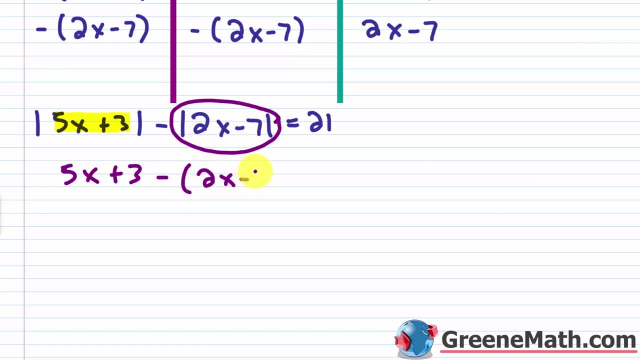 say minus- I'm going to wrap this in parentheses: two X minus seven, because again this whole thing's being subtracted away. Don't make the mistake of just putting a minus two X and then leaving this as negative seven, because this has to be changed And so does this. Okay, You got to. 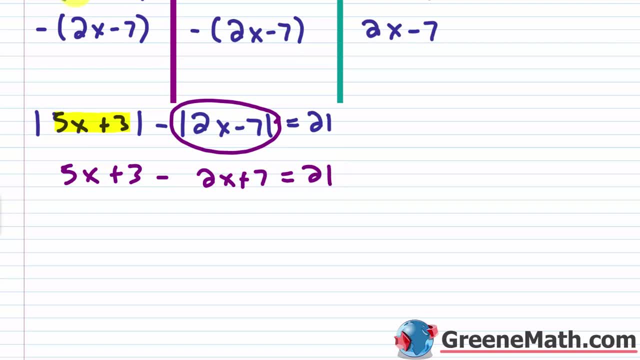 be very careful there. So then this equals 21.. Okay, So I'm going to go ahead and say five X plus two X is three X, and then three plus seven is 10.. So plus 10 is equals 21.. Let's go ahead and. 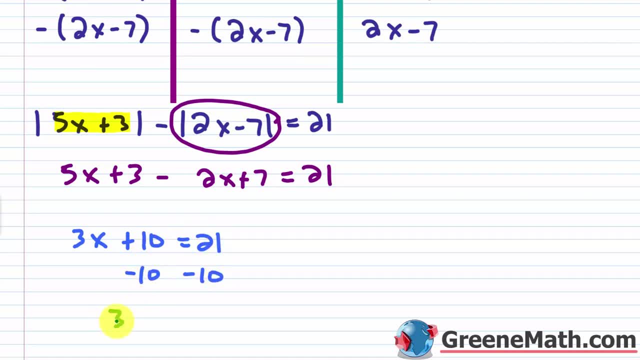 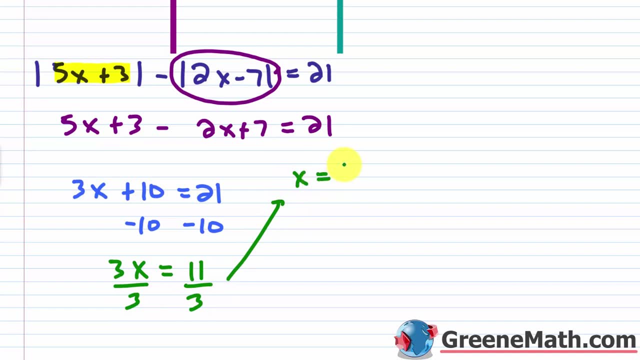 subtract 10 away from each side of the equation And we'll say that three X is equal to 21 minus 10 is 11.. Divide both sides by three. We're going to get that X is equal to 11 thirds. Okay, So once. 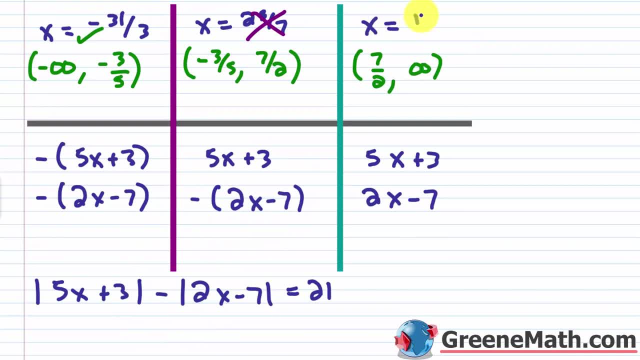 again. let me erase everything. All right. So we found that X is equal to, again, 11 thirds. Okay, So is 11 thirds in this interval? Well, seven halves is 3.5.. So it needs to be larger than that. And if you punch up 11 divided by three, 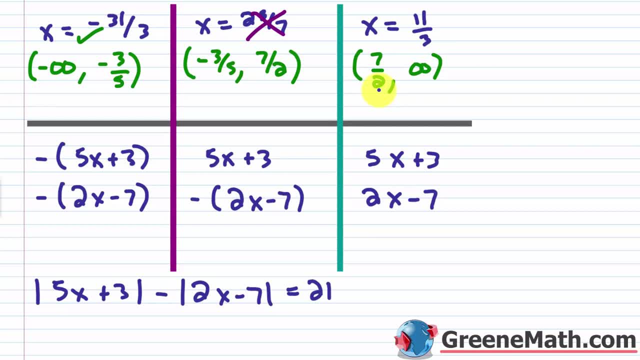 in a calculator you get 3.6 where the six repeats forever. Okay, So that is going to be larger than 3.5.. So this guy is going to work out as a solution. So the two solutions are going to be: 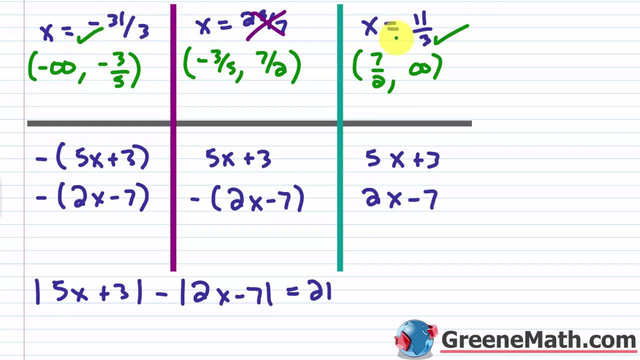 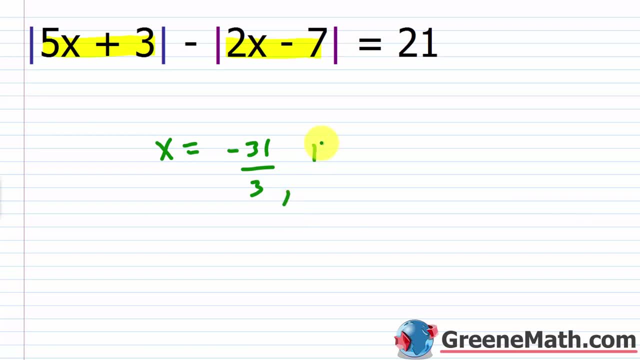 X equals negative 31 thirds, and then X equals 11 thirds. So let me go back up, So we'll say that X is again equal to. we have negative 31 thirds and also 11 thirds, All right, So let's. 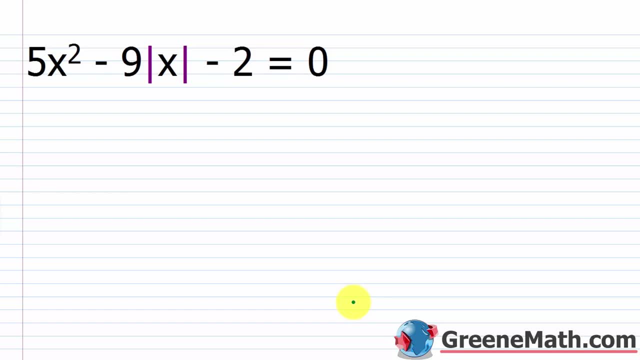 wrap up our lesson and look at: X equals 11 thirds. So let's wrap up our lesson and look at another common type of problem that you'll see. So let's say we ran into something like this: We have 5X squared minus nine times the absolute value of X minus two, and this is equal to zero. 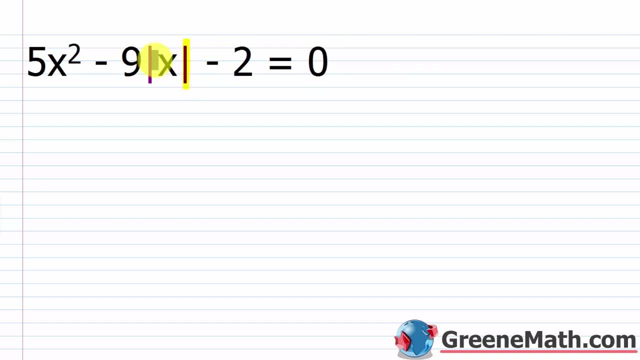 So in this particular case we have this absolute value operation. that's kind of in the middle of our equation and we can't really isolate it. So there's kind of two different ways to solve this. One of them is just to consider the two cases and then just kind of go back and think about if the 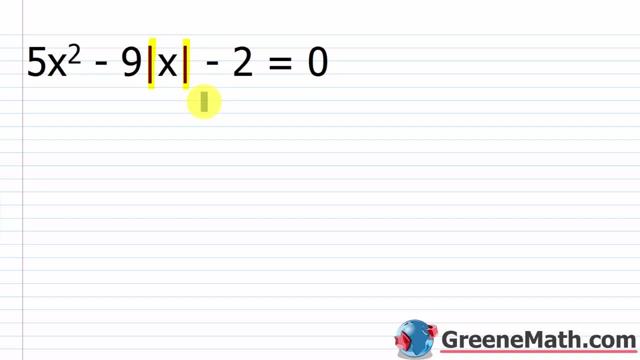 solutions that we get work right. So let's say that we have a solution that we can't really isolate, So you just plug them back in. The other one would be to kind of make a little substitution and then you can consider if things are valid or not from that. So let's try it. the 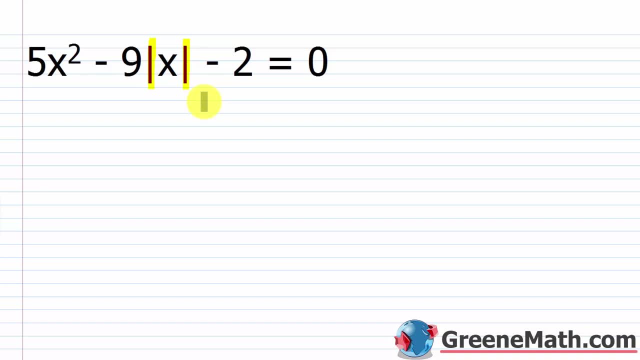 first way, and then I'll show you the substitution method. I prefer the substitution method on this, but you can do it either way. So there's two cases here. One case would be that this value here is going to be positive. So in that case we just remove the absolute value bars. So you would have. 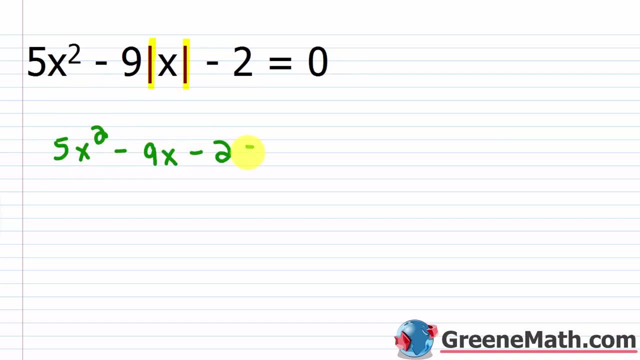 5X squared minus 9X minus two equals zero. So in this case we just remove the absolute value bars. And then the other case, kind of the case over here, would be: let's say, this expression was negative, So then I'd remove the absolute value bars and I would make X negative, X right. So we 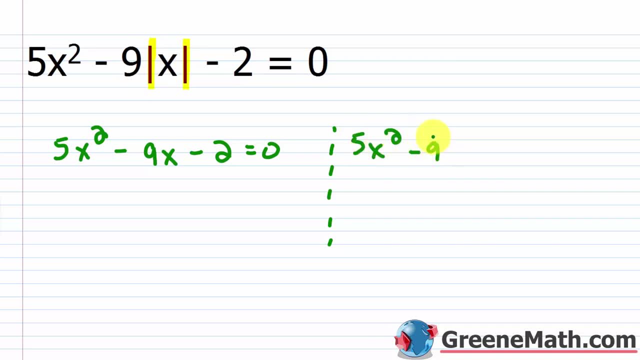 would have 5X squared minus 9.. It's being multiplied by this, and I'm multiplying it by the negative of X, and then minus two, and this equals zero. Of course we could simplify this, because negative times, negative is positive, So I can now write this as plus 9X. okay, So plus 9X. 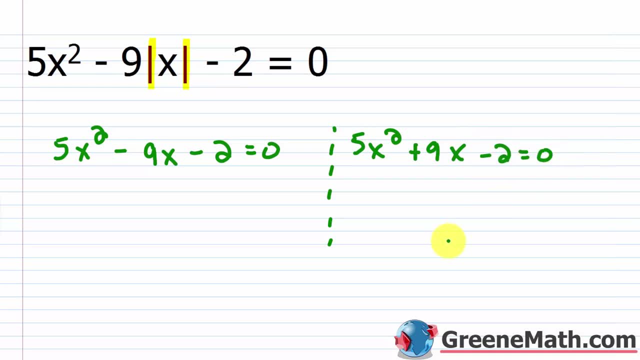 Let me kind of tighten this up. Let me tighten this down a little bit. Just move that over there, Okay. so let's start over here on the left. So this is something we can factor over here on the left. So let me kind of set this up. 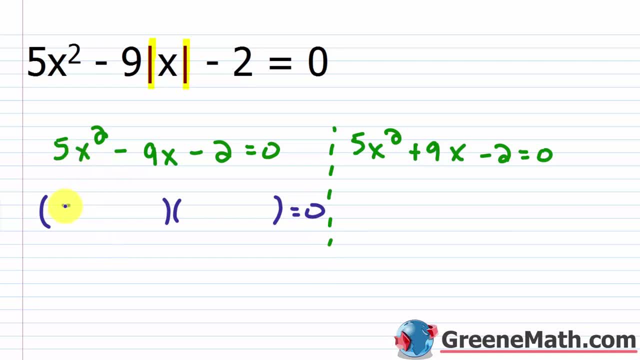 and we'll factor this guy real quick. So I know that this is going to be 5X and this is going to be X, because this is a prime number here. So I need to make sure the outer and the inner work itself out. So I'm looking for what I'm looking for: a middle term of negative 9X, and I'm looking 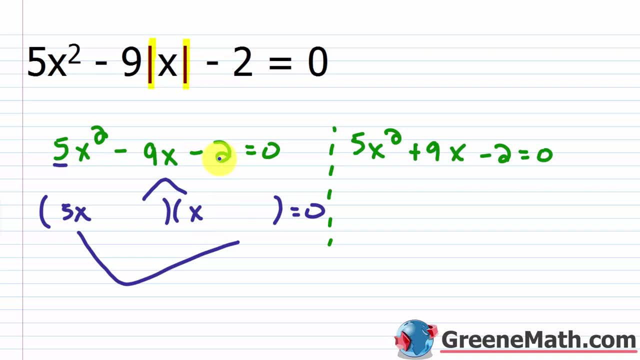 for a final term of negative two. So when we think about negative two, we're going to have a two. We know something's got to be positive and something's got to be negative, okay. So we also know that the factors there could be, you know, one and negative two, or it could be negative one. 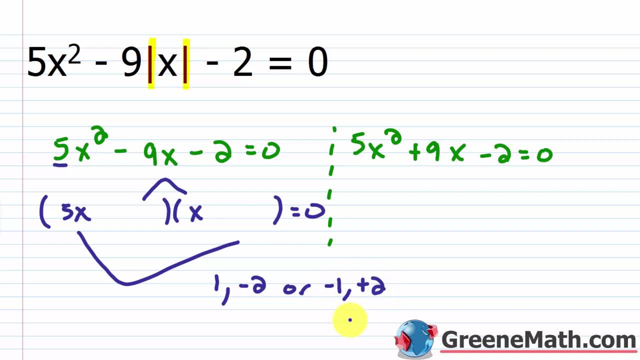 and positive two. okay, So let's say I put my negative two here and my positive one here. Would that work? So in this case, 5X times negative two would give me negative 10X and then one times X would be plus X. So this does work. 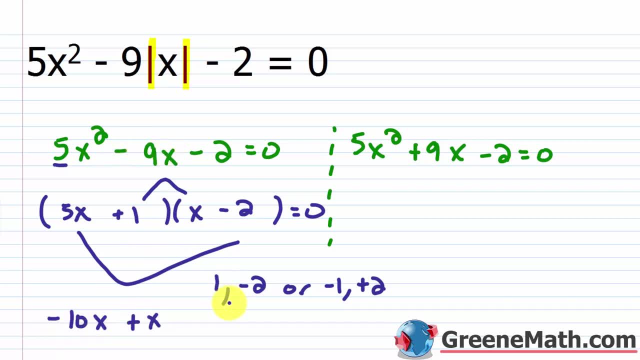 Negative 10X plus X would be negative 9X, and then, if you think about one times negative two, of course that's negative two. So this is our correct factorization. here and now we can just solve this pretty easily. We're going to take each factor and set it equal to zero, So 5X plus one. 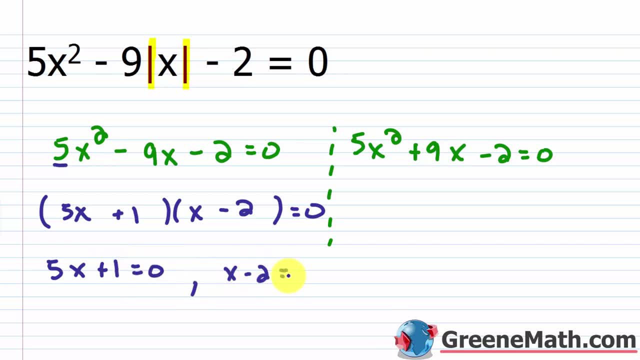 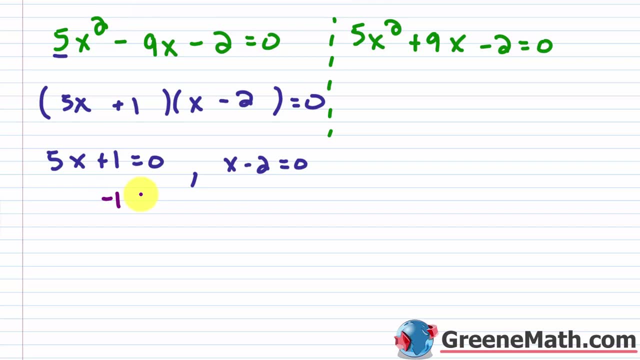 equals zero. and then we're also going to have that X minus two is equal to zero. Let me kind of scroll down real quick, get a little room going, And so, to solve this one, I'm going to subtract one away from each side of the equation. I'll have 5X zero and then I'm going to subtract. 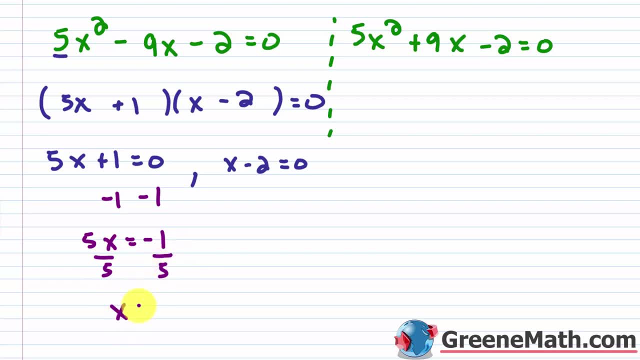 one away from each side of the equation. So I'm going to subtract one away from each side of the equation and I get X is equal to negative. one-fifth okay. Then over here, let me add two to both sides of the equation and I get that X is equal to two. okay, Now, these are just proposed. 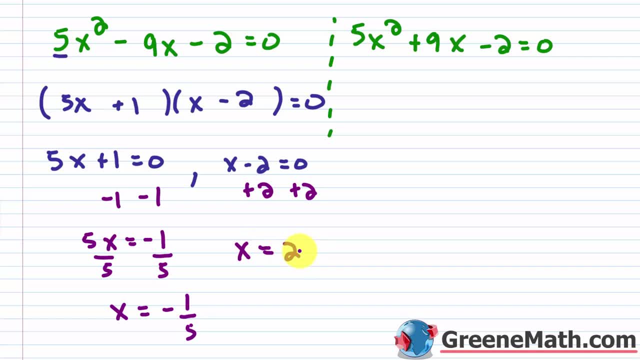 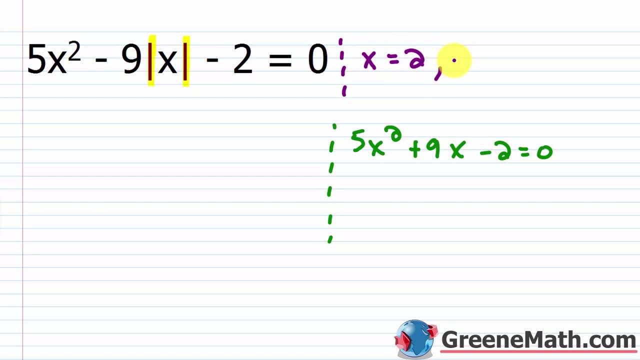 solutions. We actually need to check them in this scenario. So let me erase all this and I'm just going to copy these. So I'm just going to put this over here. We have X is equal to two and then common negative one-fifth. We'll check them in a minute. We're going to find that some of these 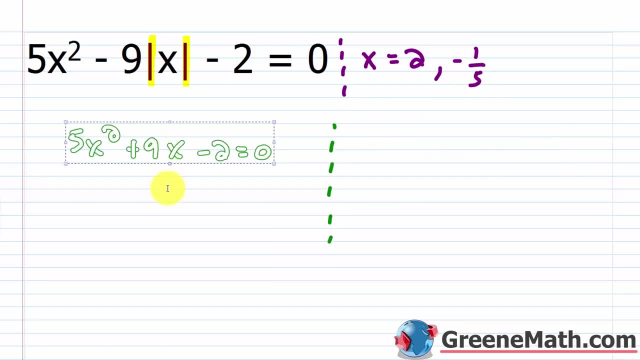 won't work, So let's move this over here. So let's move this over here, and we're going to here and let's work on this. now We'll get the solutions for this and then we'll check everything at once, okay? So for this guy, we can also solve this with factoring, So let's go ahead. 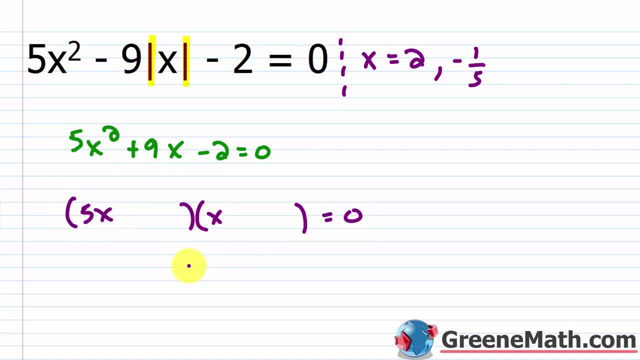 and set this up So we can again do 5X and X Again. I'm looking for the outer and the inner, such that I get a positive 9X as my middle term and a negative two as my final term. 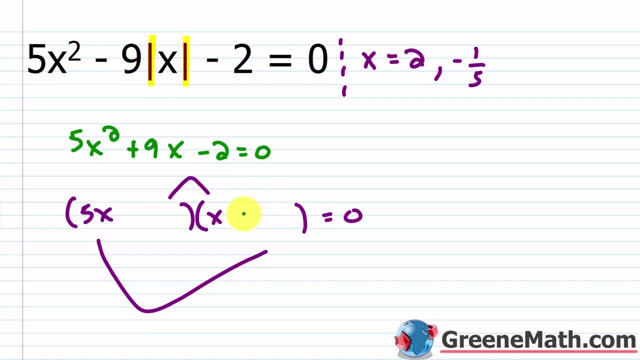 So, instead of doing a negative two here, I'm going to do a positive two. and instead of doing a positive one-fifth, I'm going to do a positive two. So, instead of doing a positive one-fifth, I'm going to do a negative one, right? Because my outer would be 10X and my inner would be. 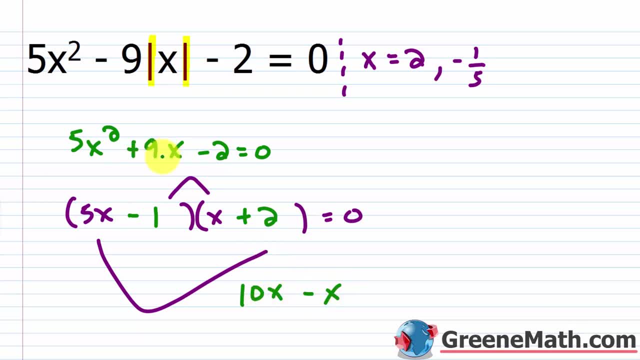 minus X. So 10X minus X would give me my positive 9X, and then negative one times two would be negative two. Okay, so we're good to go there, All right. so now I'm just going to set each of. 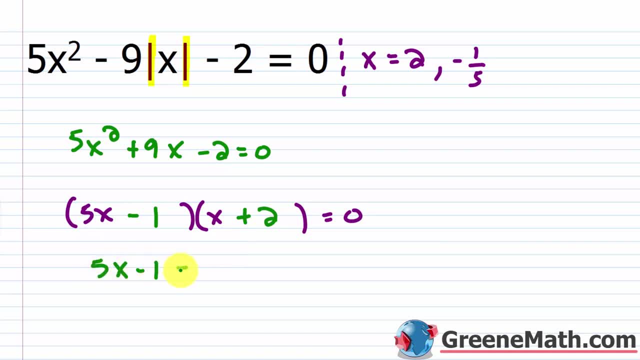 these equal to zero. So 5X minus one. if that equals zero, we're going to find that we add one to each side of the equation. We'll get that 5X is equal to one. divide both sides by five. 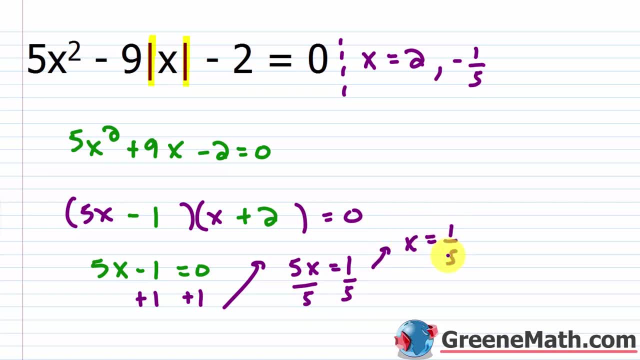 and we're going to get that X is equal to one-fifth. Okay, so let me just write that in here. So we have one-fifth, and I'll just erase this. We don't need this information anymore. And then we also have X plus two. We're going to set that. 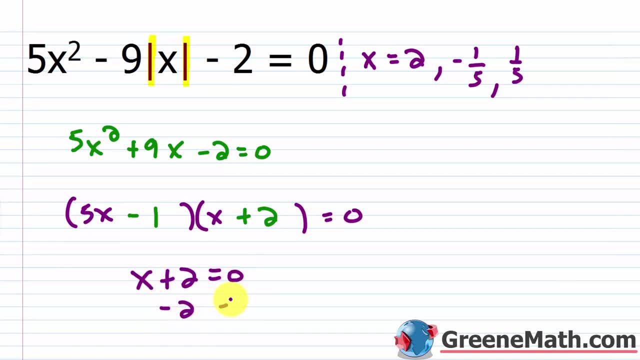 equal to zero. Of course, that gives me a solution. If I subtract two away from each side, that X is equal to negative two. Okay, let's put negative two in there, All right? so let's erase everything. and now we just want to check our solutions and see what works and what doesn't. Okay, 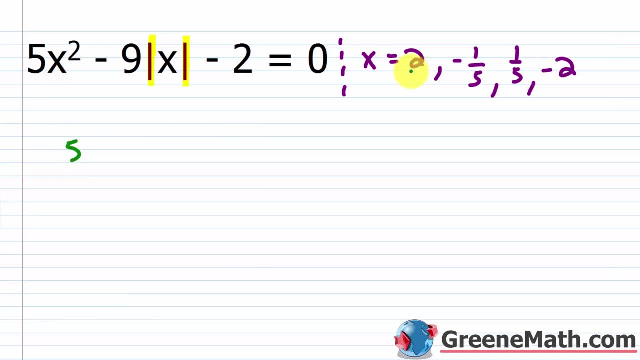 so we have five times for X. I'm going to start by plugging in a two, So you'd have two, then minus nine times the absolute value of two. right. plug in an N for X, then minus two, and this equals zero. Okay, so two squared is four, So you'd have five times four. 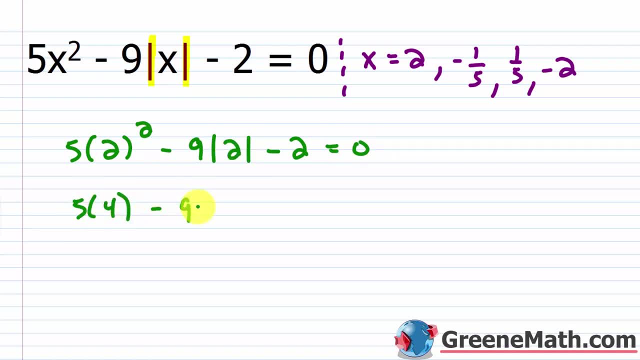 then minus nine times the absolute value of two. The absolute value of two is two, so nine times two, then minus two, and this equals zero. Five times four is 20, then minus nine times two is 18, then minus two, and this should equal zero. And this is going to work out right: 20 minus. 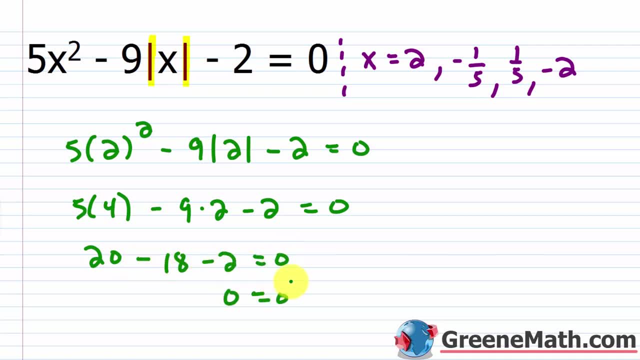 18 is two. two minus two is zero. So you get zero equals zero. so this guy checks itself out. now let's work on negative one-fifth now. so let's erase this and we'll do negative one-fifth. so i'm going to erase that and that i'm going to put negative. 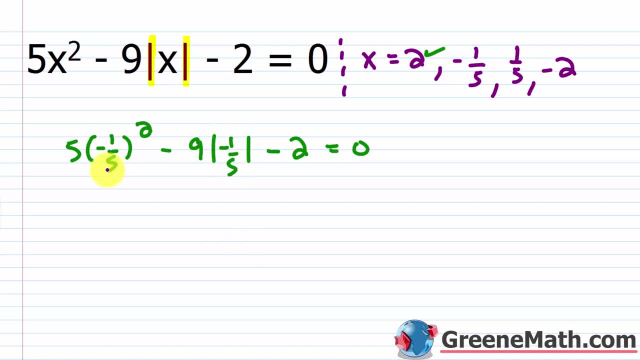 one-fifth in there. all right. so essentially, if i square negative one-fifth, i would get one twenty fifth. so i have five times that guy. then minus nine times the absolute value of negative one-fifth is one-fifth, and then minus two and this should equal zero. so this guy is going to cancel with. 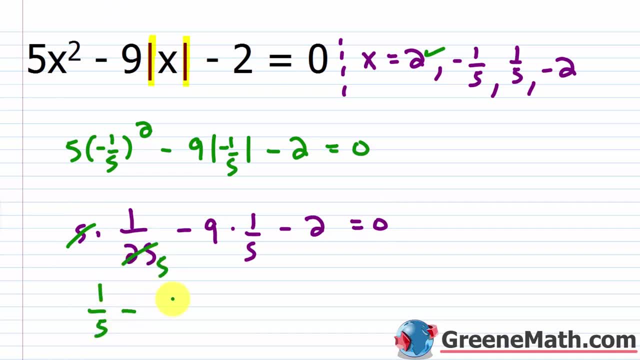 this guy give me a five, so you've got one-fifth minus nine-fifths. you can go ahead and do that real quick because they have a common denominator: one minus nine is negative eight, so that would be negative eight-fifths. so you have negative eight-fifths and then we're subtracting away. 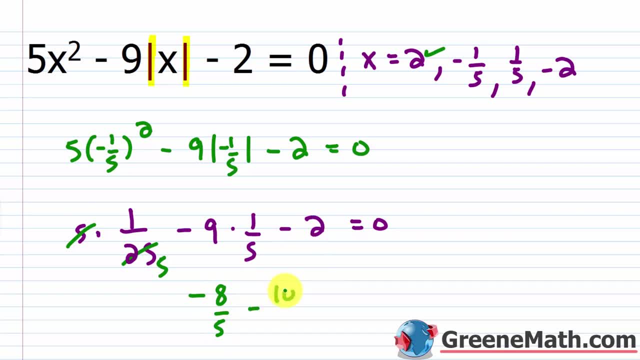 two. so i can go ahead and write that with the common denominator and say: minus ten over five, right, ten over five is two and this should equal zero, and obviously it doesn't right. if we do this, it would be negative eighteen-fifths, okay, negative eighteen-fifths, and that is not. 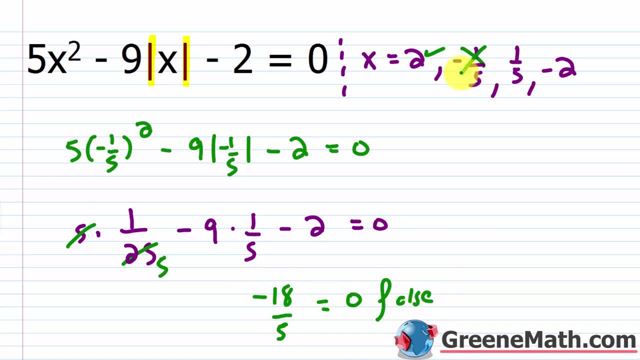 equal to zero, so that would be negative eighteen-fifths, and that is not equal to zero. this is false, so we're going to reject that solution. now i don't actually need to check one-fifth, because i'm going to get the same kind of result here. if i squared, one-fifth is the same. 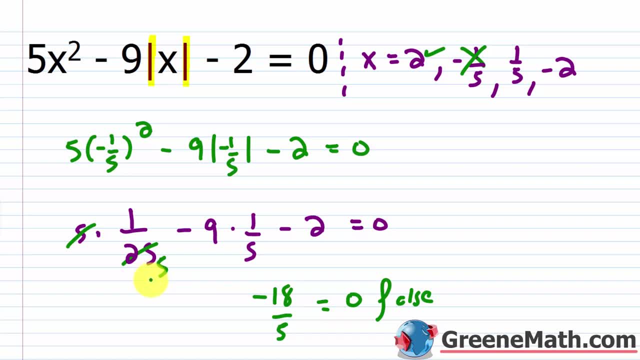 as squaring negative one-fifth. in either case, i'm going to get one twenty-fifth, if i take the absolute value of one-fifth is the same as taking the absolute value of negative one-fifth. so this would be the same and this would be the same, so you can go ahead and reject that as well. okay, so. 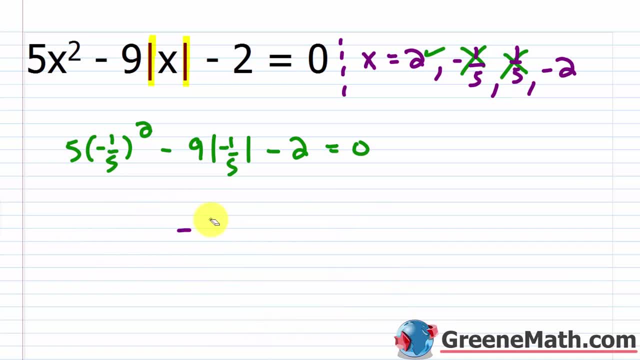 get rid of that, then the other guy that you're going to have was negative two. so let's go ahead and check that. but again, you know that's going to work, because two worked. you're going to end up with the same scenario, right? because negative two squared, or two squared each, give you four. so in each case, 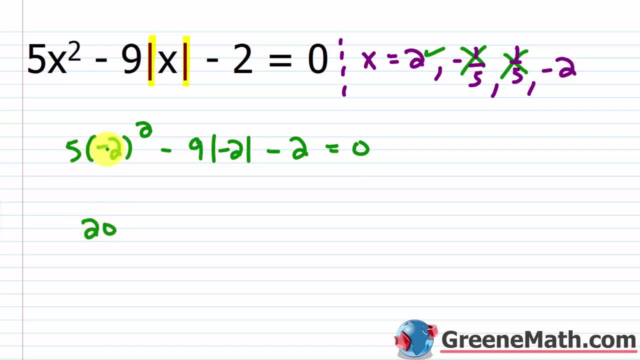 you're going to have twenty there, because five times four is twenty. then you're subtracting away nine times two in each case, because whether i put a negative two in there or positive two, when i take the absolute value of that i get two right either way. so nine times two is eighteen. 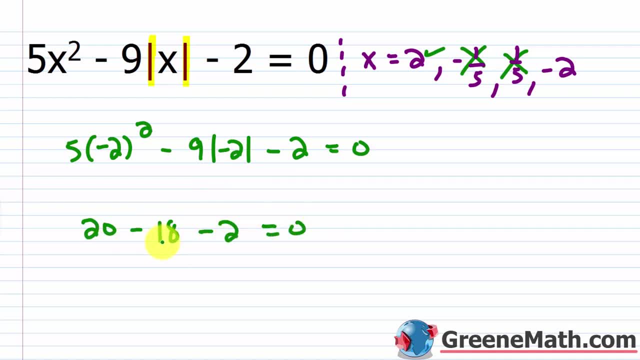 and then you've got minus two and this equals zero. again, twenty minus eighteen is two. two minus two is zero. so you get zero equals zero. so this does work out as well. so this gave us two solutions: x equals two or x equals negative two. so i can just erase those, just kind of tighten this down and say: 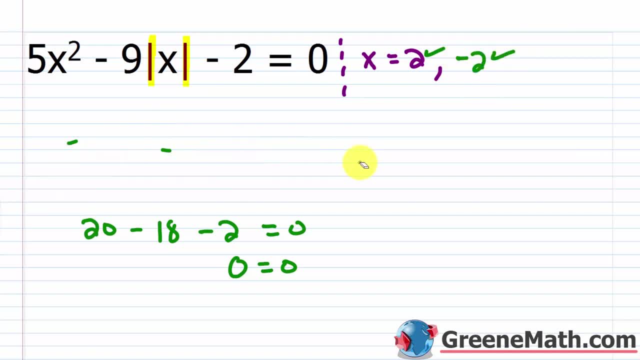 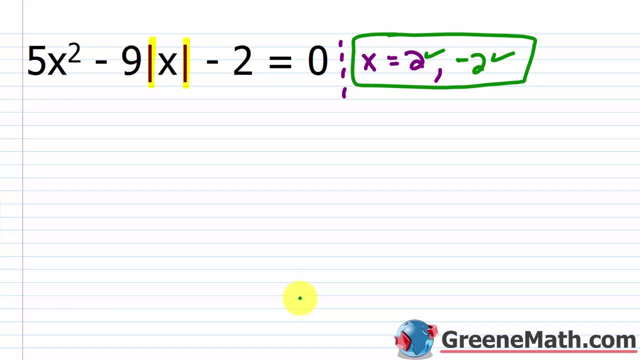 negative two there and now let's think about doing this in alternative way. so for this method, we're going to focus on using a substitution technique. we use substitution to solve things earlier in the course, so it shouldn't be something new for you. basically, what we're thinking about here is: 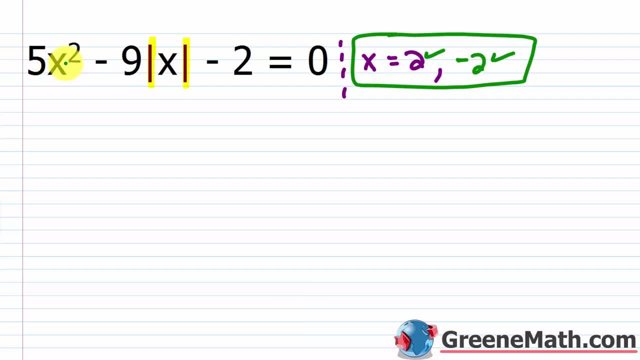 the fact that x squared is equal to zero. so we're going to focus on using a substitution technique where x squared is always non-negative and so is the absolute value of x squared, right? so if i think about x squared and i think about the absolute value of x being squared, this would produce the same thing, no matter what i plug in for x, right? if i plugged in, let's say, negative three, let's say i plugged in a negative three in each case, well, here negative three squared is nine, and here negative three. if i take the absolute value first, i get three. when i square that, i get nine as well, right? so what i can do here is i can just. 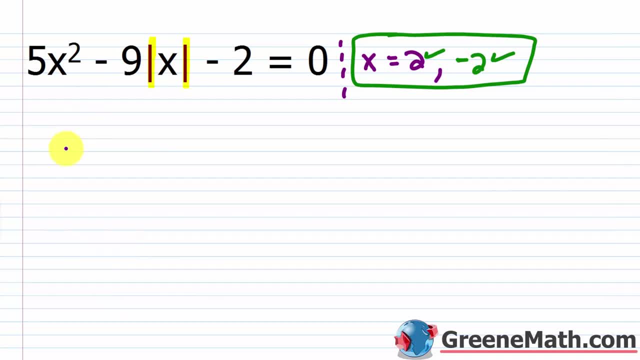 rewrite this and i can say that we're gonna have five times the absolute value of x- that's squared- then minus nine times the absolute value of x, then minus two, and this equals zero. okay, so now i have the absolute value of x here and i have the absolute value of x here, okay, so what i'm going? 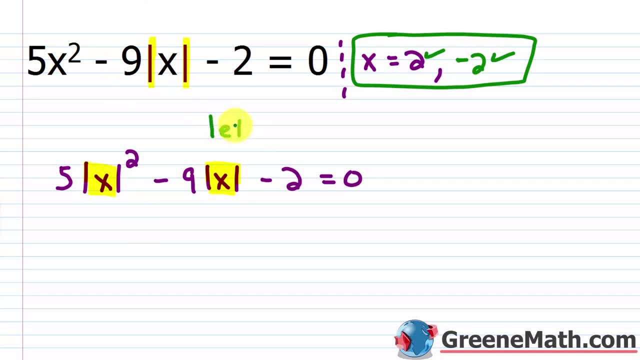 to do is just make a little substitution. so i'm going to let u be equal to the absolute value of x. okay, so now i'm going to replace the absolute value of x in each case with u, so i'm going to have that five u squared minus nine, u minus two is equal to zero. so this: 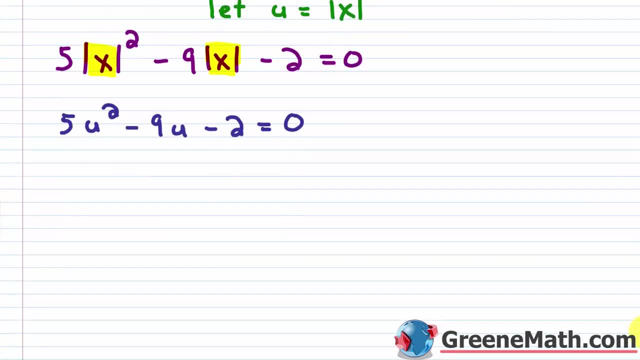 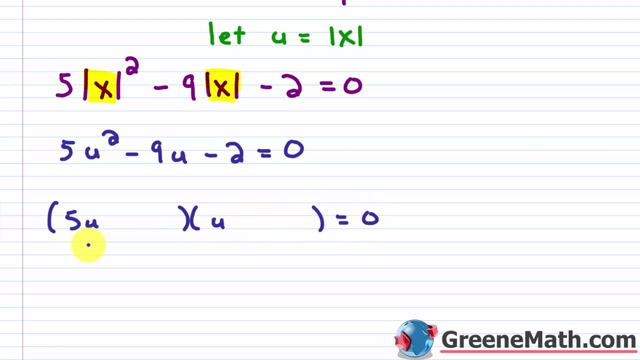 is something we can again solve using factoring. let me kind of scroll down for a minute. so i'm going to put a five u here and a u here. this equals zero and of course i need my outer and my inner to sum to negative nine u and my final to be negative two. okay, so we know we're going. 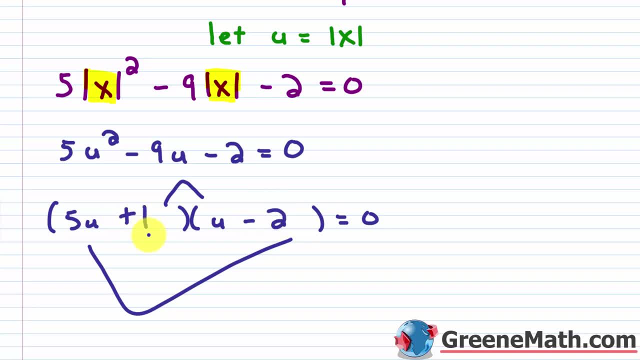 to do that with a negative two here and a positive one here. we saw that earlier. okay, so we know that five u times negative two would be negative 10 u and that one times u would be plus u. so this gives me my negative nine u and, of course, one times negative. 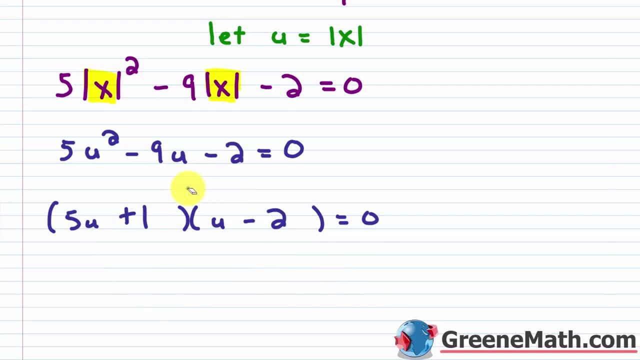 two is negative two. okay, so let's erase this and let's kind of solve this real fast. so i would set five? u plus one equal to zero. subtract one away from each side of the equation, you get five? u is equal to negative one. we're going to divide both sides by five and we're going to get that? u is. 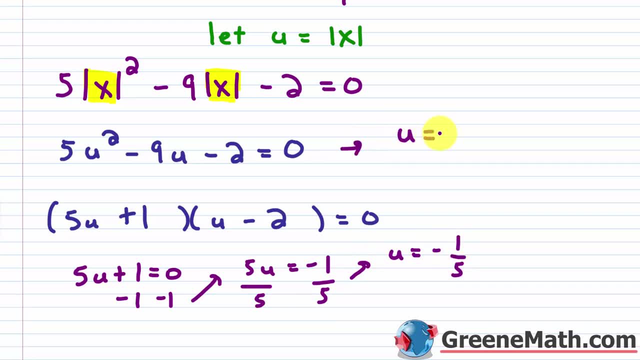 a negative one-fifth- okay, so let me write that over here. u is equal to negative one-fifth- okay, so let me erase this. i don't need that anymore. the other guy is really easy. you can solve that mentally. you have: u minus two equals zero, so u minus two equals zero. add two to both sides of. 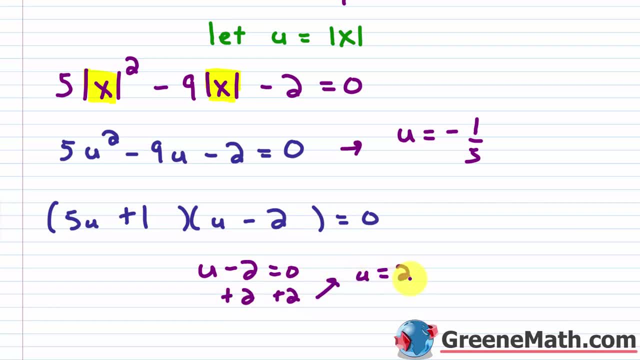 the equation and we get u is equal to two. okay, so let's put a two there. so you might be thinking you didn't get all the same solutions that you got using the previous method. well, we did. we just have to go back and substitute again. so let me erase all of this. we're going to get two and two. 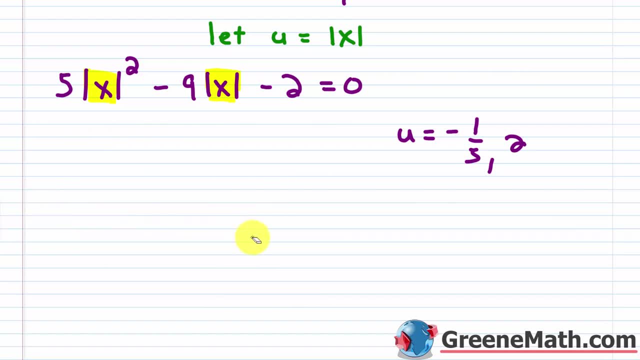 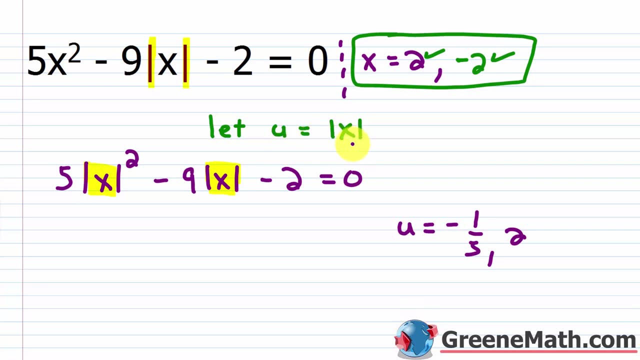 don't really need it anymore, okay, and we're just going to scroll up, we're going to think about what u means. so i told you that u is equal to the absolute value of x. so if u equals negative one-fifth, i can say the absolute value of x, because that's, u is equal to negative one-fifth. 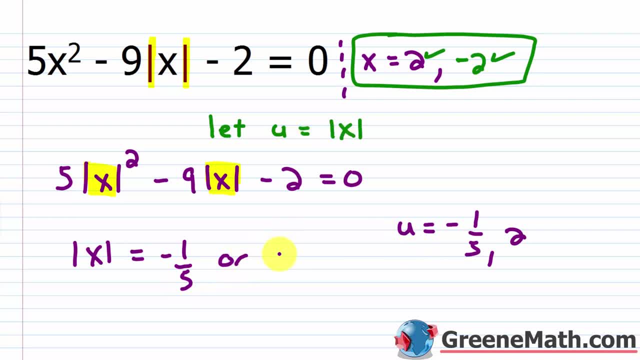 okay, then i can also say that the absolute value of x- because again that's u- is equal to two. now, here's where we save some time. we can throw this guy out right away. right, throw this out, because the absolute value of x cannot be equal to a negative value. okay, if the absolute value operation. 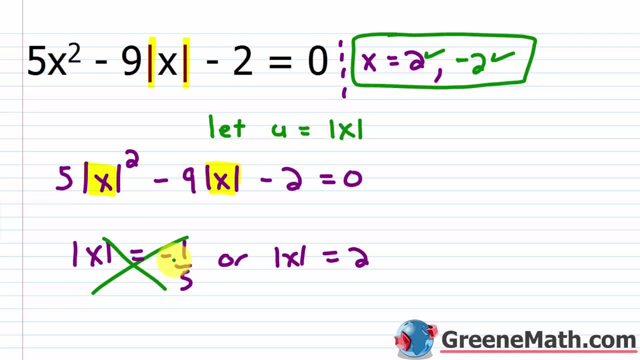 is isolated on one side, you can't have a negative on the other. okay, the absolute value operation will always give you a non-negative answer. so that doesn't work. for this one, the absolute value of x equals two gives me two solutions. right, it could be true that x is two, or x is negative two which? 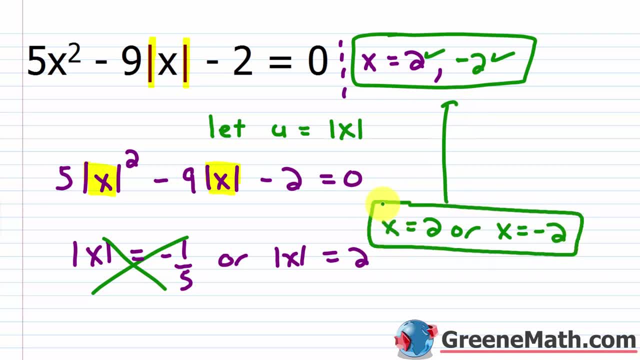 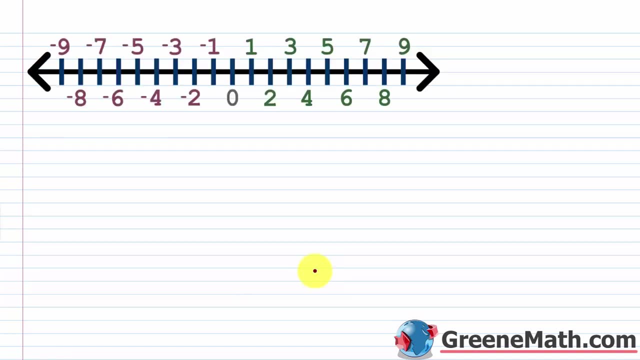 is exactly what we found with our other method. this one, i think, is just a little bit quicker because it leads to you rejecting kind of the extraneous solutions right away and you're just left with the good ones. in this lesson we want to review solving absolute value inequalities. so in the last lesson we talked about 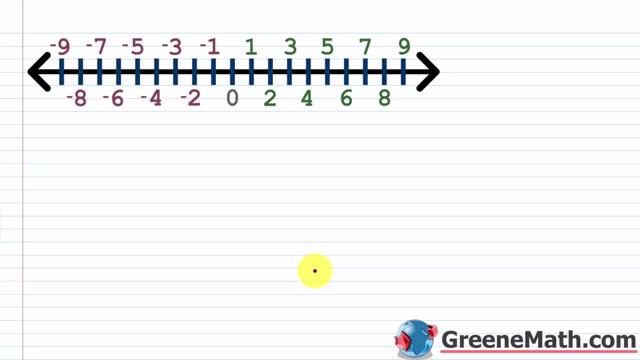 solving absolute value equations. in this lesson we're just going to go one step further and talk about solving absolute value inequalities. now, before we kind of jump into some problems, let's just take a moment here and think about absolute value as a concept. so if i asked you for the 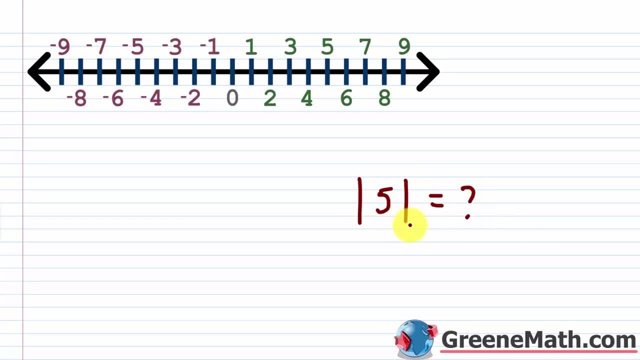 number five. what am i asking you for? remember, the absolute value of a number is the distance from zero to that number on the number line. so if i want to know the absolute value of five, i'm asking: how far away is five from zero on the number line? we know, with any positive number it's just the. 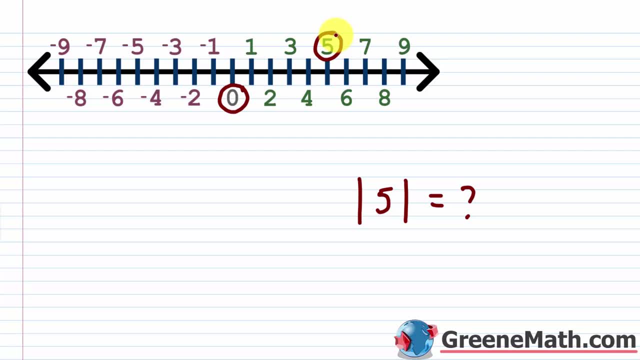 number right. so five would be five units away from zero and we can show that it's one, two, three, four, five, right. and it doesn't matter that i started at zero and went to five. i could start at five and go to zero. we're not measuring anything to do with direction, we're measuring the distance. okay, that's. 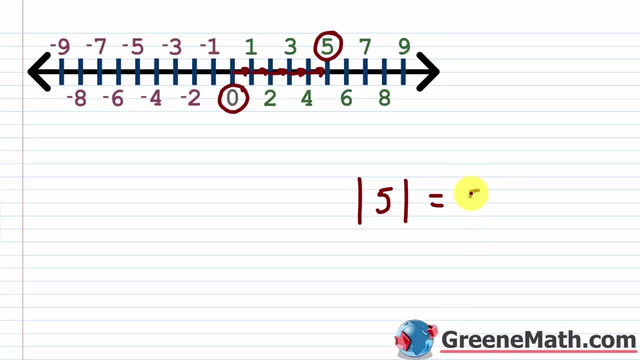 what we're focused on. so the absolute value of five would just be five. the absolute value of, again any positive number is just the number. so if i wanted the absolute value of, let's say, eight, it's just eight. if i wanted the absolute value of one million, it's just one million, right so? 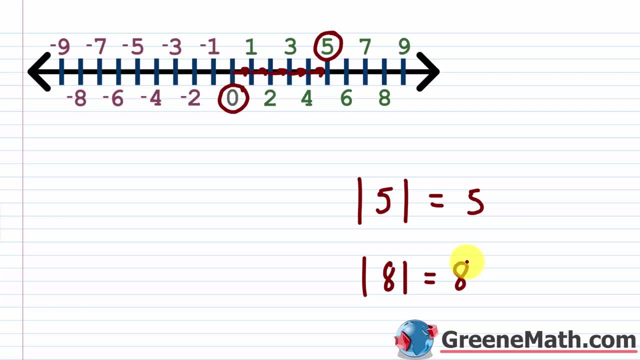 on and so forth. now, when we work with absolute value, we've got to be aware of the restrictions or things that happen when we take the absolute value of a number. if i take the absolute value of a negative, i end up with a positive right. so the absolute value of 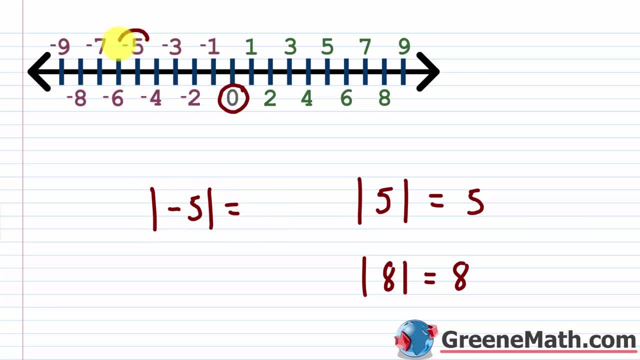 negative five would be one. let's go to negative five on the number line and i'm also five units away from zero. so i would go one, two, three, four, five units to get to zero. so this answer here is also five, right. so i took the absolute value of something that's negative and i got a positive. 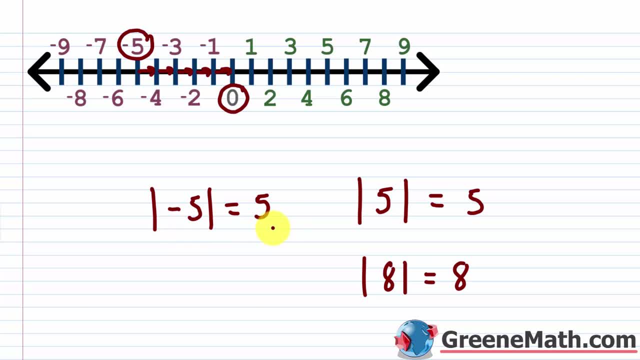 because i'm measuring four minutes. i could find five minutes, four minutes of negative here, and i did that. so, okay, it's just one. i'm in Smooth state and i'm measuring what's going to happen. so what you're looking at here is about taking a negative mes fingertip enough. 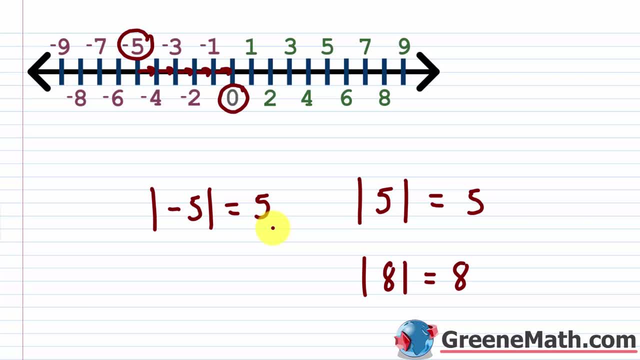 and i've got it measured now here. let's say: this is a hundred, but i don't want to do this right. so right now it's going. that's what's going on, and what do i do to order that? so zero as a result. Okay, If I took the absolute value of zero, I would get zero, And that's. 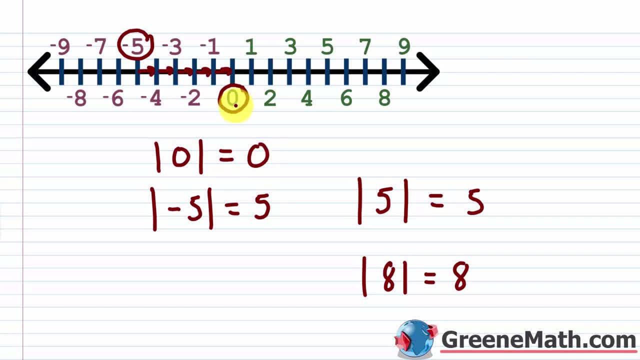 because zero is zero units away from itself on the number one. So the main thing to understand here is that the absolute value operation is always going to give you a result that is non negative, So zero or positive. Okay, Very important to understand that because it will come up later. 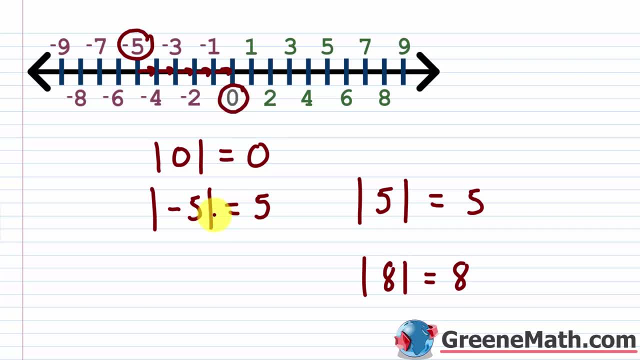 on in the lesson. Now we also want to think about one other thing here. I want you to notice that five and negative five have the same absolute value, right? If I did eight and negative eight, those would also have the same absolute value. Okay, So numbers like these, five and negative- 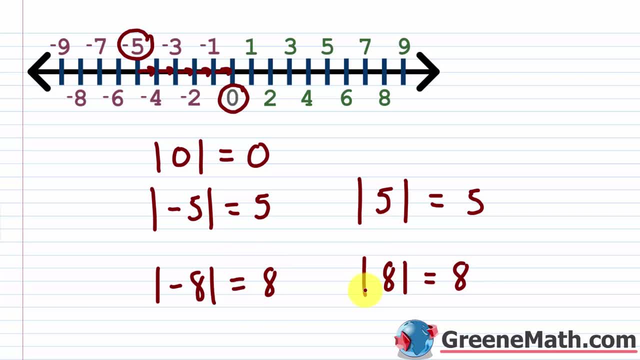 five or eight. negative eight or 2 million and negative 2 million. these are known as opposites. Okay, They're going to have the same absolute value. Okay, Cause they're the same distance away from zero, but they lie on opposite sides of the number One's: on the negative side. 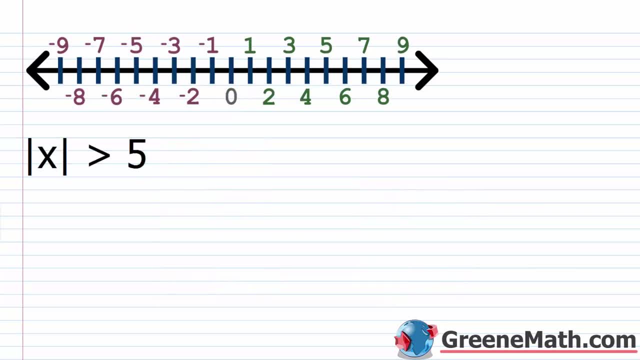 one's on the positive side, So we call them opposites, All right. So now that we understand the constant value operation, we're going to go ahead and look at the opposite side of the concept of absolute value. Let's think a little bit about how we can solve an absolute value. 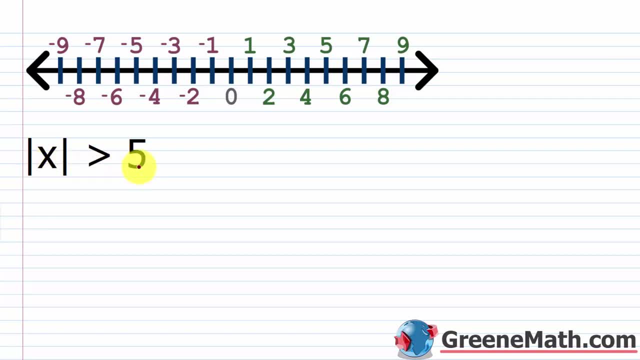 inequality. We're just going to start with some very simple examples here, and then we'll get into some more challenging material. So we're going to start with. the absolute value of X is greater than five. So, using our understanding of absolute value, what am I asking for? What can I? 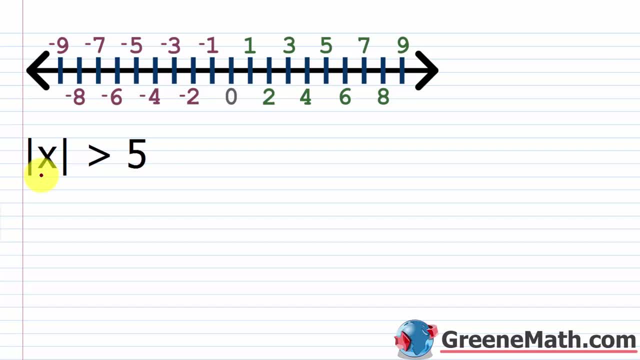 plug in for X here. that would satisfy the inequality. Well, remember, if I'm taking the absolute value of something, I want to know the distance from that to zero on the number line. The absolute value of X is greater than five is saying that X can be any value. whose distance? 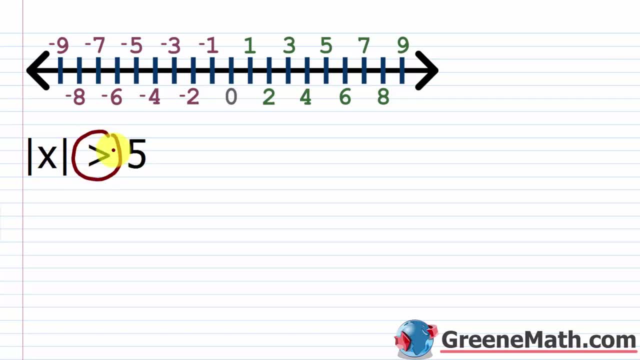 from zero is greater than five. So to find this, I could start at zero and I could go five units to the right And I could shade from five on, but five wouldn't be included because it's got to be strictly greater than five. So I'll put a parenthesis at five or you can use an open. 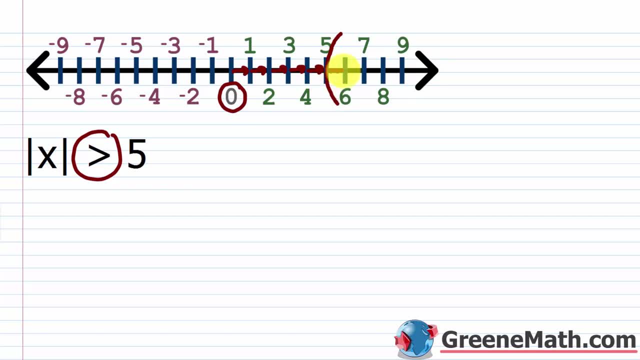 circle if you want, if that's what you're doing in your class, And I want to shade everything to the right here because that would be part of my solution, right? So if I plugged in a six there, absolute value of six is six. six would be greater than five, That's true, Okay. 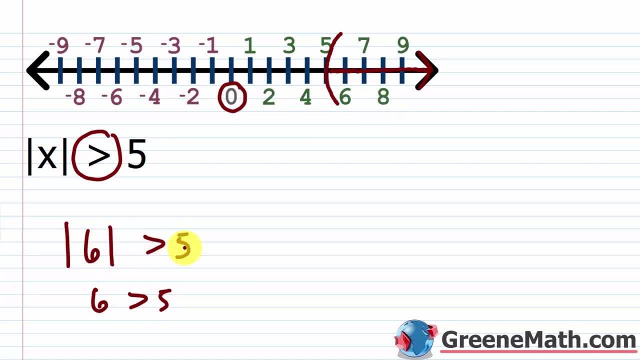 so that would work If I plugged in an eight. the absolute value of eight is eight. eight is greater than five, That's true. So any number larger than five would work. That's pretty obvious. Everybody gets that. But also I've got to look in the other direction of 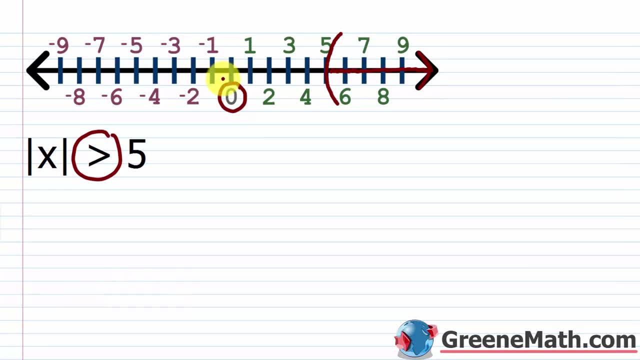 zero because again, when we think about absolute value, it's a distance, So I can also travel a little to the left. I can go one, two, three, four, five units here, So anything less than negative five would work as well. Negative five does not work, So I'm going to put a parenthesis. 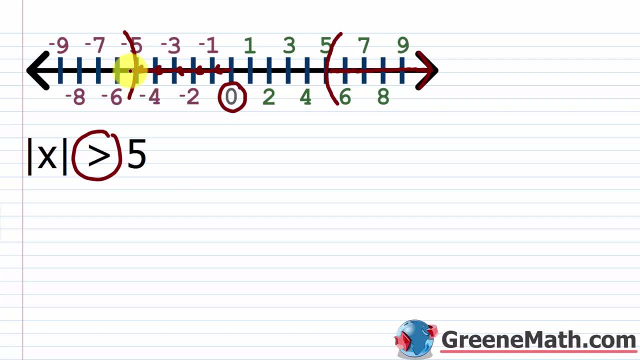 there, And again you could use an open circle, if that's what you're doing, And then I would shade everything to the left here And then we could try some numbers out in this range. Let's say we picked negative seven, So we plug in a negative seven for X, The absolute value of 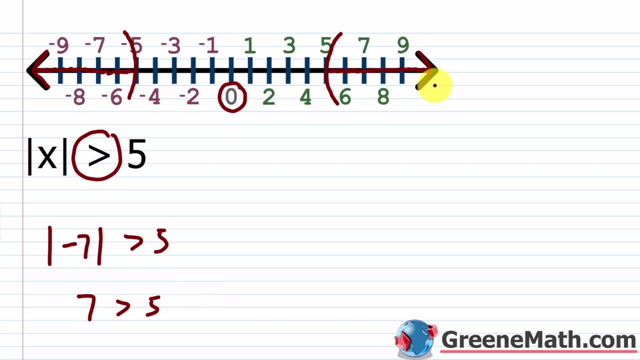 negative. seven is seven. Seven is greater than five. That's true. So what we have here for our solution is a compound inequality with or. So we can basically say that our solution is that X is greater than five. or remember our keyword: or X is less than. 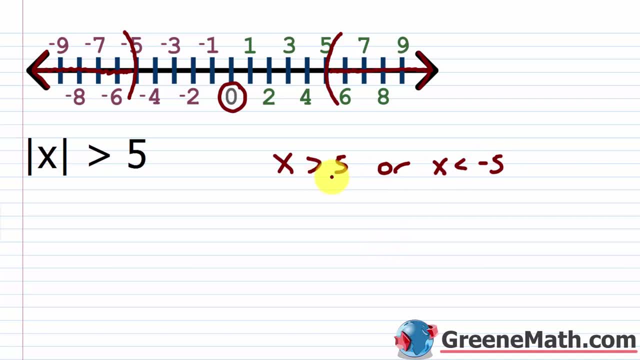 negative five. So we could also notate this in interval notation. It would be the union of the two solution sets. So I would have from negative infinity out to, but not including negative five, And then the union with you have anything larger than five. So 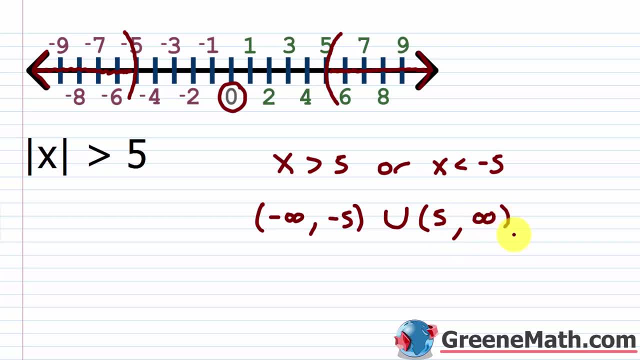 a parenthesis next to five, again out to positive infinity. Okay, Notice how I use a parenthesis with each, with negative five and five because they're not included. All right, So let's look at a general rule that we can follow when we're solving these guys, And this first rule. 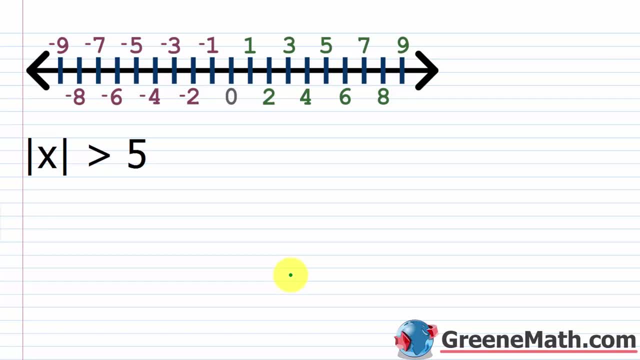 I'm going to give you is just the simplest case scenario. We'll look at a different rule in a minute that will cover more challenging problems. So we saw that the absolute value of X is greater than five led to X is greater than five or X is less than negative five. So in general, 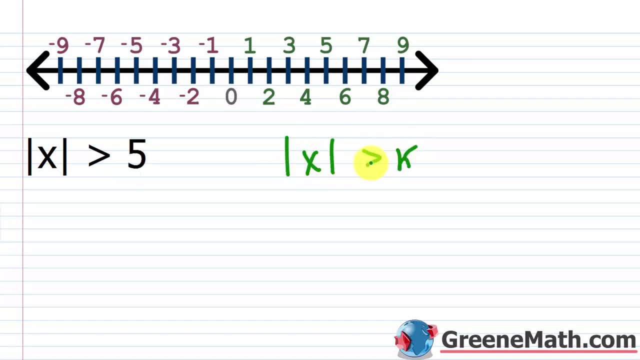 the absolute value of X is greater than K, So this is a greater than case, where we say that K is greater than zero. Okay, This has to be the case. to use this rule, Then what's going to happen is we set up a compound inequality with four, So X can be greater than K, or you could say the negative of. 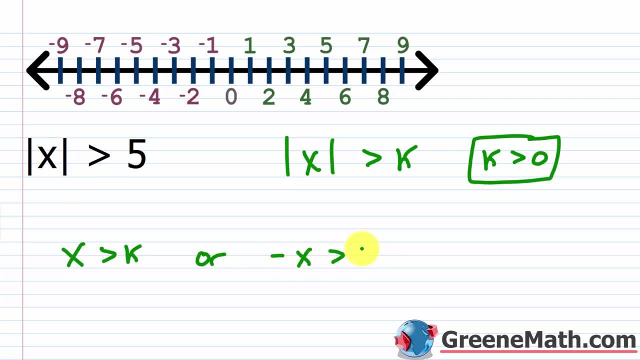 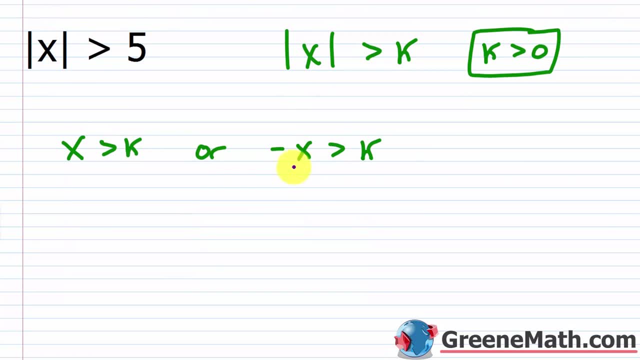 X, because the absolute value will make that positive is greater than K. Now what happens here? when you see this in your textbook, what they do is they divide both sides by negative one, so that it's solved for X. And so you're going. 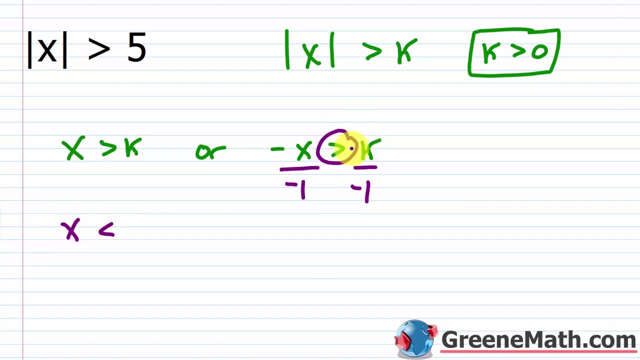 to get that X is less than. remember, if you divide by a negative you've got to flip the direction of the inequality symbol. So a greater than becomes a less than, and then K over negative one is just negative K. So what we see is that X can be greater than K or X can be less than negative. 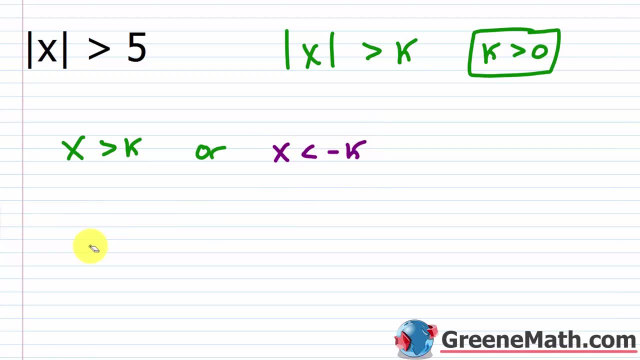 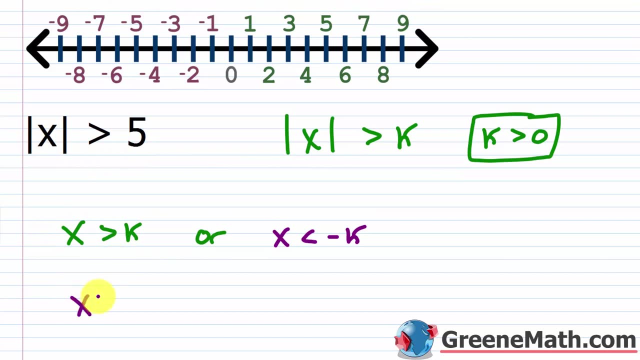 K. Okay. So this is what you're going to see And again, when we worked with this first example here, it looks just like it. let's say we say the absolute value of X is greater than K, but let's say we divide it over these two side by a negative thing that you get an problems is that. 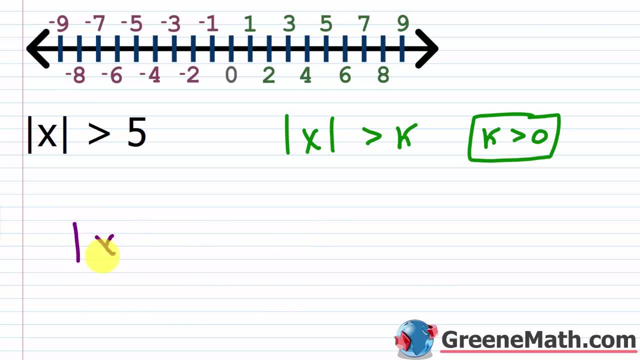 the absolute value e of X is greater than five. We got just this: x was greater than five or X was less than negative five. Okay, So that's where that comes from. So if I gave you a problem like, let's say, the absolute value e of X is greater than 14.. 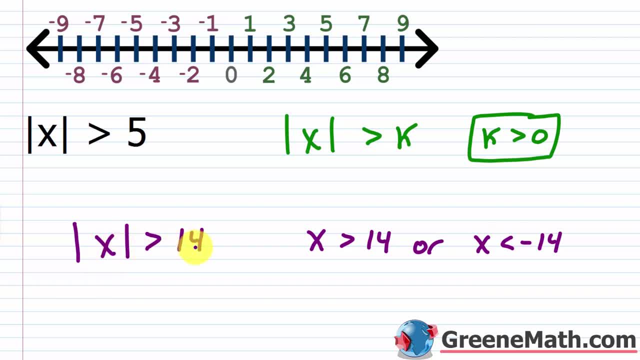 Well then, you can very quickly say that X is greater than 14,, X is greater than 14.. The second scenario- you just think about it like this- Flip the direction of the inequality symbol, so my greater than becomes less than. 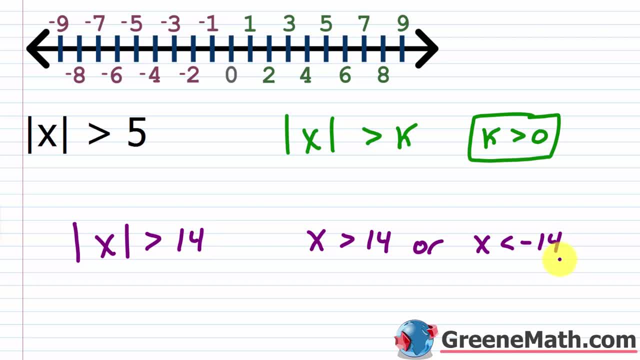 and then change the sign of the number out here. So from 14, I get negative 14.. So if you could just remember that you flip the sign and then make the number negative, you're good to go. okay, That's all you need to remember. 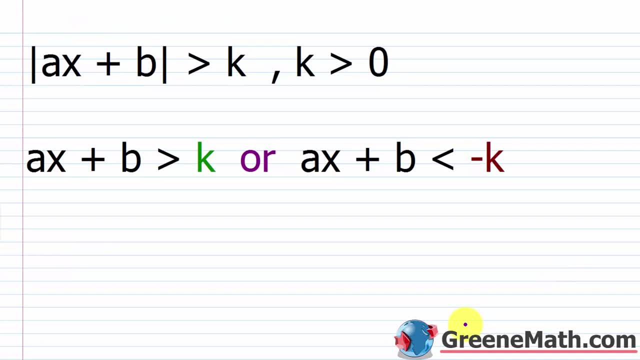 So let's look at our rule when it's more complicated, So when we get more challenging problems, we're not gonna always have the absolute value operation isolated at the start, So we've gotta get it in this format of the absolute value operation on one side. 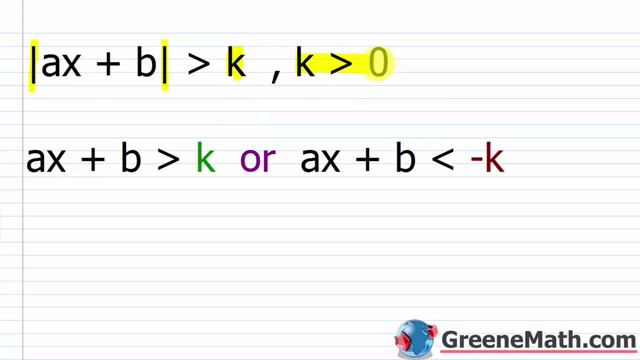 and a number on the other. okay, Notice how I've said that k is greater than zero. Again, if it's zero or less than that, we'll talk about those special cases at the end of the lesson. But I wanna isolate this to where the absolute value. 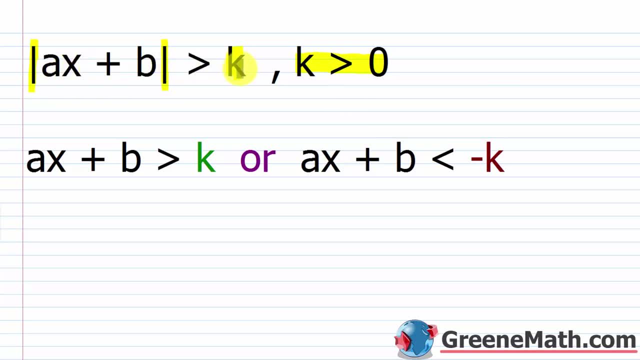 of some expression: ax plus b is greater than k. So this is gonna set up to this expression: ax plus b is greater than k, or ax plus b is less than the negative of k. all right, So same process For the first one. I just remove the absolute value bars. 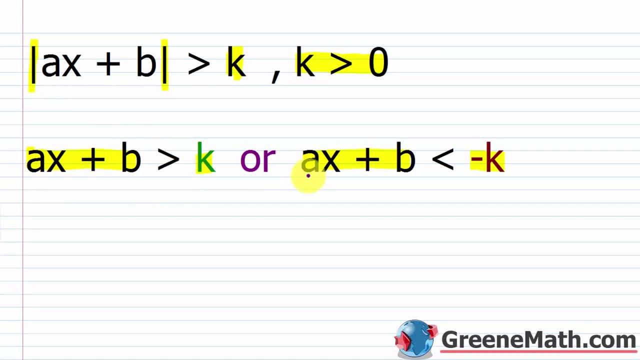 I copy what's there. it's very simple. For the second one, I remove the absolute value bar, so the expression doesn't change. I flip the direction of the inequality symbol, so now it's a less than, and then I make that number negative. 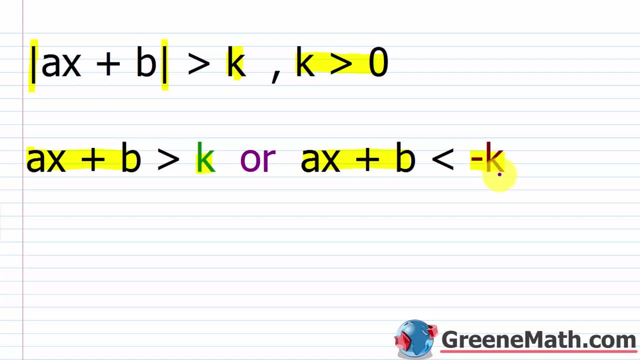 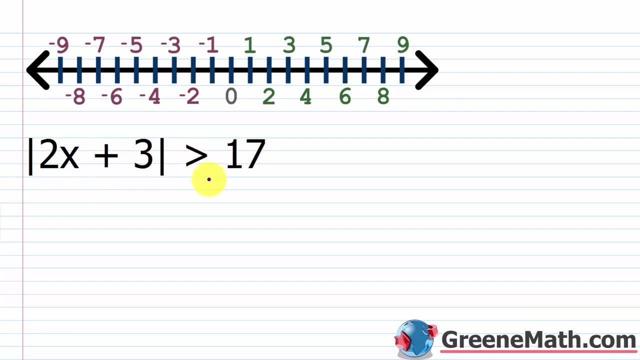 So instead of just k, it becomes negative k. all right, So let's look at an example. All right, so for this one we have, the absolute value of two x plus three is greater than 17.. So the first case is, I just remove the absolute value bars. 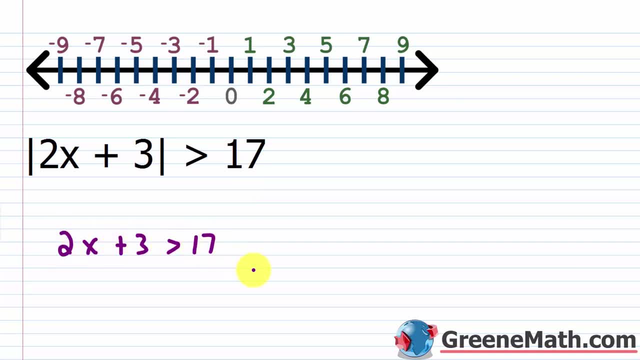 So I'll have: two x plus three is greater than 17.. Then, or my second case, I remove the absolute value bars, so two x plus three, I flip the direction of the inequality symbol, so it's a less than. 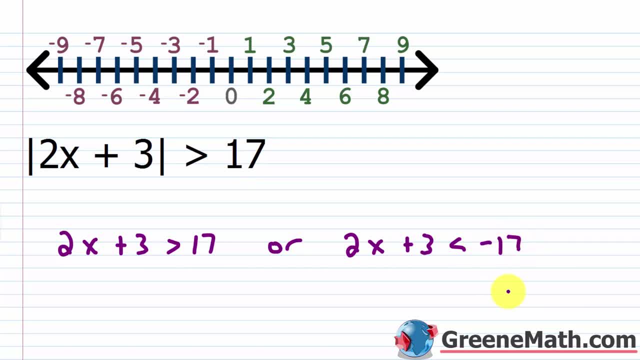 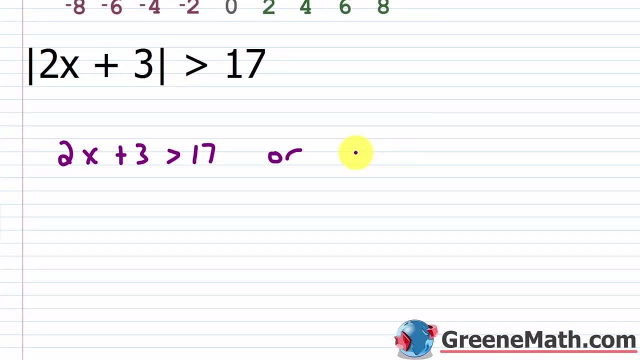 and then I make this number negative. So it's gonna be a negative 17,. okay, And if you have trouble remembering that, you can always just make the expression over here. You could always say it's the negative of this guy. So the negative of two x plus three is greater than 17.. 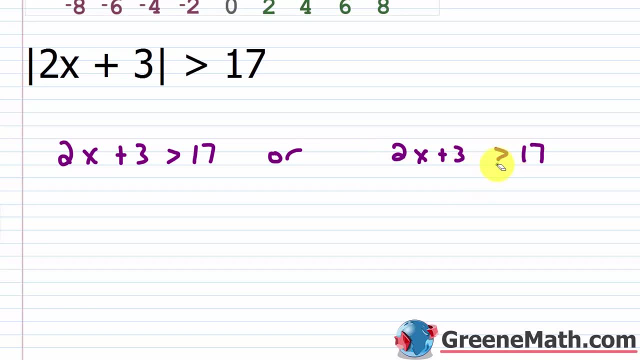 When you divide both sides by negative one, you're gonna get it into that format, So this would flip and this becomes negative. okay, So that's another way you can kind of remember. All right, so let's quickly solve these two inequalities. 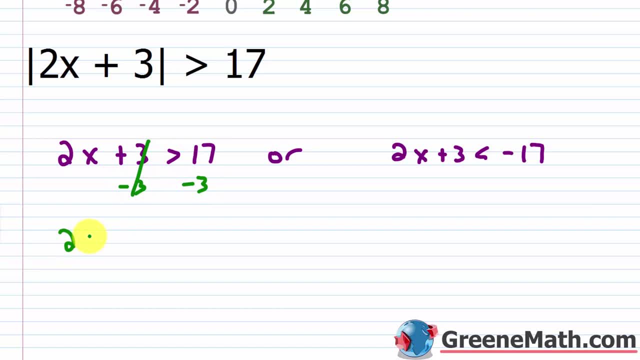 For this one. I would just subtract three away from each side. I would get two. x is greater than 17 minus three is 14.. Divide both sides of the inequality by two: I get x is greater than seven. Okay, over here, if I subtract three away. 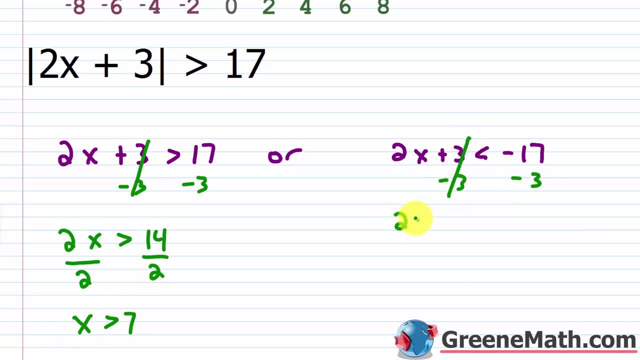 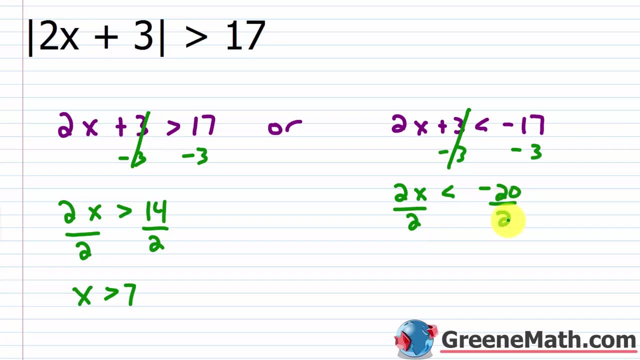 from each side of the inequality that cancels. I get two. x is less than 17.. I get x is less than negative. 17 minus three is negative 20.. Divide both sides by two and we're gonna get that x is less than negative 10, okay. 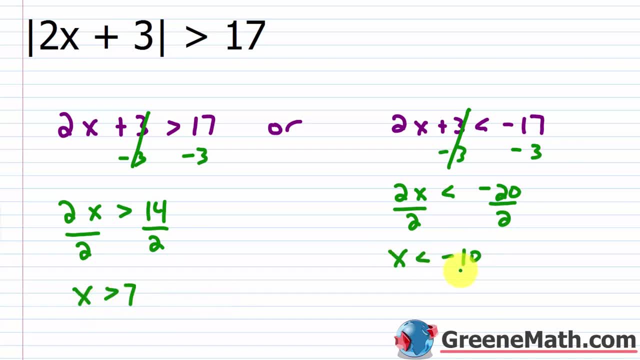 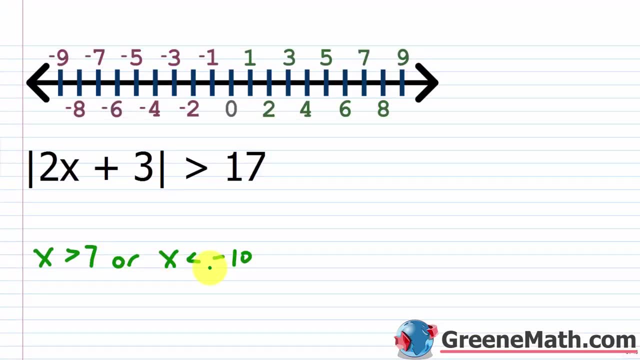 So we got that x is greater than seven or x is less than negative 10. So let's erase this, Okay. so let me put my or here, So you could write it like this as your solution: You can of course do interval notation: 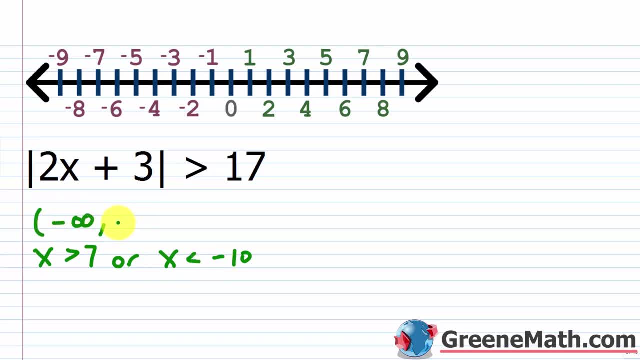 So from a negative infinity up to, but not including negative 10.. So it's the union with you've got not including seven, and then up to positive infinity, okay, So negative 10 is not included. You've got a parenthesis there. 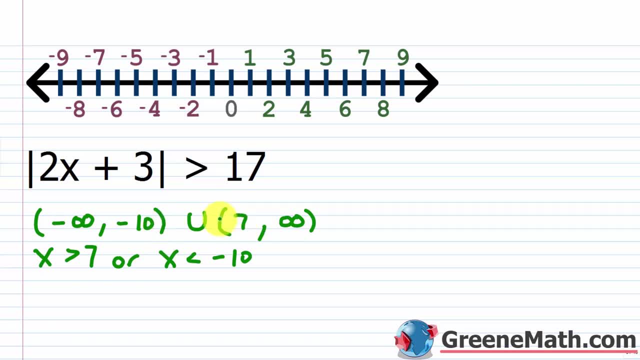 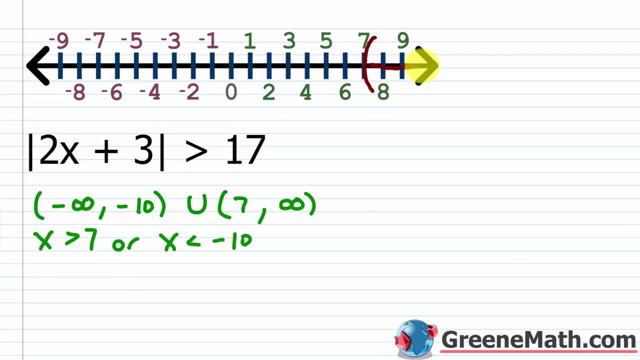 Seven is not included. You've got a parenthesis there. Now, graphically on our number line, we can put a parenthesis at seven and we can shade everything to the right. Okay, all that, And then, in terms of x being less than negative, 10,. 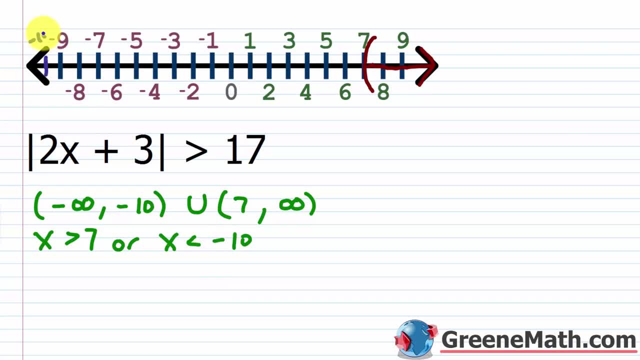 we don't have a notch for negative 10, but we can just make one real quick. So we'll say this is negative 10.. And let me make that a little bit better. And then I'm just gonna put a parenthesis there. 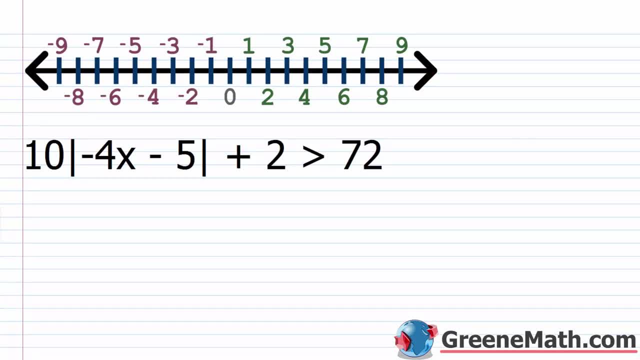 and I'm gonna shade everything to the left. All right, let's take a look at another one. So suppose we have 10 times the absolute value of negative. four x minus five plus two is greater than 72. So again, the idea here is to isolate. 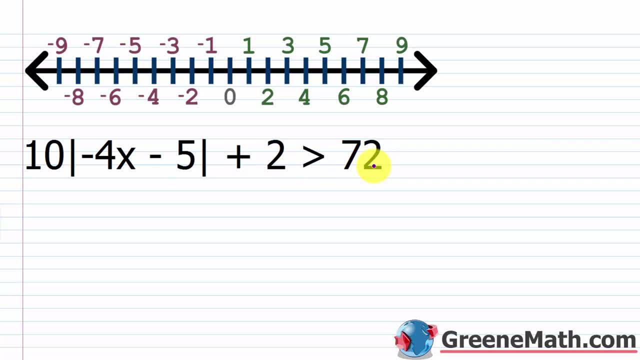 the absolute value operation. on one side, have a number on the other, So what I'm gonna do is I'm just gonna subtract two away from each side of the inequality to start. That cancels. You've got 10 times the absolute value. 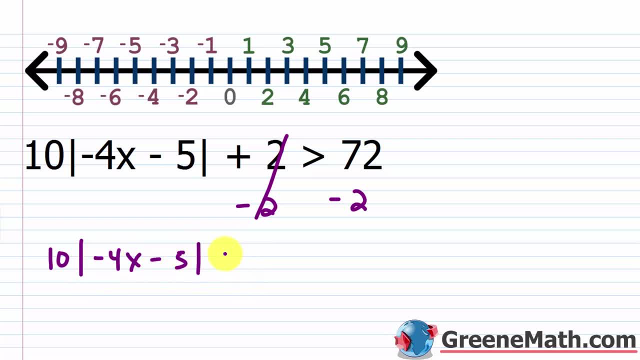 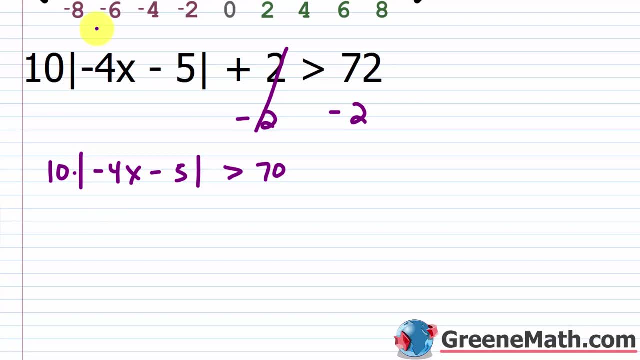 of negative four x minus five, And this is gonna be greater than 72 minus two is seven. So now, since 10 is multiplying this absolute value operation, I can just divide both sides of the inequality by 10.. So that cancels. 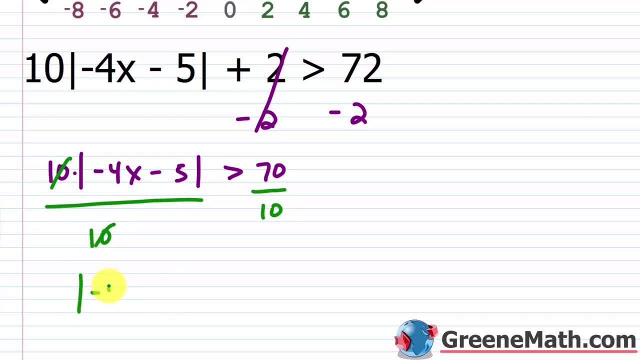 Now I've isolated the absolute value operation, I've got the absolute value of negative. four x minus five is gonna be greater than 70 over 10 is seven. Okay, so let me erase this. All right, so we know our scenario here, with a greater than. 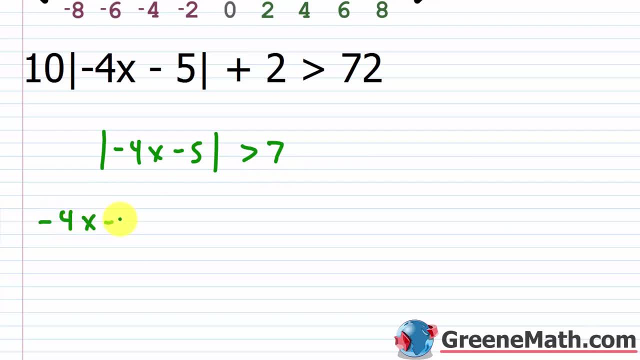 We wanna remove the absolute value bars, So negative four x minus five is greater than seven. Then, or we wanna remove the absolute value bars, So negative four x minus five. We wanna flip the direction of the inequality symbol, So this is less than. 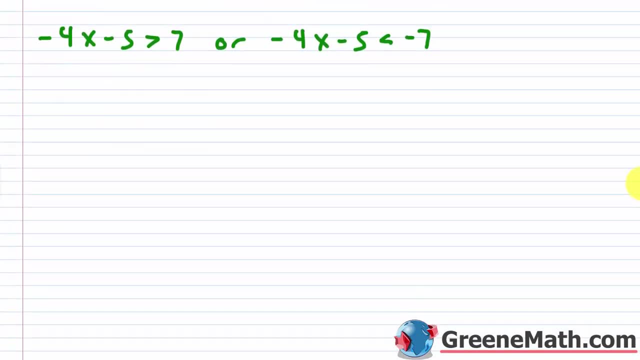 We wanna make this negative, So this is negative seven. Okay, so let's solve our compound inequality. Let's add five to each side of the inequality That cancels. You get that negative four. x is greater than 12.. We divide both sides by negative four. 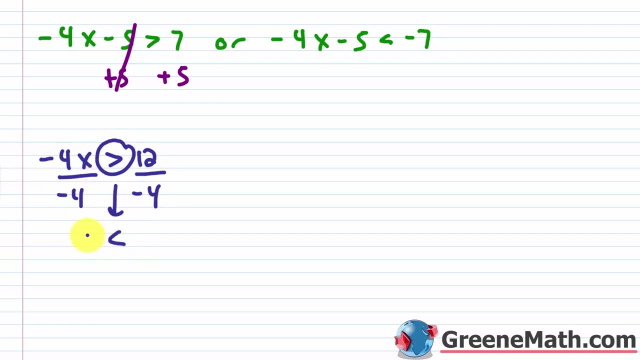 Remember this has the flip: We divide it by a negative, So this is a less than now. So you've got x is less than 12 over negative. four is negative three Over here if I add five to each side of the inequality. 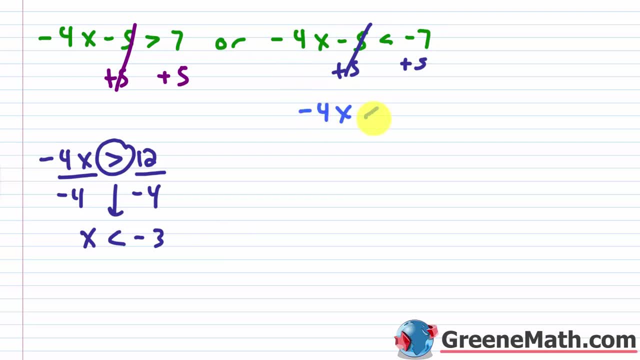 that cancels, You're gonna get negative four. x is less than negative. seven plus five is going to be negative two. We divide both sides by negative four. Again, if I divide by a negative, I've gotta flip that guy. So this becomes a greater than. 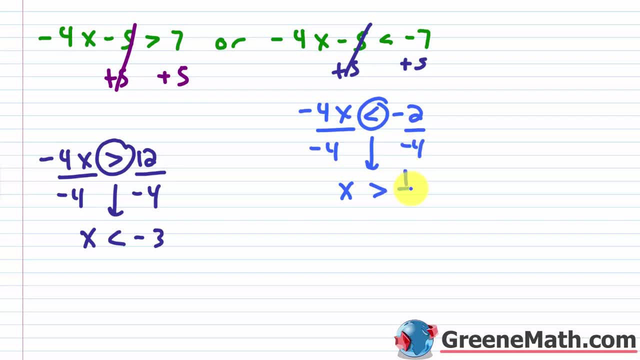 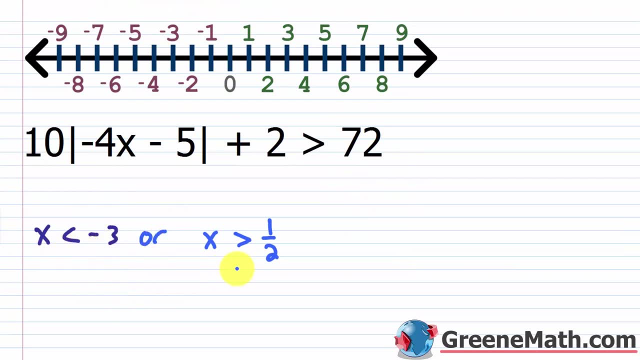 So we have: x is greater than Negative, two over negative, four is positive 1 1⁄2.. All right, let's erase everything So we can write our solution as x is less than negative three or x is greater than 1 1⁄2. 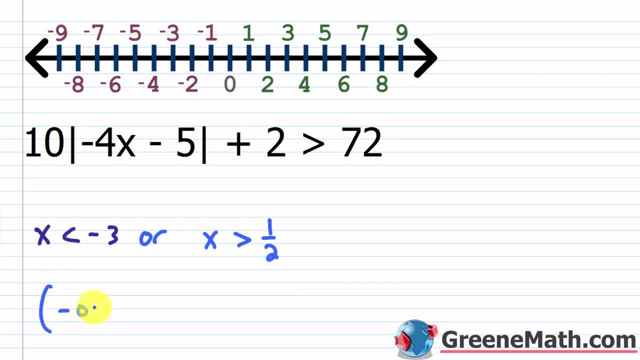 Again an interval notation. You're coming from negative infinity up to, but not including negative three. So the union with you don't include 1 1⁄2, but out to positive infinity, okay. So again, negative three and 1 1⁄2 are not included. 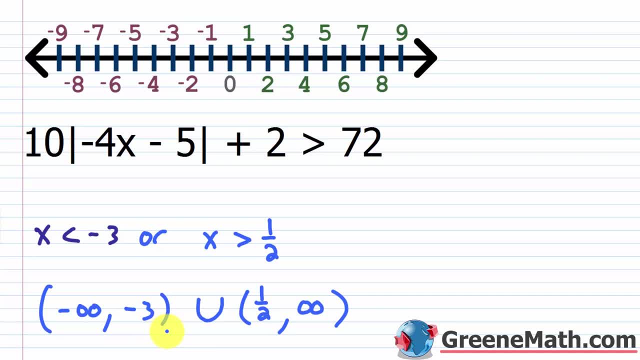 You have a parenthesis next to each. So now, graphically at negative three, I'd put a parenthesis face down, I'd put a parenthesis facing to the left And I would just wanna shade everything going to the left here. So all of that. 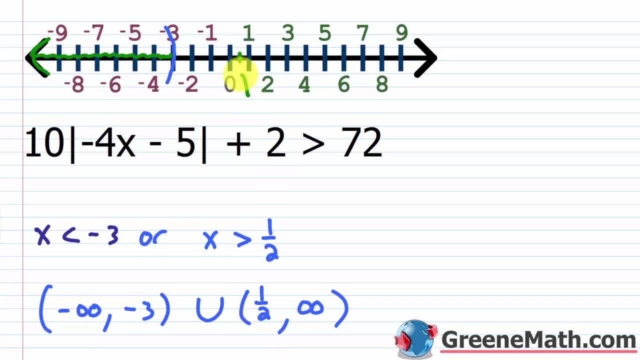 And then at 1 1⁄2, which would be about right here. let's say I'm gonna say that's 1 1⁄2.. I'm gonna go ahead and put a parenthesis there. Let's put a parenthesis there. 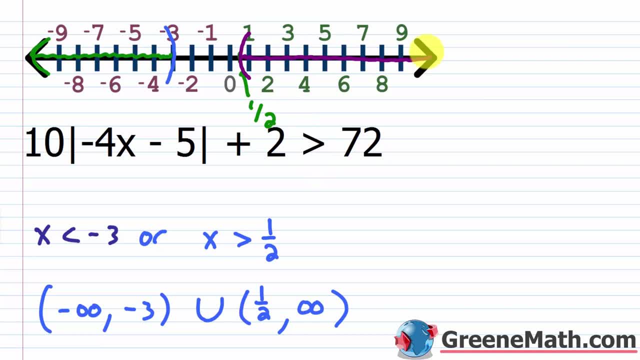 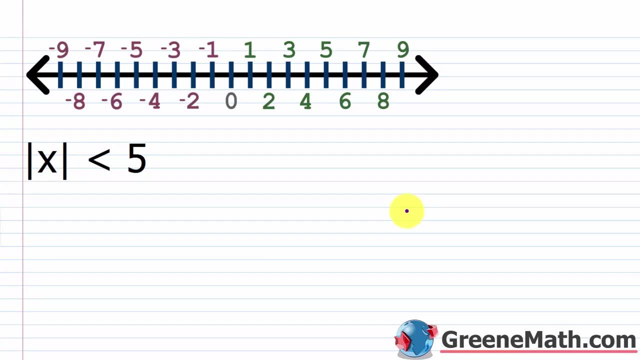 And again, let's just shade everything to the right. Okay, so that's my solution: region, All right. now let's talk about the other scenario, which is when we have a less than So. if I had, the absolute value of x is less than negative three. 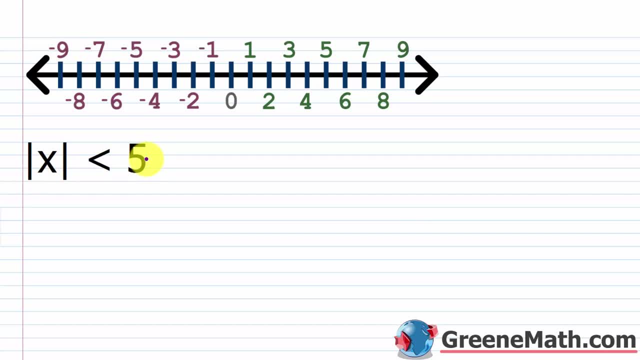 x is less than five. I'm gonna follow the same procedure, but I'm gonna use an and compound inequality. So in other words, I'm gonna remove the absolute value bars, So I'm gonna say x is less than five. Then I'm gonna say and: 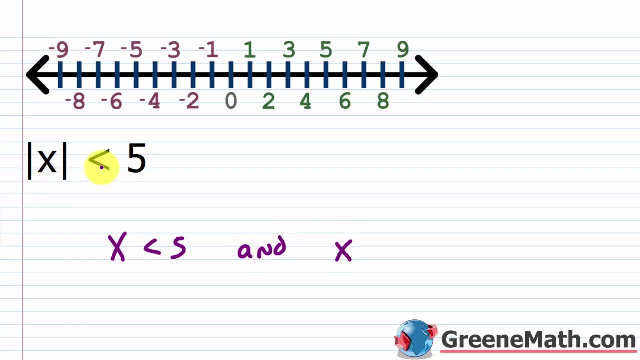 Then the next one: I'm gonna remove the absolute value bar, So I'm gonna have x. I'm gonna flip the direction of the inequality symbol, So this is greater than I'm gonna make the number negative. So this is a negative five. 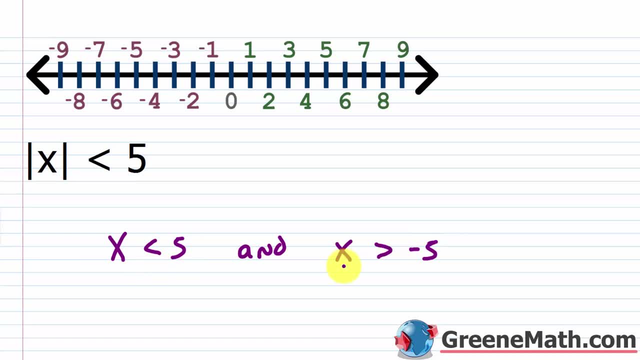 So it's the exact same process, but we're using an, and now okay, Because we're gonna have a between. So x will be between negative five and five. You could really write this as a three-part inequality and say that negative five is less than x. 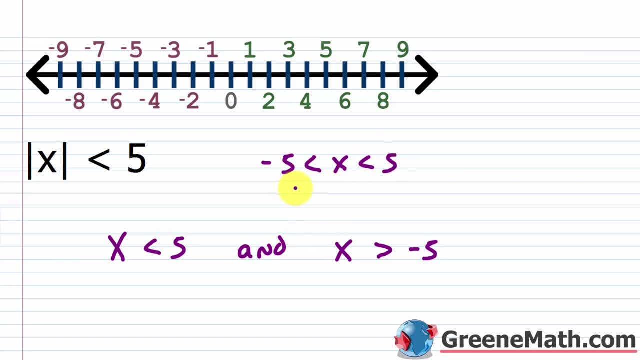 which is less than five. Or you could read that as x is greater than negative five and less than five. Now, conceptually, why does this make sense? I'm asking for all the numbers whose absolute value or whose distance from zero is less than five. 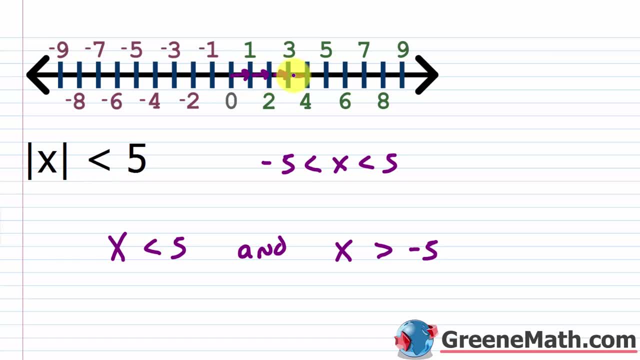 Again, if I started at zero and I went five units to the right, I couldn't be five because it's gotta be less than five. So I'd put a parenthesis there, facing to the left, If I started at zero and went the other way. 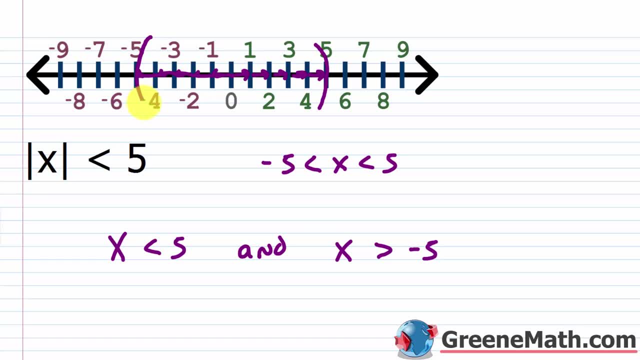 again, I'd go five units. It couldn't be negative five, but it could be anything greater there. So it would have to be between negative five and five on the number line. Those are the only values that would satisfy this If I plugged in a negative two. 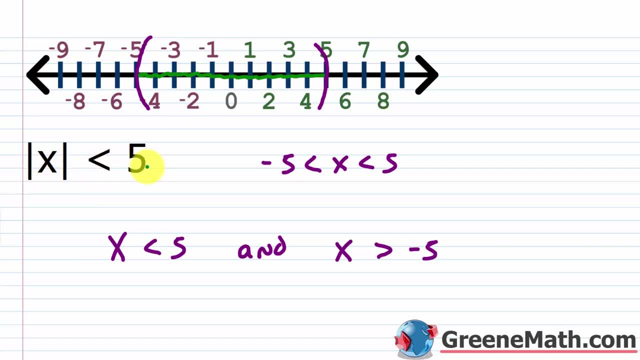 the absolute value of negative two is two. Two is less than five. That works. If I took something outside of the range, let's say I took six, The absolute value of six is six. Six is not less than five, So it's gotta be in that range of numbers. 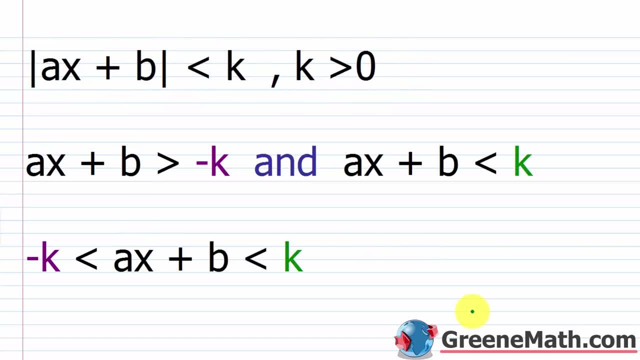 to work and satisfy that inequality. If we see something more complex, we can just write down this rule. So I isolate my absolute value operation on one side. It's the same thing we saw with the greater than, but just now I'm gonna have an and. 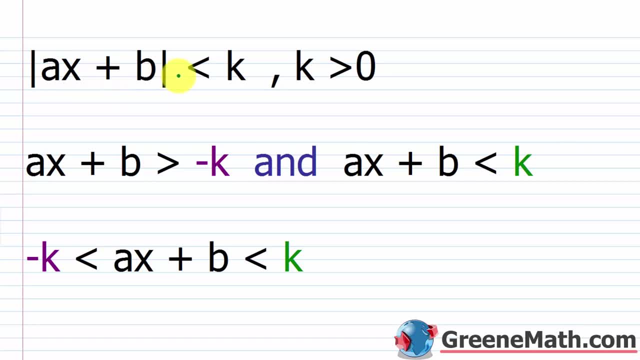 So it's the exact same procedure. So the absolute value of ax plus b is less than k. where k is greater than zero, We say we have: ax plus b is greater than negative k and ax plus b is less than positive k. 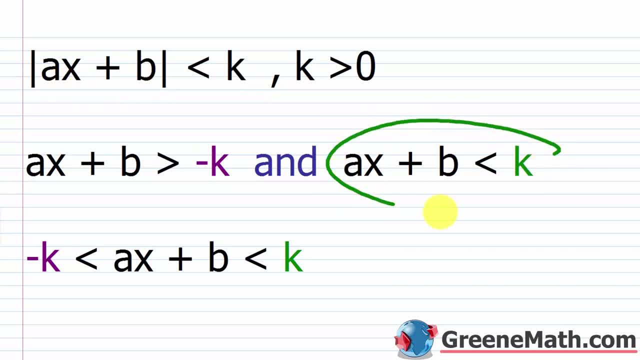 So again the first scenario: just remove the absolute value bars. So that's this here. The second scenario: remove the absolute value bars, flip the direction of the inequality symbol so you get a greater than, and then make this number out here negative. okay, 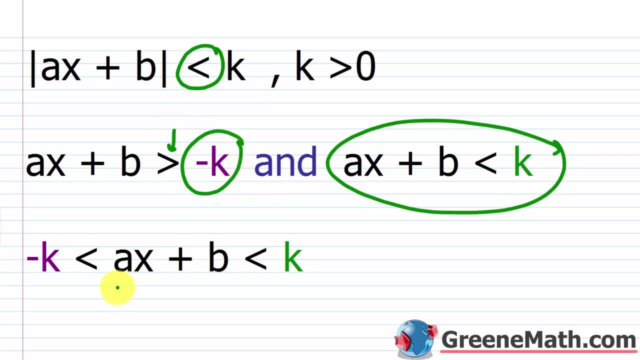 The only difference is you're using an and statement. So, really, if you wanna make this easier on yourself, just write it as a three-part inequality, So the expression goes in the middle and it's greater than the negative of this and it's less than the positive of this. 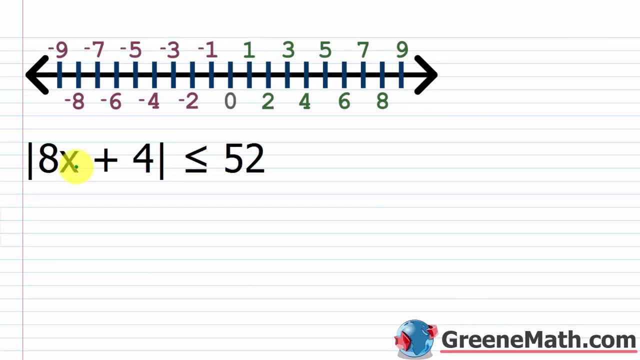 All right, let's take a look at an example. So suppose we had the absolute value of eight x plus four, and this is less than or equal to 52.. Well, this guy's already isolated for me, so I don't have a whole lot of work here. 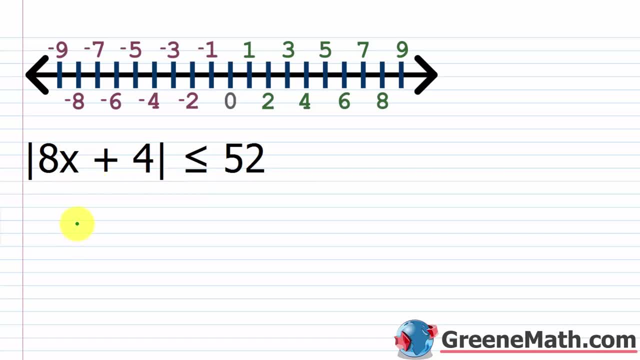 All I've gotta do is follow my rule. So I'm gonna drop my absolute value bars. I'll have: eight x plus four is less than or equal to 52.. Then, and okay, I'm gonna drop my absolute value bars. So eight x plus four, flip the signs. 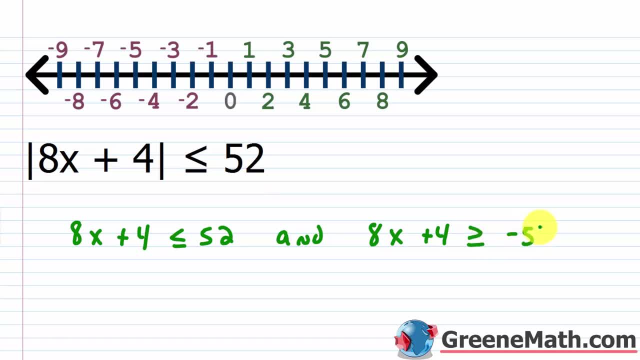 this becomes a greater than or equal to make 52 negative. So it's negative 52.. Now I would advise you to do this, okay, So I would advise you to do this okay. So I would advise, when you solve these, 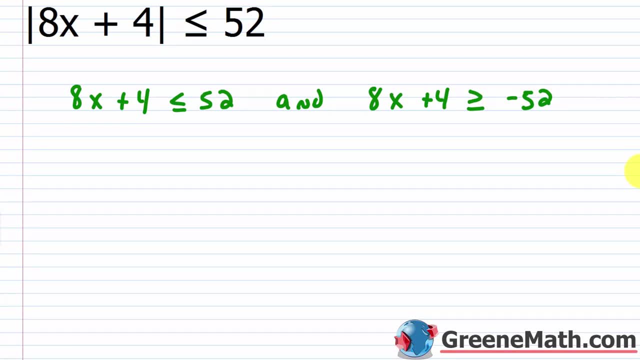 to put it as a three-part inequality, because it's just easier to work with. So I'm gonna put that negative 52 is less than or equal to eight x plus four, which is less than or equal to the number 52.. So if I wanna solve for x in the middle, 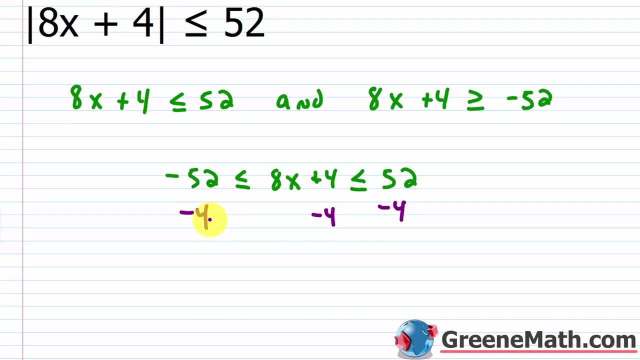 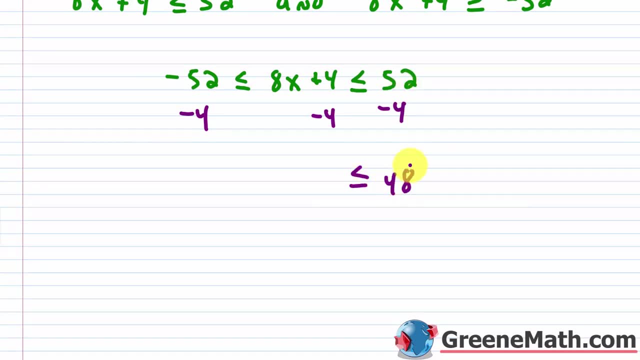 I would subtract four away from each part. Let me scroll down and get some room going. So on the right-hand side, 52 minus four is 48. And then this cancels. so I've just got eight x in the middle. 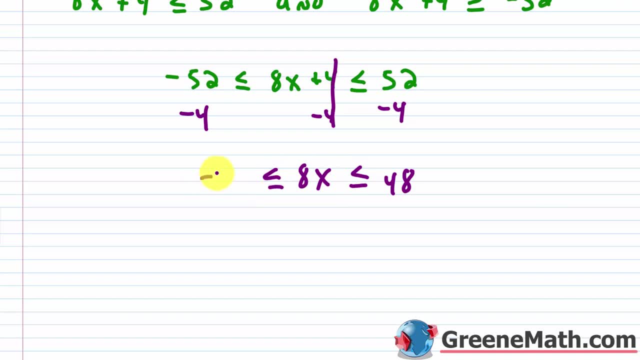 On the left-hand side, negative 52 minus four is negative 56.. All right, so to get x isolated in the middle, I'm gonna divide each part by eight. Let me make that a little better. So negative 56 divided by eight is negative seven. 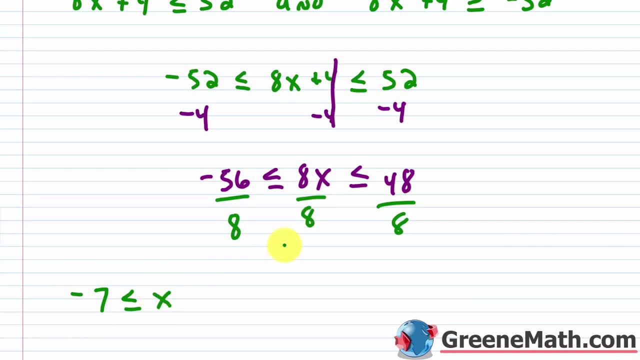 This is less than or equal to, eight over eight is one. so we just have x here in the middle. This is less than or equal to 48 over eight is six. So I have that x is basically between negative seven and six. 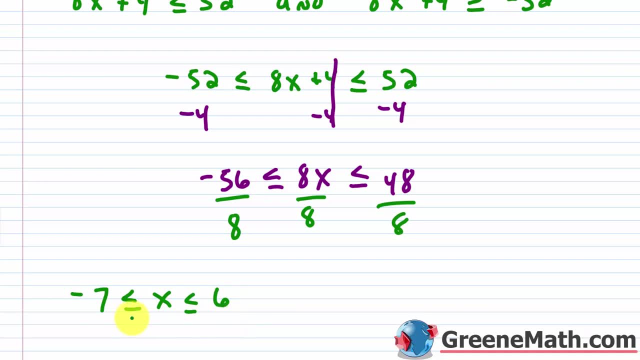 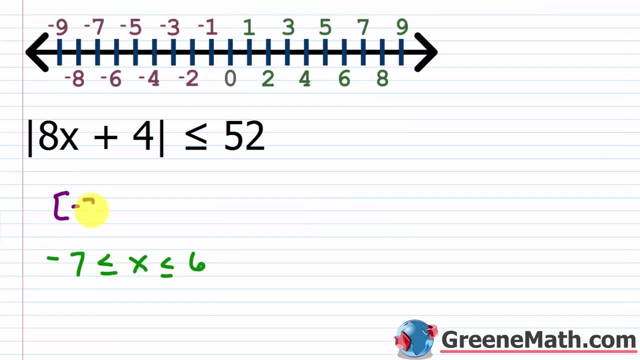 and negative seven and six are both included here because we have non-strict inequalities. So let me erase all this And again, we can write this in interval notation. We can use a bracket here at negative seven and then a bracket at six to show these are both included. 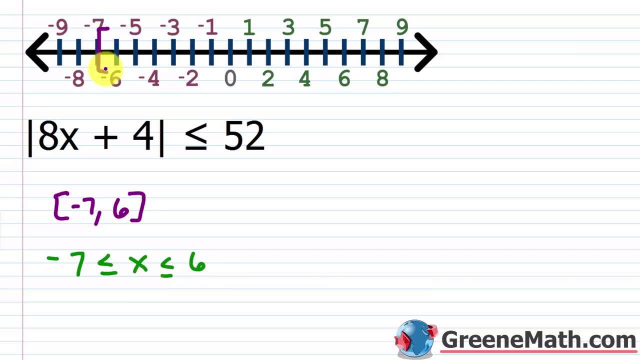 On the number line. I can use a similar process. So at negative seven I put a bracket, At six I'm gonna put a bracket, And let me make that a little better. And again I'm just gonna shade everything between. 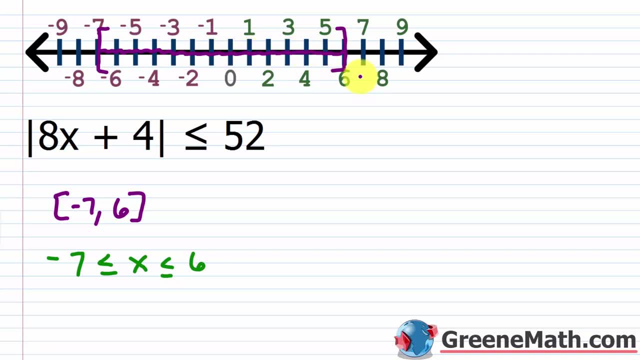 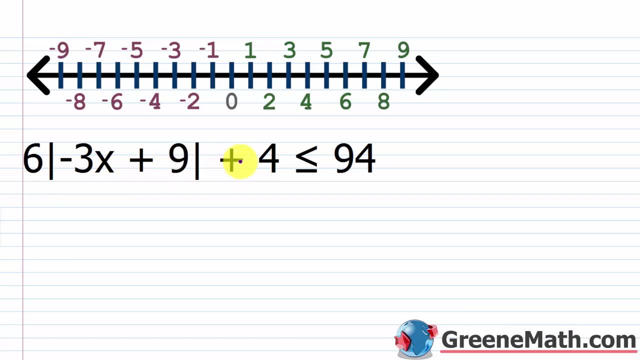 So from negative seven to six, all those numbers work, including negative seven and six. All right, let's look at another one. So we have six times the absolute value of negative three x plus nine. then plus four is less than or equal to 94.. 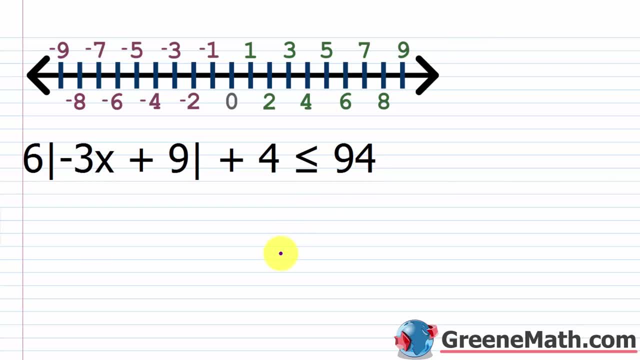 So again I've gotta isolate my absolute value operation so I can use my little rule. So I'm gonna subtract four away from each side of the inequality That cancels. I've got six times the absolute value of negative three x plus nine. 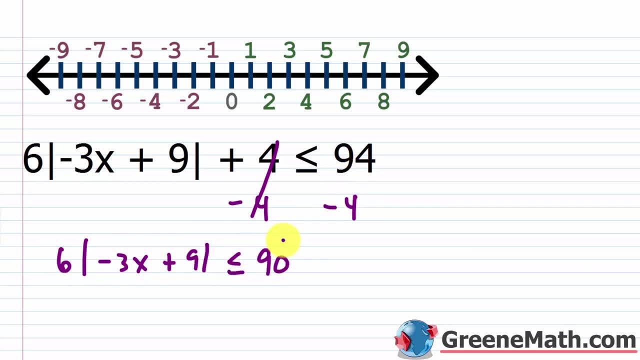 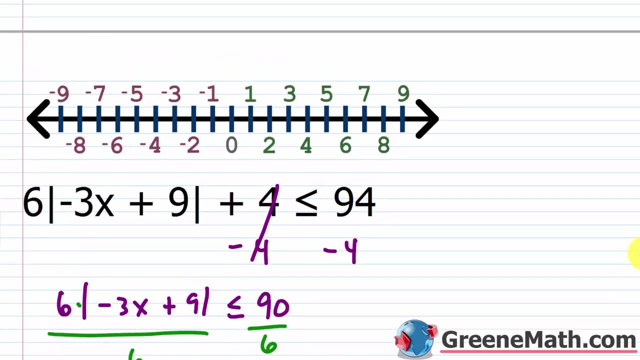 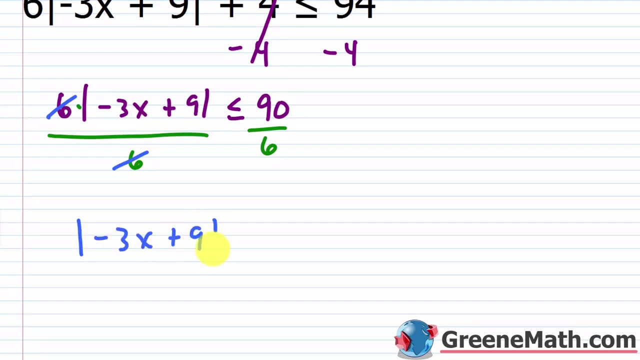 This is less than or equal to 94 minus four is 90. So now I'm gonna divide both sides by six, Because that's what's multiplying this absolute value operation. So let me get some room here. This cancels, We'll have the absolute value of negative three x plus nine. 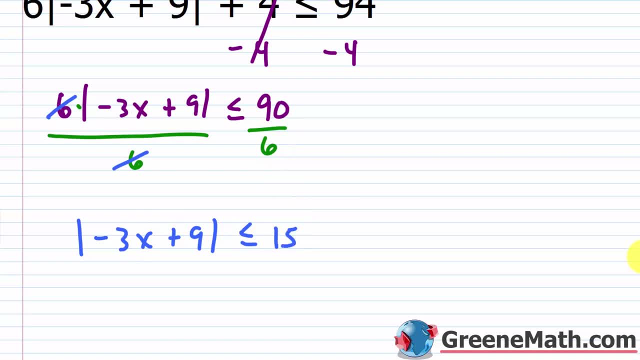 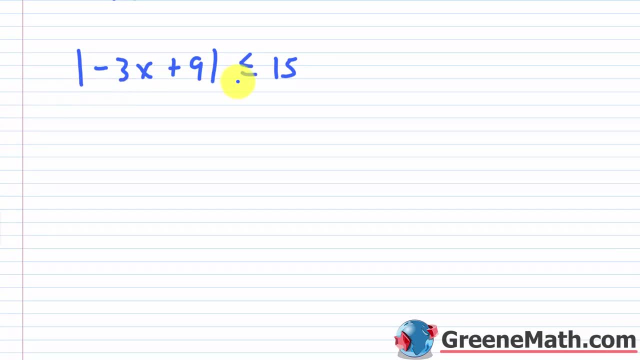 is less than or equal to 90 over six is 15.. Okay, let me get a little bit more room. So now we're ready to set up our compound inequality with: AND. So again, first scenario: just remove the absolute value bars. 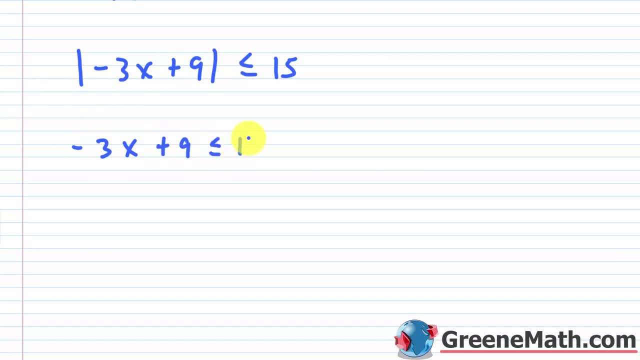 So negative three x plus nine is less than or equal to 15.. Then, AND okay, You've got negative three x plus nine. Again, remove the absolute value bars. flip the sign So it's a greater than or equal, to make this negative. 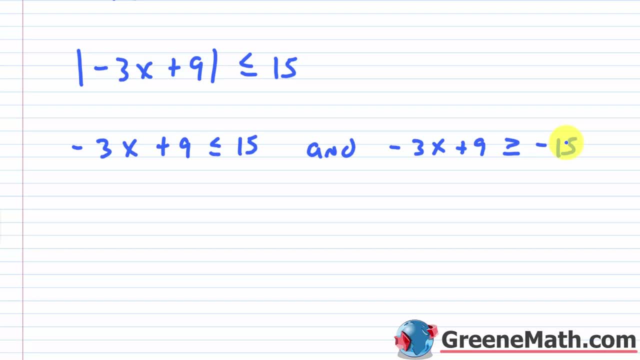 So this is negative 15.. And again, it's easier to just write this as a three-part inequality. This makes it faster to solve. So negative 15 is less than or equal to negative three x plus nine, which is less than or equal to 15.. 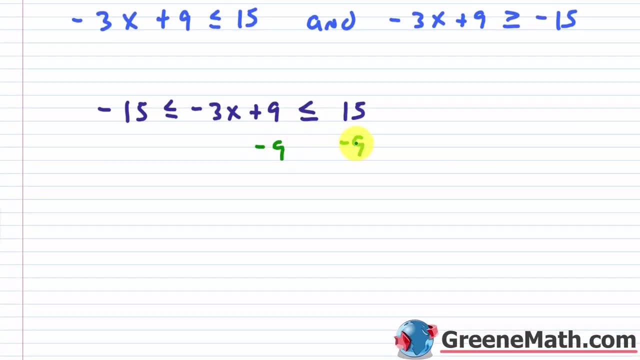 All right, let's solve this guy. So we're gonna subtract nine away from each part here. Negative 15 minus nine is gonna be negative. 15 minus nine. Negative 15 minus nine is gonna be negative. 15 minus nine. Negative: 24,. this is less than or equal to: 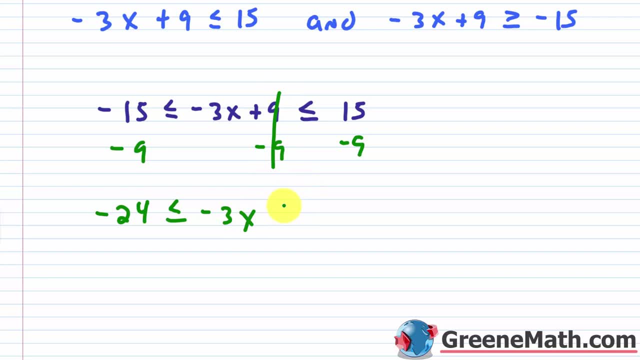 You've got your negative three x here and this cancels, And this is less than or equal to 15 minus nine is six. All right, so to get x by itself, let's divide each part by negative three And remember, even though it's a three-part inequality- 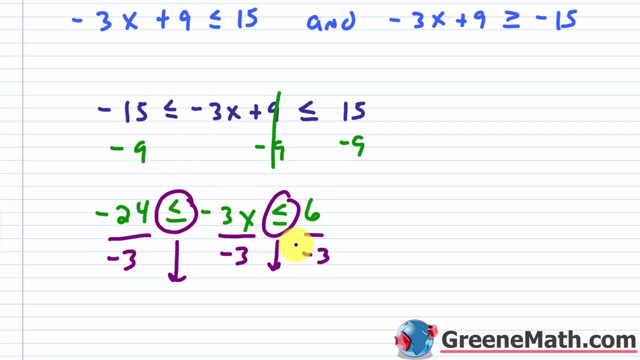 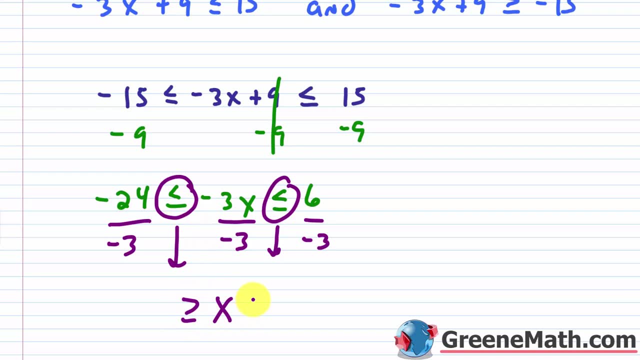 we've still gotta flip these signs. Very important. you do that okay, Otherwise you will get the wrong answer. So x is gonna be in the middle by itself. I'm gonna flip the signs to greater than or equal to Negative 24 over negative three is positive eight. 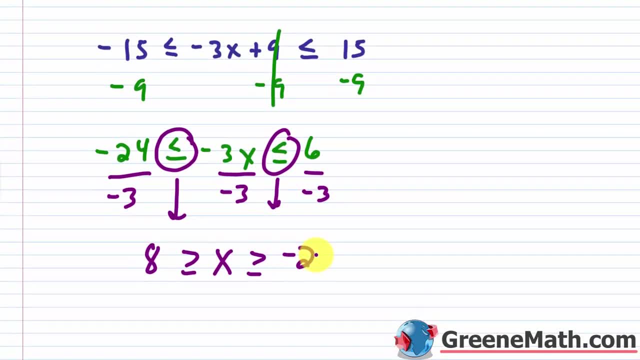 and six over negative three is negative two. So I'm just gonna reorder this and say this is: x is greater than or equal to negative two, and it's less than or equal to eight. So let's erase everything, All right? so let's go ahead and write this: 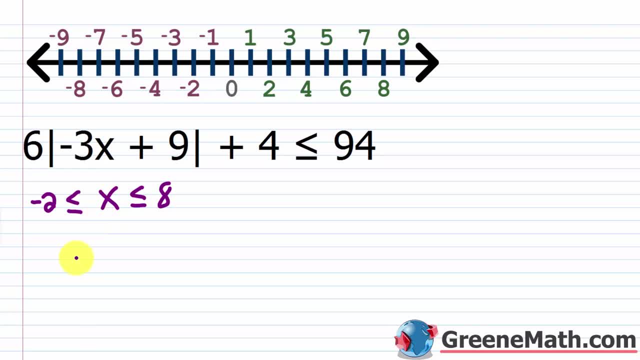 in interval notation. Again, our endpoints are included here. So I'll put a bracket and then a negative two, and then I'll put eight and then a bracket. Okay, so this is interval notation. Again, negative two and eight are both included. 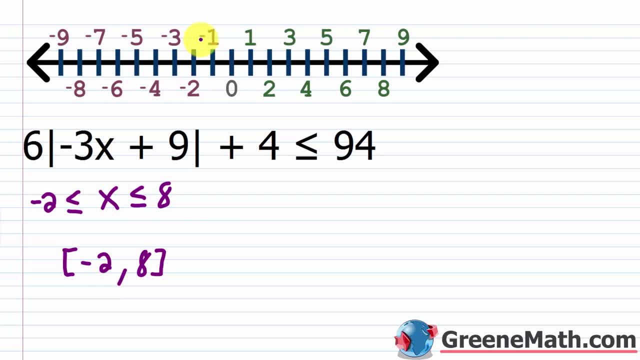 so we use our brackets. Then on my number line I could put a bracket at negative two and a bracket at eight. I could just shade everything in between. so that's my solution. region Again: from negative two to eight, with negative two and eight included. 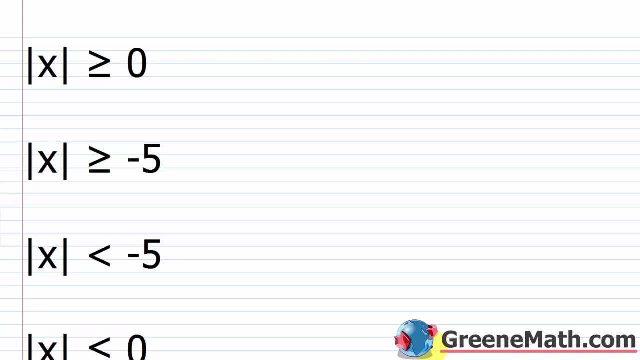 All right, now let's talk about the special case scenarios that come up. Basically, you have to think about things. If you get a right side of zero or a negative, you have to think about what's going on. okay, If I get something like the absolute value of X. 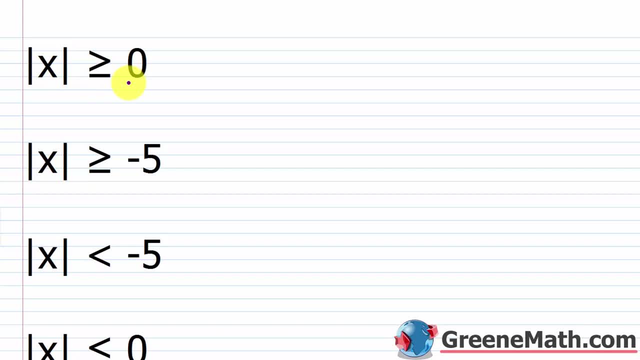 is greater than or equal to zero. this is true for all real numbers. okay, So if you get the absolute value isolated on one side and it's greater than or equal to the number zero, it's true for every real number, because the absolute value operation. 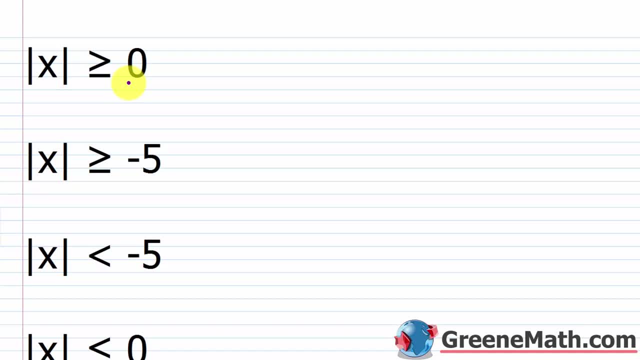 is either zero or some positive amount. So if the result from your operation is zero, you're okay, right, It works. If it's some negative, it still works right, Because you're gonna get a positive. If it's positive, it still works. 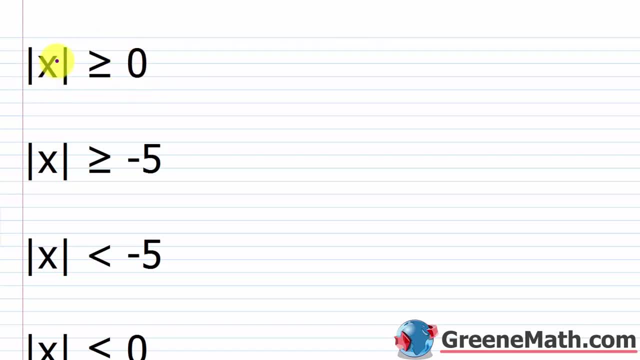 If it's negative, it still works right. So the absolute value of X is greater than or equal to zero when it's run through the absolute value operation. So this is all real numbers. okay for an answer For the absolute value of X. 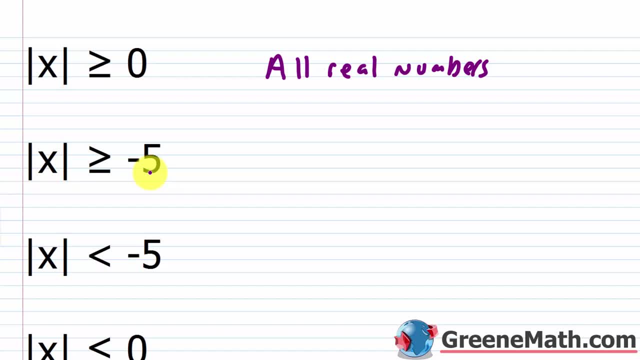 is greater than or equal to negative five. again, absolute value is always non-negative, So it's always gonna be zero or higher and it's always gonna be greater than the number negative five. right, It'll never be equal to it. 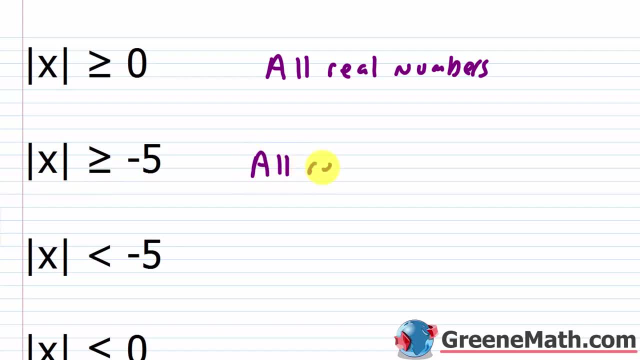 but if it's a negative value, it'll always be greater than that and it's gonna be less than or equal to zero. Okay, So if you see a negative over here and you've got a greater than all real numbers is your solution? 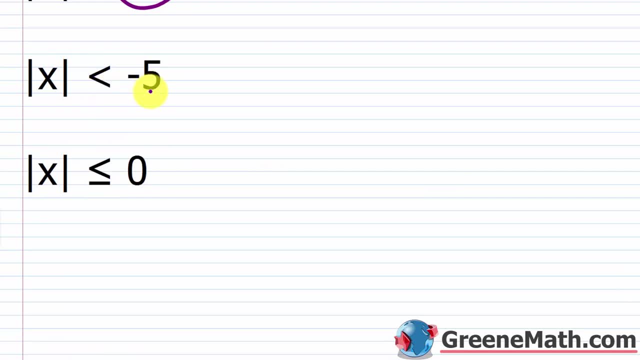 All right. what if you've got a less than and a negative over here? Well, here you can't get a solution right. The absolute value of X is less than negative five. That's not possible, okay, It can never be less than a negative. 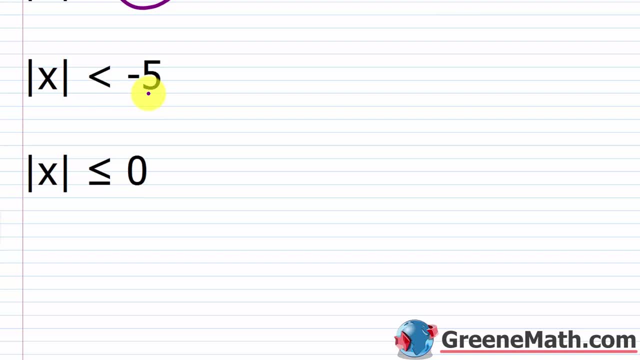 It can't be less than zero. okay, It can be zero or positive, That's it. So for this guy there's no solution. okay, Now, this one's a tricky one. okay, What if you saw the absolute value of X? 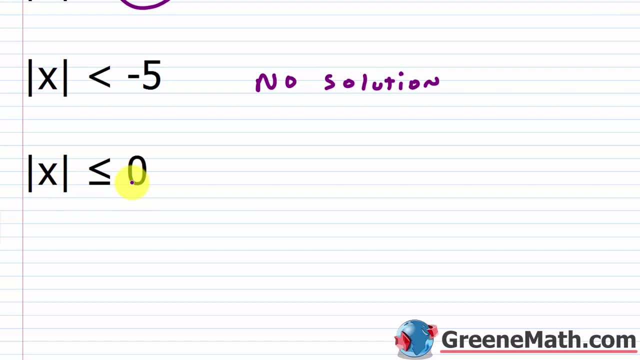 is less than or equal to zero. Well, we know that it can't be less than zero, but it can be equal to zero. So this one will have one solution: You basically need to set X equal to zero, and that's your solution. 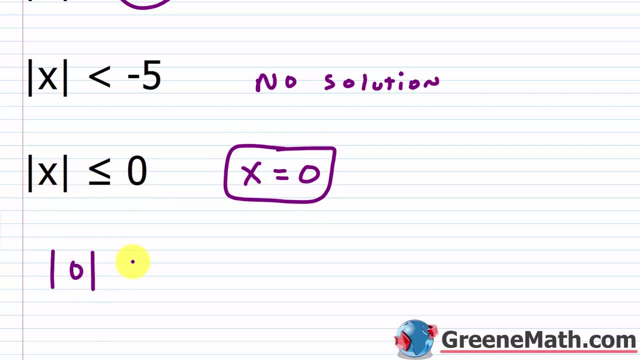 If X equals zero here, that works right. The absolute value of zero is less than or equal to zero. Right, zero is less than or equal to zero. That is true, okay. But if I use any other number, it does not work okay. 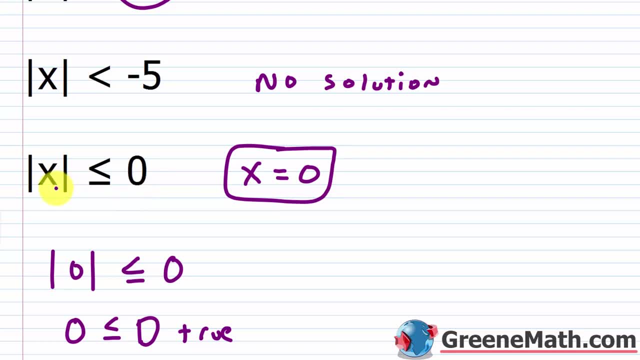 So what I wanna do with this type of scenario: if I've isolated the absolute value operation and it's less than or equal to zero, I just set that expression inside the absolute value bars equal to zero and I solve. and that's gonna be my solution. 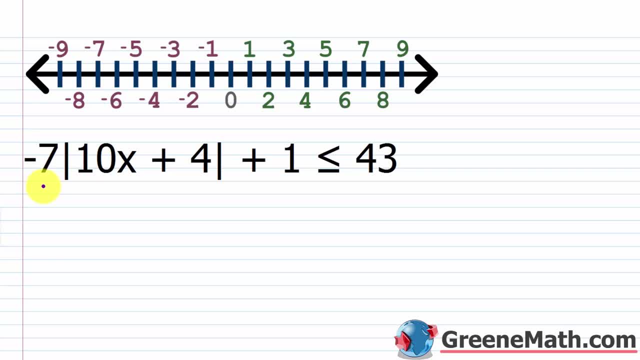 All right, let's look at a few examples. So we have negative seven times the absolute value of 10X, plus four plus one is less than or equal to 43. So again, we wanna start by isolating the absolute value operation. 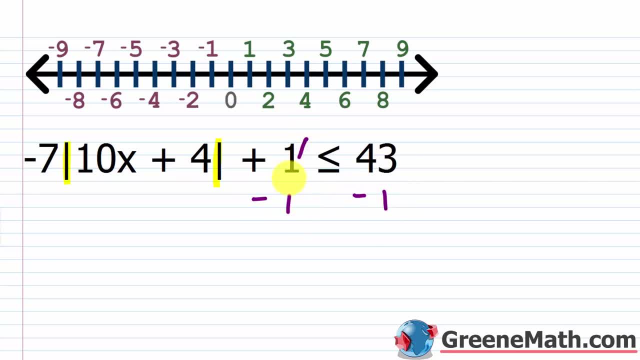 So I'm going to subtract one away from each side of the inequality. That's gonna cancel. I've got negative seven times the absolute value of 10X plus four again is less than or equal to 43. minus one is 42.. 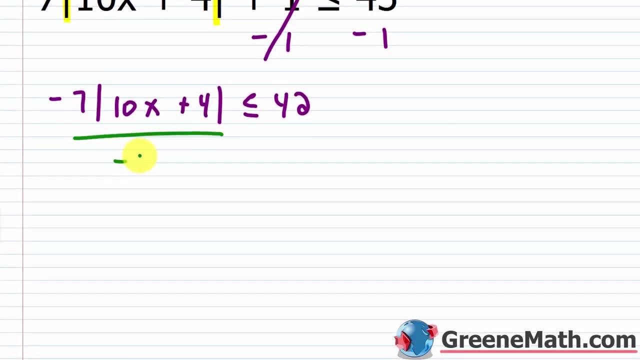 All right, let's get some room going. So now I'm gonna divide both sides of the inequality by negative seven. This cancels. I'm gonna have the absolute value of 10X plus four. Now I divide it by a negative. 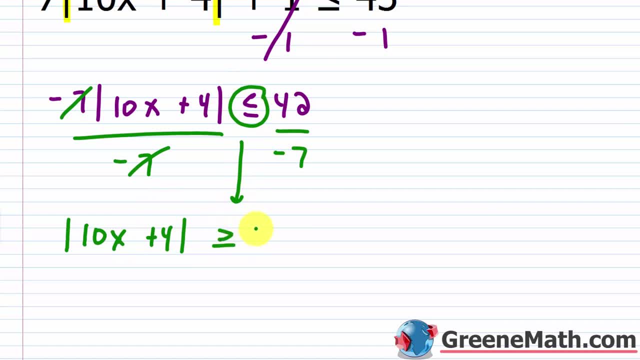 so this has gotta get flipped. So it's gonna become a greater than or equal to 42 over negative seven is negative six. Now you can stop here. The absolute value operation is isolated and it's greater than a negative value. What do we say about that? 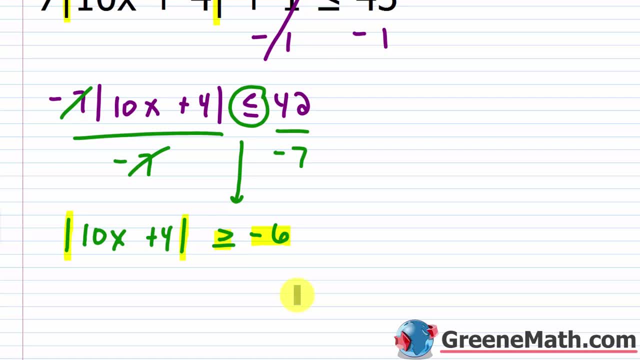 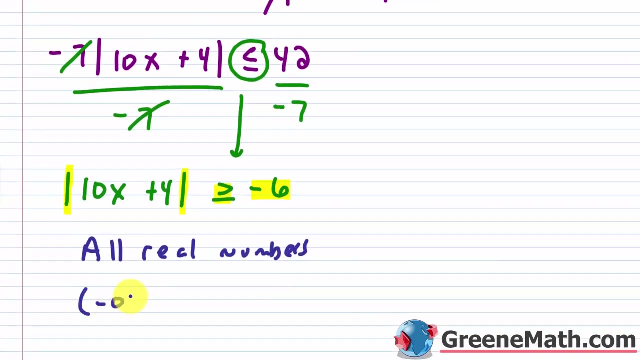 The absolute value operation is always going to be zero or some positive amount, So it will always be greater than negative six. So this is true for all real numbers. So you can stop and say all real numbers In interval notation. you can put from negative infinity. 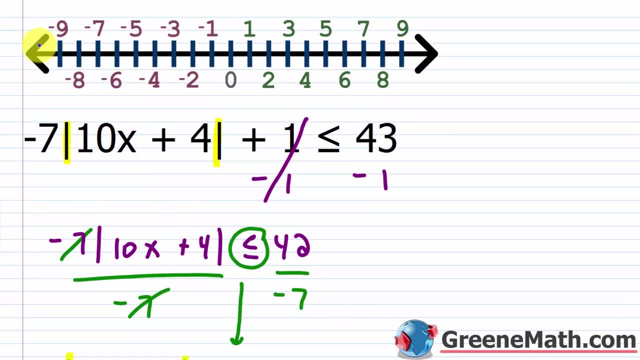 to positive infinity. And if you wanted to show this on a number line, you could basically just shade the entire number. okay, This would be your graphical solution: Just shade the entire thing. All right, let's take a look at another one. 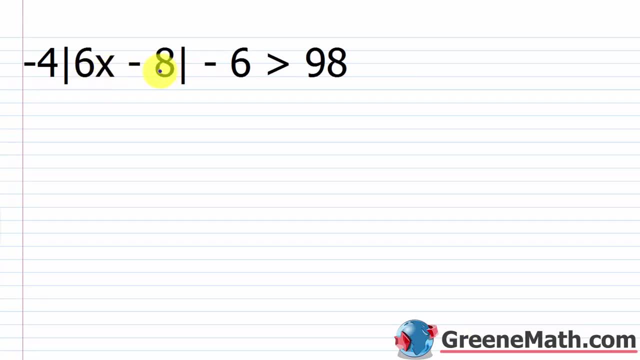 So suppose we had negative four times the absolute value of six X minus eight, then minus six is greater than 98. So again, I wanna isolate this part right here first. Very important, you do that. So let's add six to both sides of the inequality. 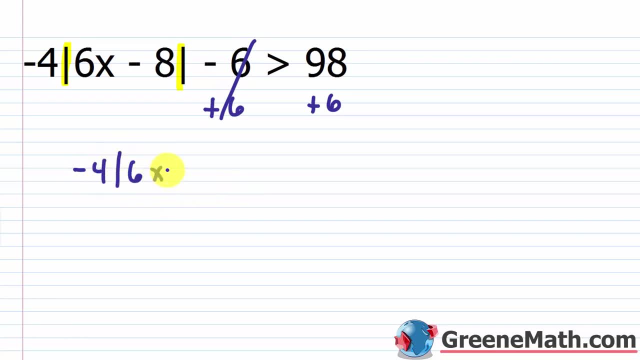 That cancels. You've got negative four times the absolute value of six X minus eight, And this is greater than 98 plus six is 104.. Let's divide both sides by negative four, So we know this cancels. I've got the absolute value of six X minus eight. 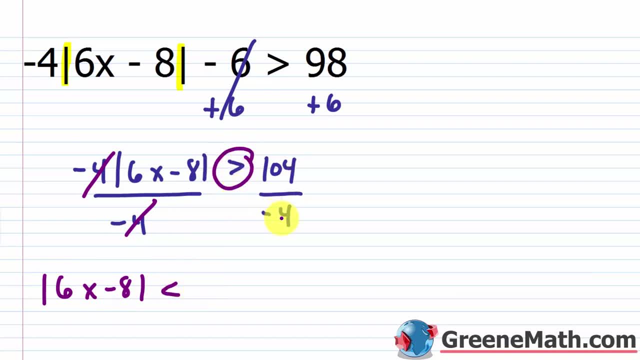 This is gonna get flipped, So it'll become a less than Then. 104 over negative four is negative 26.. Now can the absolute value of something ever be less than negative 26?? No, it cannot Again. it's gotta be zero or some positive amount. 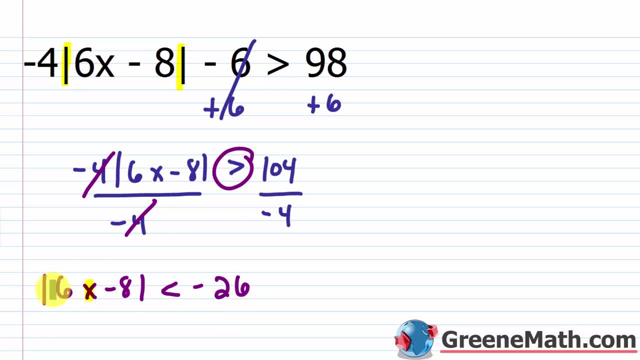 So it doesn't matter what I plug in here for X. Whatever, this result here is inside the absolute value bar. once I take the absolute value, it's gonna be zero or positive, So it can never, ever, ever be less than negative 26.. 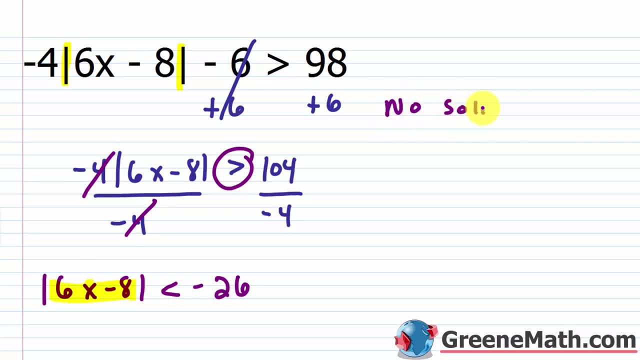 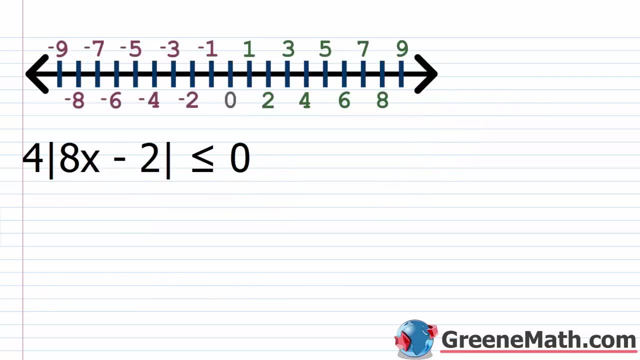 So there's no solution. No solution, okay, And again you can put that symbol for the null or empty set. All right, let's take a look at one more. So we have four times the absolute value of eight. X minus two is less than or equal to zero. 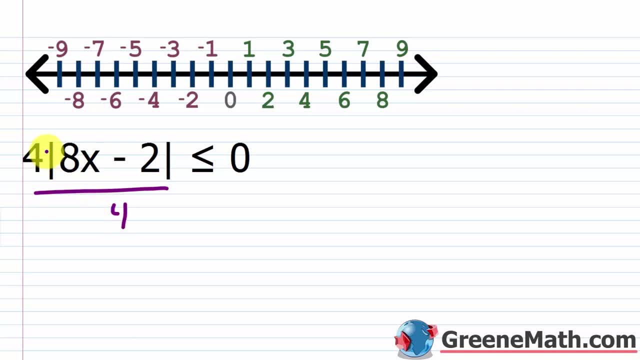 So again I can do this. I divide both sides by four so that I can isolate the absolute value operation. So this cancels. I get that the absolute value of eight X minus two is less than or equal to zero over four is zero. 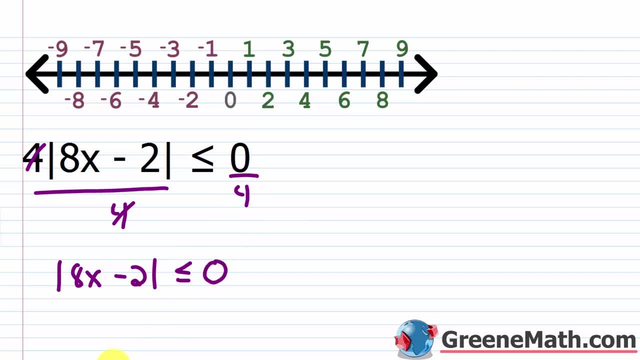 Now the only way again that this works is if we set this expression here: eight X minus two equal to zero, Because it can never be less than zero. That's not ever gonna work right, Because once we take the absolute value, 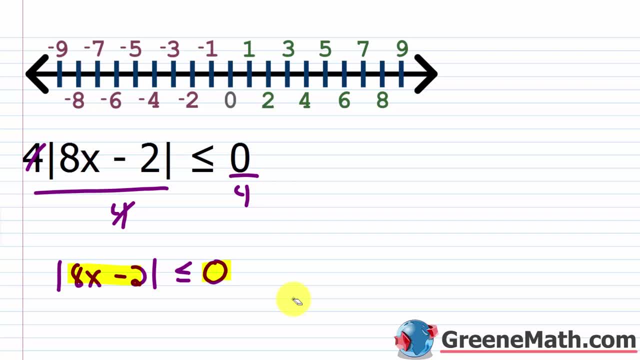 it's gonna be zero or something positive. So we can get it to equal zero, but we can never get it to be less than zero. So there's only one solution here. So eight X minus two is equal to zero. Add two to each side of the equation. 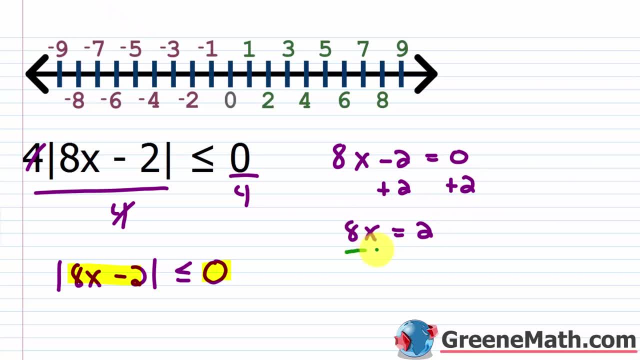 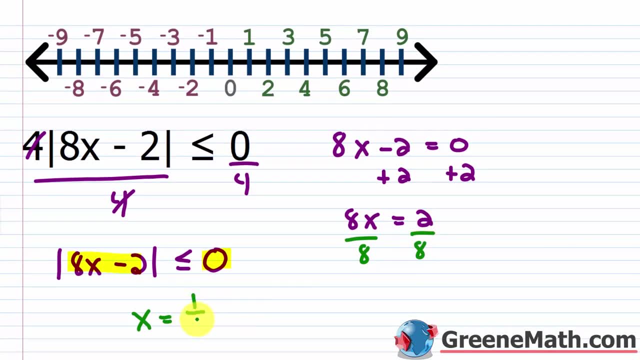 You'll have eight. X is equal to two. We're going to divide both sides by eight. We're gonna get that X is equal to two over eight. is one over four? okay, or one four? So the only way to make this true is if X is one four. 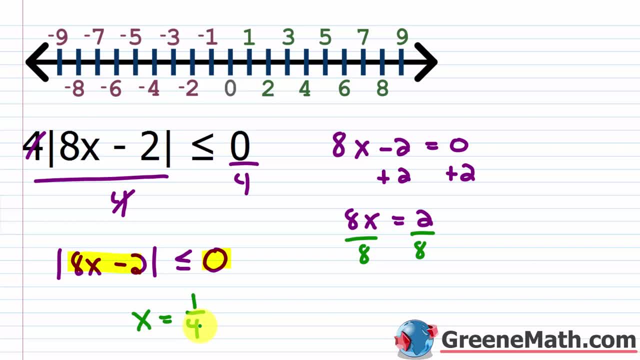 This is not a range of values. If we looked at this on the number line, you would basically just go to one fourth- Let's say this is one fourth here, And you would basically just put a dot there and say, my solution is just that number. 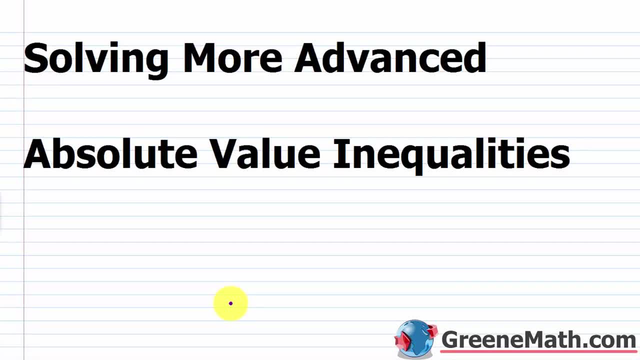 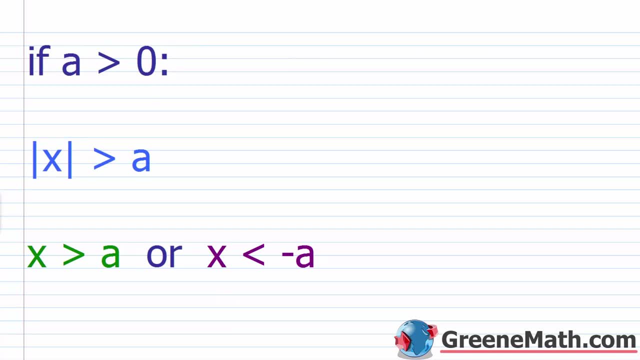 In this lesson we wanna discuss how to solve more advanced absolute value inequalities. So over the course of the last few lessons we've discussed some methods that can be used to solve some more advanced absolute value equations. Now again, we're just gonna go one step further. 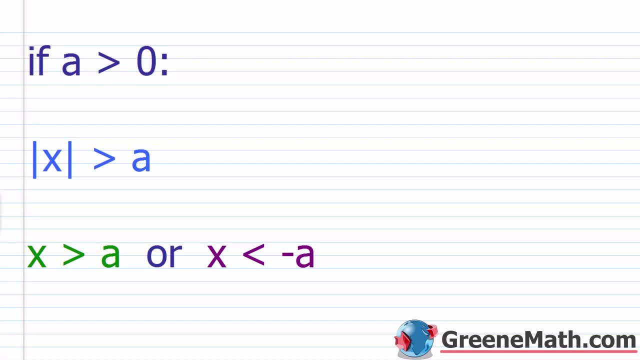 and think about how to apply these same strategies when inequalities are involved. So before we kind of jump into the examples, I just wanna take a minute to refresh your memory on absolute value inequalities, just the basic processes that we use when we're solving these guys. 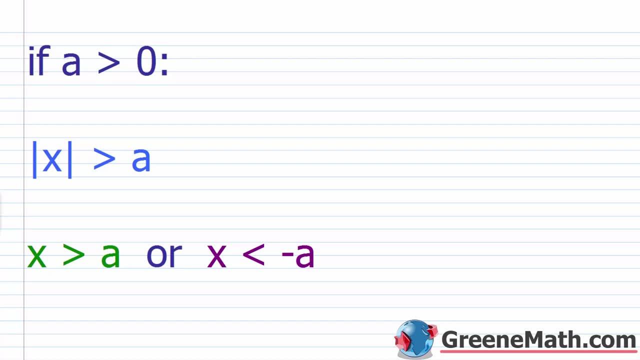 because it's been a while since we looked at them. So I think it's important just to get a little quick refresher in. So we should know that if A is greater than zero, so A just represents some positive real number. If we have, the absolute value of X is greater than A. 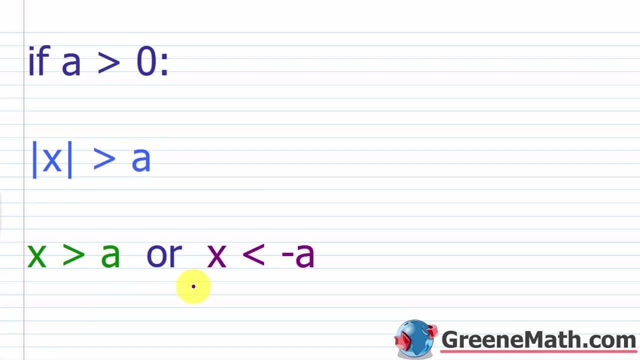 okay, greater than this positive real number. this gives us an OR right, A compound inequality with OR, So X can be greater than A, or X can be less than the negative of A. So as a quick example, let's say we had the absolute value of X. 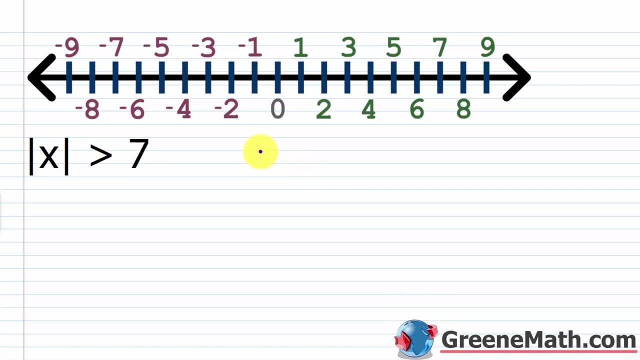 and this is greater than seven. We should know that. again, this sets up as X is greater than seven or X is less than negative seven. Graphically it's really easy to figure this out. Again, I'm thinking about what values here for X. 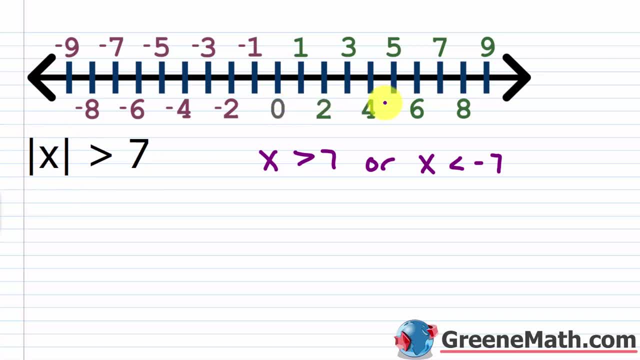 have a distance from zero that is greater than seven. Well, if I start at zero and I go seven units to the right, it can't be seven itself, but it can be anything larger, right? So I just put a parenthesis at seven. 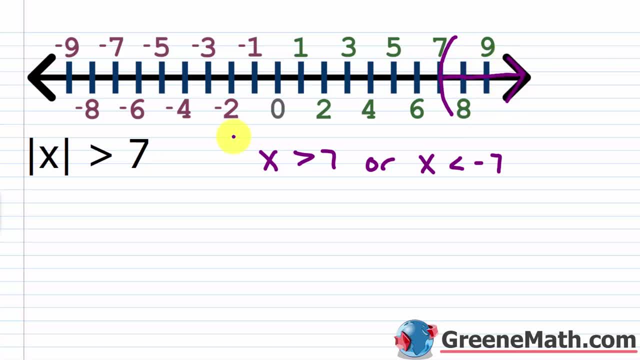 to say it's not included, and I shade everything to the right. Same thing goes in the other direction. If I start at zero and I go seven units to the left, I put a parenthesis at negative seven, I just shade everything to the left like that. 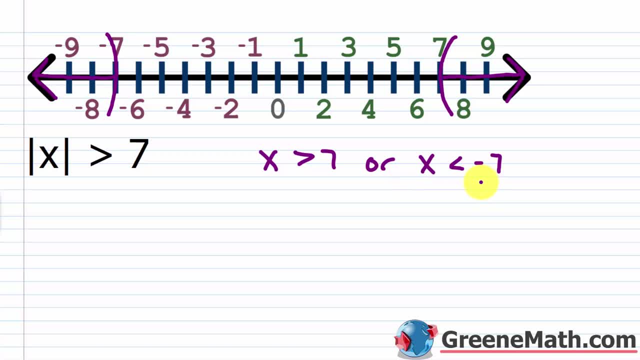 So this would be my solution graphically, And we also have this solution here kind of in our standard notation, And you can even use interval notation if you want. You can say from negative infinity up to, but not including, negative, seven, And then the union with seven is not included. 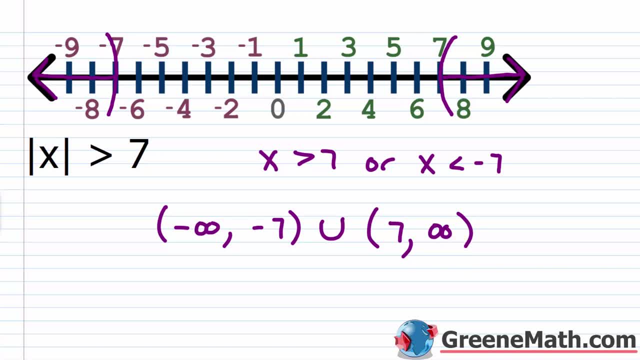 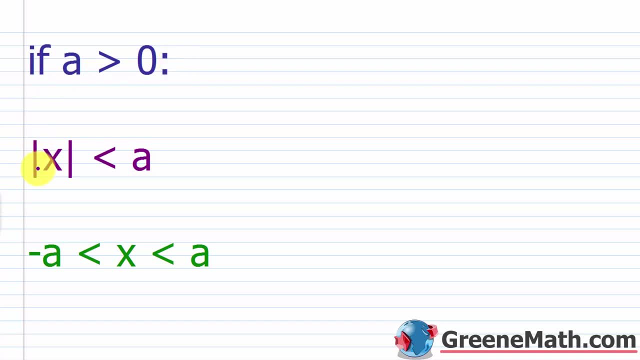 again out to positive infinity. okay, So let's take a look at kind of the other scenario that happens. So if A is a positive real number, again, if A is greater than zero, if the absolute value of X is less than this positive number A, 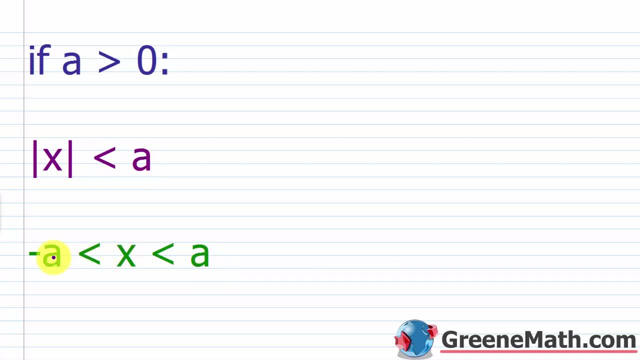 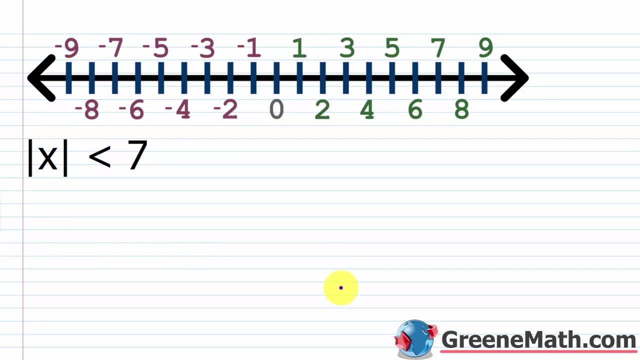 well then, X is gonna be between negative A and A right X is greater than negative A and it's less than A. So here we have a compound inequality with and. So let's look at this quick example here. Suppose we have the absolute value of X. 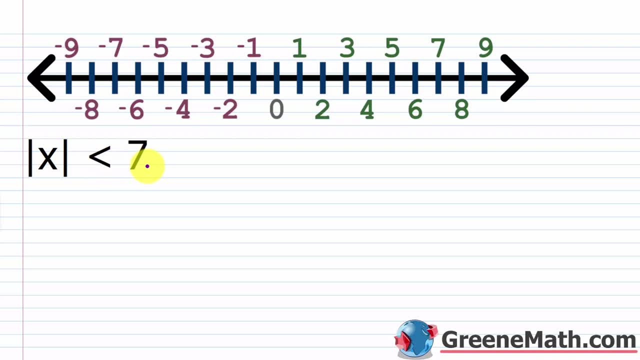 and now it's less than seven. okay, So we're gonna have a compound inequality with and. So basically, X is going to be greater than the negative of seven and it's gonna be less than seven itself Again. basically, to think about this graphically, 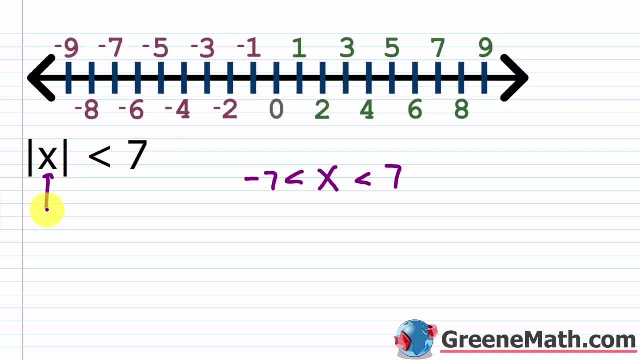 I'm thinking about all the values whose absolute value or whose distance from zero is less than seven. So, starting at zero, I could basically travel up to, but not including seven, So again at seven. I just put a parenthesis there. 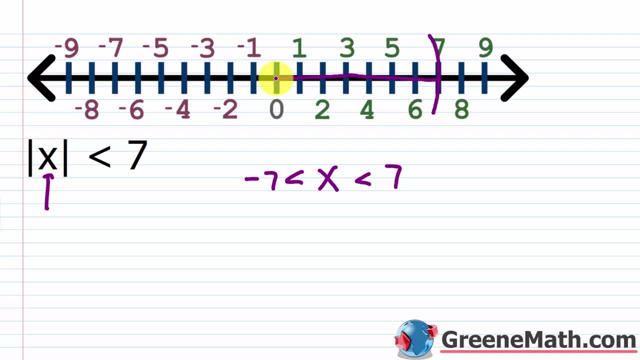 And again I could go the opposite direction. So, starting at zero, I could go down to- okay, down to, but not include negative seven. So I'd put a parenthesis there as well. So that would be my graphical solution: Again, from negative seven to seven. 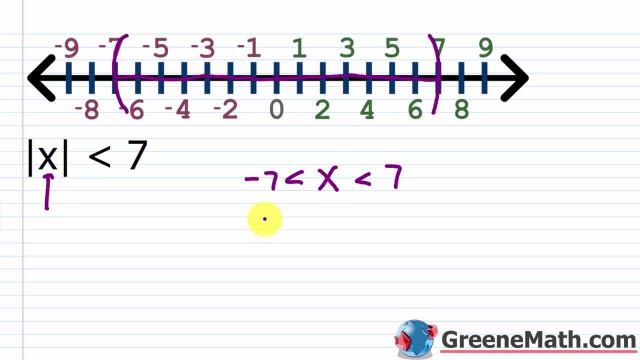 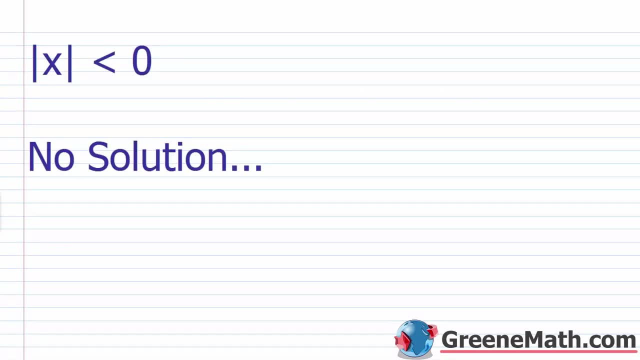 with neither of those included, And then in interval notation I'd have negative seven, comma seven, again with a parenthesis next to each. All right, so two special cases that come up that we need to be aware of. Again, if the absolute value operation. 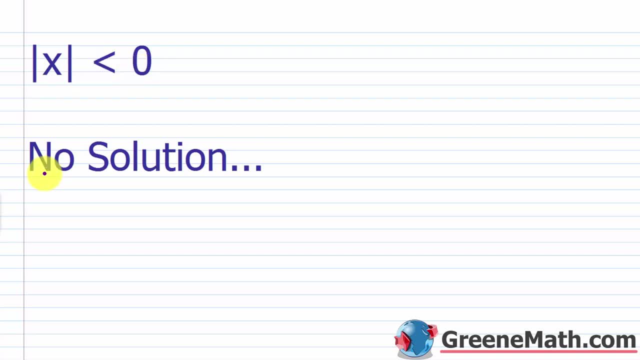 in this case, is the absolute value of X. if we say this is less than zero, there's no solution here. okay, There's nothing I can plug in for X and take the absolute value of and say that it's going to be less than zero. 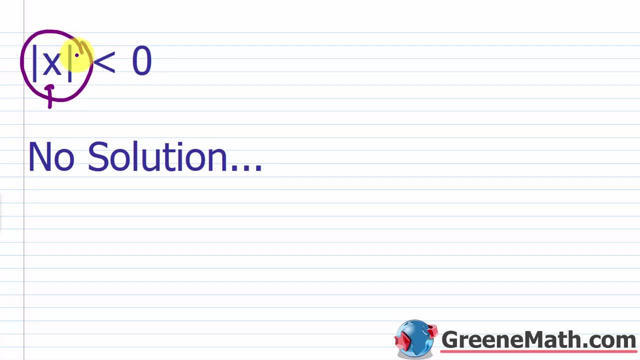 because the result of this operation here is going to be zero, which is obviously not less than zero, or it's gonna be some positive number, which is also negative. Now we're gonna be less than zero. So in this situation there is no solution. 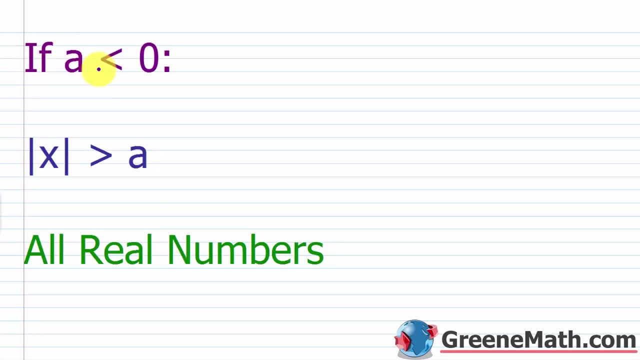 And our last special case we're gonna come across: if A now is a negative number, if it's less than zero, so some negative real number, then if we have the absolute value of X is greater than this negative real number, well then we're gonna have a solution. 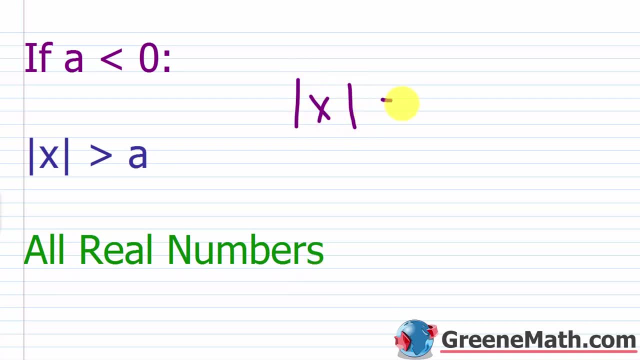 that's all real numbers, right? If I have, the absolute value of X is greater than negative five, well, that's always true, right? No matter what I plug in for X, the result of this will either be zero, which is greater than negative five. 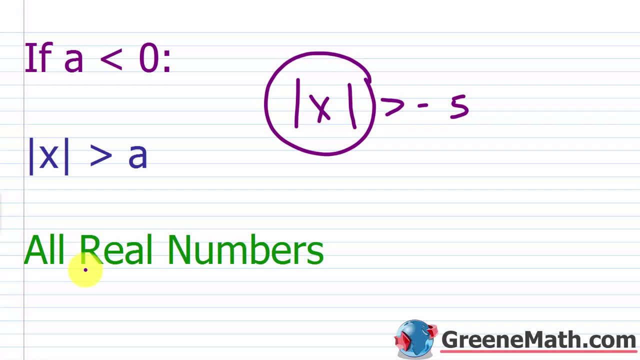 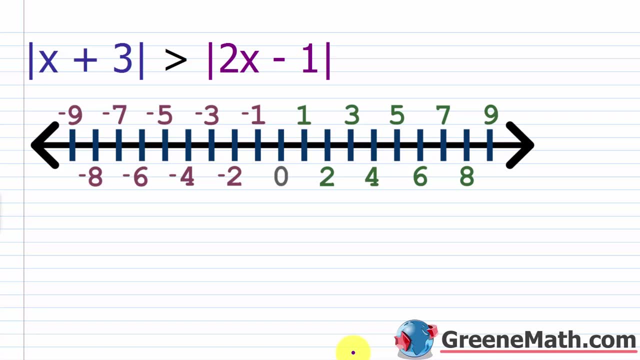 or it'll be positive which is also greater than negative five. So this is always true, or you could say true for all real numbers. Okay, so now let's get to kind of the first example, And hopefully you saw the lesson where we solved more advanced absolute value equations. 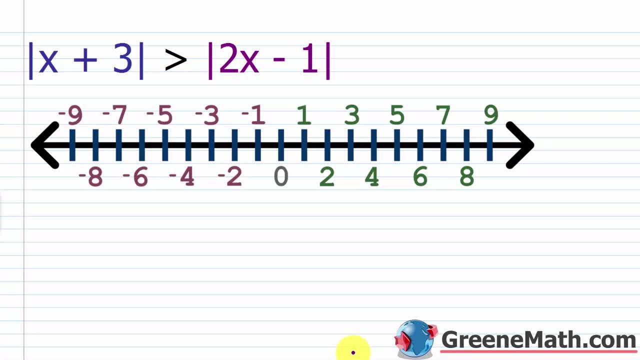 If you did that lesson already, this is gonna be a breeze for you. We're basically using the same concepts, okay, So suppose you had something like: the absolute value of X plus three is greater than the absolute value of two X minus one. 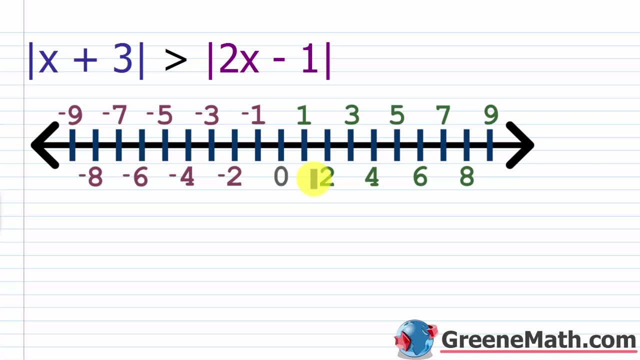 Again, if you get these, what you wanna do is you wanna think about where the expressions inside of the absolute value bars are gonna be zero. okay, You're thinking about kind of the turning point. So where could this guy go from negative to positive? 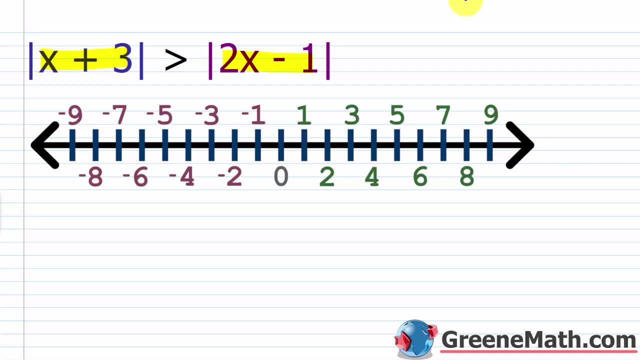 or from positive to negative. Well, that can only happen when that expression is equal to zero, okay, So if I say X plus three is equal to zero, and I solve that, I get that X is equal to negative three, okay. 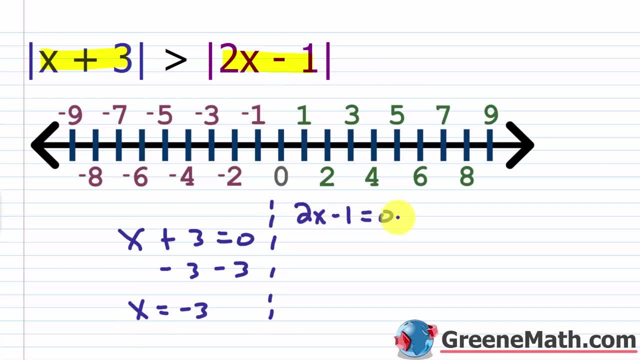 And then, alternatively, if I say that two X minus one is equal to zero, I add one to each side of the equation, I get two X is equal to one. divide both sides by two and I find that X equals one half okay. 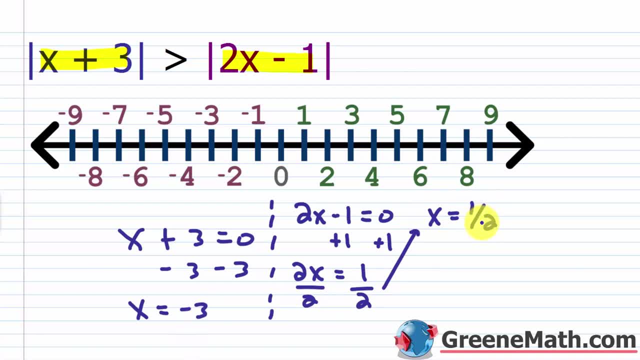 So we're gonna use these numbers negative three and one half to kind of split the number line up into three intervals. okay, And I'm not gonna do it on this number line here. I'm gonna use a table, because I find it to be a little bit easier. 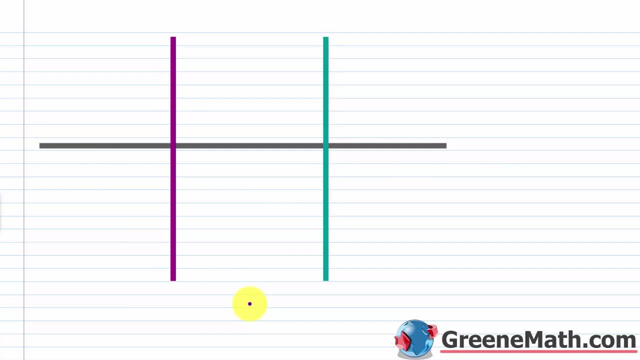 So the numbers we were working with again are negative three and positive one half, So we're using that to split the number line up into three intervals. I just prefer to do this on a table because it's just easier for me to organize things. 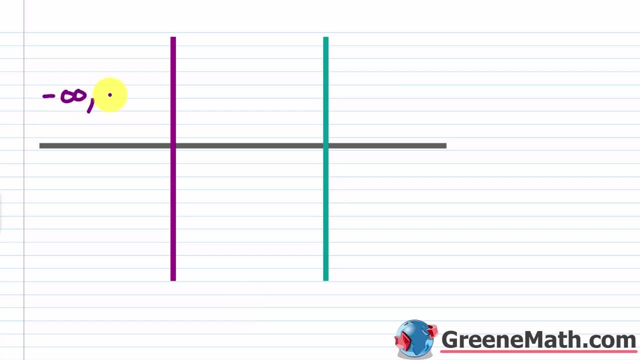 So the first interval will be from negative infinity up to, but not including, negative, third. okay, So that's my first interval, Then my second interval: negative three. I'm gonna include that, okay, And this is gonna be out to, but not including one half. 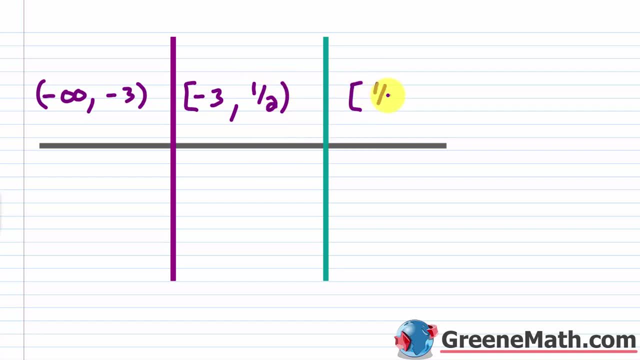 Then my third interval will be anything that includes one half or larger. okay, So from one half out to positive infinity. Now what we're gonna do here? let's go back up So we have: the absolute value of X plus three is greater than the absolute value of two X minus one. 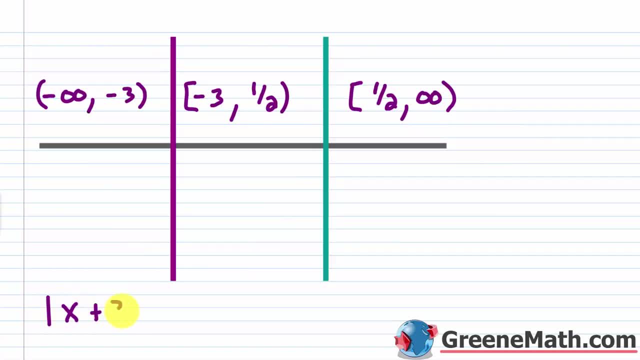 Let's go ahead and write that real quick. So the absolute value of X plus three is greater than the absolute value of two X minus one. Okay, so what we're doing here is we're looking at each interval, We're thinking about. 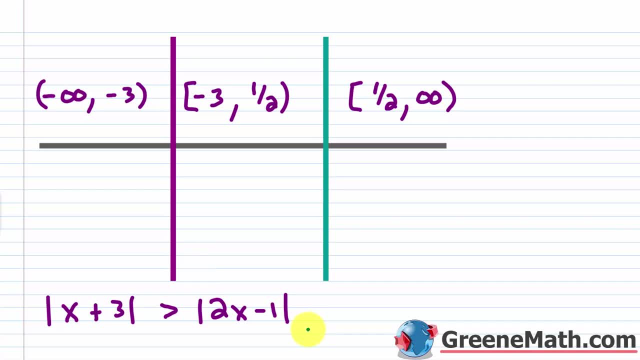 is the expression inside of the absolute value bars negative? Is it zero or is it positive? okay, That's what I wanna consider. So for this guy right here, think about the fact that in this interval it's going to be negative, right. 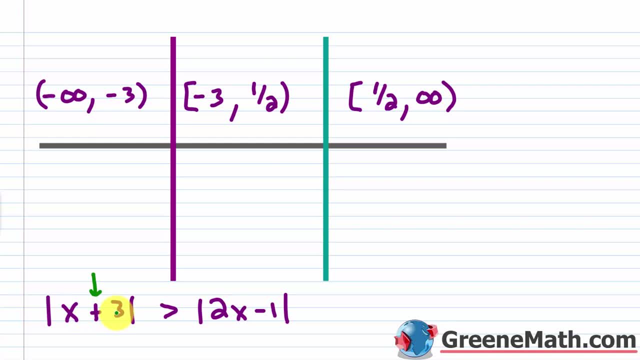 I know that X plus three is equal to zero when X equals negative three. So anything less than negative three means it's going to be negative, right? So in this interval, I will replace this expression here, this absolute value of X plus three. 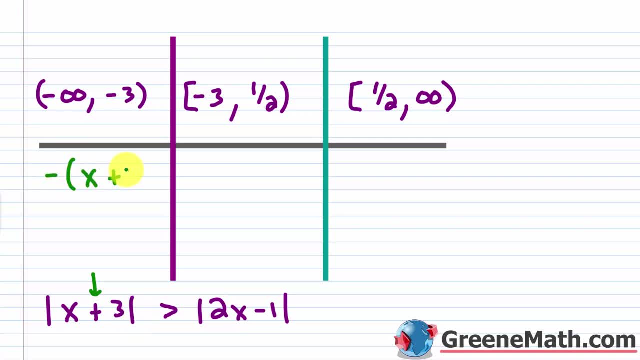 with the negative of X plus three. okay, So I just wrap it in parentheses and put a negative out in front to express that. Okay for this guy right here, this two X minus one, it's also gonna be negative, right. 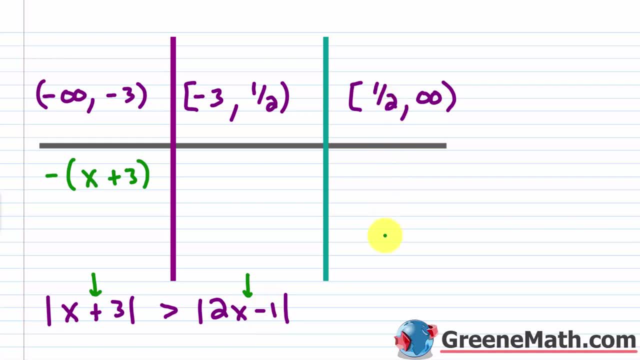 Because two X minus one is going to be zero when X is one half. So if we're less than a half, which we are in this case, it's going to be negative. So again, I just wrap it in parentheses. So two X minus one put a negative out in front, okay. 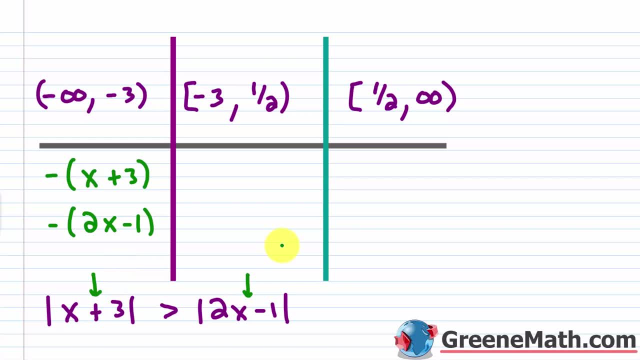 And we'll deal with this scenario in a second. Let's just kind of move on and write everything. So in this interval here we have from negative three up to, but not including one half. So at negative three, we know that this guy would be zero. 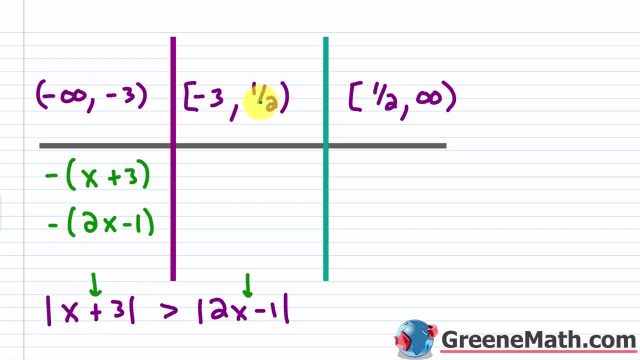 but anything larger than that means it's going to be positive. okay, So whether it's zero or some positive value, I can just take the expression itself. So I can just say it's X plus three here And again, this is still in a format. 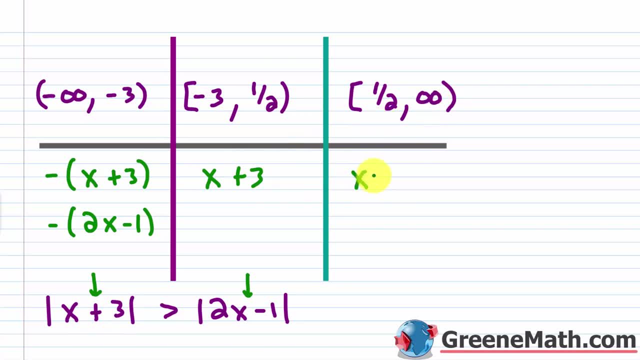 of where it's larger than negative three. So in this interval it'll also be just X plus three. okay, Then for two, X minus one. again, it's made zero when X is one half And this interval between negative three. 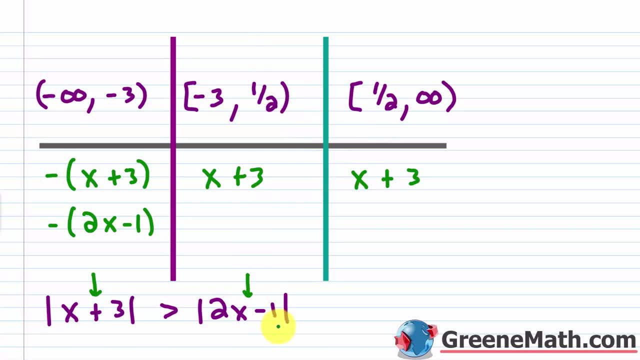 including negative three up to, but not including one half, it's still going to be negative, right, Because that's less than one half. So I would say the negative of two X minus one, And then here it could either be zero if X is a half. 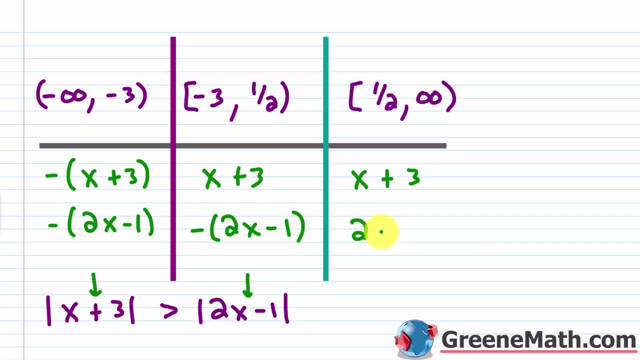 or some positive value. So I just dropped the absolute value bars and write the expression: So two X minus one. okay, So a very simple process. Again, if it's zero or positive in that interval you replace the absolute value expression with just what's inside the absolute value bars. okay, 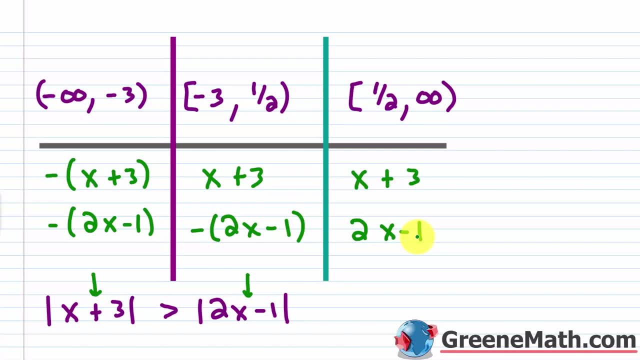 It's all you need. If it's a negative, okay, then what you want to do is drop those absolute value bars, wrap it in parentheses, put a negative out in front. You're basically changing it into its opposite, All right. 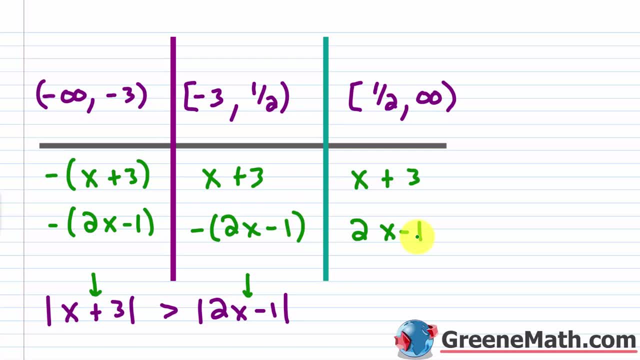 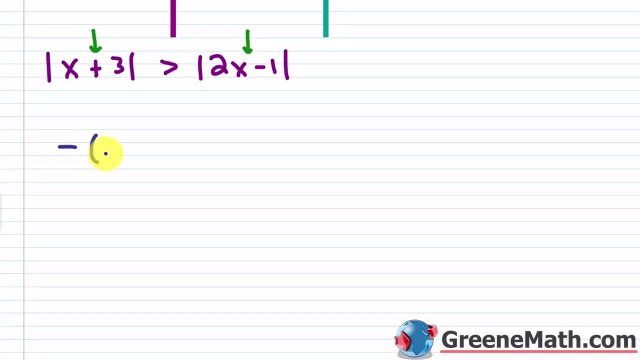 So now we've got a lot of work to do, We've got to go through the different possibilities. So the first possibility is that both of these are negative. So let's kind of scroll down and crank that out. So I'm gonna have the negative of X plus three. 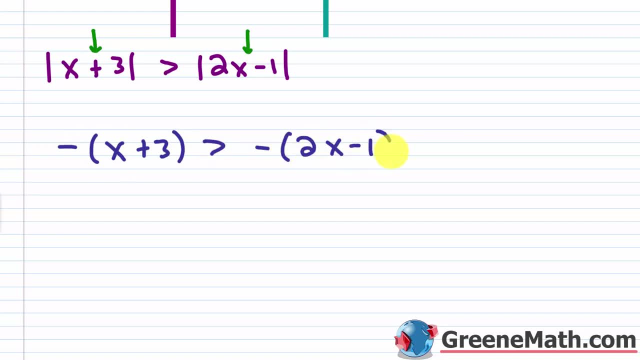 is greater than the negative of two X minus one. Now, if we want, we can clear the negative. So we're gonna have two negatives by just dividing both sides by negative one, But again, because we're working with inequality and we divide it by a negative, 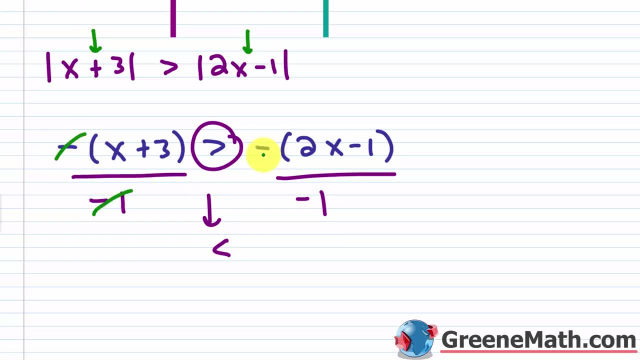 we've got to flip that guy, okay. So this is gonna cancel and this is gonna cancel. You have X plus three. now is less than two X minus one. Let's go ahead and subtract two X away from each side of the inequality. 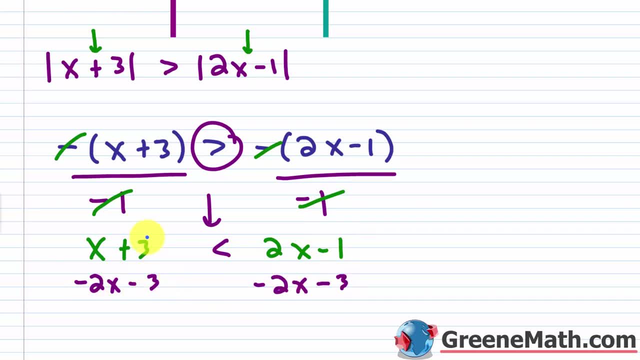 And let's also subtract three away from each side of the inequality. So this is gonna cancel. This is gonna cancel. We'll have X minus two, X, which is negative, X, And this is less than You've got: negative one minus three. 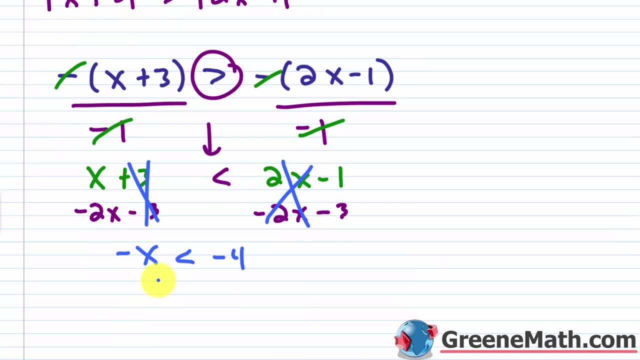 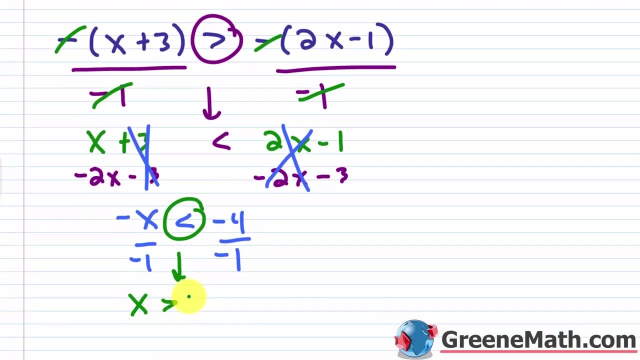 which is negative four. As a final step, let's divide both sides by negative one And again we divide it by a negative. So flip this guy, You're gonna get that X is greater than four. okay, So X is greater than four. 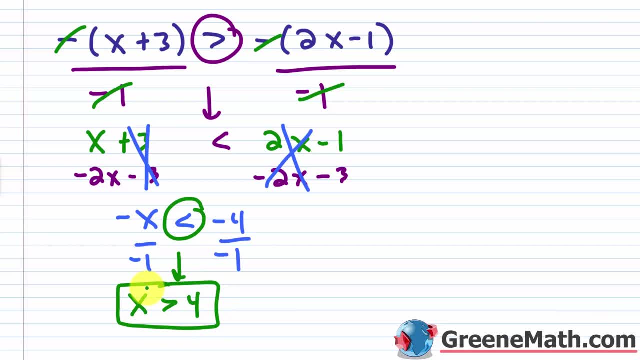 Now we wanna compare X is greater than four to the interval that we're working with. The interval that we're working with specifically says that X is basically coming from negative infinity up to, but not including negative three. X is greater than four is not in that interval. 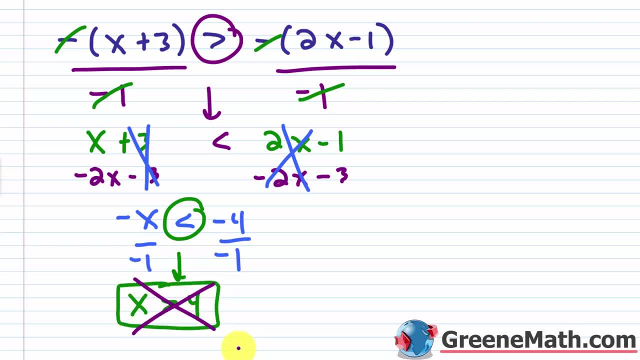 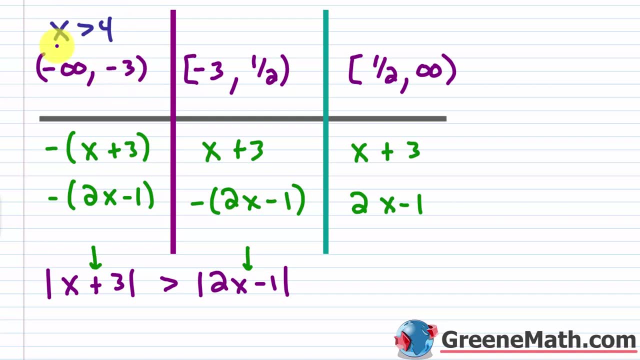 So this solution is gonna be rejected. okay, Let me erase all this and I'll kind of write it in the column. So I'm just gonna write: X is greater than four. here And again, this is not within our interval. So we reject that solution, okay. 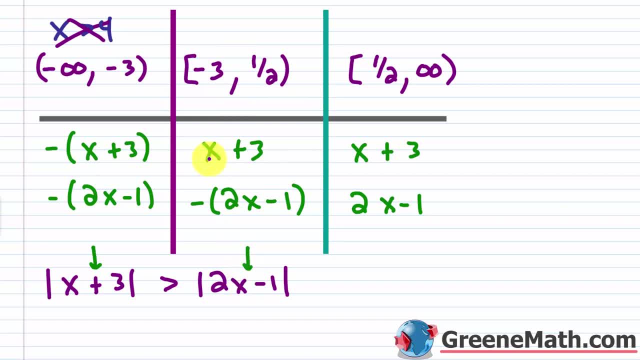 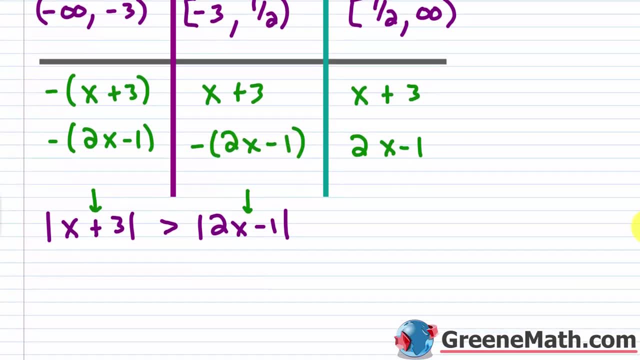 Now let's think about this interval here Again, where the X plus three is positive and we're gonna use the negative of two X minus one, okay, So let's scroll down And we're gonna say that we have X plus three is positive. 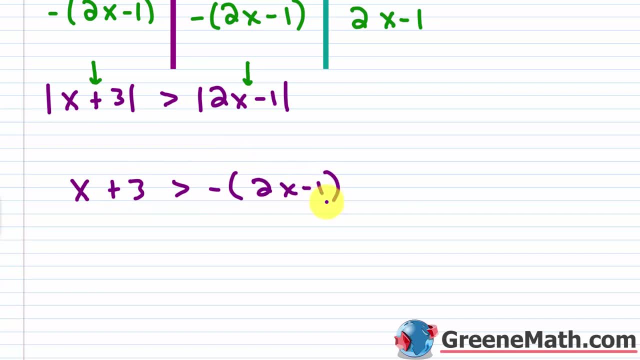 and then this guy is gonna be negative, So the negative of two X minus one. okay, So let's go ahead and solve this guy. I'm gonna distribute this. This will be negative two X plus one. So if I add two X to both sides of the inequality, 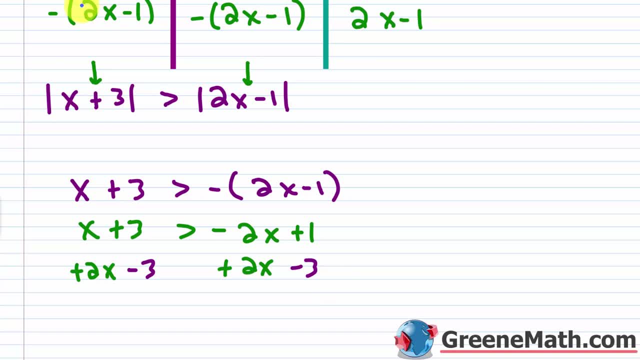 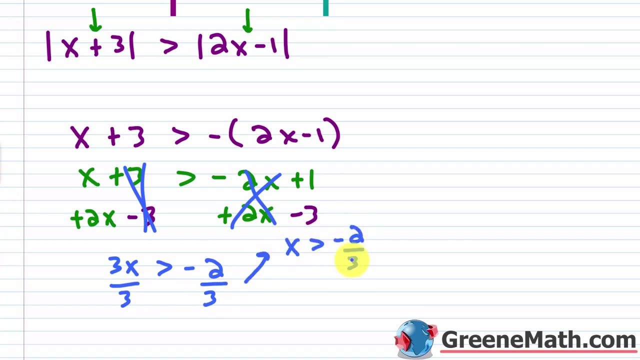 and I subtract three away from each side of the inequality. this will cancel. This will cancel. X plus two. X is three. X This is greater than one minus three is negative 2. Divide both sides by 3. And we get that x is greater than negative 2 thirds. Okay, So let me. 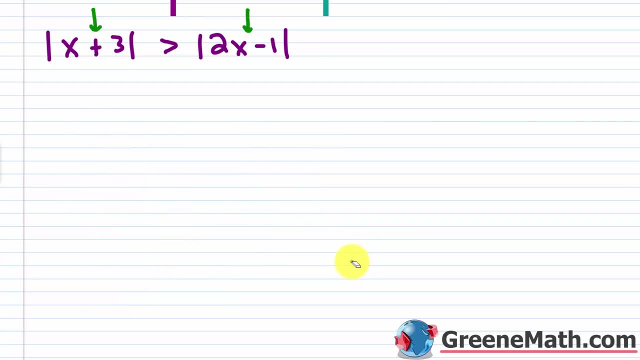 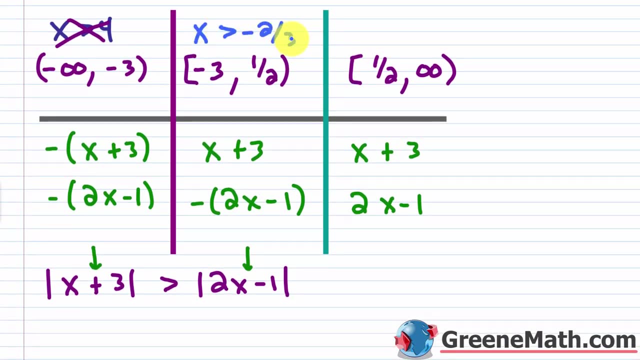 erase this real fast. x is greater than negative 2 thirds. Let me write that up here. So x is greater than negative 2 thirds. Okay, Is that in our interval, The interval is from negative 3, including negative 3, up to, but not including 1 half. Well, yeah, it is. So this is a partial 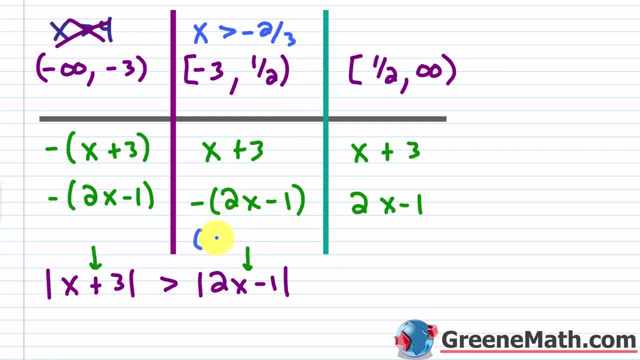 solution, Okay. So for right now I'm just going to write this guy as, again not including negative 2 thirds, because it's strictly greater than up to, but not including 1 half, Okay, And then we'll think about this solution And if we have a solution there, we'll have two partial 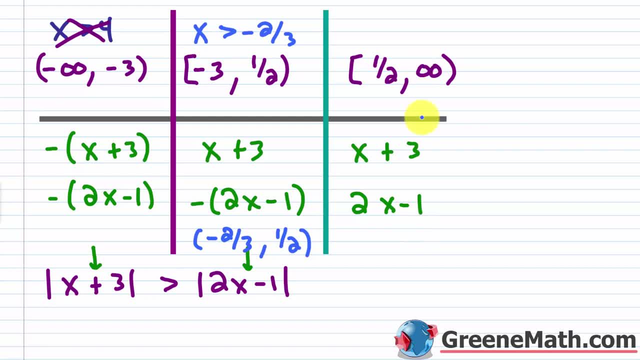 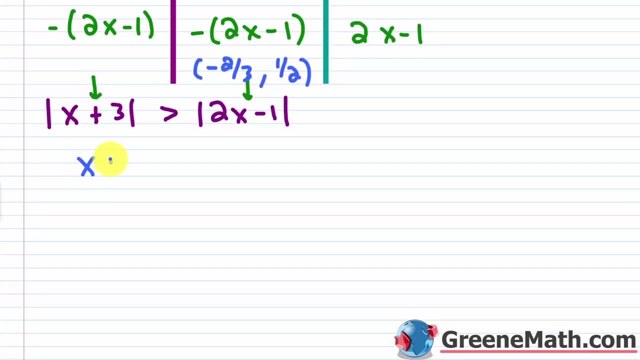 solutions we can put together as a full solution. Okay, So in this case everything's positive, So we can just drop the absolute value bars and go with what we have. So you'd have: x plus 3 is greater than 2x minus 1.. Let's subtract 3 away from each side of the inequality, So that would: 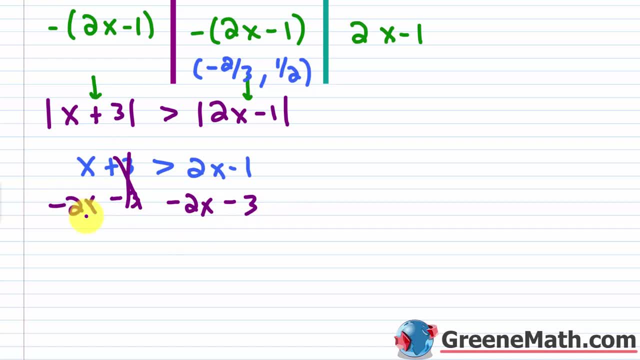 cancel. Let me subtract 2x away from each side of the inequality, So that would cancel. x minus 2x is going to give me negative x. This is greater than Negative. 1 minus 3 is negative 4. Let's divide both sides by. 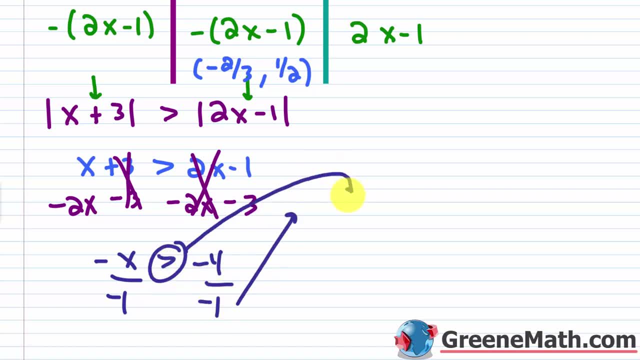 negative 1. So we know that this is going to flip right, So this is going to end up being a less than. So you have: x is less than positive 4.. Okay, So again, let me erase all this. So we say x is. 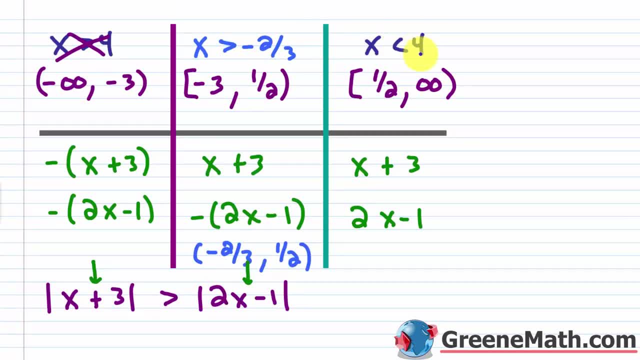 less than 4.. Does that fit in our interval? Yeah, it does Right, Because we have from 1 half out to positive infinity. x is less than 4 fits in there. You could basically say it's another partial solution. You would include 1 half and you would go up 2, but not include 4.. Okay, So if 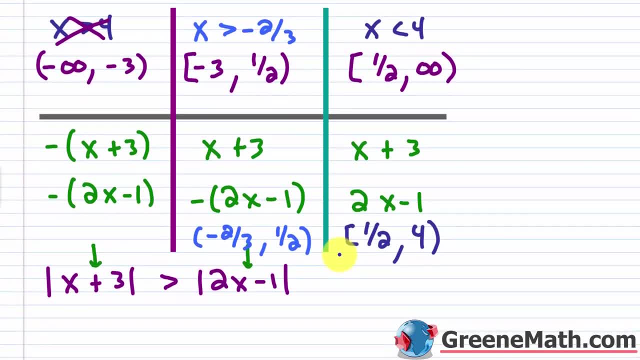 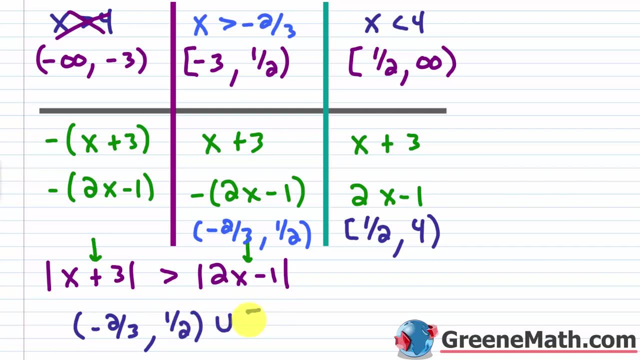 I take these two partial solutions and I just take the union of the two. So, again, from negative 2 thirds- not including that, up 2, but not including 1 half and the union width, you have 1 half which is included up to 4.. Okay, So this would be your solution set And basically, 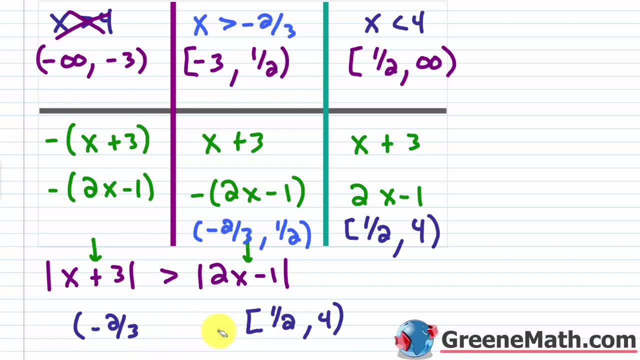 when you combine the two, you can get rid of this part right here and just kind of slide this down, And that's what you're going to get right. You're going to get from negative 2 thirds, not including that up 2. but 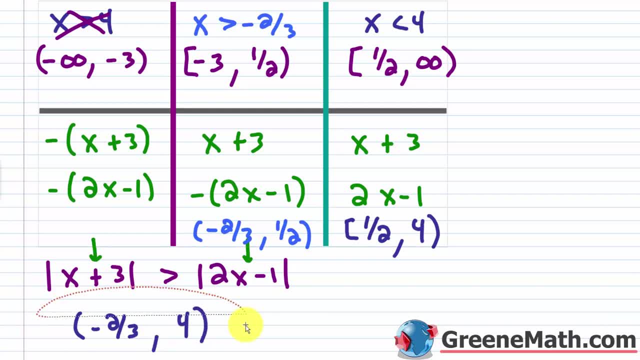 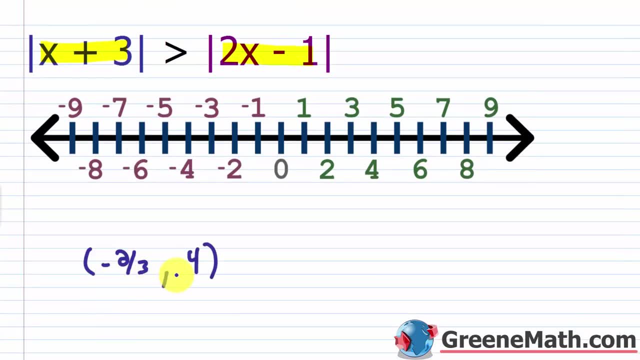 not including 4.. Okay, So let me kind of drag this up to our original page And we'll paste our solution here Again: from negative 2 thirds, not including that, up 2 and not including 4.. So negative 2 thirds. let's just go ahead and say that about right here, And I'm just going to mark that. 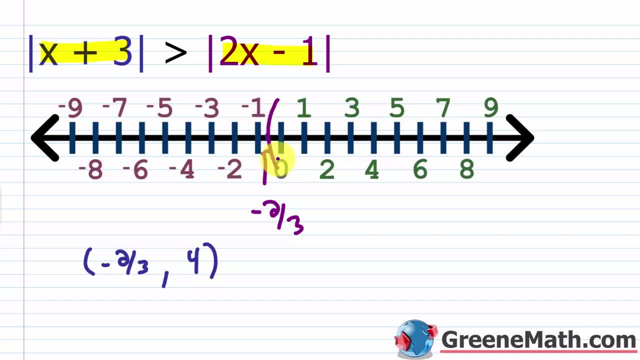 as negative 2 thirds. So I'd put a parenthesis there, because it's not included. 4 is not included. Just shade everything in between, Okay, And then we can also write this saying that x is greater than negative 2 thirds and less than 4.. Okay, So this is your interval notation. This is: 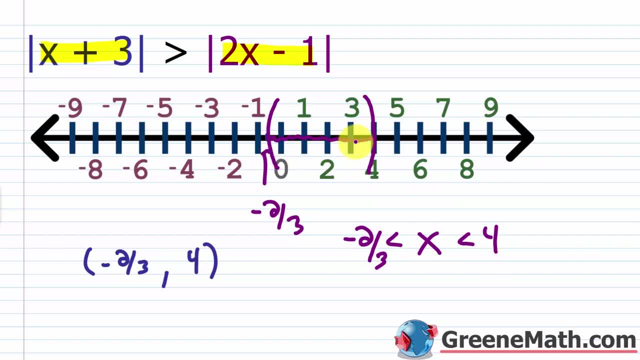 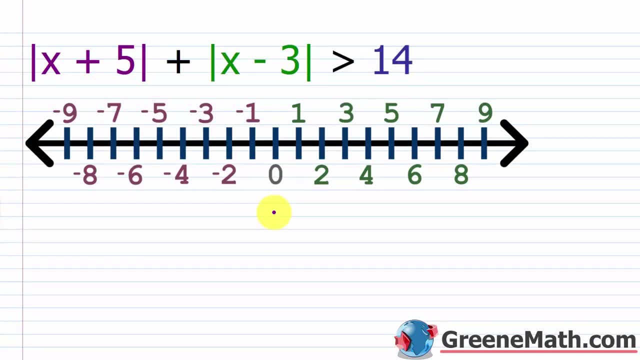 your standard notation. And then this is graphically So. those are the solutions. for again, the absolute value of x plus 3 is greater than the absolute value of 2x minus 1.. All right, let's go ahead and take a look at another example. 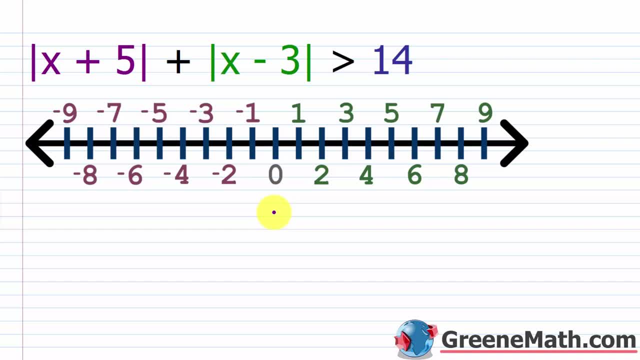 So this guy here is going to be a little bit more complicated, but we're going to solve it using the same strategy. So we have the absolute value of x plus 5. And then, plus, we have the absolute value of x minus 3.. And then this is greater than 14.. So the first thing we want to do is just take what's. 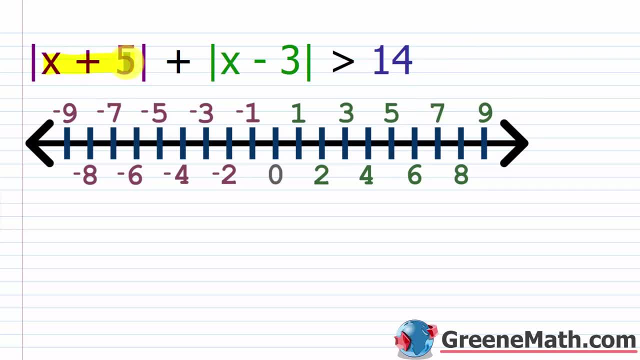 inside of the absolute value bars in each case. So this expression here: x plus 5.. And this expression here: x minus 3.. We just want to set those guys equal to 0 and see what the result is. So if we 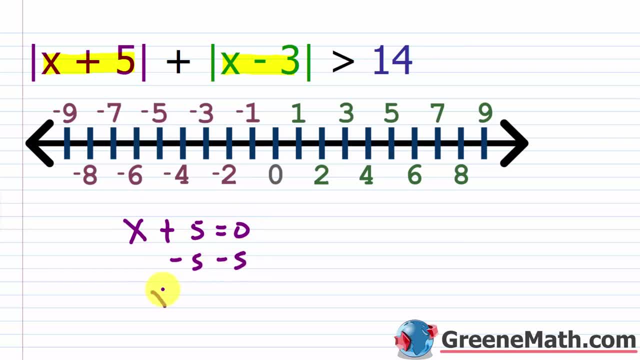 subtract 5 away from each side of the equation, we get x is equal to negative 5.. Then for the other guy we have x minus 3.. So x minus 3 equals 0.. Add 3 to both sides of the equation: We get x is. 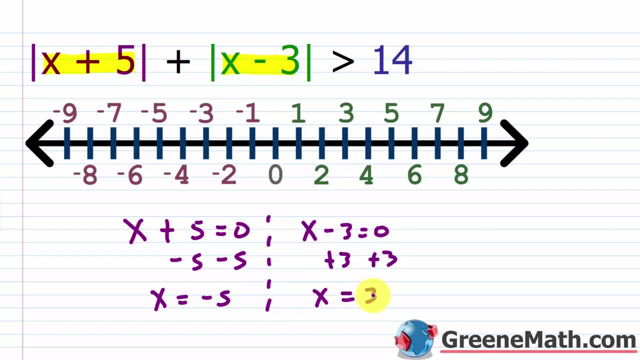 equal to 3.. So again, these two numbers are going to help me split the number, line up into kind of three intervals We're going to have from negative infinity to negative 5, with negative 5 not being included. Then we'll have negative 5 to 3, with negative 5 included and 3 not, And then 3,. 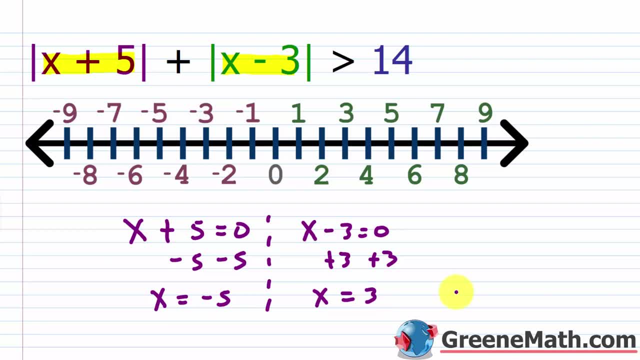 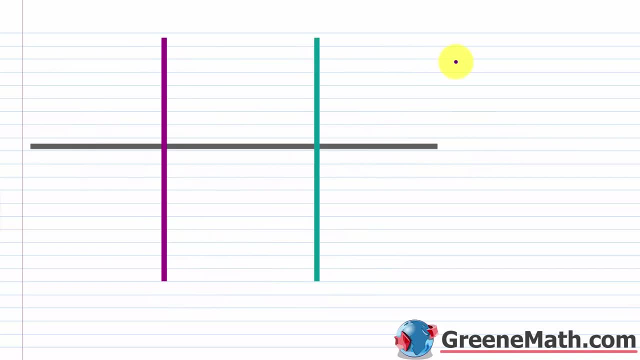 included and anything larger. Okay, so let's set this up using a table. Again, I don't like to use the number line itself, I like a little table. It helps me organize things. So again our numbers. I'm just going to write them here. We had negative 5 and positive 3.. So again from negative infinity. 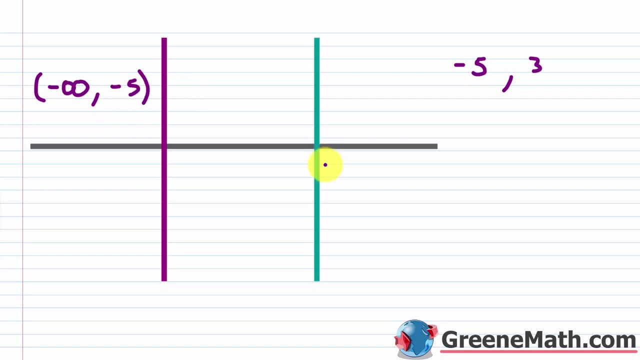 up to, but not including negative 5. And then negative 5 will be included here. So negative 5 is included, And then up to, but not including 3. And then 3 will be included And then out to positive infinity. Okay, so we're going to have negative 5 and positive 3. And then negative 5. 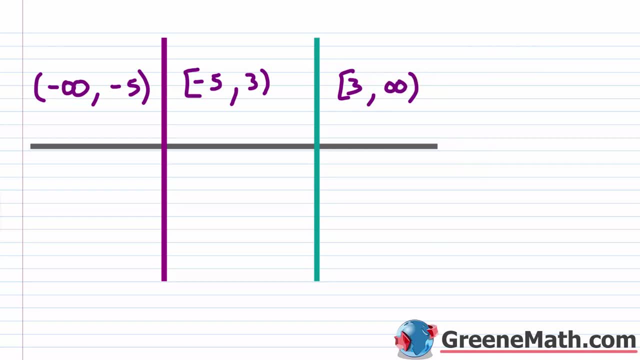 is included. Okay, so let's rewrite our inequality Again. if we go back up, we have the absolute value of x plus 5, then plus the absolute value of x minus 3. And this is greater than 14.. So let's. 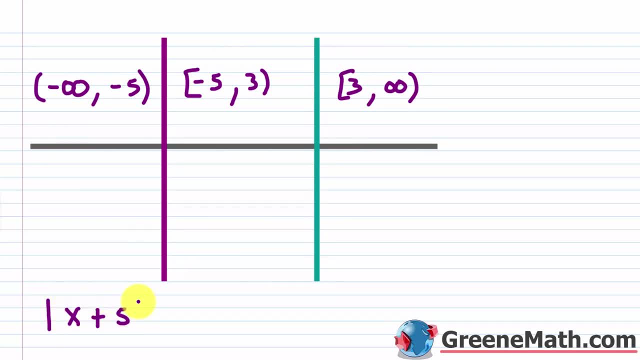 write that. So we have the absolute value of x plus 5. And then, plus, we have the absolute value of x minus 3. And this is greater than 14.. Okay, so we know, in this first interval, the one all the way to the left, where we're coming from: negative infinity going up to, but not including. 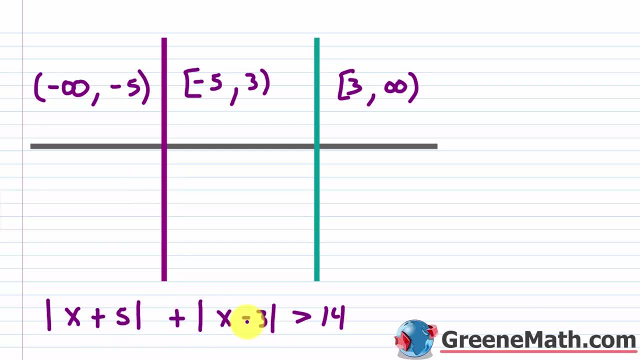 negative 5.. Both of these guys are going to be negative, right? So we're going to have negative infinity, And then we're going to have, so we're going to have negative infinity, And so we have the absolute value of x minus 3.. You can see this guy's negative And this: 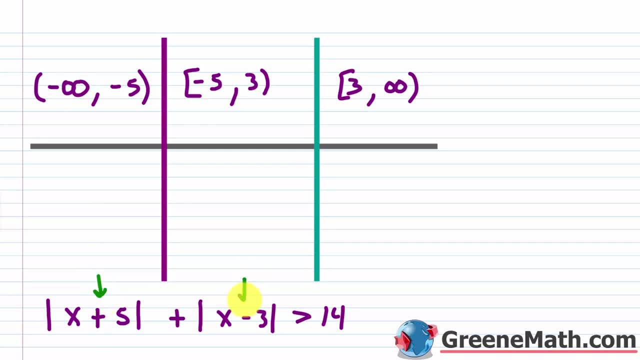 guy's also going to be negative. And then if we go back up, in fact it would be negative. All right, so we have x plus 3.. So now the absolute value of x minus 3 is equal to three. Okay, so that means we actually have negative 5, negative minus 3.. And again we can add: 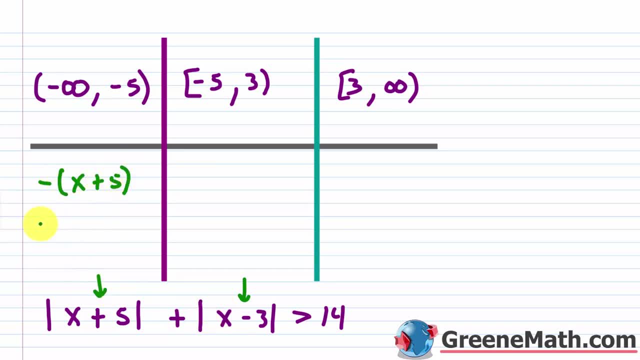 that to 0,. all right, because 1 times x will be just the derivative And it's the average taking any negative 5.. So 0 times 3 will be negative 4.. Okay, what we're going to run to three, but not including that. Well, now this guy right here, this X plus five, that expression. 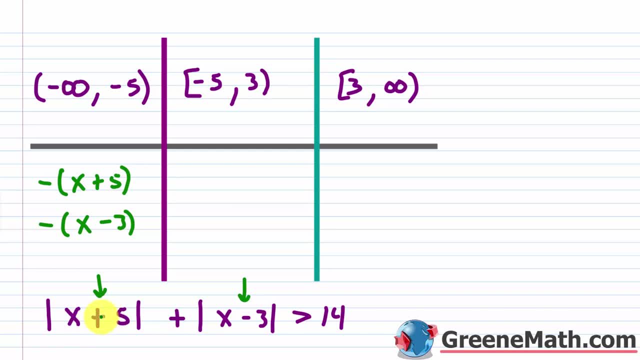 is going to be either zero or positive, So I can replace it with the expression itself. So we'll put just X plus five. And then this guy right here, this X minus three is still going to be negative, right? Because again it's zero. when X is three, we're less than three, So it's still. 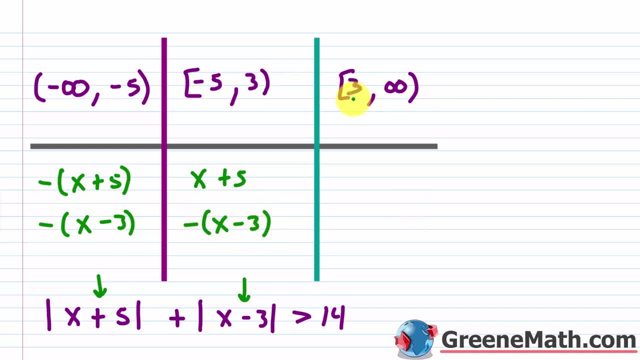 going to be negative. So we put the negative of X minus three. And then this last case where we're three or anything larger, well then this X plus five is going to be positive. And then for X minus three that could be zero or positive. So again, we just put X minus three there. Okay, So again. 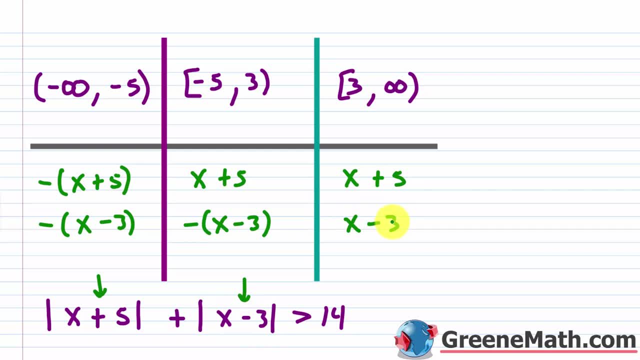 if it's zero or positive. you just take what's inside the absolute value bars and you can write that down. Basically, think about: just drop the absolute value bars If it's negative. well then you drop the absolute value bars, wrap it in parentheses and then put a negative out in front. 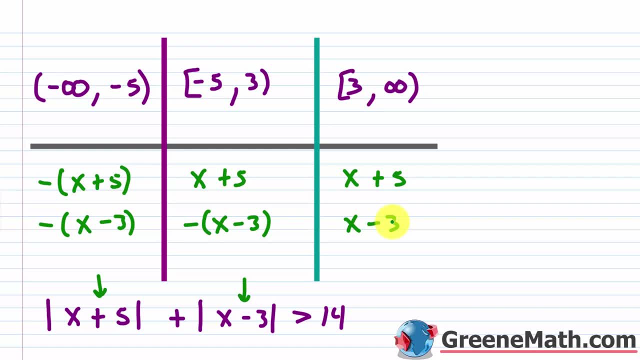 Okay, So that's all we're doing, All right? So let's go through the possibilities now. And you can see that we have a negative here. So let's go through the possibilities now. Again, this is the tedious part. So in the first case, both are negative, So I have the negative. 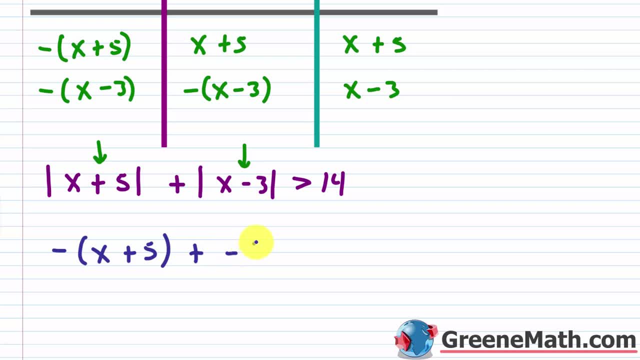 of X plus five, then plus the negative of X minus three, And you can just put the minus there instead of plus negative, doesn't really matter then greater than 14.. Okay, So I'm going to distribute this negative to each term. I'm going to have negative X minus five and then minus X. 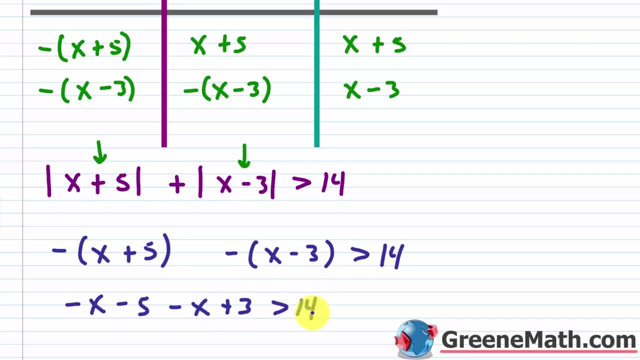 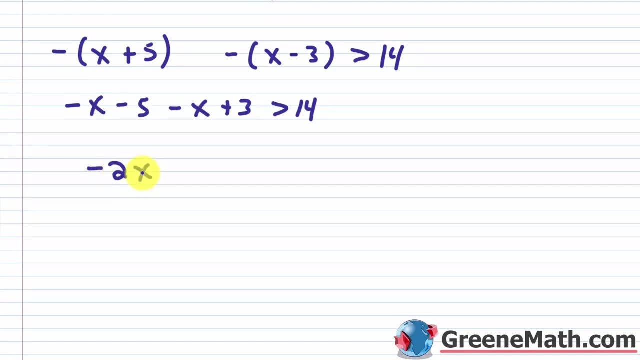 plus three, And this is greater than 14.. Let me scroll down and get a little room going. So I know that minus X minus another X is negative two X. I know that minus five plus three is negative two. This is greater than 14.. Let me go ahead and add two to both sides of the inequality We know. 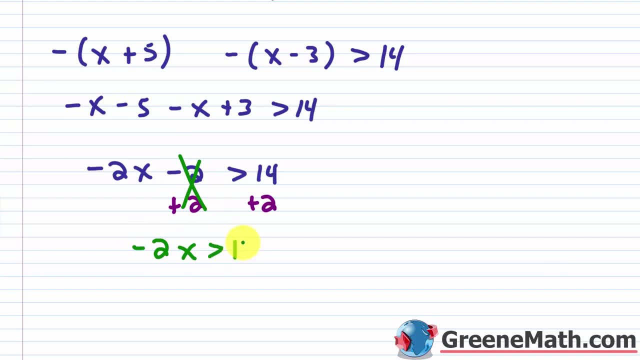 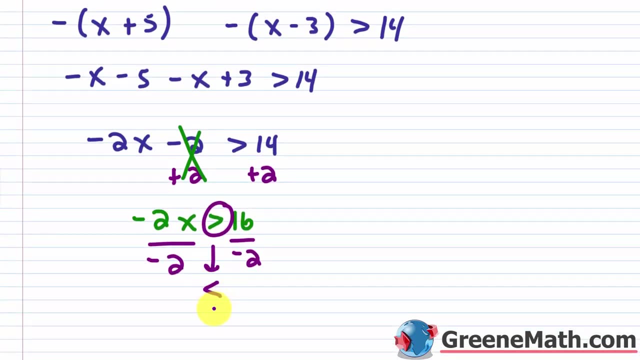 this will cancel Negative two. X is greater than 16.. So then, when I divide both sides by negative two- remember we got to flip this- So this becomes a less than now You'll have. X is less than negative eight. Okay, So X is less than negative eight. Is that in the end? Is that in? 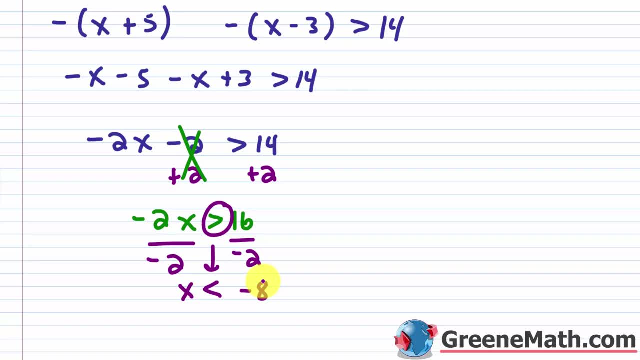 the interval that we're working in right now. Well, yeah, we said that our current interval is anything less than negative five. Negative eight is definitely less than negative five, So we're good to go right. This is going to be a valid solution for us, But, again, it's just part of. 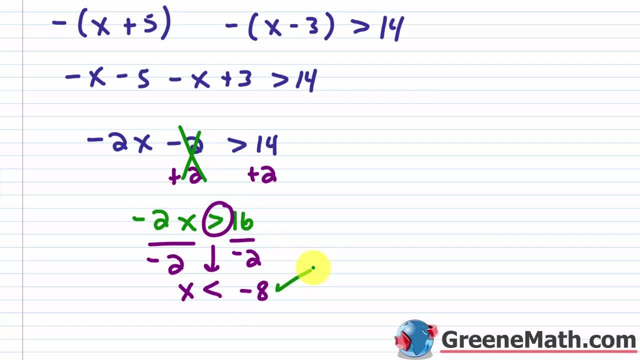 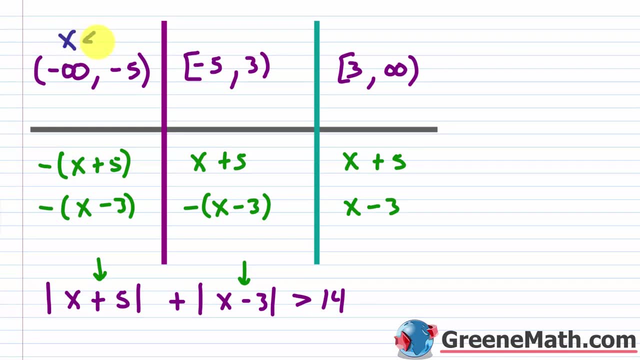 our solution, because we might have more to come. Okay, So we just consider it as a partial solution for now. All right, So let me erase all this. So again for this part, I said that X was less than negative eight, And I'm going to go ahead and just put a check mark there So we know that we accepted. 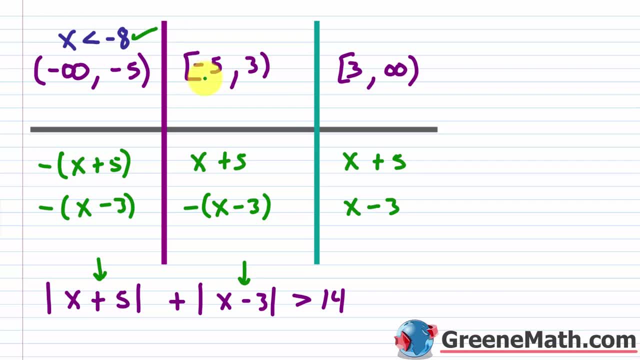 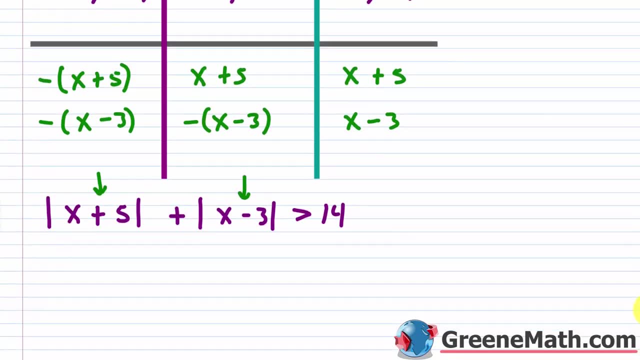 that solution. All right. For the next interval, again, from negative five and including that, up to, but not including three, this guy's positive, this guy's negative. So let's go ahead and do that. So X plus five, again that's positive, And then plus this, X minus three, that expression is going to be. 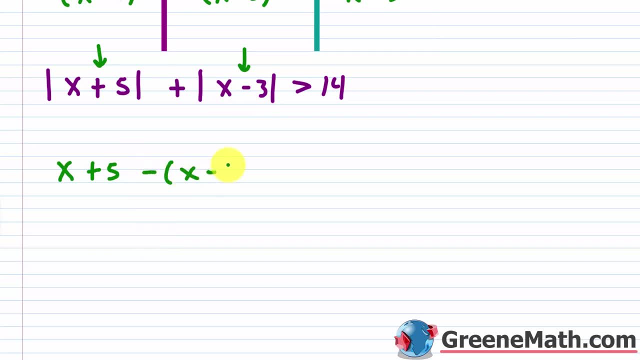 negative. So I'm going to put minus the quantity X minus three, And before we continue, let's just go ahead and distribute this So this would be minus X and plus three. make that a little quicker. Then this is greater than 14.. Okay, So X minus X, that's going to drop out. So this is gone. 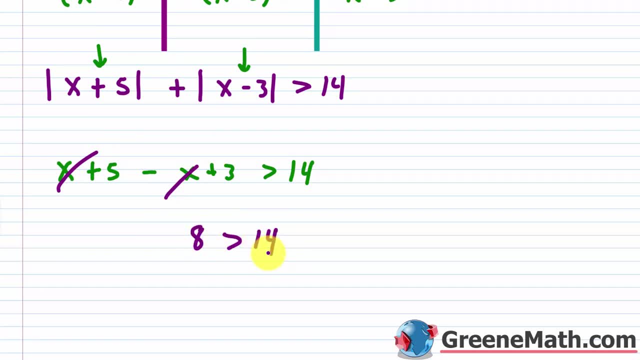 right, So you basically have that eight is greater than 14, which is false. Okay, That's never going to be true, So nothing's going to work in that interval. So you don't even have to put anything, You just say it doesn't work. All right, So the next one we're going to look at. 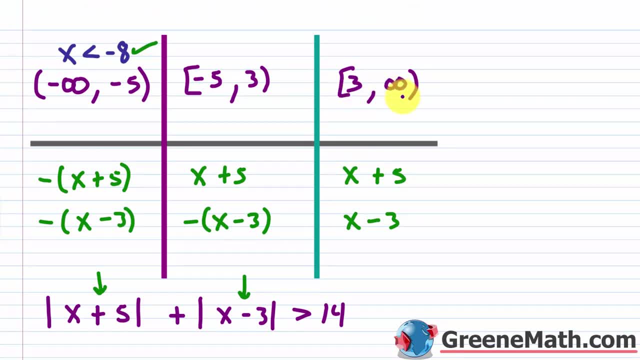 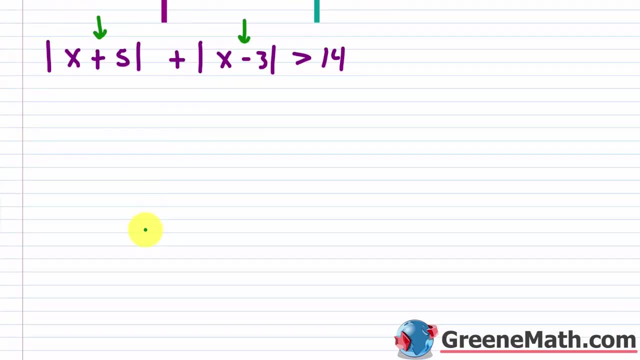 we have from three and including three out to positive infinity. And again both expressions are positive here, So we can just drop the absolute value bars in this case. So we just say X plus five plus X minus three is greater than 14.. So we just say X plus five plus X minus three is greater than 14.. 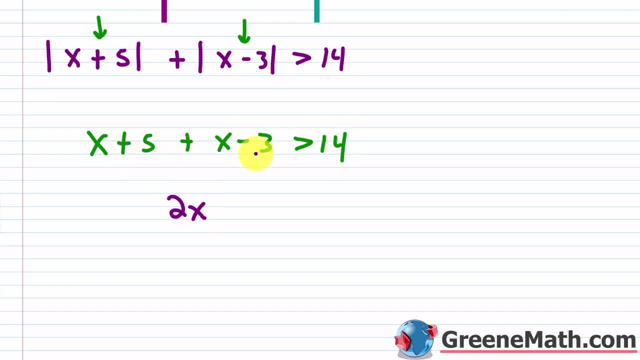 So X plus X is two X, and then five minus three is two. So plus two, and this is greater than 14.. All right, So let's subtract two away from each side of the inequality And then we can cancel this. We'll have two. X is greater than 12.. Let's divide both sides of the inequality by two. 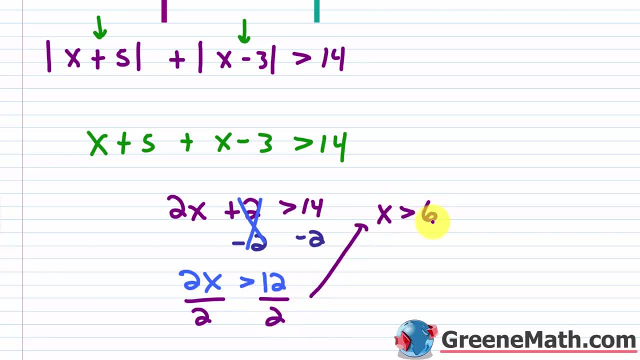 We'll find that X is greater than six. Okay, X is greater than six. Is that in our interval? Well, yeah, this interval is from three out to positive infinity. X is greater than six. That is in the interval, So we're basically good to go with that. 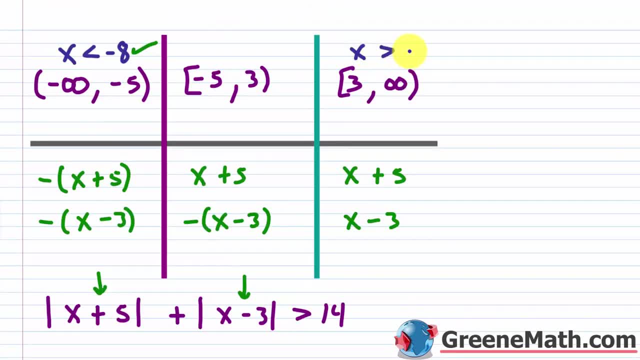 So let's erase this. We'll say: X is greater than six. Let me put a check mark there. So basically we would just combine these two as one statement. We would say that X is less than negative eight or X is greater than six. So let me just copy this real quick, Go back up and let me just paste this: 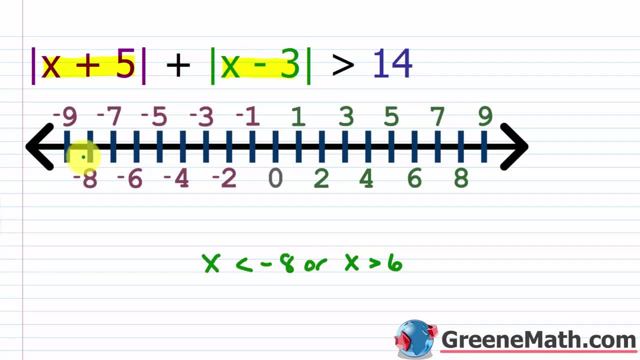 in. So again, X is less than negative eight, So find negative eight. So we're going to copy this negative eight. I'm going to put a parenthesis there, I'm just going to shade everything to the left. Or also, X could be greater than six, So find six. put a parenthesis there, shade everything to 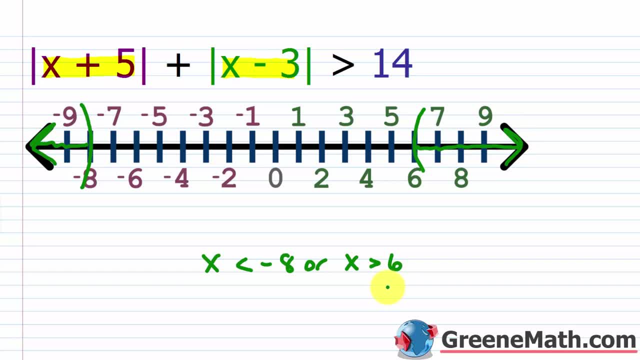 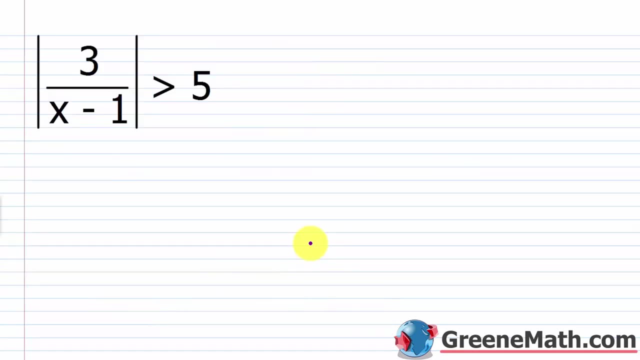 the right. Okay, In interval notation again, I could just say from negative infinity up to, but not including negative, eight and the union with anything larger than six, right, So in both cases I'm using a parenthesis to show that it's not included. All right, So let's kind of change. 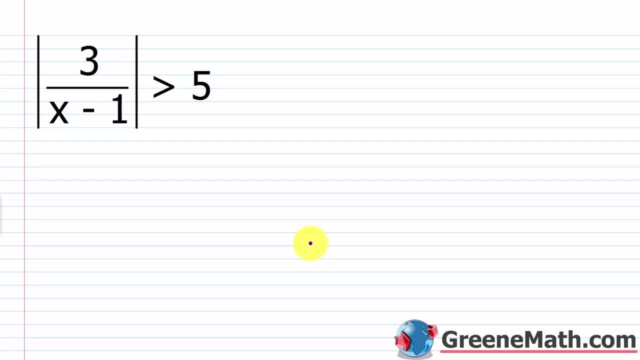 things up and look at another common type problem that you'll see in this section. So let's suppose we saw something like the absolute value of three over X minus one, and this is greater than five. So how can we solve this type of? 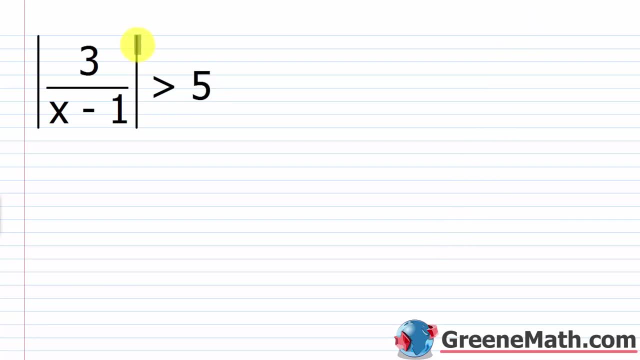 problem. Well, one approach that we can use. we realize that this guy right here, this absolute value operation, first and foremost, there's one of them and it's already isolated for us on one side of the inequality. So you have this absolute value operation and this is greater than five. 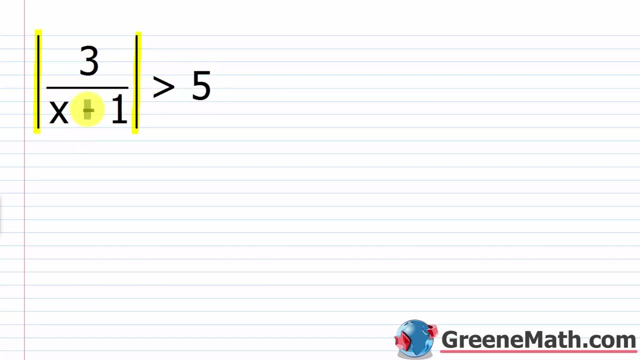 Okay, So for right now, don't even worry about what's inside of there. Just think about the fact that earlier in the lesson we said if we had the absolute value of x- and this is greater than some positive real number, a- this led to x being 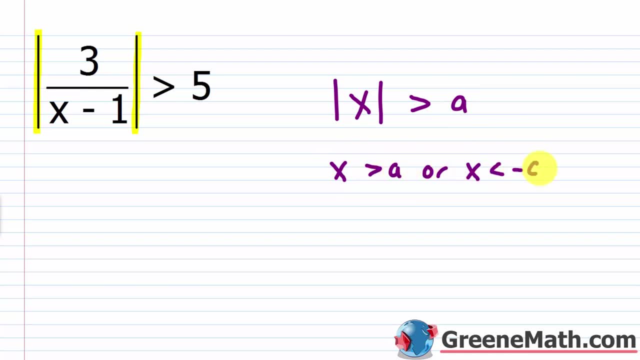 greater than a or x is less than negative. a right. We saw this with our example. we said: if the absolute value of x was greater than seven, we said x was greater than seven or x was less than negative seven. Okay, so this should be pretty crystal clear at this point. Now the thing is: 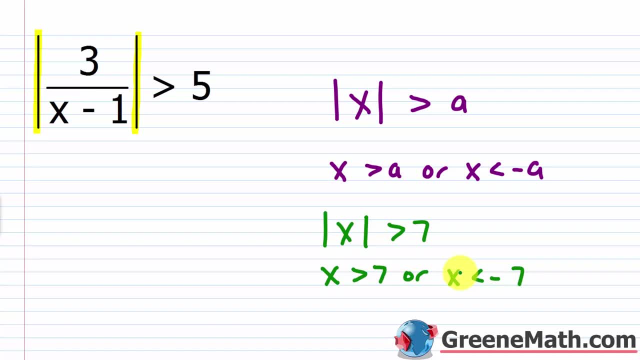 you can do this if you have a more complex expression inside of the absolute value bars. Okay, so I can replace this x with something generic like u. We'll just say u is some algebraic expression, So it could be a rational expression like we have here. It could be a quadratic. 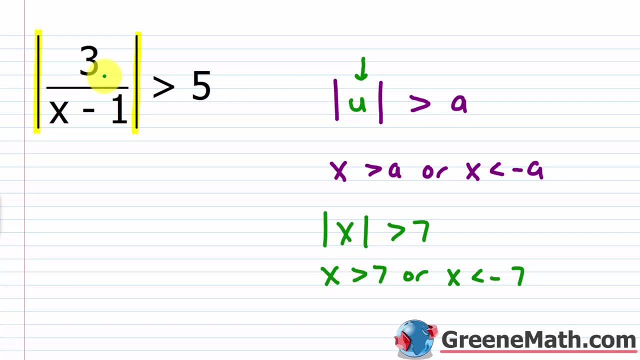 expression. It could be something more complicated than the typical linear expression that you're working with when you solve basic absolute value inequalities. So what I can do is erase this and erase the x and just put a u there. Okay, so it's the same kind of concept, It just takes more time to solve it. It's just going to. 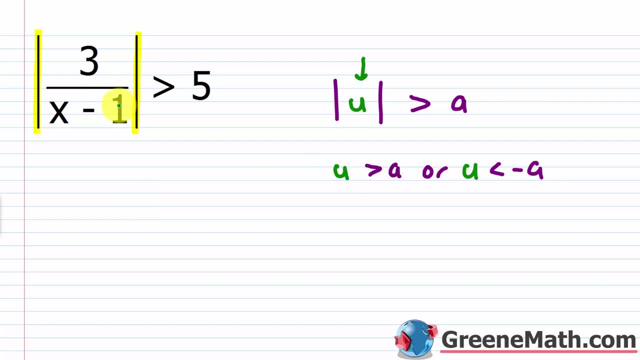 be way more tedious. Okay, so let's use this to set this up. So, basically, I'm going to take my rational expression inside the absolute value bars and I'm going to say three over x minus one, Since I have a greater than I'm going to say it's greater than this positive number five. 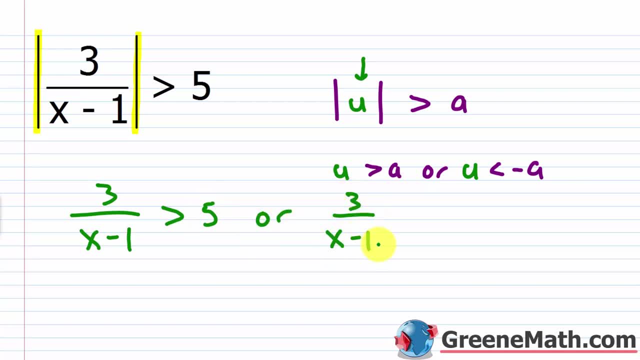 then, or I'm going to say three over x minus one, I'm going to say is less than the negative of five. Okay, I just use this rule here. That's all I did. Okay, so let me erase this. we don't need this anymore. So, basically, at this point, 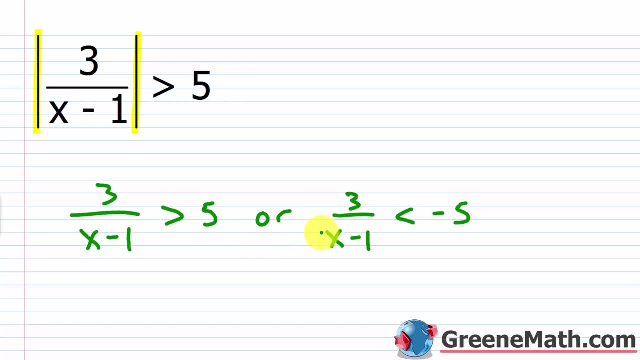 all we need to do is solve two rational inequalities and then kind of combine our two solution sets that we have. So I'm going to start out with this one right here, So I'm going to copy this. we're going to go down to a fresh sheet, Alright, so let me just paste this in here. 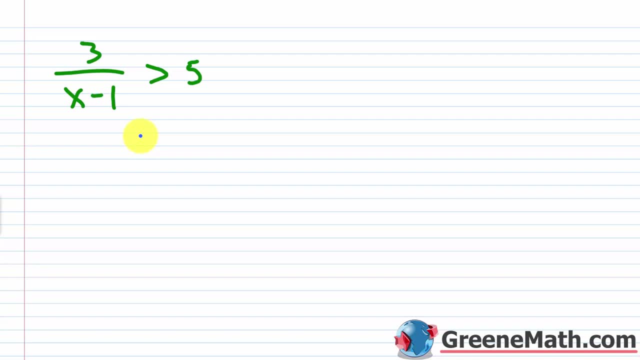 And I want you to recall that the very first thing you want to do when you're solving a rational inequality is get it in the format where you have a single rational expression on one side and zero on the other. Okay, so the way we're going to do this is we're going to go to the 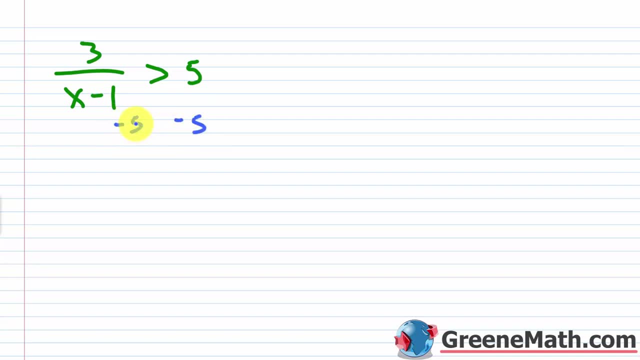 we're going to do that here is we're just going to subtract five away from each side of the inequality, And so this would cancel and become zero. So essentially I would have what I would have: three over x minus one, and then we'd have minus five and this is greater than zero. Okay. 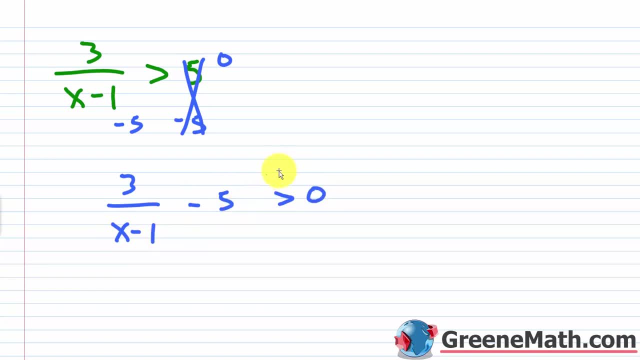 So now I want to get a common denominator going. let me just kind of slide this down a little bit, And what I'm going to do is just multiply this by the quantity x minus one and then over the quantity x minus one, So now I'll have a common denominator negative five times. 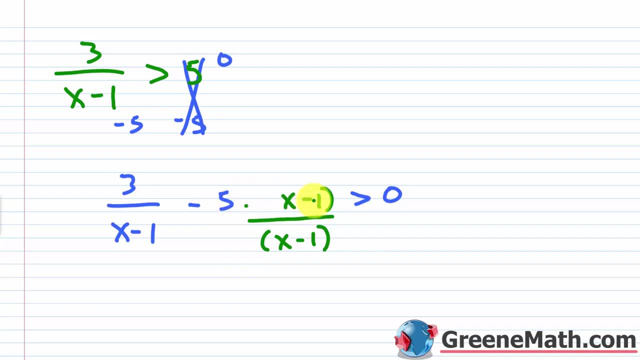 x is negative five x, and then negative five times negative one is going to be plus five. Okay, So kind of continuing. now I have a common denominator So I can just combine the numerators. So we have three. And then let me make this more clear: This is negative five x. 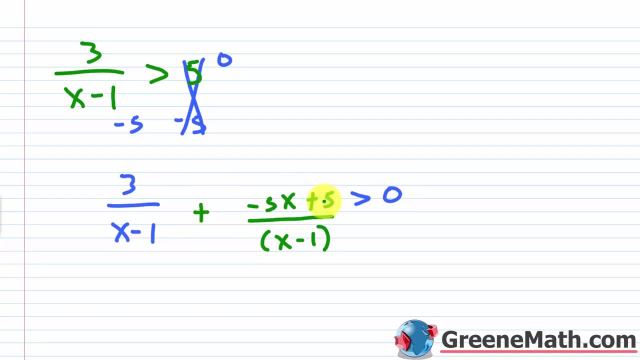 And I'll just put a plus here. So we have three plus five, which is eight. okay, you have eight and you have your negative five x. So let me write negative five x plus eight as the numerator, And this is over the common denominator, which is x minus. 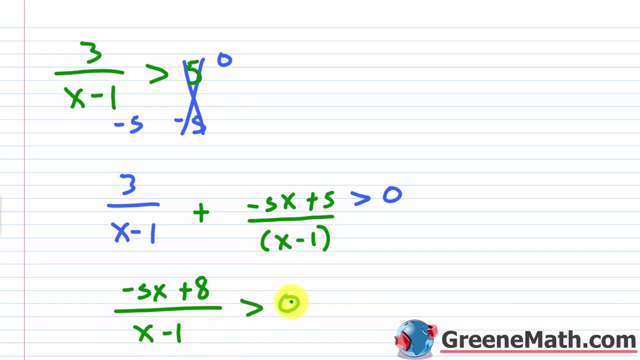 one, and this is greater than zero. Okay, So now we've accomplished kind of the first task. we have a single rational expression on the left side in this case, and we have zero on the other. Okay, So the next thing we want to do is find out where the critical values are. 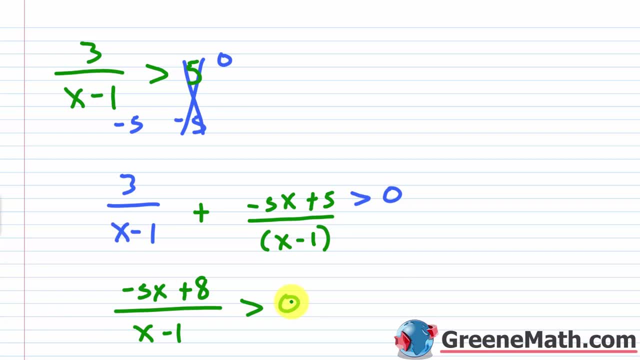 or some people call them endpoints or boundaries, whatever you want to call them. Okay, I'll just say critical values. So that is going to occur: where the numerator is going to be zero and where the denominator is going to be zero, I would take this numerator, which, in this case, is negative five. 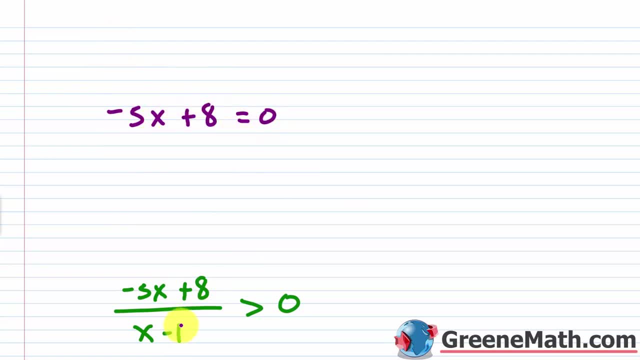 x plus eight and I would set it equal to zero. So that's one of them. Then I would take the denominator, which is x minus one, set that equal to zero. So both of those guys. when we solve that, the two solutions there are the critical values or again endpoints, So let me add one to both. 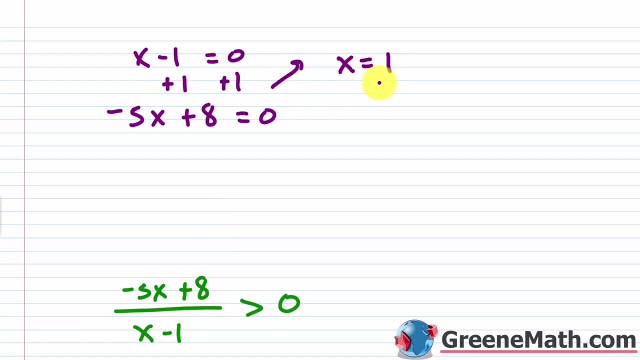 sides of this equation. That gives me x equals one. So that's one of those guys. Let me subtract eight away from each side of this equation. This is going to cancel. You'll have negative five. x is equal to negative eight. Divide both sides by negative five. 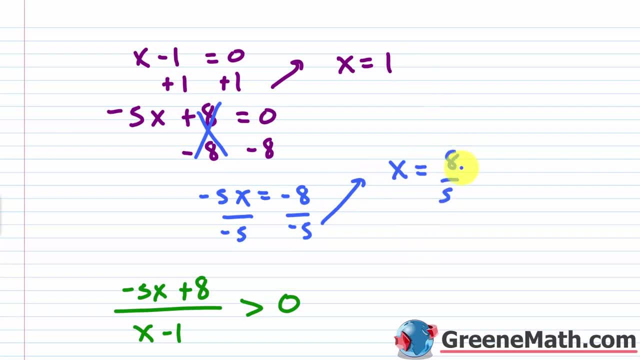 You're going to get that x is equal to eight fifths, So these are our two critical values. So we're going to use that to split the number line up into three intervals. So basically you'll have from negative infinity up to, but not including one, and then between one and eight. 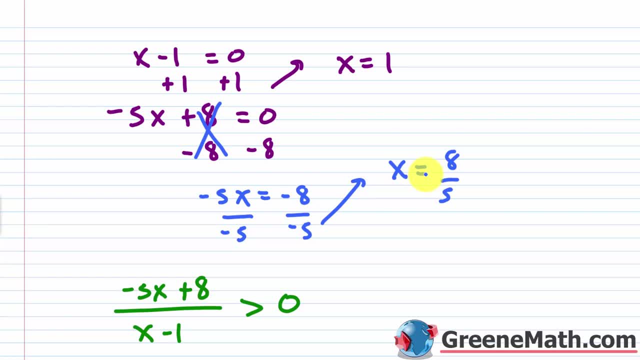 fifths- right, Neither is included. And then anything greater than eight fifths- Okay, So those are the three intervals you're going to have. You're going to pick a number in each interval. Okay, You're going to test that number in the original inequality You're going to see. 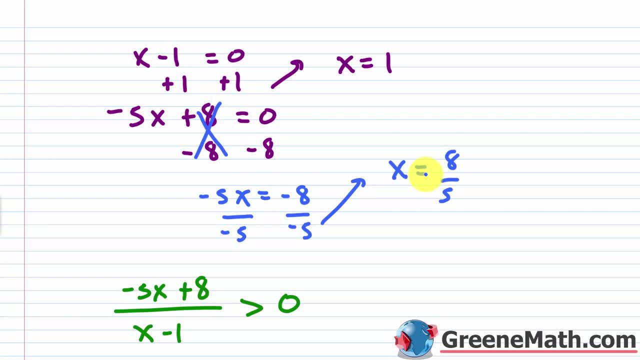 if it satisfies it. If it does that interval works, It's part of your solution set. If it doesn't, it gets rejected. It's not part of the solution set. So you can use a table for this if you want, or you could do a number line For these. I prefer to actually use a number line. 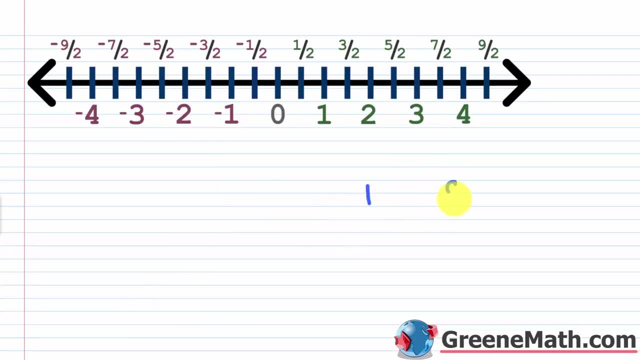 So let's do that All right. So the critical values: again we have one and we have eight fifths, So one is right here. So let me just draw a nice little vertical line, and it won't be perfect, but we'll put that in there. And then eight fifths is 1.6.. Now I've kind of divvied. 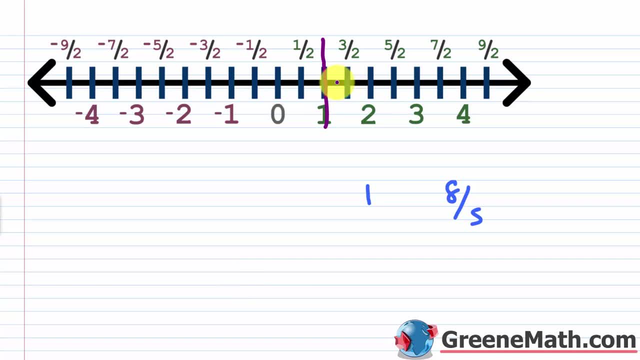 the number line up in a different way, You'll see that the notches here are separated by 0.5 or a, so from one we go to 1.5, or you could say three halves, So eight fifths again is 1.6.. If this is, 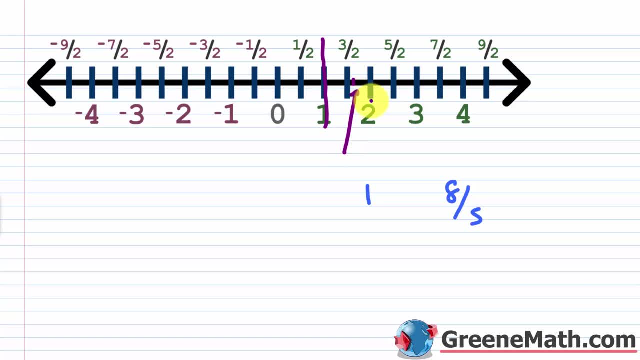 1.5,, 1.6, let's just say it's about right there. Let's say this is eight fifths. Okay, So let's go ahead and put another kind of vertical line there. We're going to divvy up the number line and just. 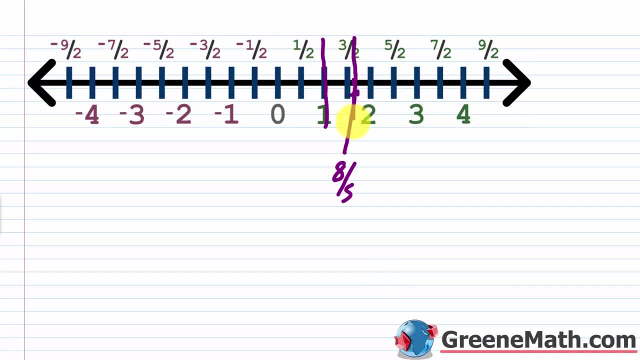 basically say that. let me kind of make that a little better. We'll say that this is interval A, basically anything less than one, anything between one and eight fifths, we'll call that interval B, and anything larger than eight fifths we'll call that interval. 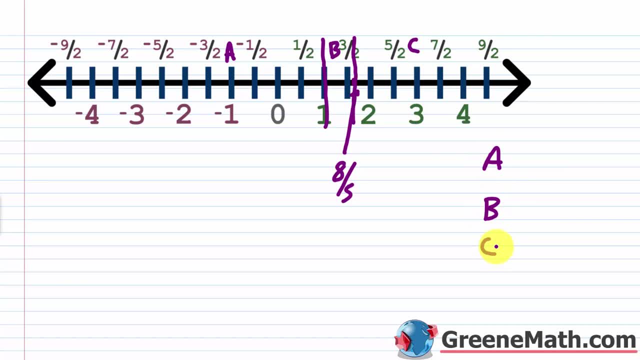 C. So we'll have A, B and C. So the original inequality was three over X, minus one is greater than five. So just take values in each interval, check them see if they work Again. if they do, it's part of your solution. If they don't, it's not part of your solution. Very, very easy. 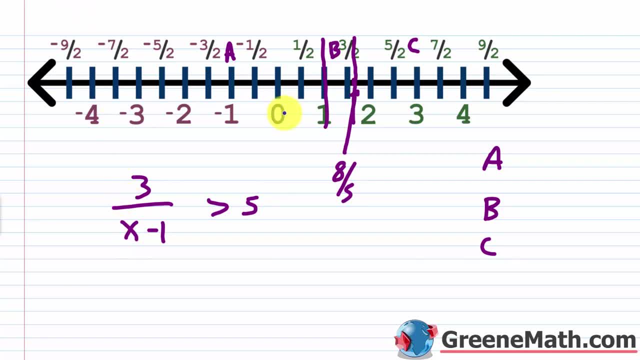 just a very tedious process. So from interval A I'm going to pick zero. plug that in there. Zero minus one is negative one. So three over negative one. Is that greater than five? No, this would end up being negative three. Negative three is certainly not greater than five. 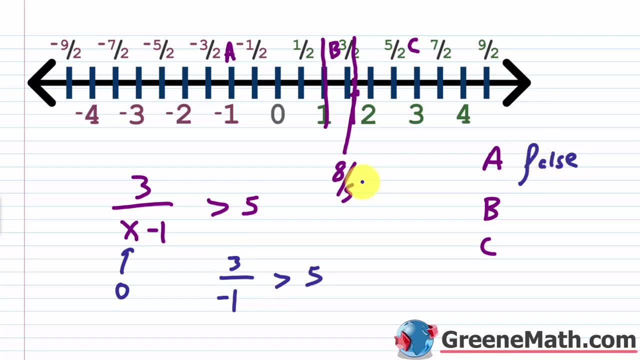 So this is false. right, In interval A, nothing's going to work. So for interval B again, I'm between one and eight fifths, or between one and 1.6. I think the easiest number to use there would be 1.5. So let's go ahead and plug in a 1.5 there. 1.5 minus one would be 0.5. So you would. 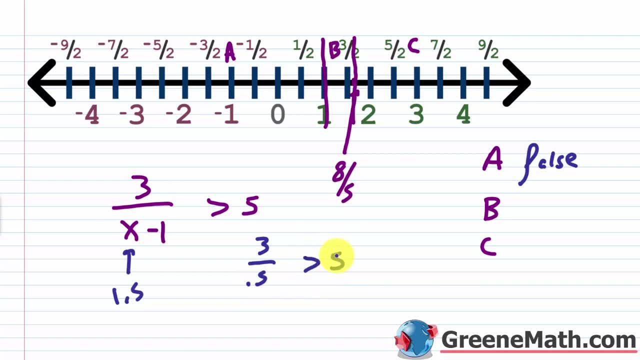 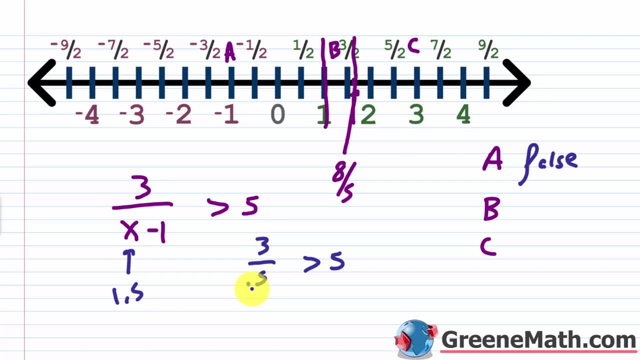 multiplying three by two. right, If you divide three by a half, you could say: when you crank that out, you get three times two, which is going to be six. Is six larger than five? Yes, it is So, this is true. All right for the last one. let's take a look at something in interval C. I'm going 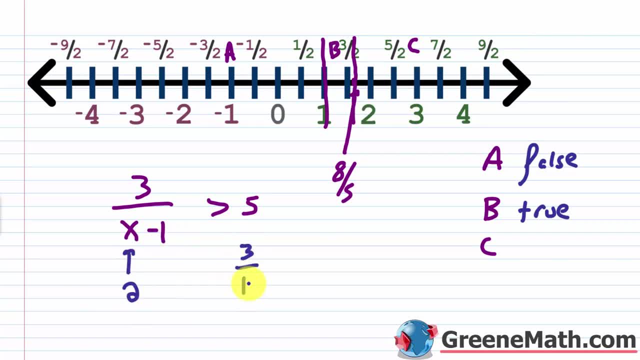 to pick two. So two minus one is one, Three over one is three. So you basically have that three is greater than five, Which is false. Okay, Let me write that a little better. So false, Okay. So only numbers, or only? 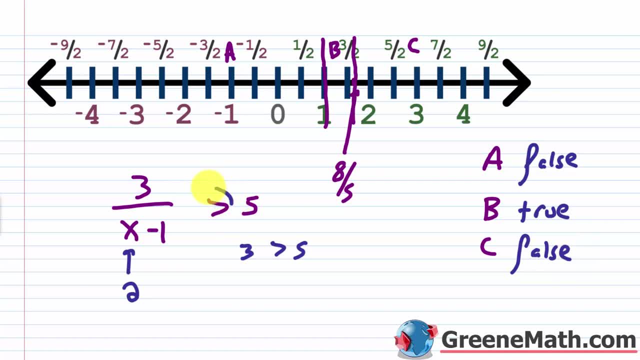 values in interval B are going to satisfy this inequality. It's a strict inequality, So the end points we don't even need to consider. Okay, They won't work, They will be excluded. So the solution for this part is going to be anything larger than one up to, but not including. 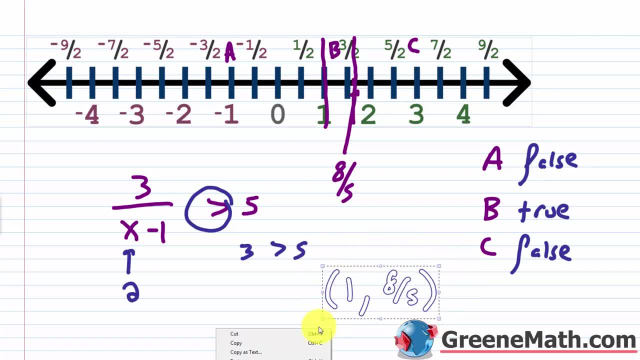 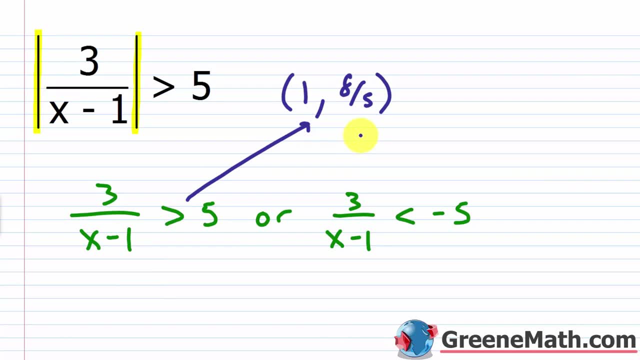 eight bits. So let's just copy this and we'll go back up And again, this is just going to be a partial solution. So this is for this one, And we could really write that X is greater than one and it's less than eight fifths. Okay, So this is just a partial. 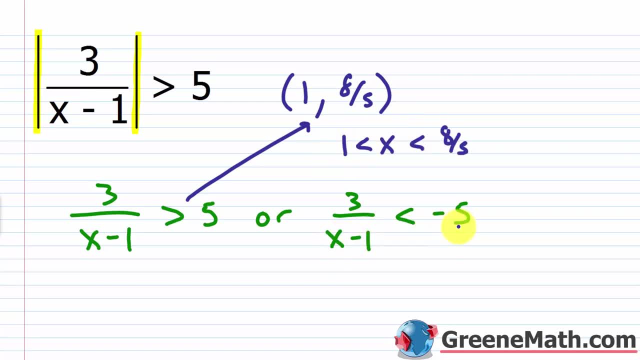 solution. We're going to work on this guy now and see what else we can find. So let's copy this and let's go down. All right. So let's paste this other scenario here We have three over X minus one, and this is less than negative five. So again, I want to get one rational expression on one side. 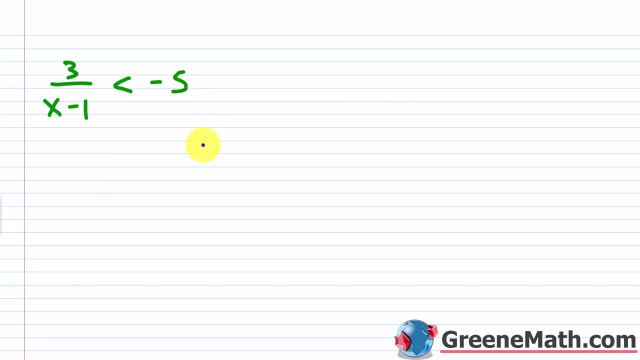 action and zero on the other. So same process as last time. So I'm going to add five to both sides of inequality. I'm going to have that three over X minus one, then plus five is less than zero. I'm going to get a common denominator. So let me again move this down. 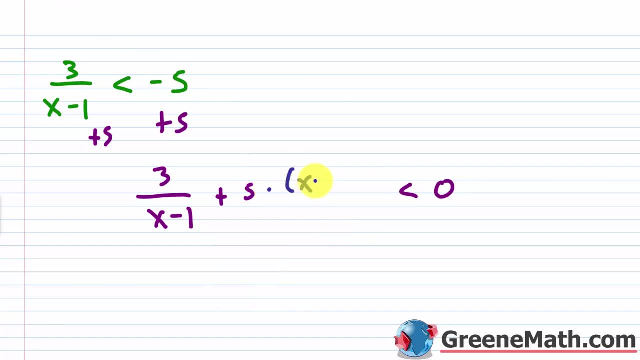 So I'm going to multiply this by X minus one over X minus one, And this is going to lead to three over X minus one. Plus, you have five times X, which is five. X, and then minus five times one is five, And this is over X minus one. Okay, Then this is less than zero. 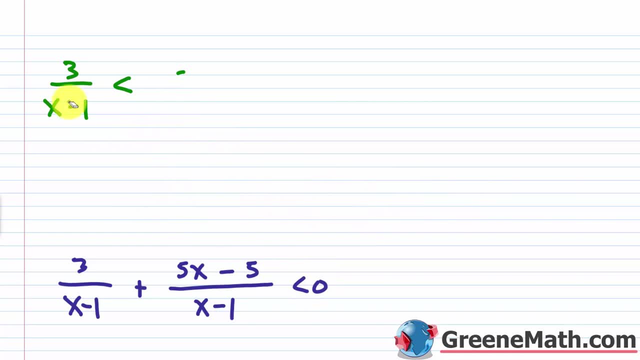 So let me erase this and we don't need this for right now. We'll write it again when we need it. So let me just drag this up and we make that three a little bit better. Okay, So now we're just going to kind of combine the numerators. We have a common denominator, So we'd have five X. 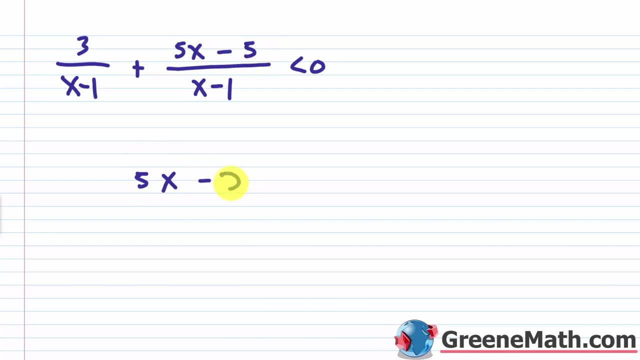 and then three minus five is negative two, So minus two. this is over X minus one And this is less than zero. Okay, So at this point again, I want to take my numerator, set it equal to zero. take my denominator, set it equal to zero. That will give me the two end points or critical values. 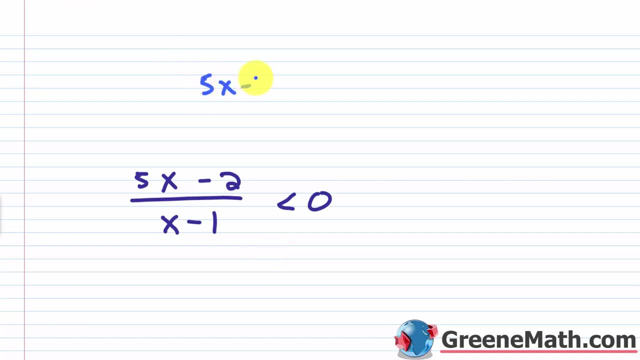 or boundaries. Okay, So we would have five X minus two is equal to zero. add two to both sides of the equation. I'm going to get that five X is equal to two. We would divide both sides by five and find that X is equal to two fifths. Okay, So that's one critical value, And then X minus one. we know if 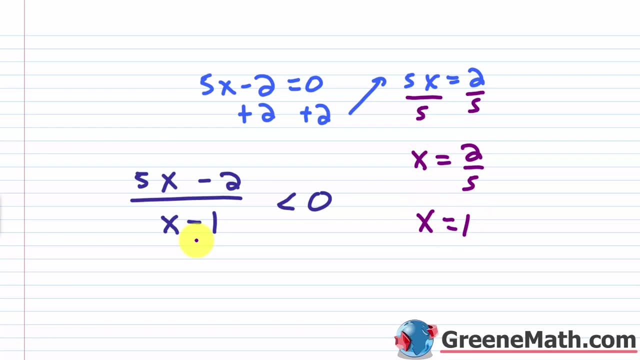 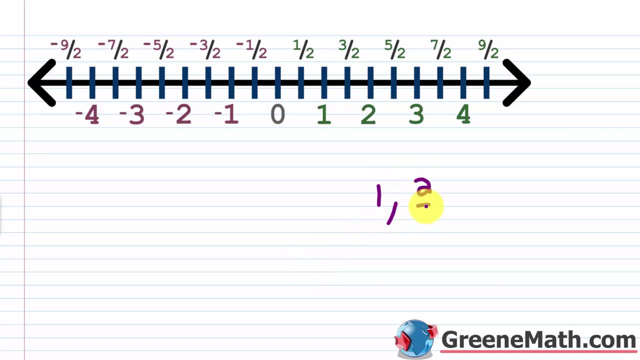 we set that equal to zero, We would get that X equals one. right, We solved that earlier. Okay, So let's go up And again the two critical values. we have one, and then we have two fifths. Okay, So one is right here. 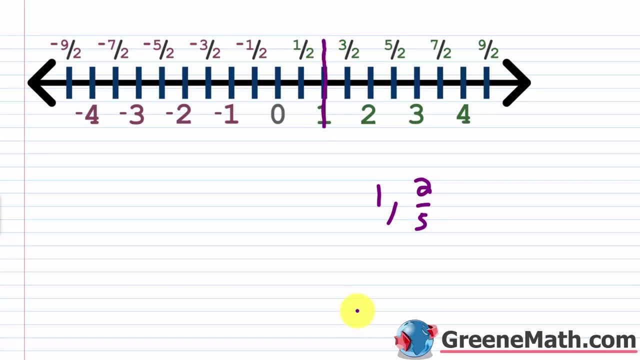 Let's just put a vertical line there. Two fifths in decimal form is 0.4.. So I have a notch for one half 0.4 would be just a little bit less. So let's just say it's right there. So this is. 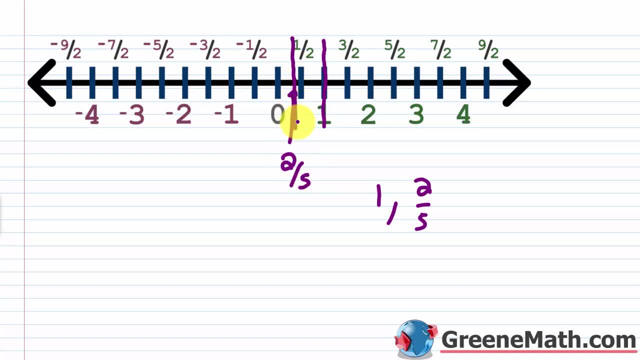 going to be my two fifths. Let me just put a vertical line there. Okay, So we have interval A, interval B and interval C. Again, interval A, in this case, is going to be anything that's less than two fifths, Interval B will be between two fifths and one, and interval C will be anything. 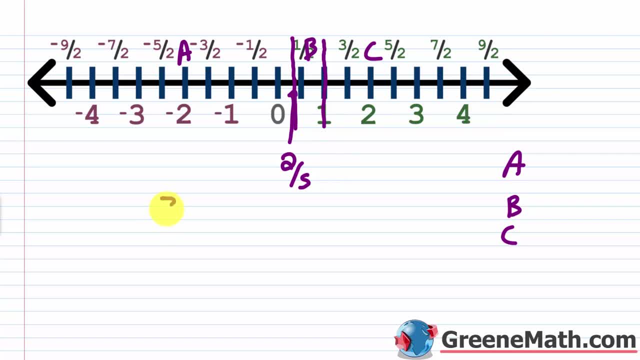 larger than one. So the inequality we're working with is three over X minus one, and that's less than negative five. So let's choose a number from interval A. Again, I'm going to choose zero, because it's easy to work with. So zero minus one is negative one. You would have that three. 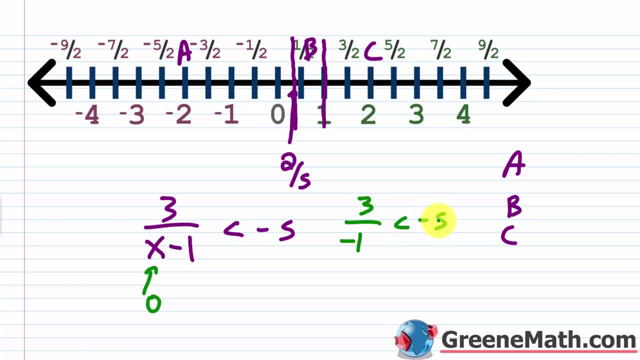 over negative one is less than negative five. That's going to be false, right? This would be. negative three is less than negative five. Negative three is a smaller negative value than negative five, So it's actually a larger number, right? So this is going to be false, Okay. What about for interval B? Well, it's kind of a. 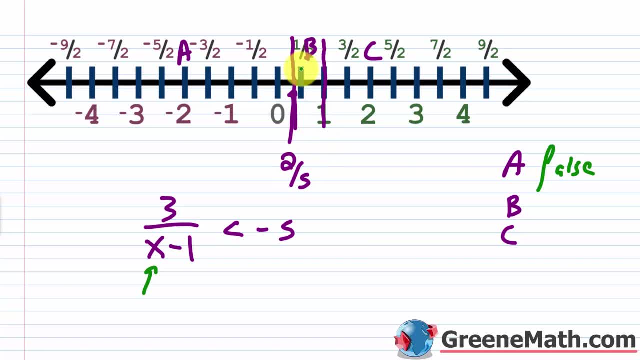 tight window, but between two fifths and one you can use one half. So if I do 0.5 there, I'm going to have 0.5 minus one, which is negative 0.5. So I would have three over a. 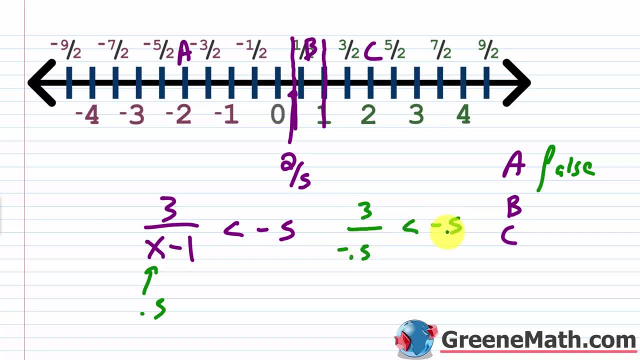 negative 0.5. And this is less than negative five. Of course, if I divide three by negative 0.5, it's like multiplying three times negative two. So this would basically be negative six. here Negative six is a larger negative than negative five, So it is less than negative five. So this: 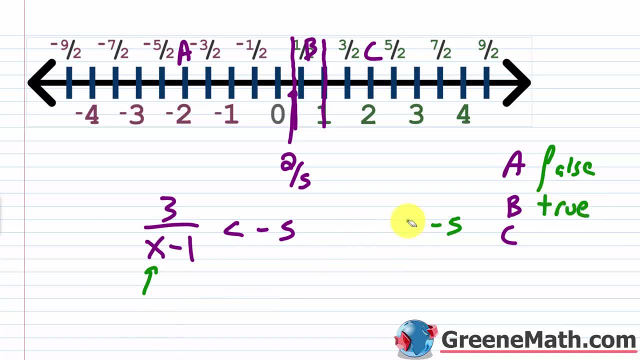 is true. Then for interval C, again, I'm just going to choose two. Nice and easy to work with. two minus one. So I'm going to choose two minus one. So I'm going to choose two minus one. So one gives me one. so i would have that three is less than negative five, which is obviously false. 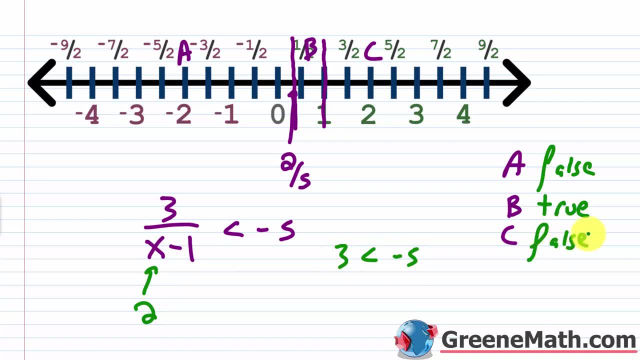 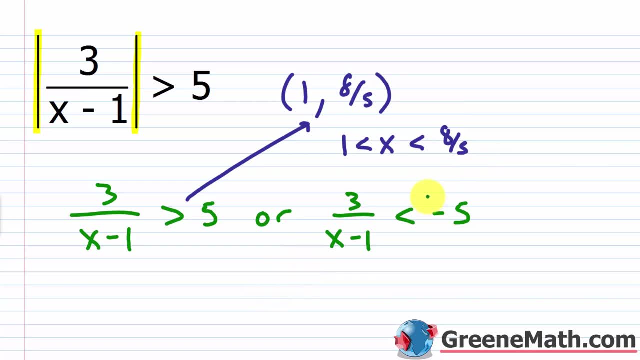 okay. so my solution here is going to be, for interval b, anything between two-fifths and one. so between two-fifths and one. okay, so for this guy, my solution is again between two-fifths and one. so now it's going to be the union of these two solution sets. so let me erase this. i don't need. 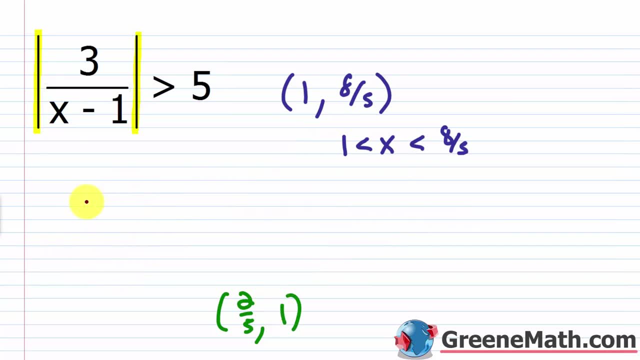 any of this anymore, because i'm thinking about the problem as a whole now. so i'm just going to start with this one. so i'm going to say between two-fifths and one. again, neither is included. and the union with this guy, which is between one and eight-fifths, neither is included. okay, now you. 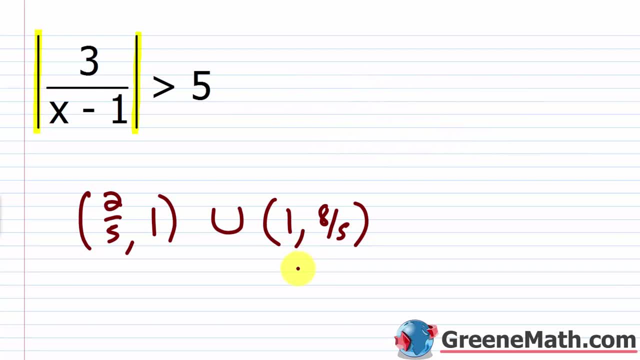 could also write this with our kind of standard way, using that: or we can say that x is going to be greater than two-fifths and less than one, and then or you have this solution. so you have that x is going to be greater than one and less than. 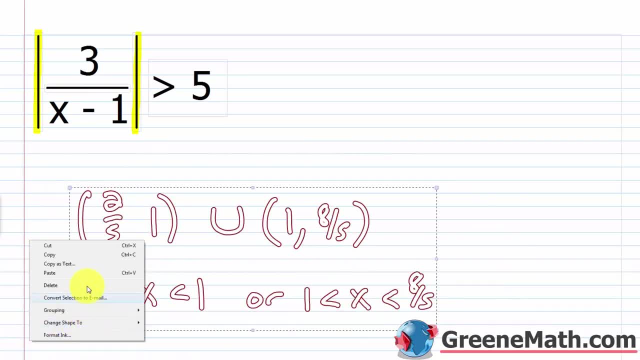 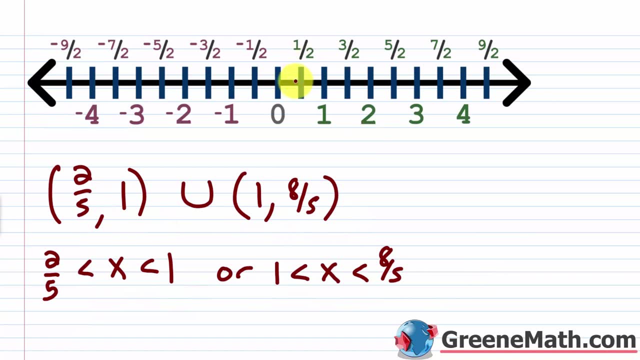 eight-fifths. okay, so let's copy this and go to the number line. we'll make a nice little graph to finish this off. all right? so the first thing i'm going to do is just make a little notch for two-fifths. so again, that's 0.4. so i'm going to put it right there and just say this is two-fifths. 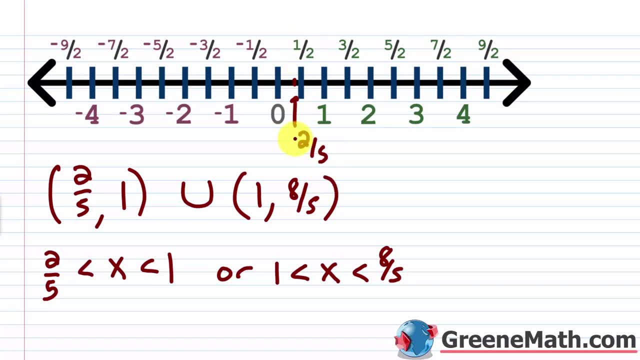 again, this value here for this notch is one half. so two-fifths would be less than that. then for eight-fifths i'm going to say again: that's 1.6 as a decimal. so three halves is 1.5. so it's going to be a little bit more than that. so let's say it's right there. so this will be my 8: 5.